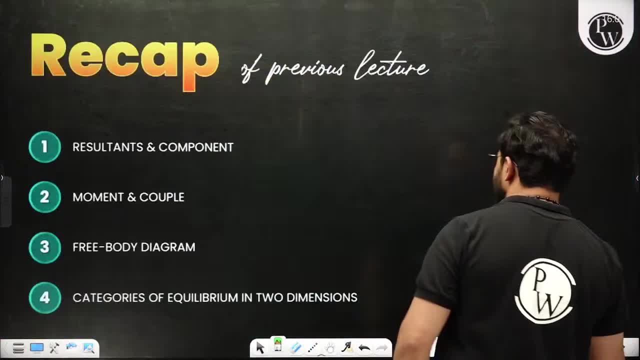 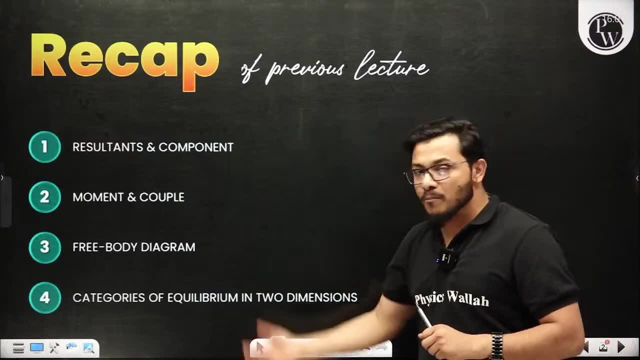 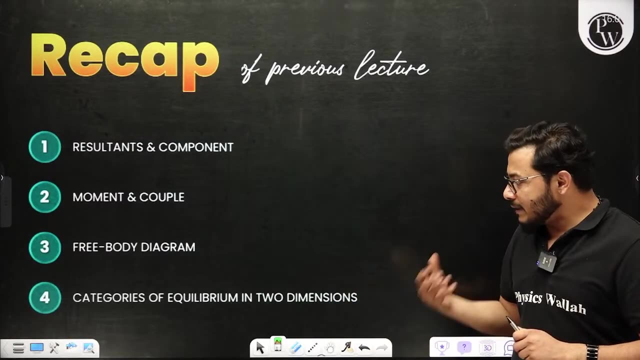 to you about force component, what we call it and how to find out the resultant. Let me recall the last lecture quickly a time. What did you do in yesterday's class? So in the last lecture you talked about resultant component moment and à pe x And you talked about john. 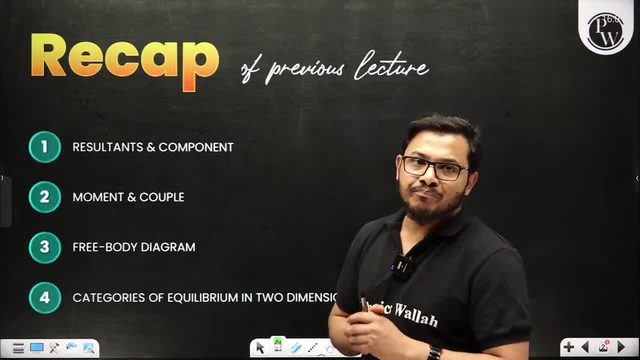 porqueydri de an, the category of disciples in 2ensions. So yesterday we had seen all these topics in the lecture. So we will talk about all the topics in the lecture of science and mechanics with one-to-one practice. So today we are. going to talk about the problem of 브 shi a departure dzisiaj這些 vêberty we talked سیура inกہ's past tensejust continue as we have done before that today. So yesterday's lecture. 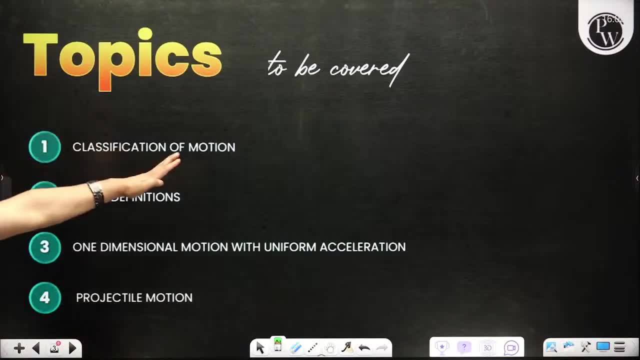 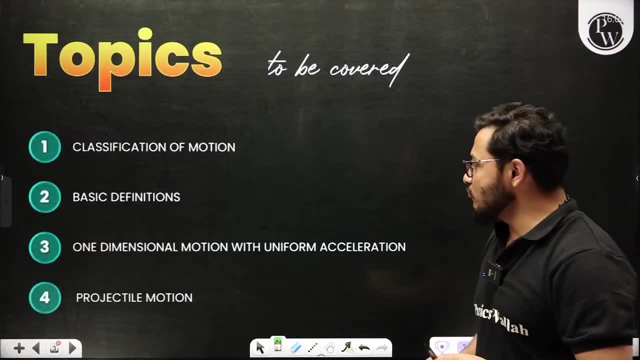 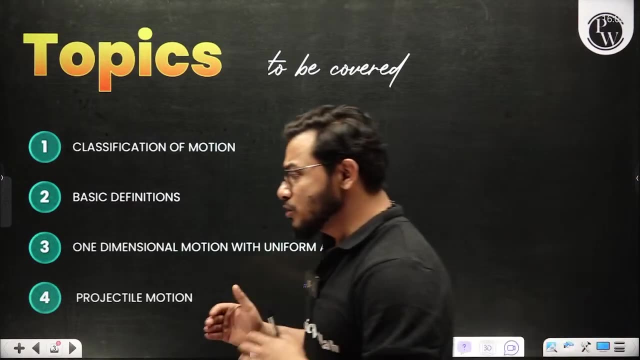 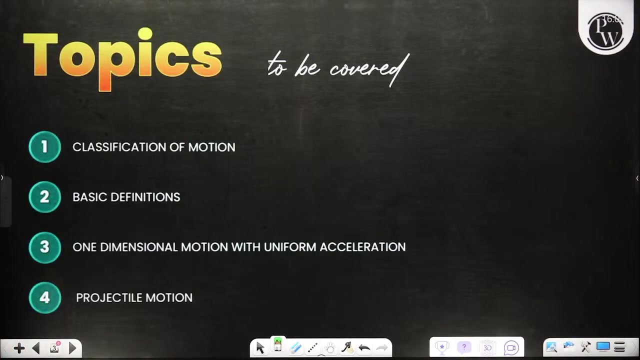 new topic is going to start. that my part is your classification of motion, some basic definitions. you have to explain basic basic definition and then after that, one dimensional motion with uniform acceleration you have to talk, and some formula of projectile motion, some things here I have to start. so once quickly message and tell: start the session. you can start the session. 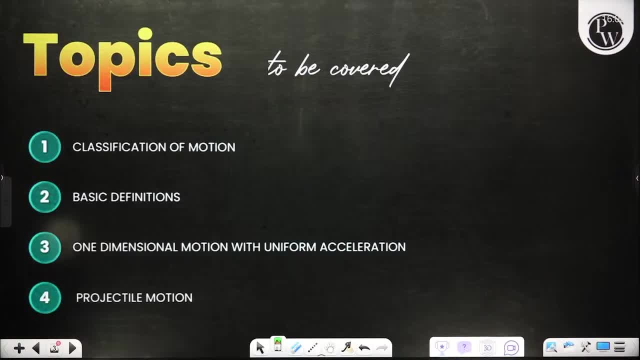 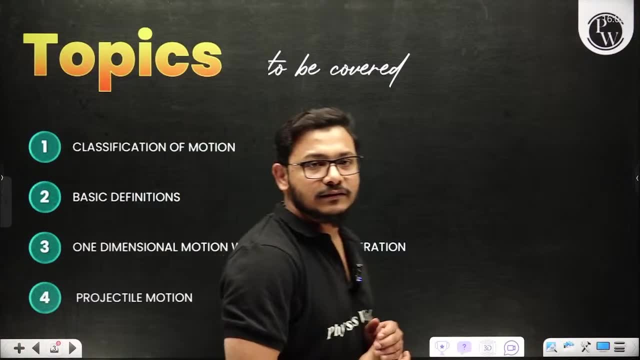 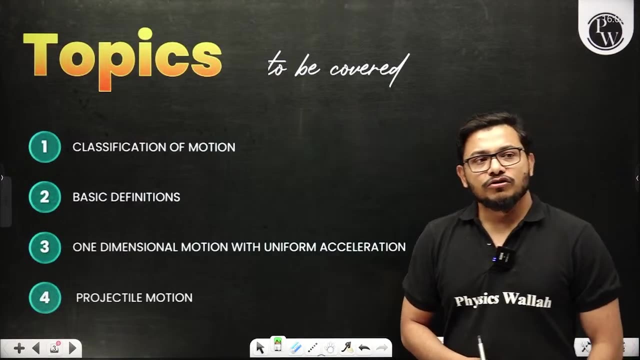 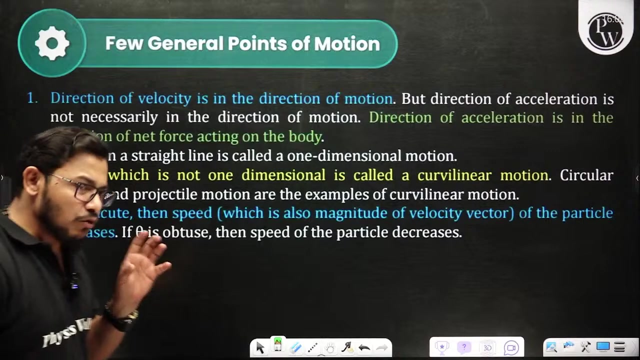 now. are you ready? please tell quickly. are you ready? we can start. all the people are ready, so let's start then. so in the class, whatever part you have here, I first of all talk, that brother first understand about some points, talk about some general points. and what is the some general point? 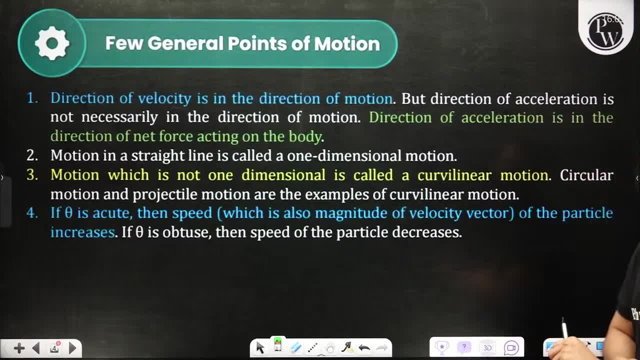 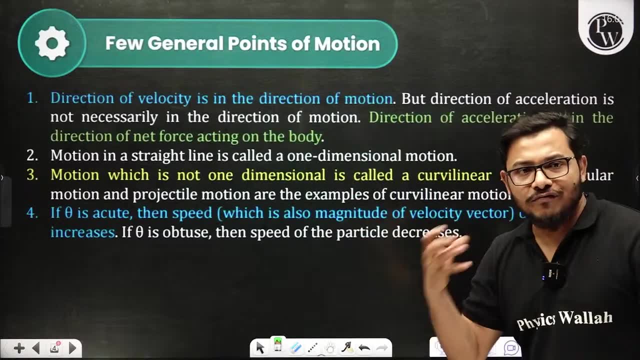 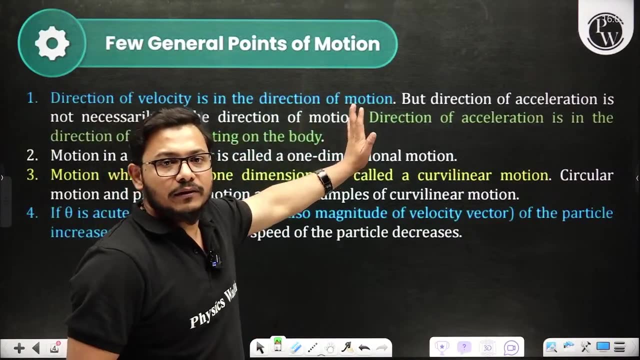 Which points could you have? first of all, we talk about them. why there one minute? one point: You have been seen here that what you have is the Direction of Velocity. what you are talking about The Direction of Velocity which is in direction of motion, which is 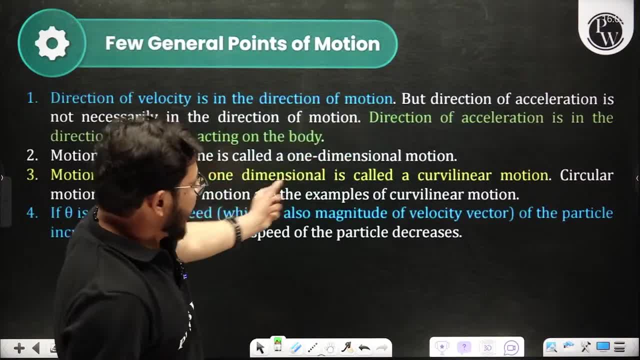 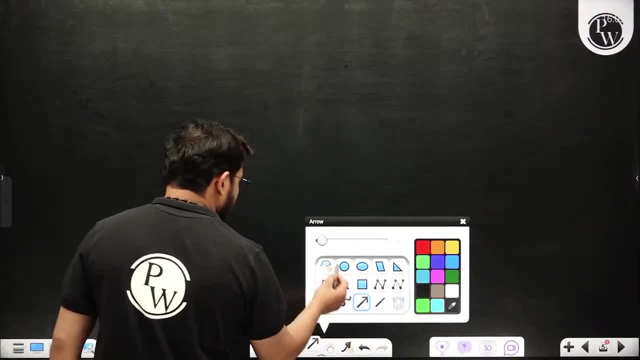 Direction of Velocity, which is in the direction of motion, which means and the direction of acceleration is ours. and I am telling you that you will understand one thing in the question, like when I give you to the question, like what is a question? come here example, brothers. 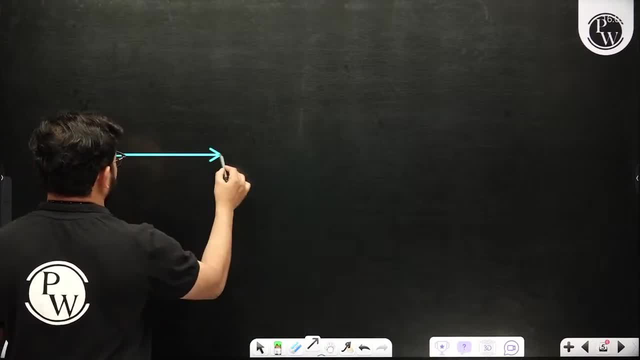 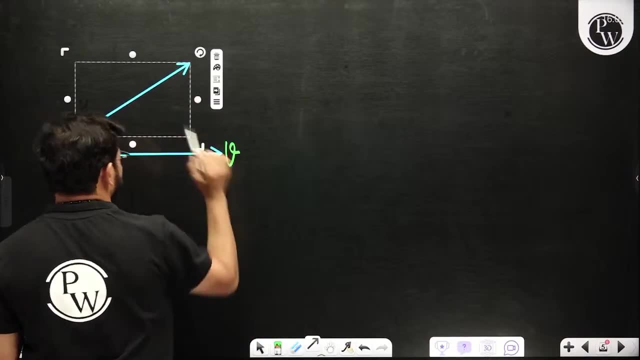 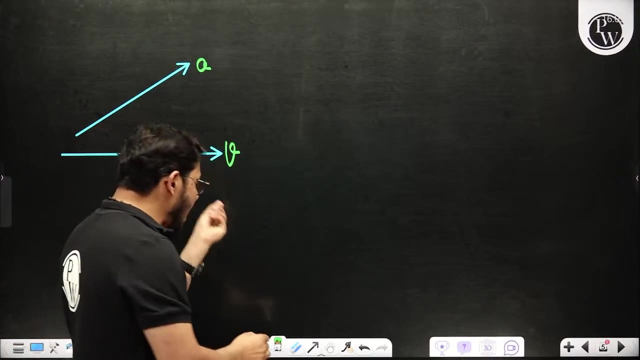 For example, in this direction there is a velocity vector and this velocity vector is v, And let's assume that you have acceleration and that one is the acceleration. So always remember that by looking at the velocity vector v, you can decide the direction of motion. 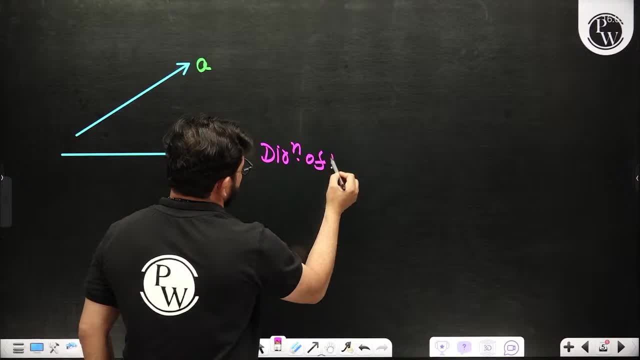 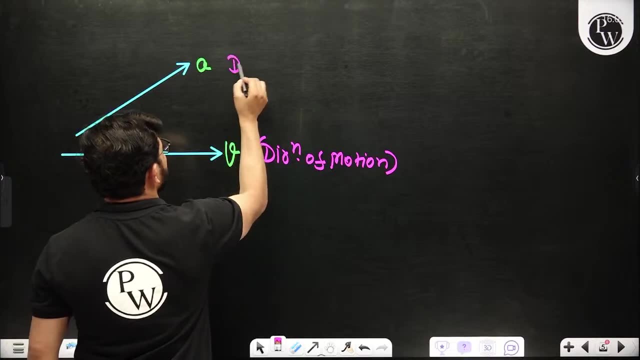 What can you decide The direction of motion? In this direction you have velocity. The direction of motion will be there And by looking at the acceleration you can decide the direction of force. By looking at whom can you decide The direction of force? 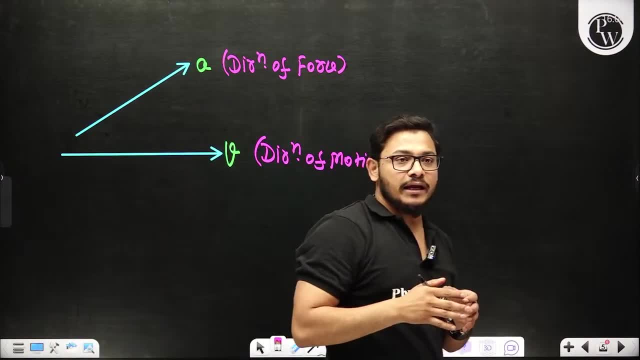 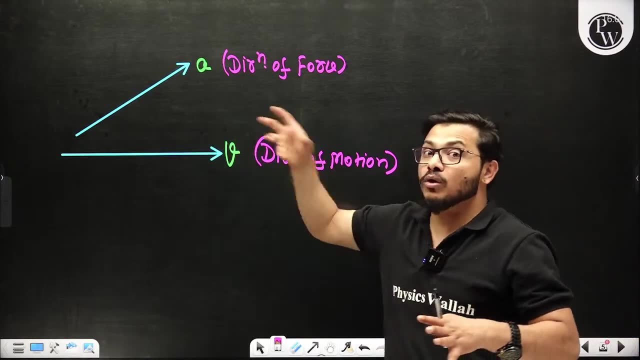 Look, you don't understand that acceleration and velocity are in the same direction. We have to have a bad concept set in our mind that by looking at the acceleration you can tell the velocity, you can tell the motion. This is wrong. You can't tell the motion. Please always remember. 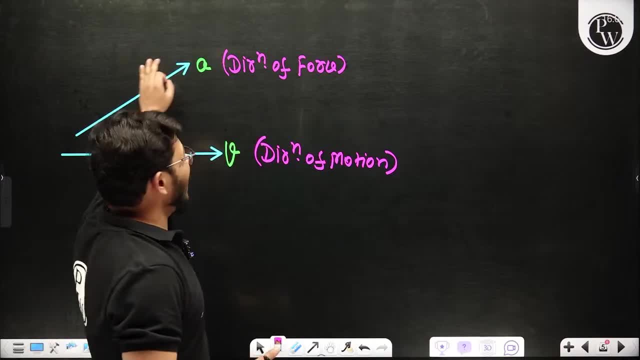 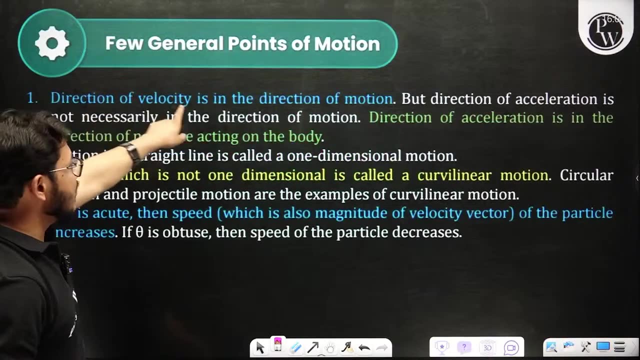 By looking at the velocity v you can decide the direction of motion, And by looking at the acceleration you can decide the direction of force, Force and the direction of motion. So this is my first point: By looking at the velocity you can tell the direction of motion. 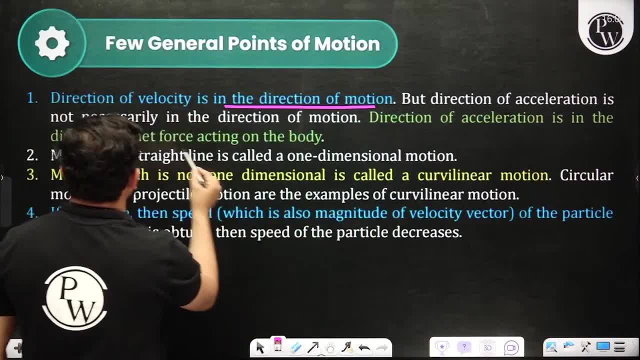 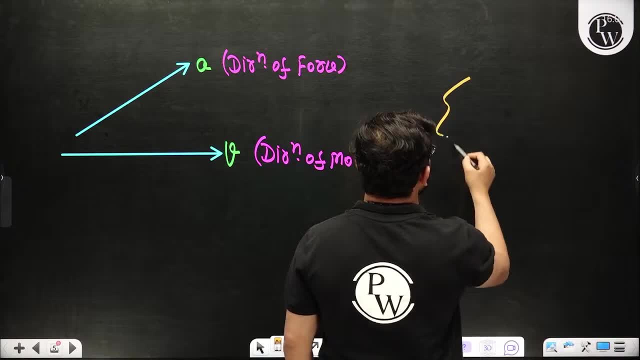 And by looking at the acceleration you can tell the net force acting on a body. Now there will be a great concept here. Let's assume that there is a lot of force on this body. One force is this, one is this, one is this: 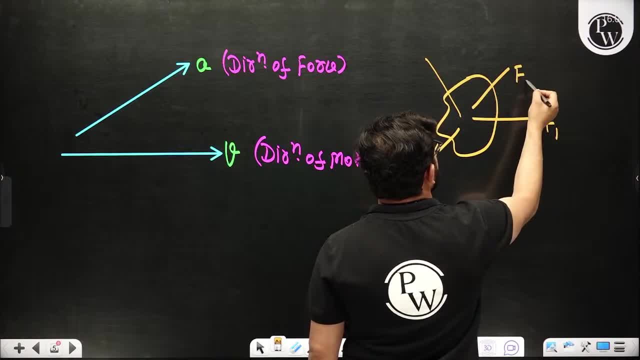 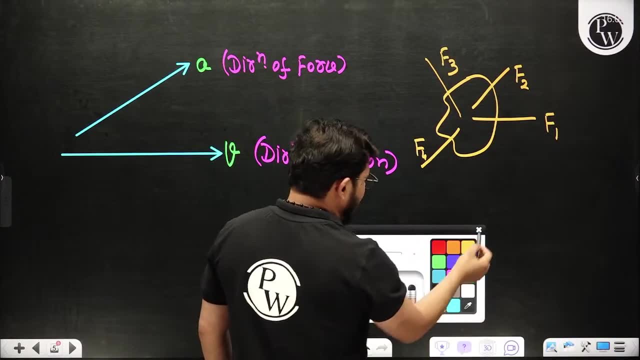 You have applied a lot of force. Suppose this is F1, this is F2, this is F3, this is F4. If someone asks you in the question that, tell me the total net force on this body, So tell me what will be the net force. 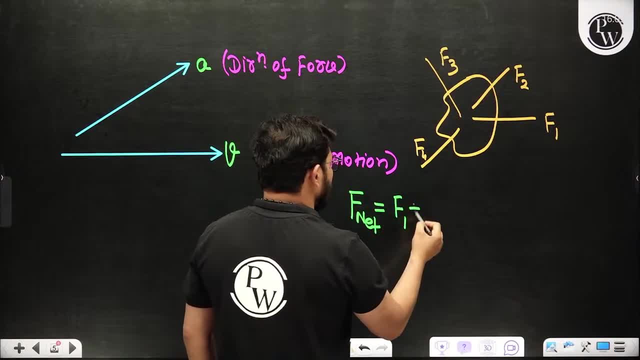 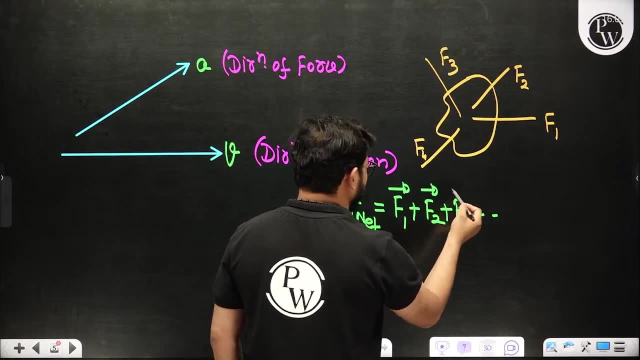 You will say, sir, add all these forces, So F1 plus F2, plus F3 and plus dot dot. What did you add to all these forces? What did you add to all these forces? That is called net force. Look, there is another way to write net force. 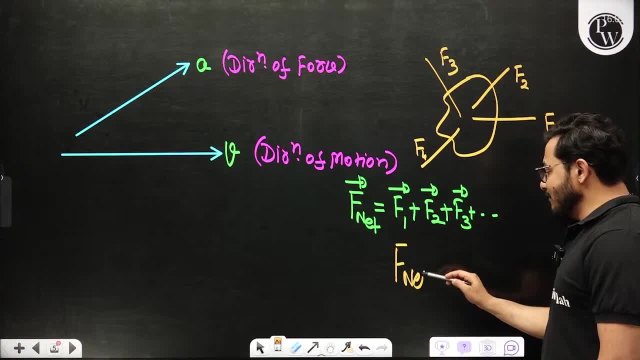 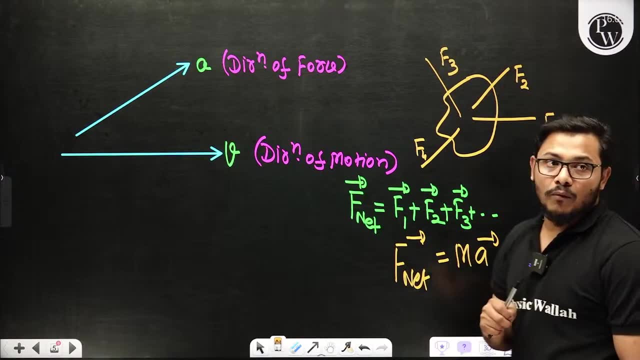 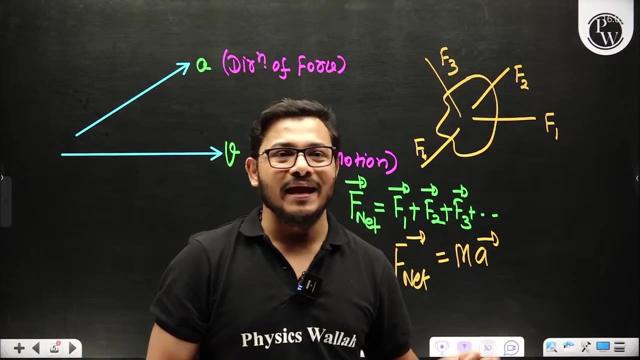 You can write net force like this: The net force becomes is equal to m. What a great thing you have written. If you know the acceleration of any body, If you multiply that acceleration with mass, then the answer that will come from mass into acceleration will be net acceleration. 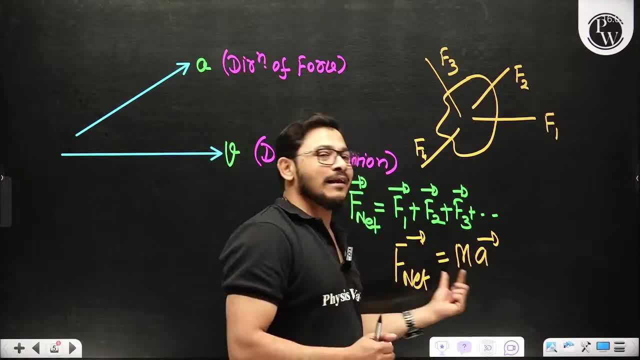 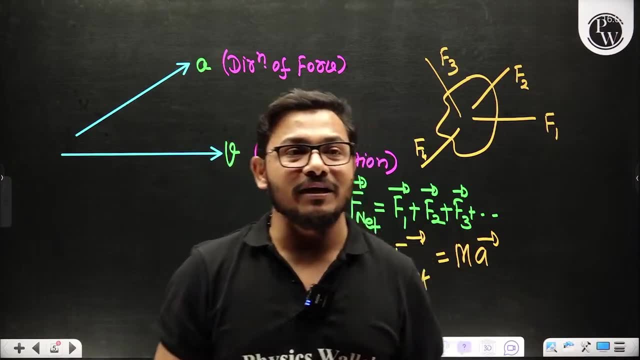 If you write mass into acceleration together, then whatever will come from mass into acceleration that one is become is equal to the total acceleration. What will come to you? Total acceleration, Total acceleration and mass into acceleration. AA is the total acceleration And m is the mass. 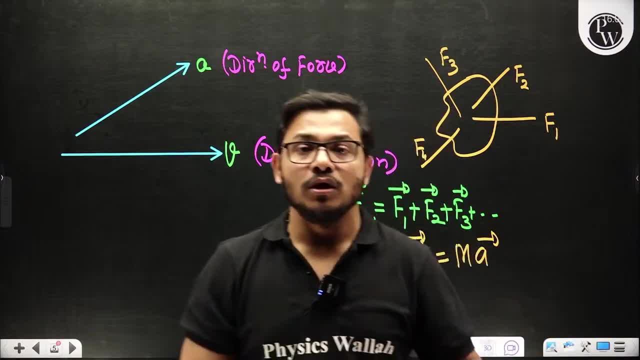 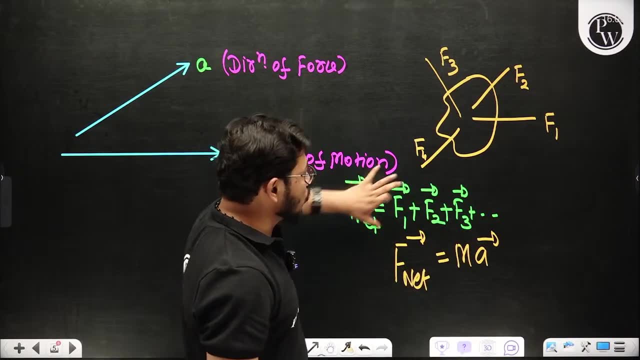 If you multiply MA, then that one is become is equal to the total force. So you have two ways to calculate the total force. Either write the net force from MA or you can do the algebraic summation of all the forces of the net force. 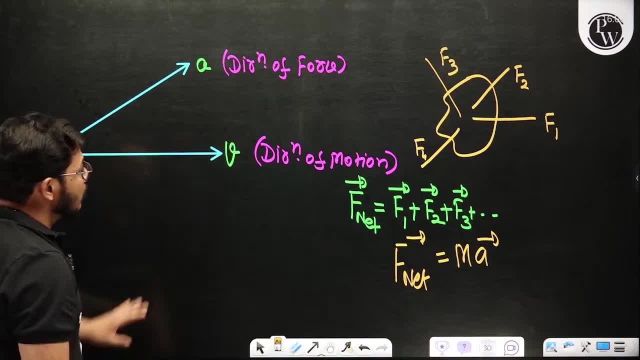 So that is also one way You solve it. from anywhere You will get the same answer. So by looking at the velocity you can decide the direction of motion, And by looking at the acceleration you can decide the direction of force. 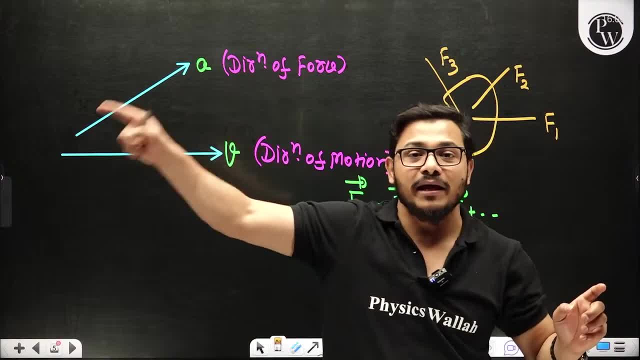 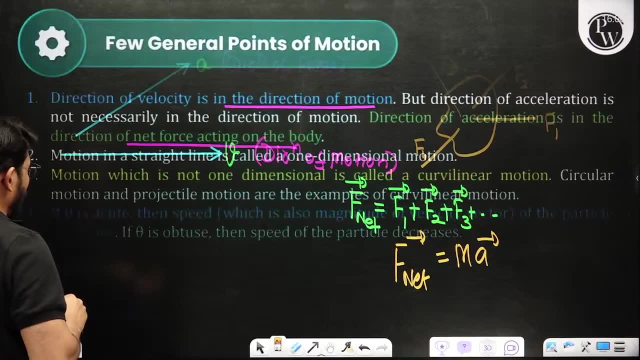 You will not say that the direction in which the acceleration is, your velocity will be in that direction. You need to understand this. I would like to tell you the second thing here, And that is also a very important point for me. I have written it here: 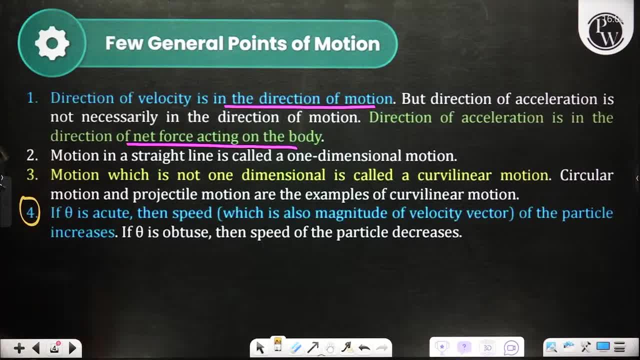 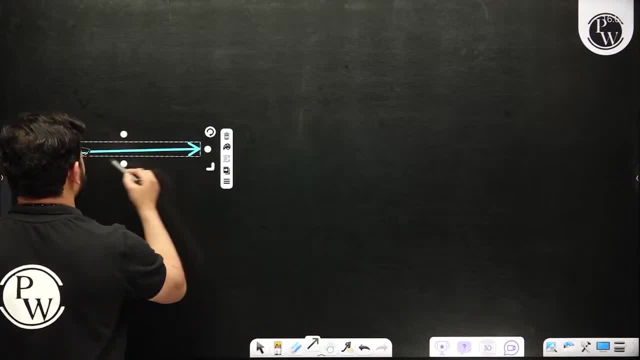 And this is the point you have. And the fourth point is very important for you. What is that point you have? Please look at it for one minute. If in any numerical question, if you have seen this, if the angle between velocity and acceleration, 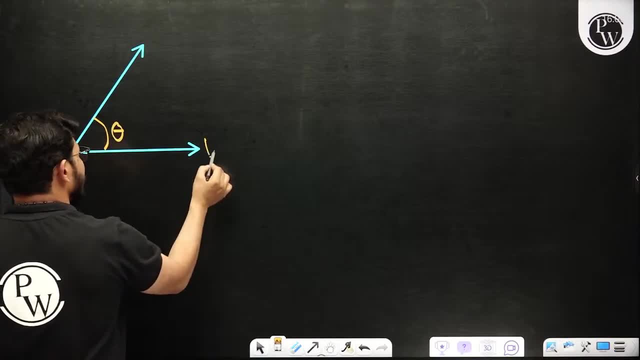 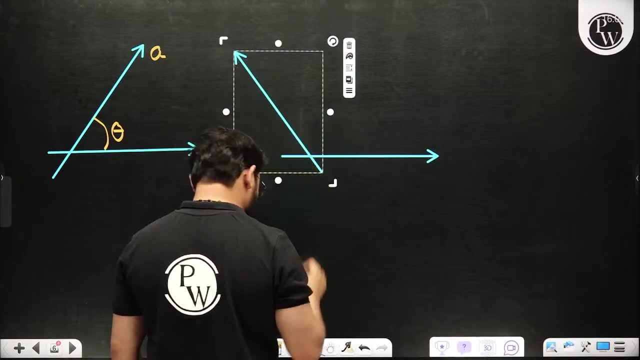 let's assume it is theta, Let's assume it is velocity And this is acceleration. If you assume, for example, if in the question it happened, that let's assume it is velocity And this is acceleration And the angle between these two is theta, 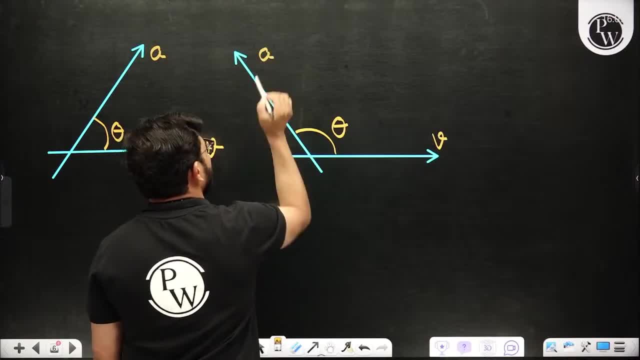 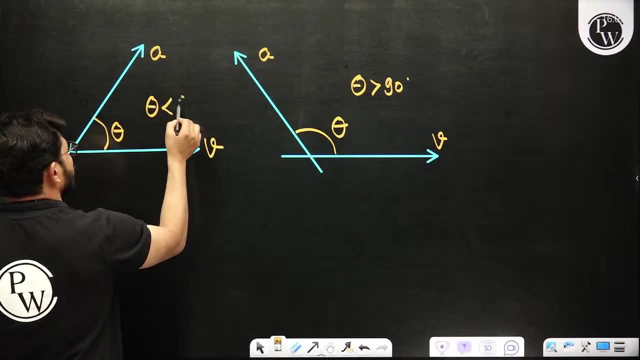 This is greater than 90 degrees. Assume this velocity as acceleration. Here this angle is theta. This is an obtuse angle, Because this is greater than 90 degrees, And here this theta is smaller than 90 degrees And this angle is acute angle. 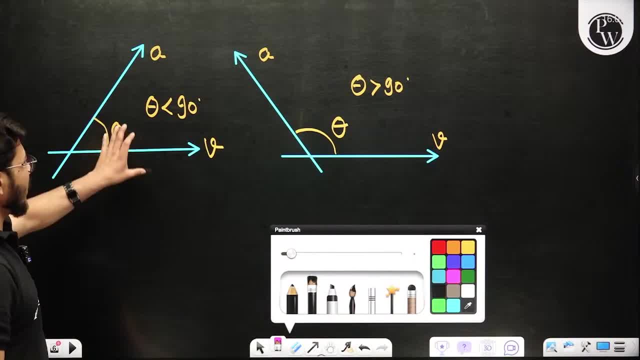 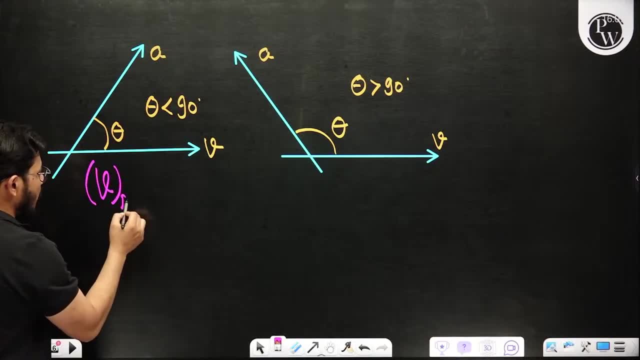 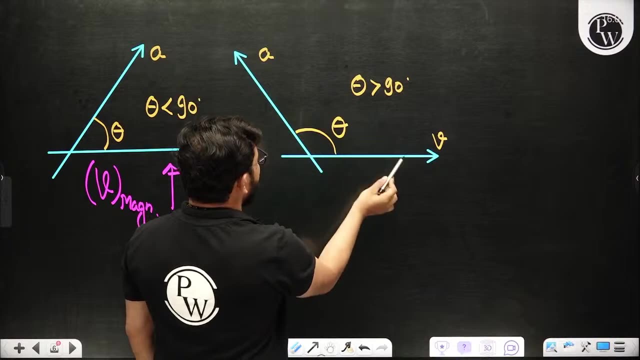 If anywhere in the question, if the angle between velocity and acceleration, if you see the angle smaller than 90 degrees, then remember, the magnitude of velocity will be increased Here. the magnitude of velocity will be increased If somewhere, if the value of this angle is greater than 90 degrees. 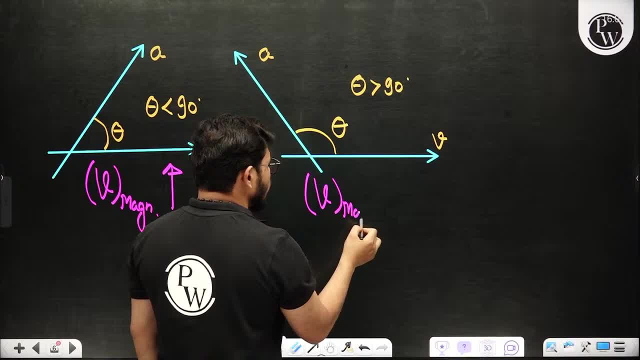 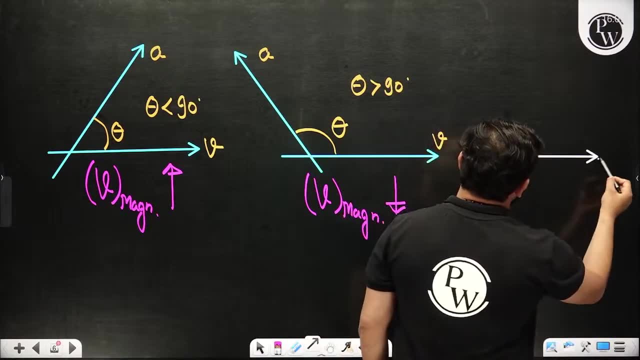 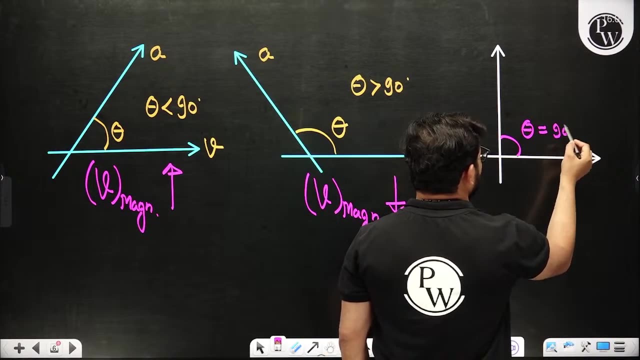 then remember, the magnitude of velocity will be decreased If, in any problem, the angle between velocity and acceleration if it is 90 degrees, if the value of theta is 90 degrees, So what will happen? The magnitude of velocity will be constant with time, it will not change. 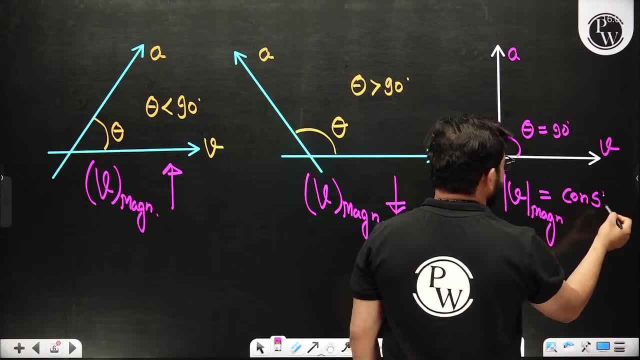 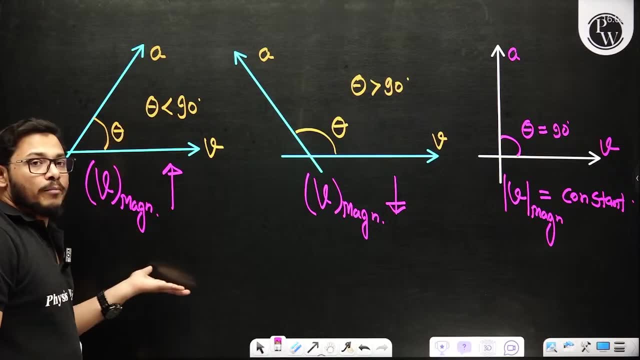 How will its magnitude be? It will be constant. Have you written a wonderful thing. If the angle between velocity and acceleration is less than 90 degrees, then the magnitude will increase. If it is greater than 90 degrees, then the magnitude will be less. 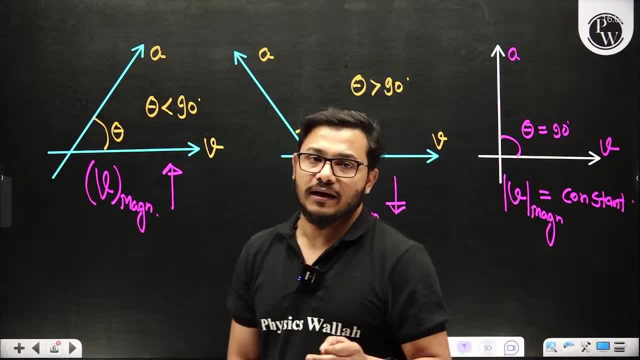 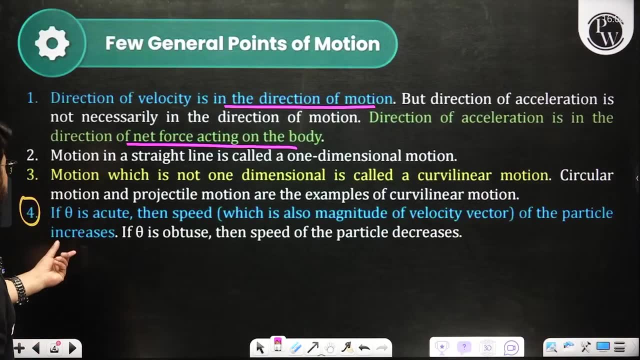 If it is 90 degrees, then the magnitude of velocity will be constant with you. You need to understand this. That only the one idea how you are talking about velocity here. So I have written all the things here that what is velocity, When will velocity increase and when will it decrease? 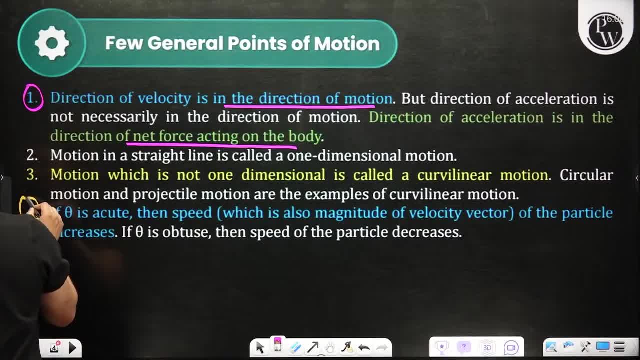 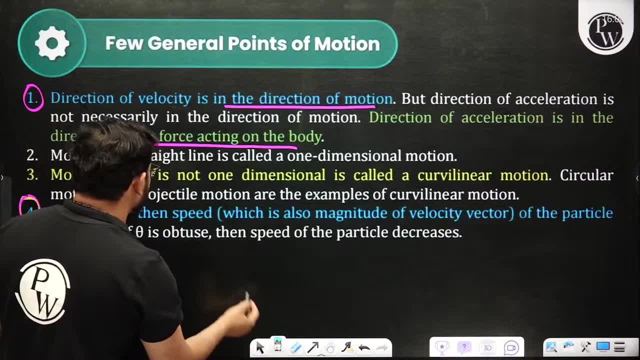 You must have understood the thing. I have discussed two points for you, the first and second. The first and fourth point. The second point is very important for you. Please read it. Look, when you see a motion alone in a straight line, any motion, then it is called one dimensional motion. 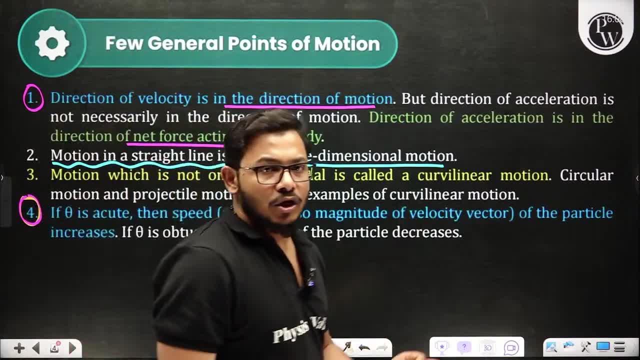 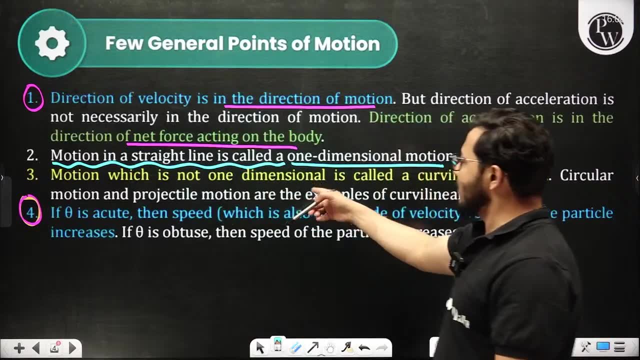 What is it? It is called one dimensional motion. The motion that you will see alone in a straight line, that will be called one dimensional motion. The motion that is not one dimensional, that motion is called curvilinear motion. What is it called Curvilinear motion? 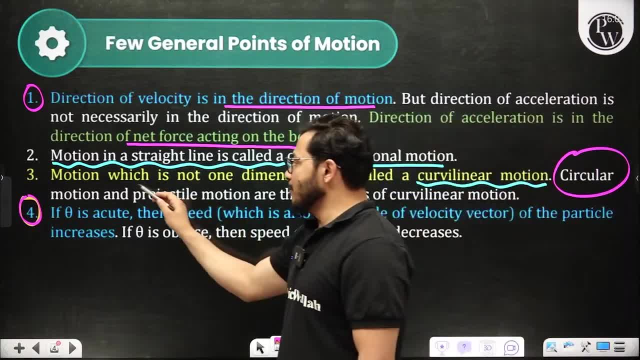 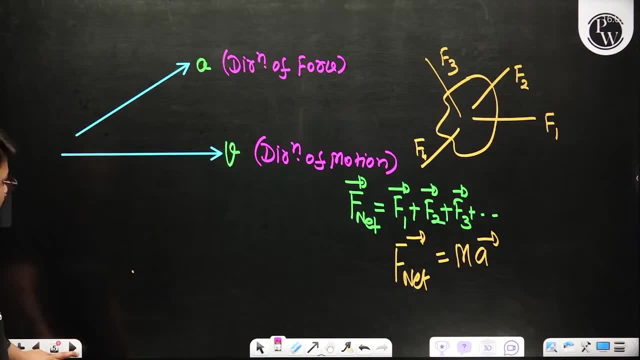 For example, you can call it circular motion or projectile motion, So these two motions are curvilinear motion for you. So, for example, let me tell you here- please see it for one minute- What am I saying to you. 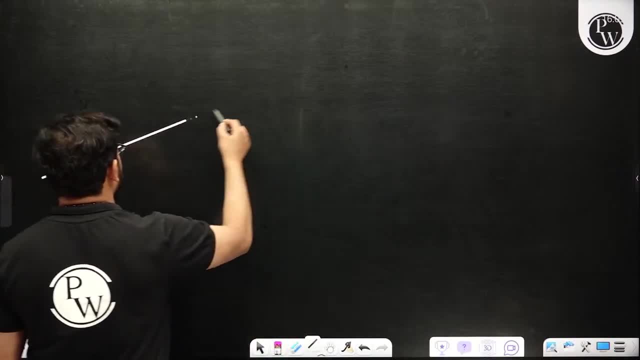 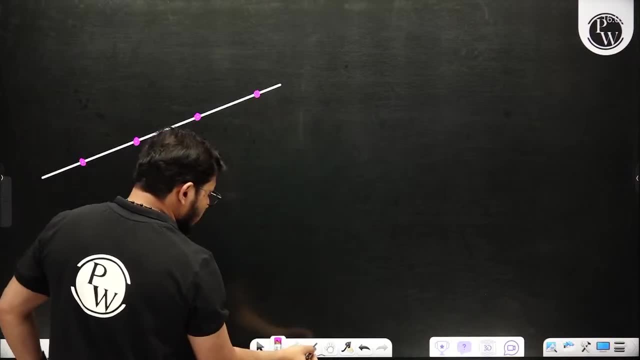 Suppose, let's say here: Imagine that a particle is moving alone along this line. The first particle came here after some time, came here after some time, came here, then came here. So this motion that is happening to you is happening alone in a straight line. 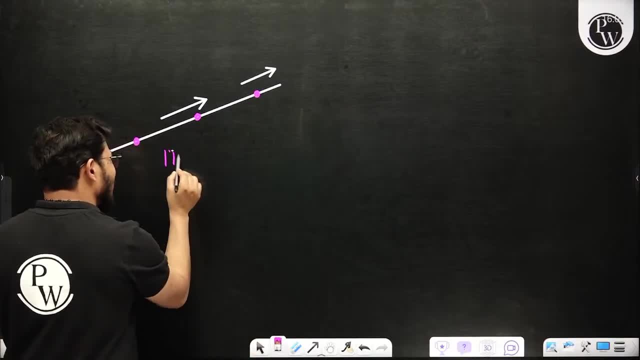 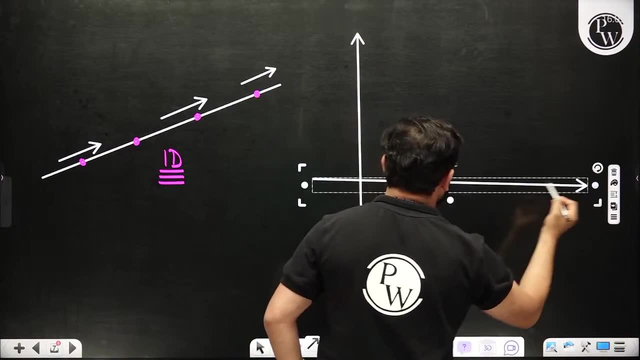 So this motion is being alone in a straight line, This motion will be called 1D. It is called one dimensional motion If the motion is not alone in a straight line, like a circular motion or a projectile motion, like a projectile motion. 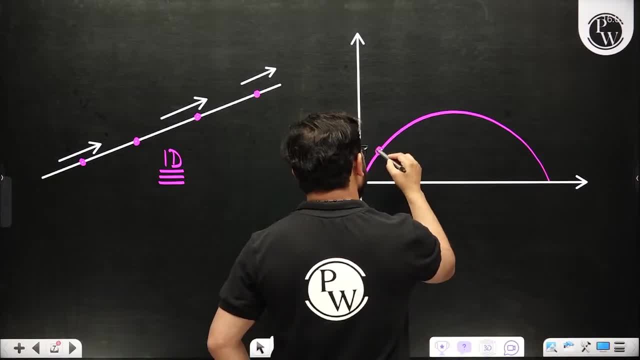 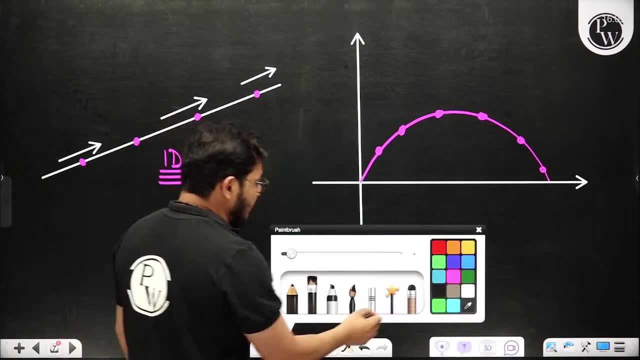 Let's assume that this motion is going on. This is not a line alone, it is a curve alone. it is a curve alone. as you can see here. When you calculate the velocity, then it is coming along this path. Let's assume this path is projectile motion for you. 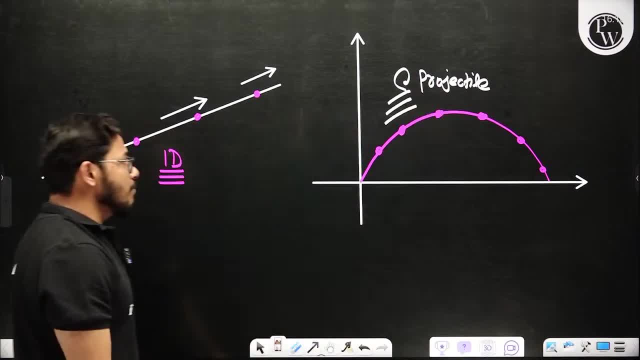 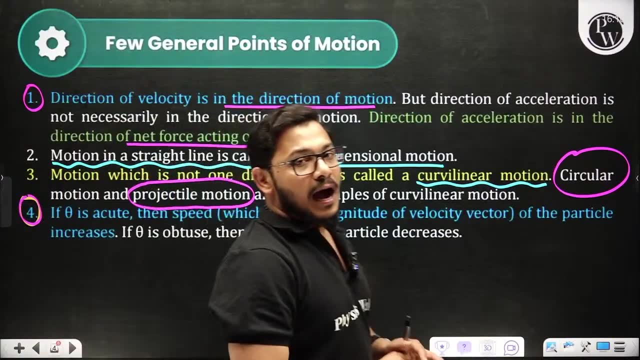 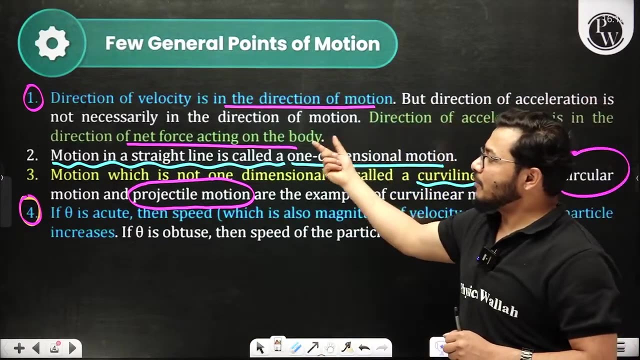 So I told you some important points regarding motion And maybe that point will be clear to you. What is the first point? Please understand again. You decide the direction of motion by looking at the velocity And you decide the direction of force by looking at the acceleration. 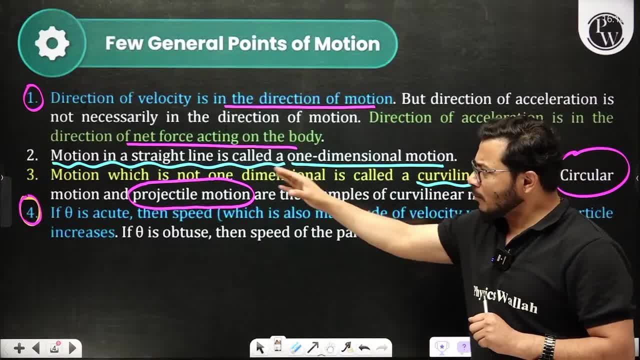 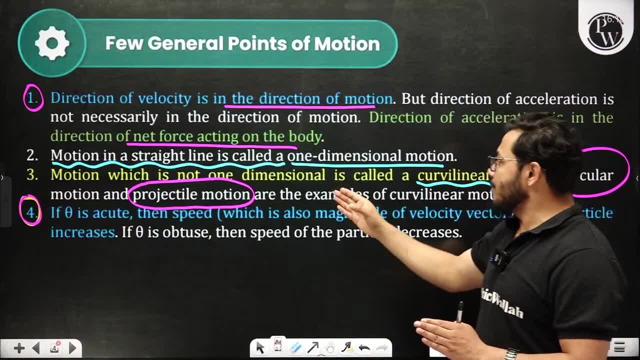 This is the first point. The second point is that the motion that is along the straight line is called one-dimensional motion. Very good, You know one-dimensional motion by the name of 1D. If the motion is not one-dimensional, then it is called curvilinear motion. 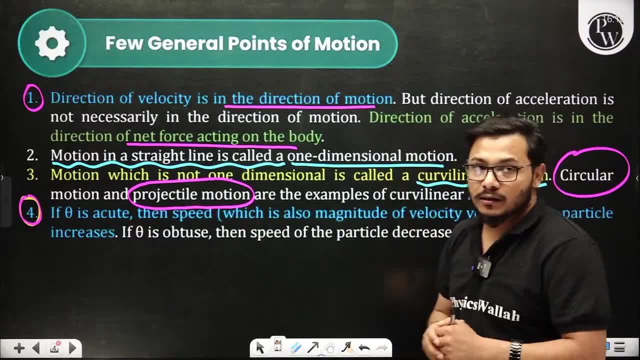 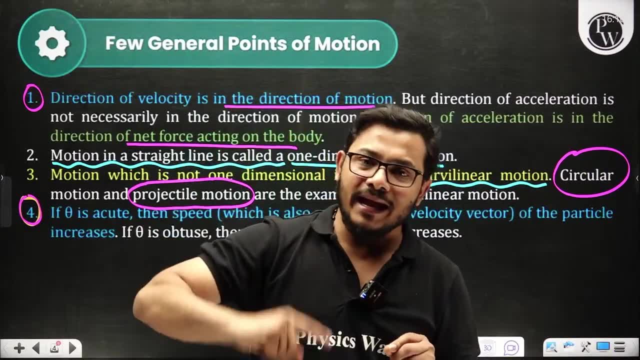 You can see the example of projectile motion and circular motion. If you see the example of projectile motion and circular motion, then the angle between velocity and acceleration: if it is smaller than 90 degrees, then the velocity will increase. If it is bigger than 90 degrees, then the velocity will decrease. 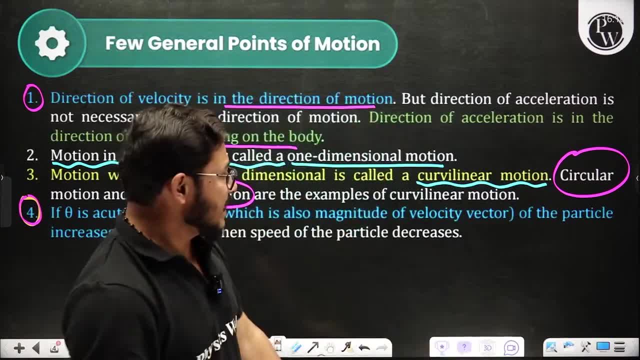 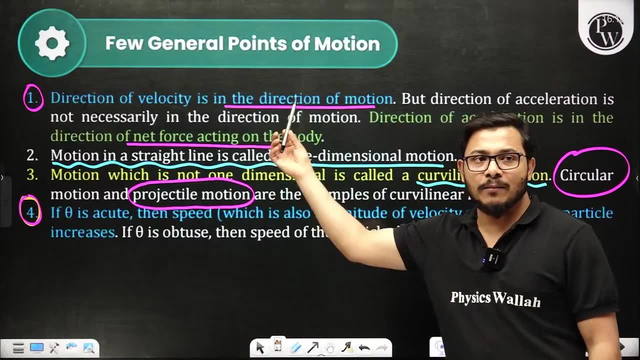 If it is 90 degrees, then its magnitude will be constant. So how many children are there who understood this concept? These four points are clear to you, So I have explained some general points related to motion to you. I hope you got the concept. 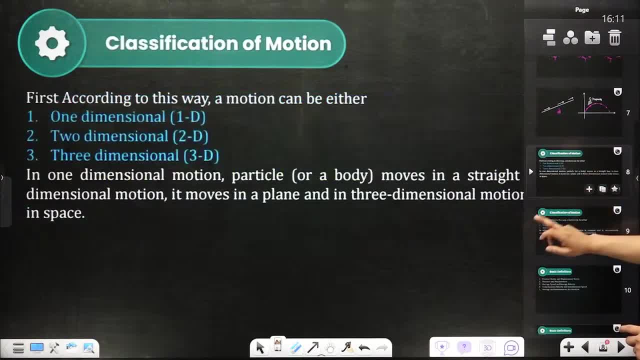 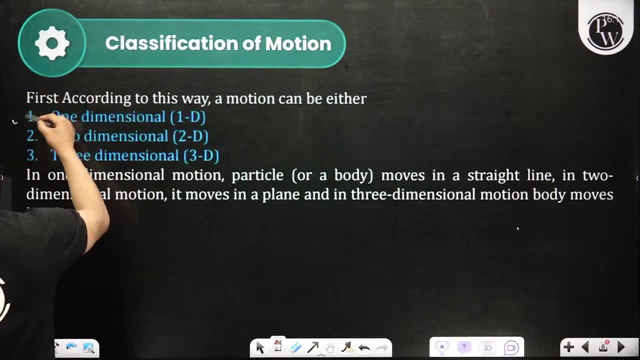 Tell me quickly. Did everyone understand? Please tell me quickly, Now you have classified motion, What is the classification of motion? One is one-dimensional motion, One is 2D and the other is 3D. We have to study only these two. 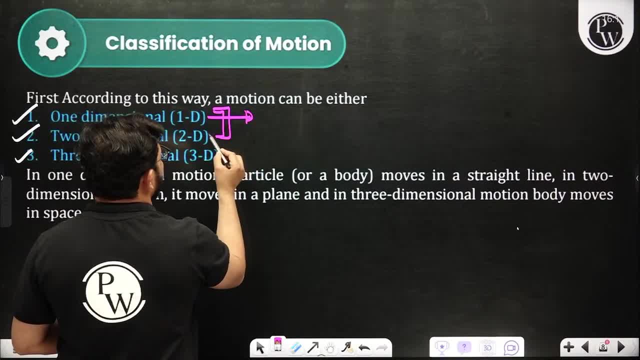 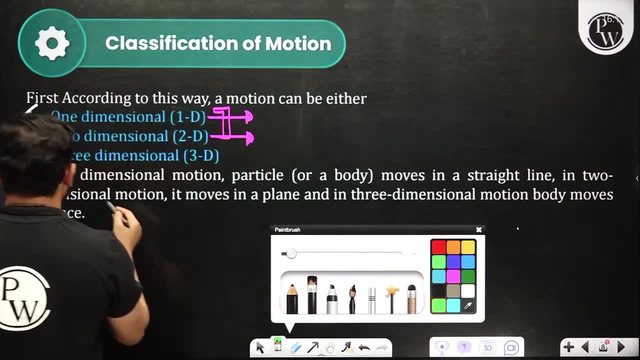 I have to study 1D, you have to study one-dimensional And you have to study 2D. It comes in the language One-dimensional and 2D Understand the meaning of one-dimensional motion. One-dimensional means along a straight line. 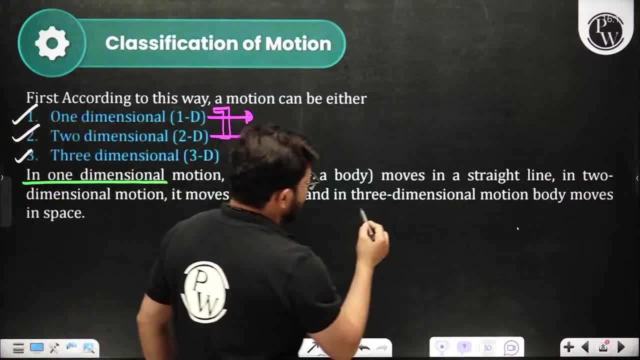 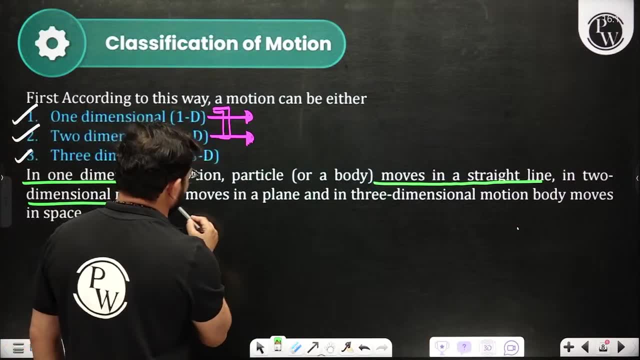 Please listen for one minute. One-D means that a particle is moving in a straight line, And two-dimensional means that a particle is moving in a curve. A particle is moving in a plane. Just understand this much: Where is that motion happening? in the plane. 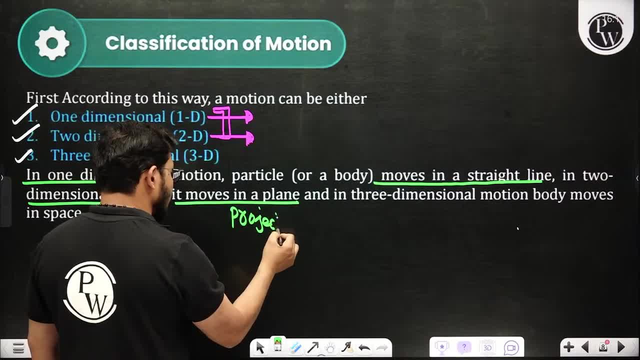 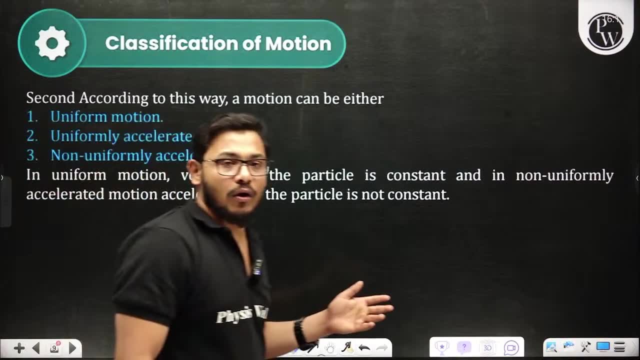 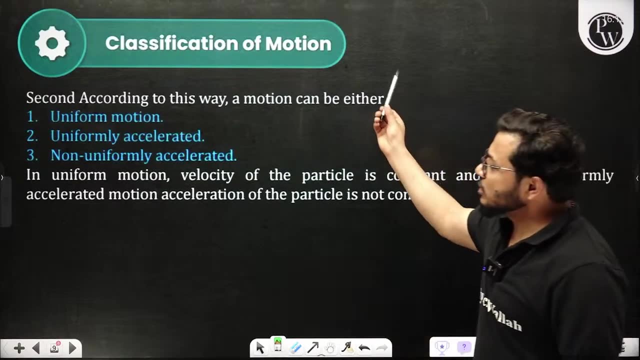 For example, projectile motion. Which motion Projectile? So this is 2D for me. You must have understood this much. There is another way to classify motion. There is another way to classify motion. What is the other way? Either, you can write the classification of motion like this. 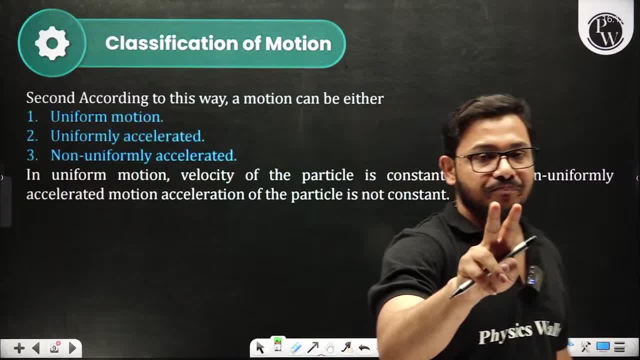 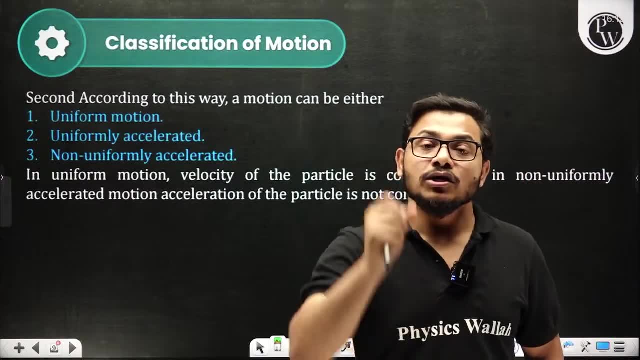 Uniform motion. I will tell you Now listen to me, please Listen to me, In SSC, JEE. In SSC JEE, In 99% case, The quotient that will be your numerical From motion, That quotient is always made from these two parts. 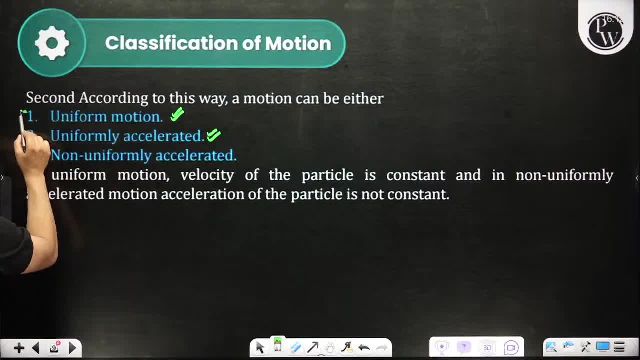 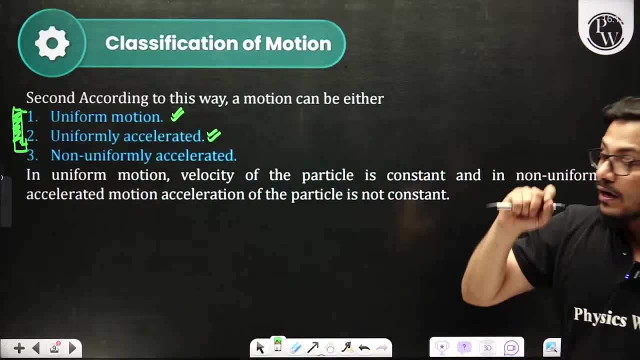 Either it will be made from here Or it will be made from here. In 99% case, The quotient is made from here. Please always rememberize that concept And how the quotient will be made from here. I will tell you that. 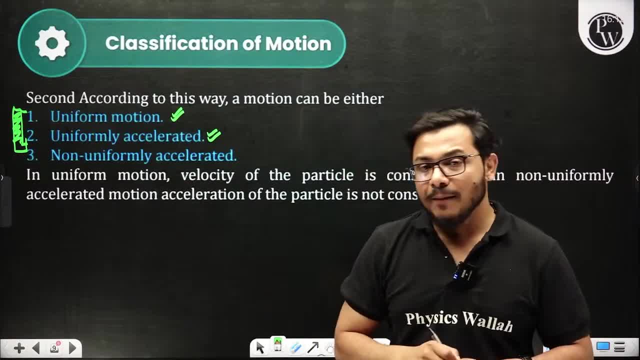 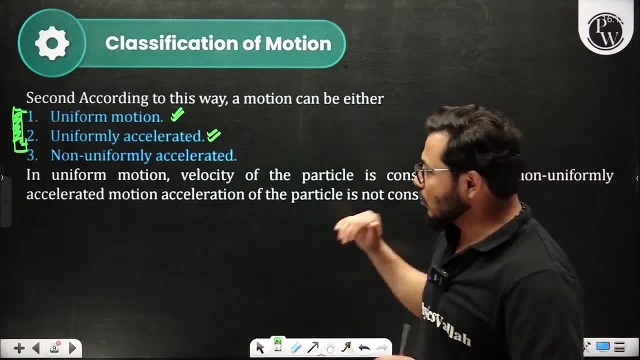 See, how can you have motion Uniform? Now you will think: What can be uniform motion? But today is the second class, But this is the first class of this chapter. Don't worry, You continue the lecture, No problem. So what is called uniform motion? 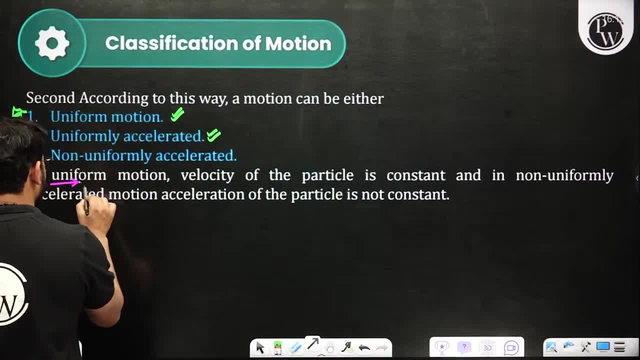 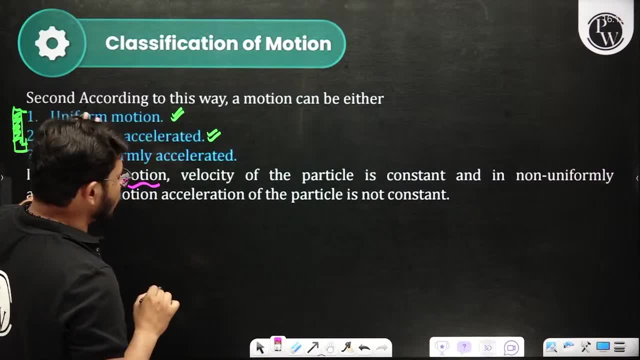 Uniform motion. See, it is clear from the name That something is uniform. How is something? It is uniform? You must know one thing: That velocity is vector quantity. So vector depends on two things, On magnitude and direction. Now, some velocity is uniform. 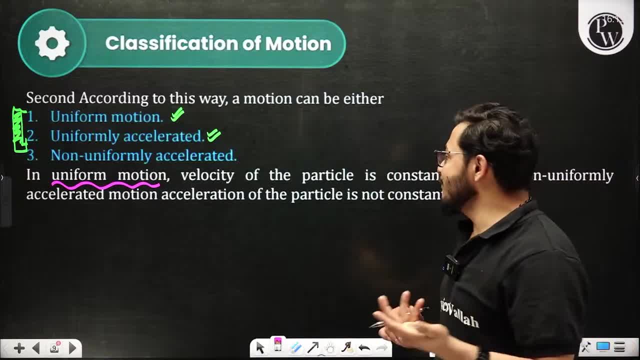 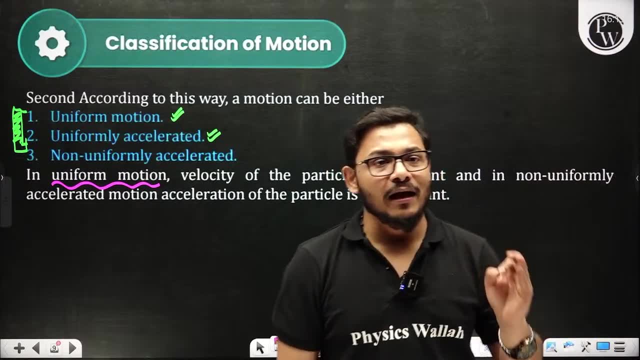 Now, when will any velocity be uniform? Any student will tell When will it be uniform. See, it will be uniform When its acceleration magnitude will be zero. So if someone asks you That if this velocity is uniform, Someone is telling you. 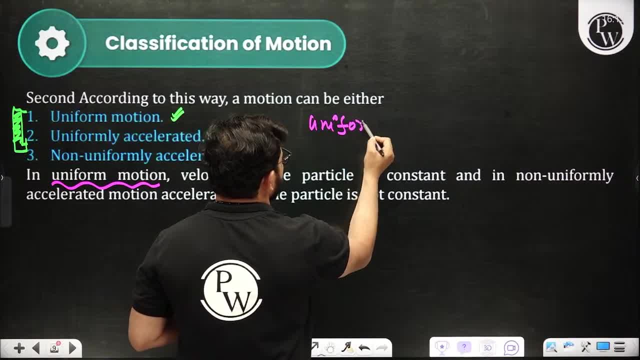 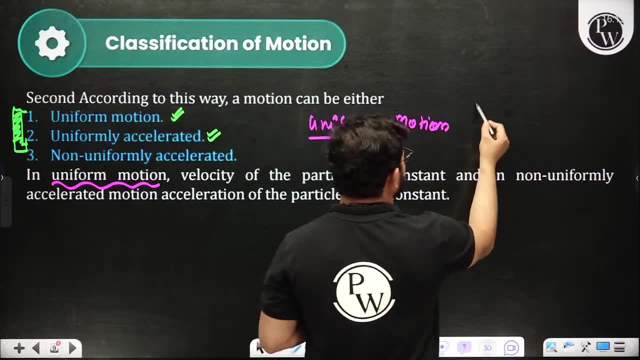 That you are having uniform motion. What kind of motion is happening? Uniform? So what is the meaning of uniform motion? Velocity should be constant. Uniform motion means Velocity magnitude should be constant. Now, when will velocity be constant? Velocity velocity will be constant. 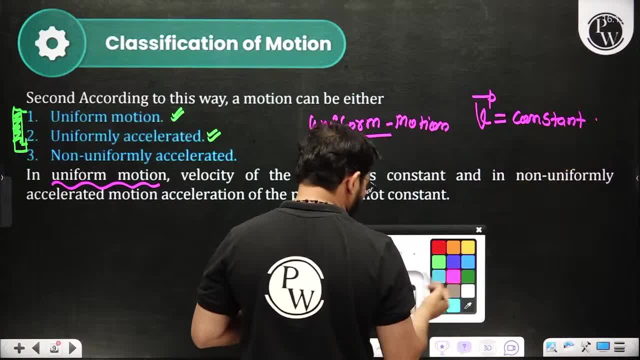 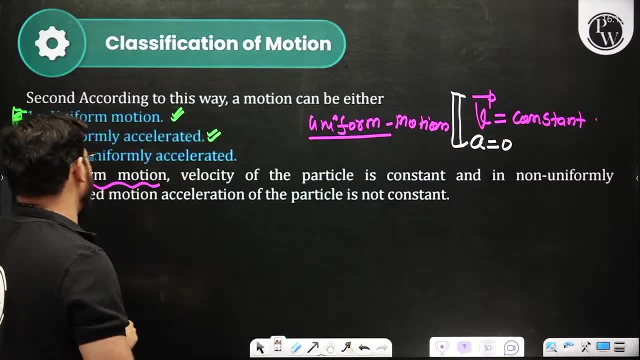 When will velocity be constant? When acceleration will be zero? When acceleration to be zero? So in uniform motion, Acceleration's magnitude in makes a zero. Acceleration magnitude is zero. The second thing that you have is uniform accelerated, Uniformly accelerated means. 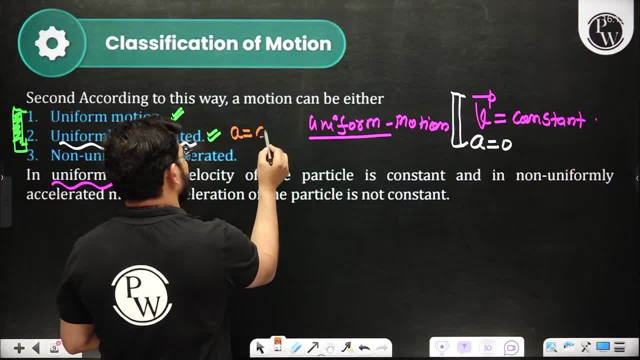 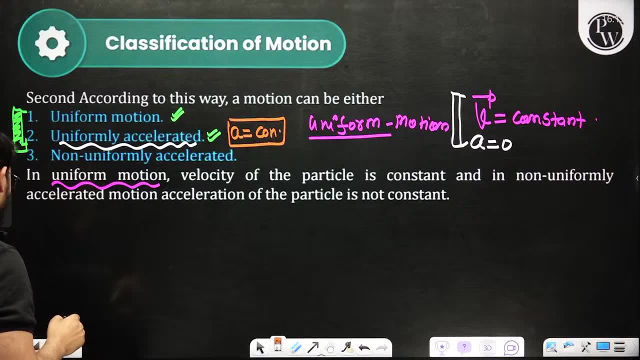 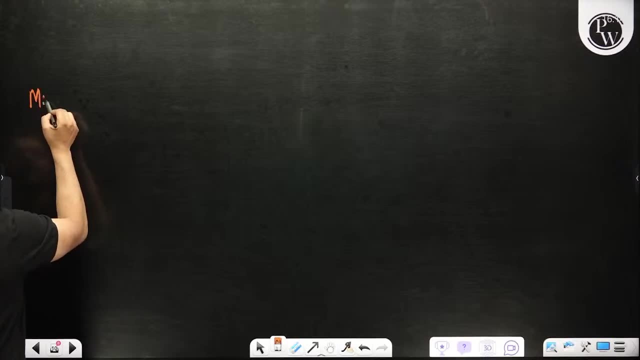 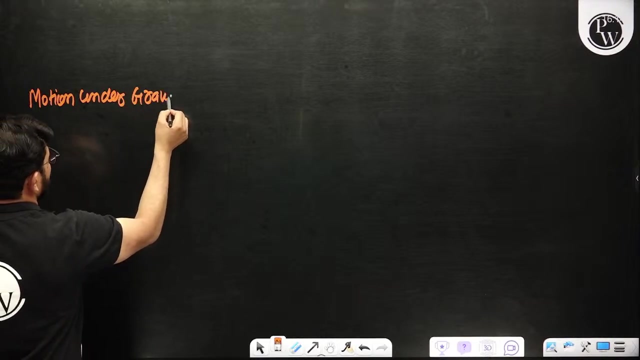 Acceleration's magnitude is constant. in this case, Acceleration's magnitude is constant, For example. let's take example of uniform acceleration, Uniform acceleration. If I take an example of uniform acceleration, then the example of uniform acceleration can be motion under gravity. Please listen for one minute. Motion under gravity. Please understand one thing a little carefully: Motion under gravity. 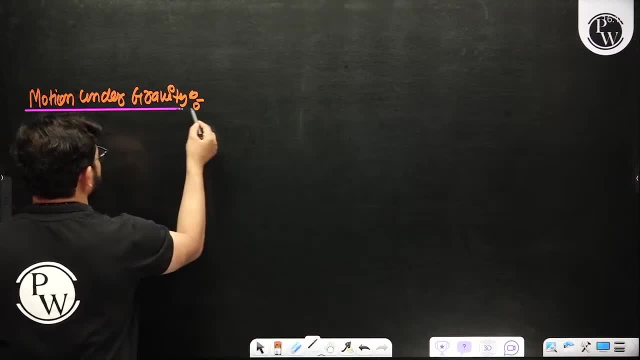 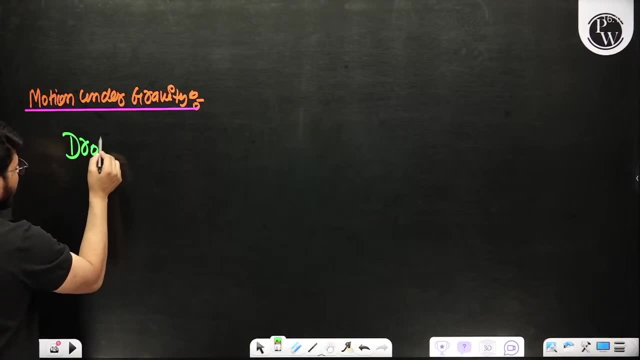 I will explain you some things here. Please listen for one minute. There are two things. One is to drop and the other is to throw. If drop is written somewhere, then you understand that the starting velocity of the particle will be zero. If throw is written somewhere, then its initial velocity will not be zero. 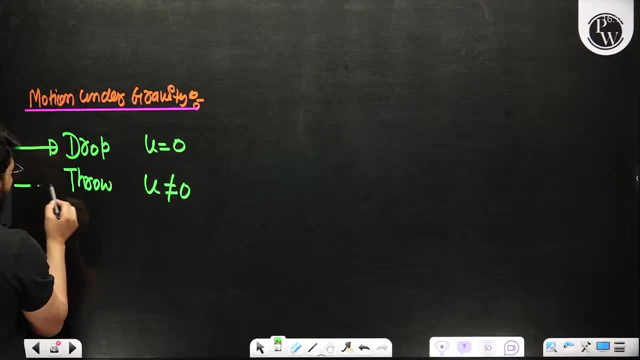 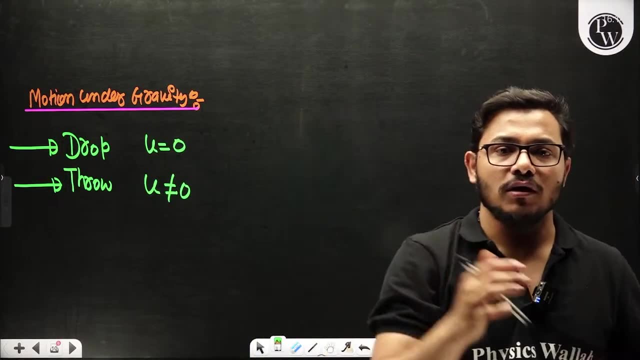 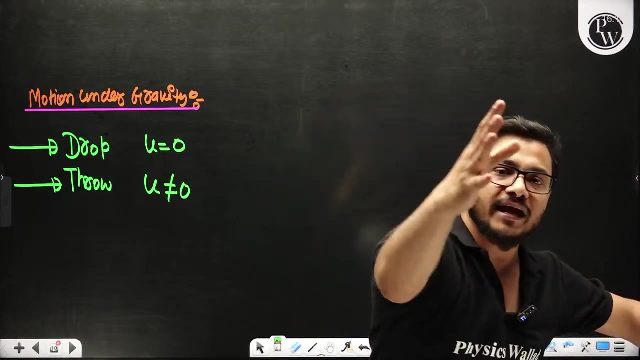 Drop means original velocity is zero and throw means original velocity is zero. What did you do to any particle? You threw it. You must have seen it while playing cricket. The ball is in your hand and you throw it. Throw means you threw the ball, So original velocity is nothing. 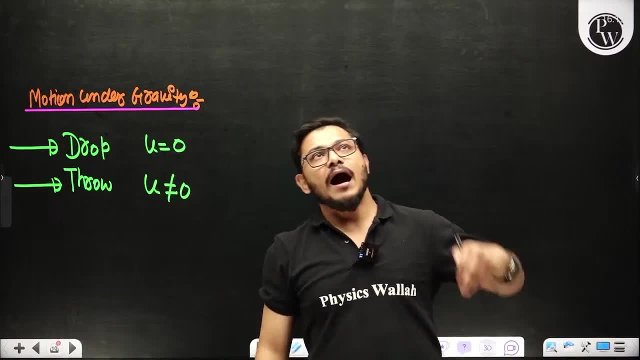 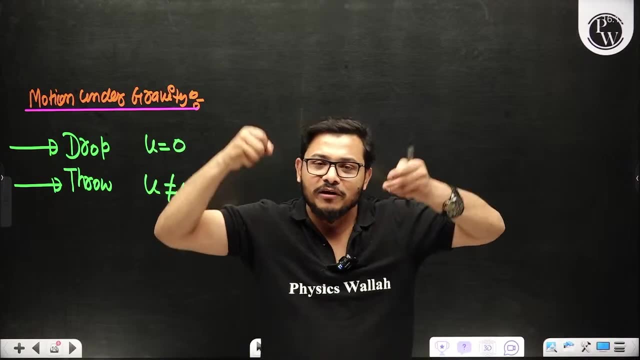 Now you have to drop. Suppose you have a fight with someone. You are standing on the top floor of the building. You have seen that you are standing with a stone in your hand. When this person will pass under my building, I will drop the stone and hit his head and he will die. This is what you think. So you are standing like this with a stone. 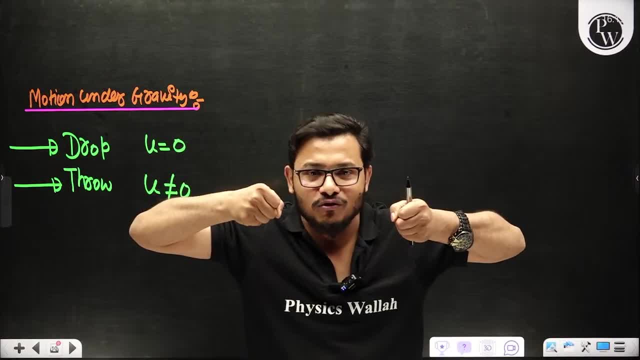 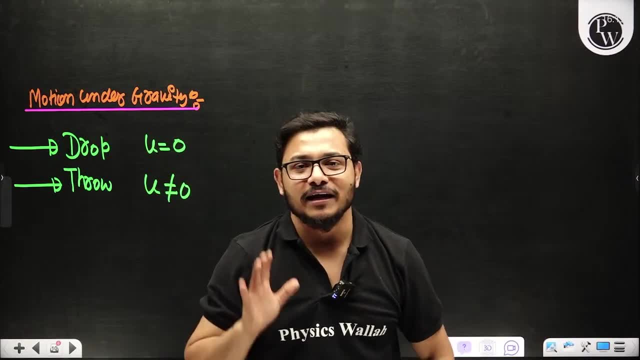 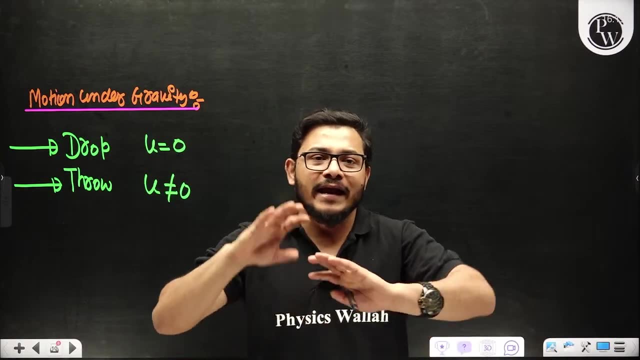 So the stone is going down And you will hit someone on the head, So this is called dropping. Drop means original velocity is zero, and you understand what I am trying to say. So what I am going to tell you here, Please see carefully. 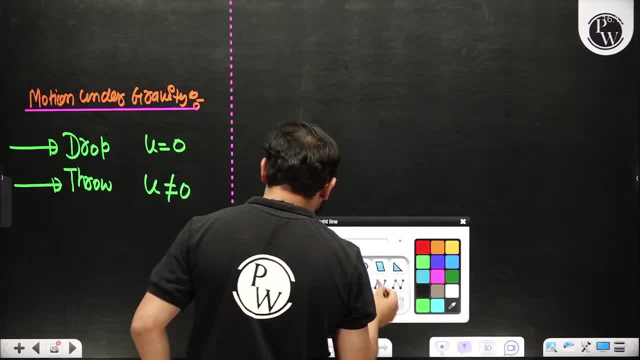 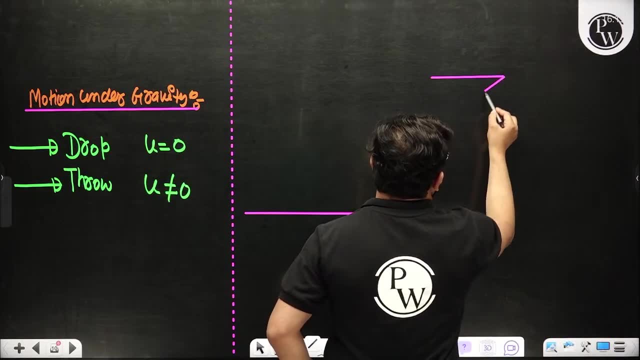 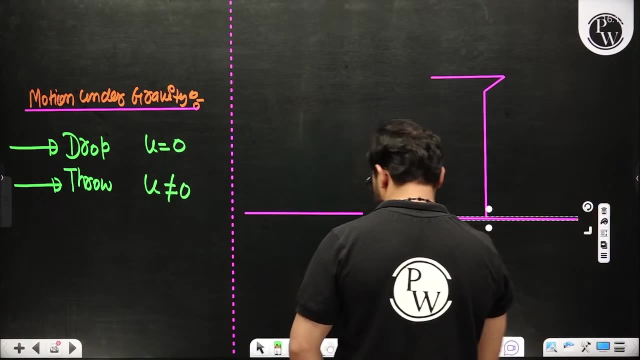 If I say this question in your question, Suppose you have the ground- Please see carefully, This is my ground. and in another case, suppose this is a building tower and we will take the height of this tower. Suppose the height of this tower is h. 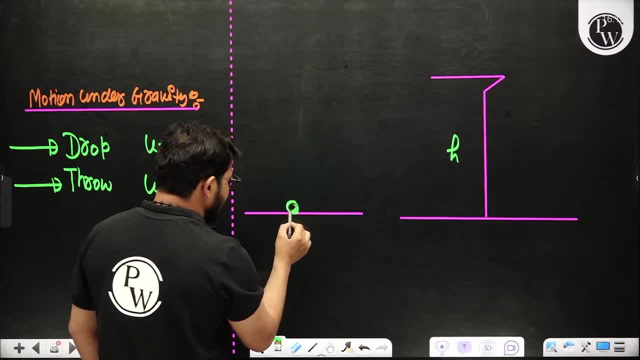 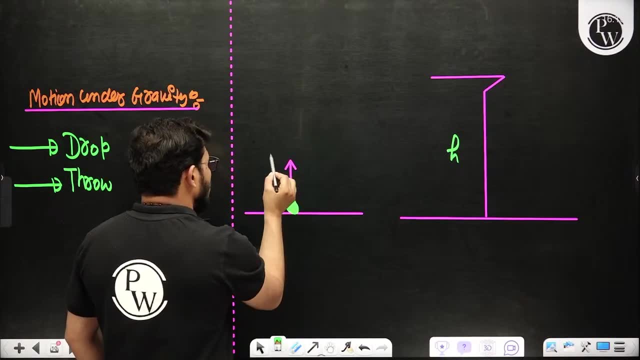 What did you do? You took a ball here. Listen to me please. What did you do to this ball? You just threw it upwards. What did you do to this ball? You just threw it. This means that you have original velocity u. 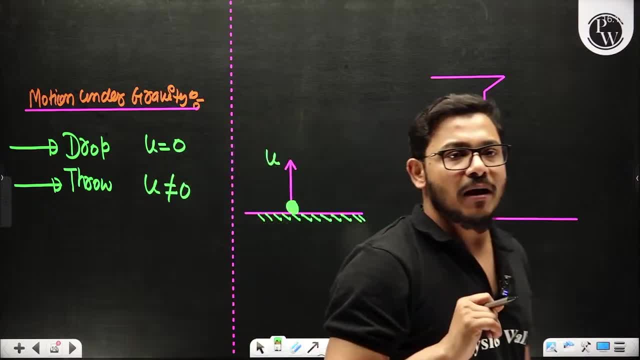 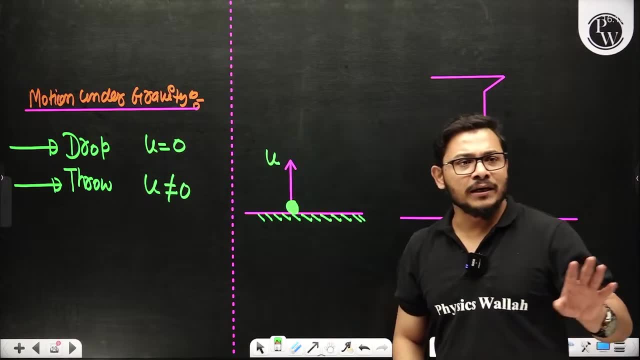 Now I will ask you one thing. Please tell me one thing. All the students will message me once. Tell me quickly, When you have thrown this ball: is the motion under the gravity? Where is the motion? Is it under the gravity? 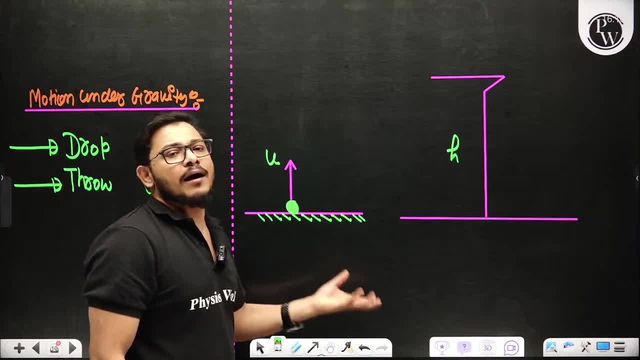 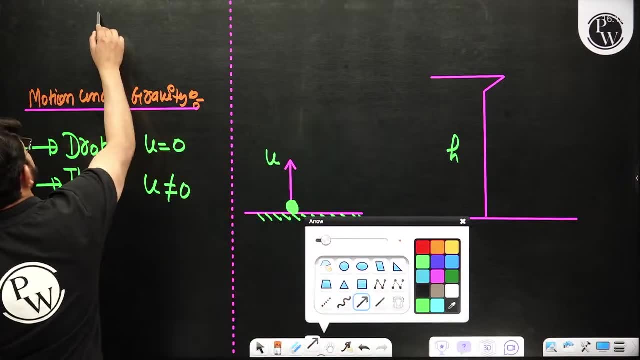 When you have thrown the ball, tell me where will the acceleration work. The motion is under the gravity. Always remember my words. Whenever any particle is under the gravity, the motion under the gravity moves. Whether the ball goes up or down, the acceleration always works downwards. 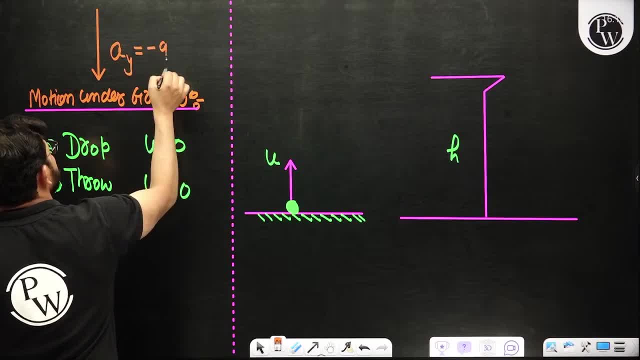 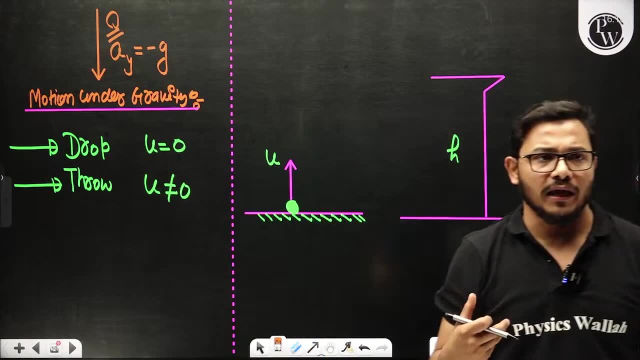 And the acceleration is in the y direction And it is always minus g. What are you saying? I am writing absolutely right. The motion under the gravity means that the acceleration of the particle will always work downwards. I hope, guys, you got the concept. 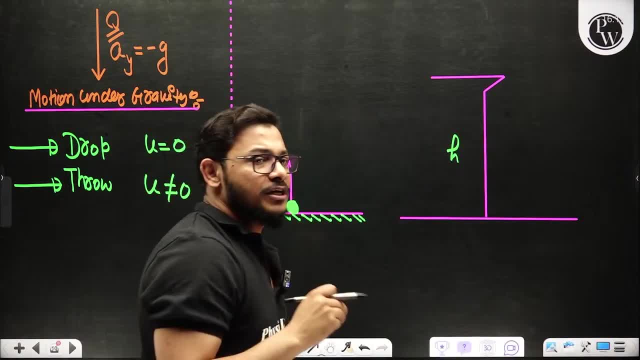 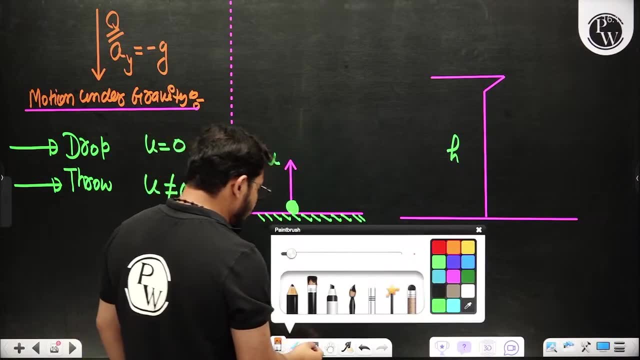 You understand what I am saying, That the motion will always work under the gravity, Because where is the acceleration working? It is working downwards. Now listen to me. I want to ask you one thing. You will tell me the answer. Suppose this particle is moving upwards. 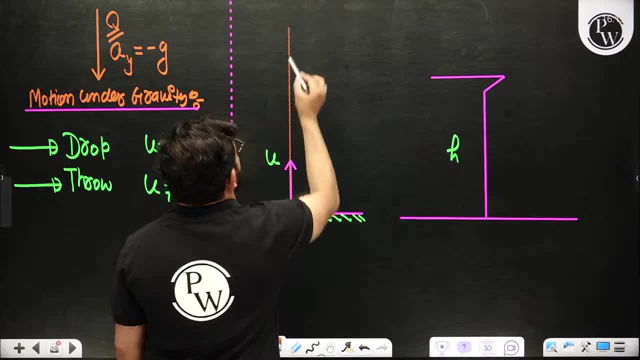 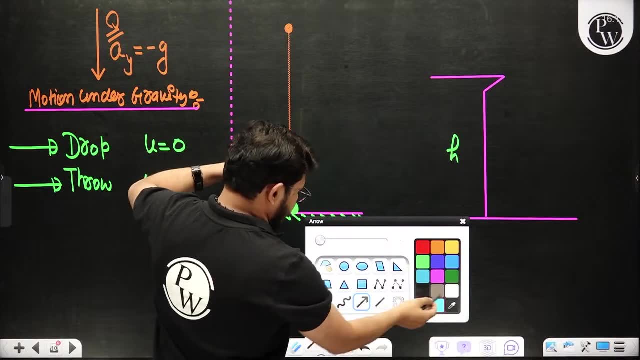 Suppose it goes up till here. I want to ask you one thing: It went up till here. Why didn't it go up after this? Listen to me. Where is the velocity? It is upwards. Where is the velocity It is upwards? 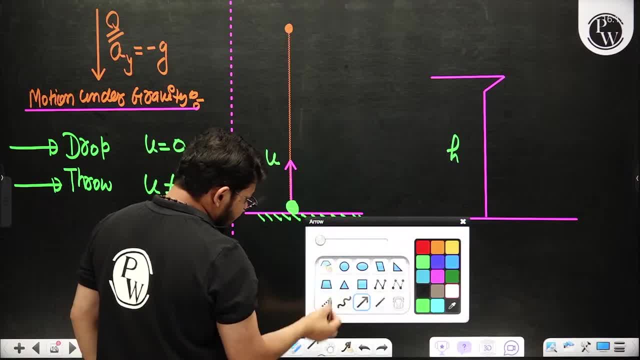 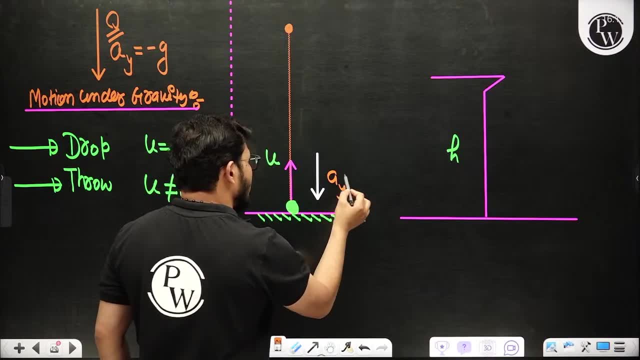 So the motion is also upwards, But it is moving under the gravity. So if I talk to you about its acceleration, you will say that the acceleration of the particle is going downwards. The acceleration of the particle is minus g. Where is the acceleration of the particle of y direction? 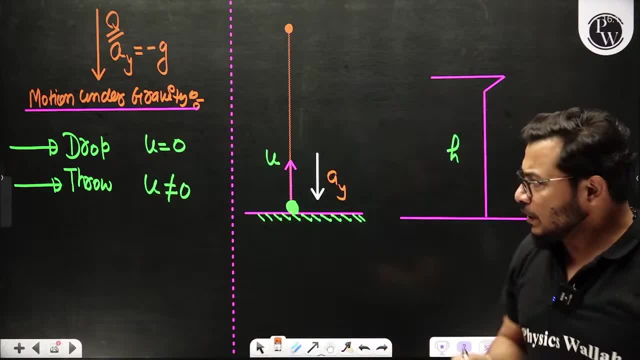 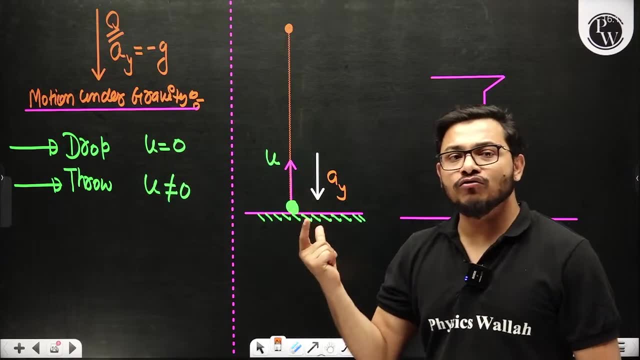 It is going downwards. I was asking you one thing. Tell me one thing: Where is the velocity and acceleration? Message me and tell me How are the velocity and acceleration of both of them. How are the velocity and acceleration of both of them? 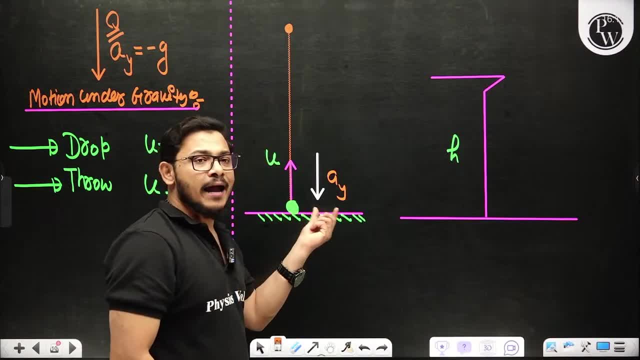 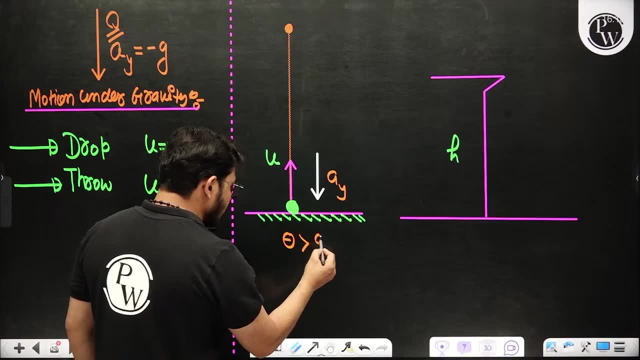 They are opposites. How are the velocity and acceleration of both of them? They are opposites. What is the angle between the two? It is 180 degrees. So is this angle greater than 190 degrees? Absolutely correct If the angle is 90 degrees. 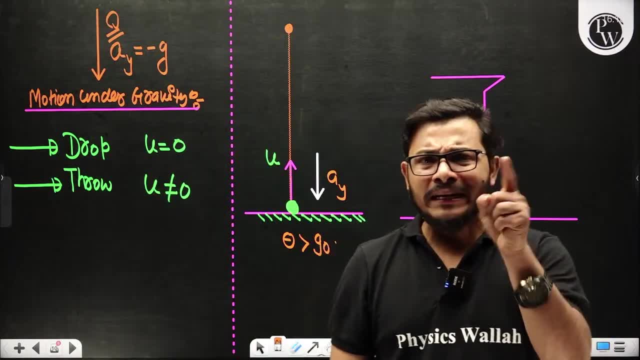 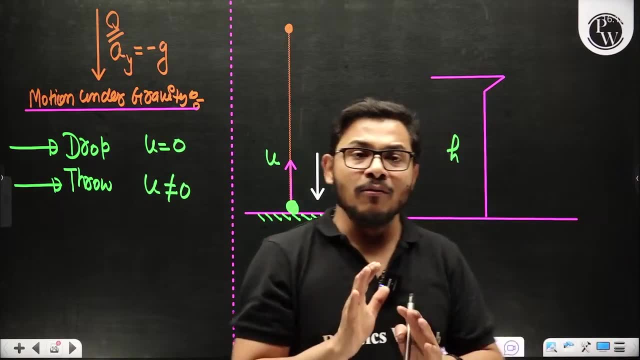 if the angle is 90 degrees? if the angle is 90 degrees, then what will be the velocity? Speak quickly. What will be the velocity? It will decrease. The magnitude of the velocity is decreasing. If it is decreasing, it means that if you throw this ball from 20 meters per second, 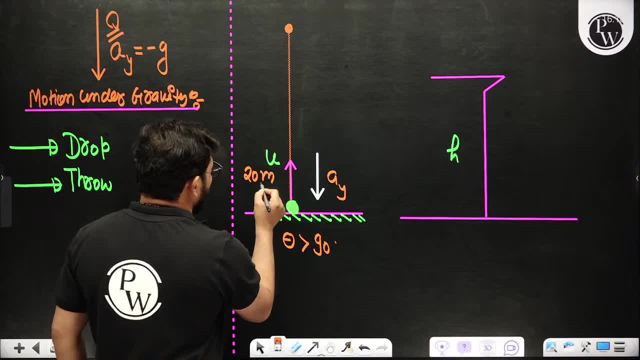 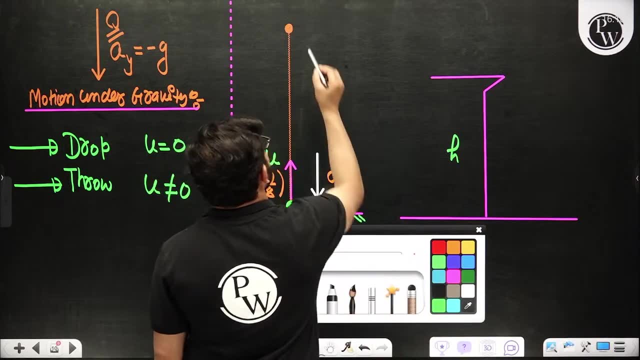 if you throw this ball from 20 meters per second, then the velocity of the ball is decreasing slowly as it goes upwards And as it decreases, its velocity becomes zero. What is its velocity? It becomes zero. I am talking about the Y-direction. 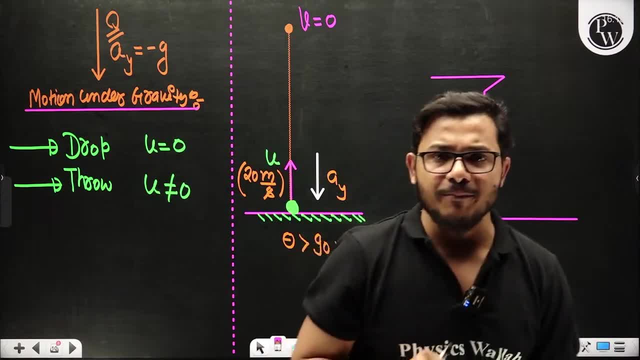 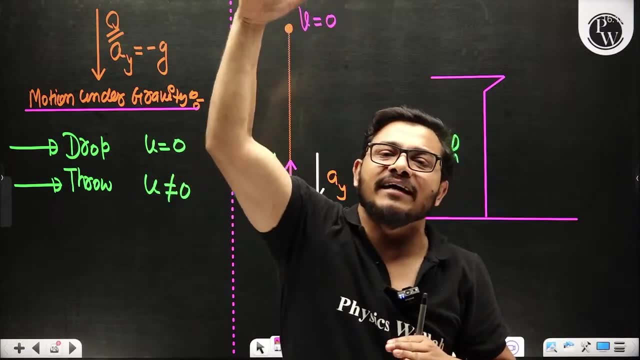 Remember one thing: if someone asks you that you threw a ball upwards, it goes upwards, it goes upwards. Till when will it reach the maximum height? So you say that when you throw a ball upwards, it is going upwards, it is going upwards. 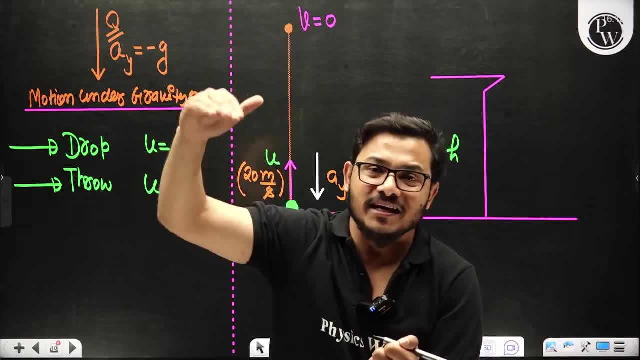 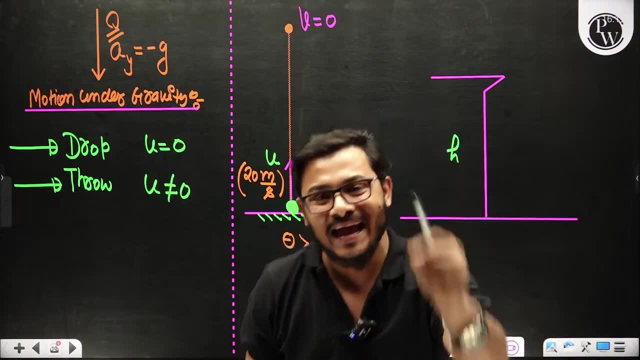 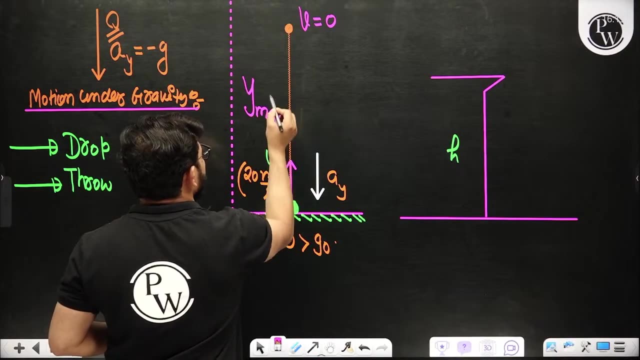 Till when will it go upwards? Till the time its velocity becomes 0 in the Y-direction. When the velocity of the Y-direction becomes 0, it will be called the maximum height, So from here. So this height, from here to here is your maximum, and you can also write this as capital H. 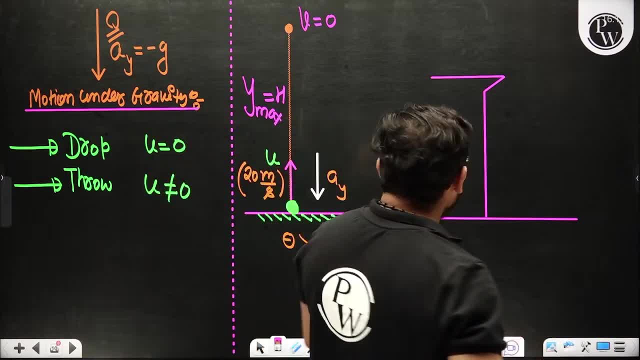 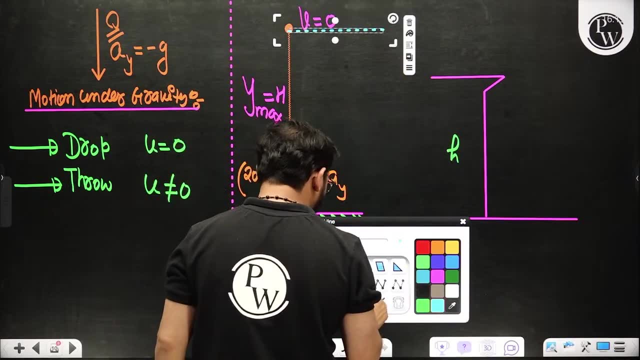 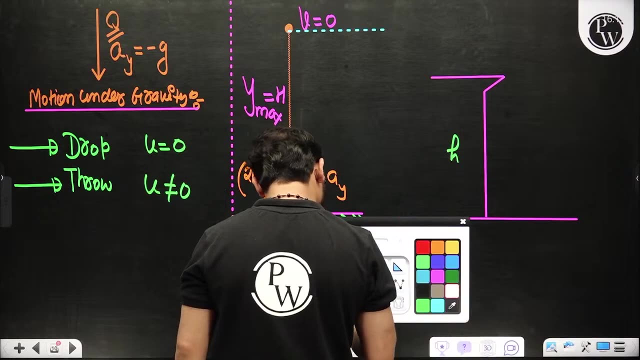 That one is called maximum height. After that, what will happen? That particle will come down from here. That particle will come down from here. Now that particle is coming down from here, Please listen again for one minute. Now that particle is coming down from here. That particle is coming down from here. 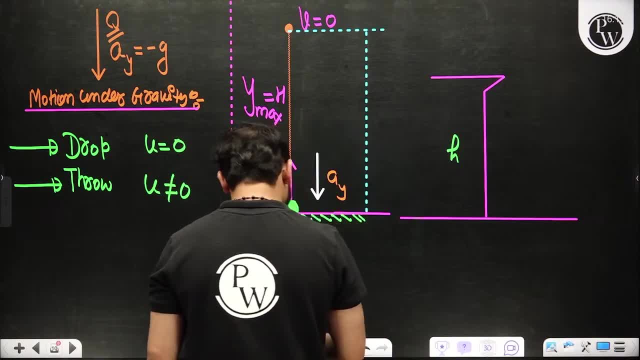 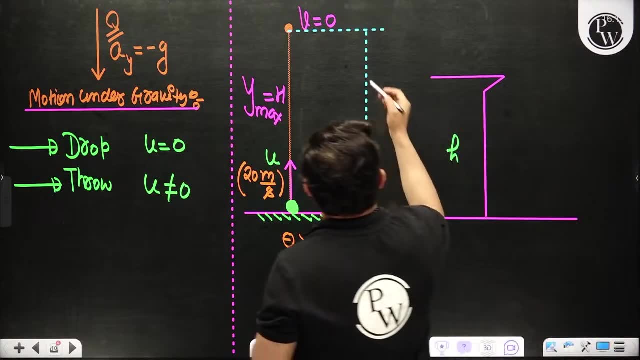 I will ask you a very interesting question. You will tell me: Look what I am explaining here. This type of questions are going to be made in SSC, JEE. Now listen to me. that particle is coming down from here. Now, when it will come down, Adil, tell me what will happen. 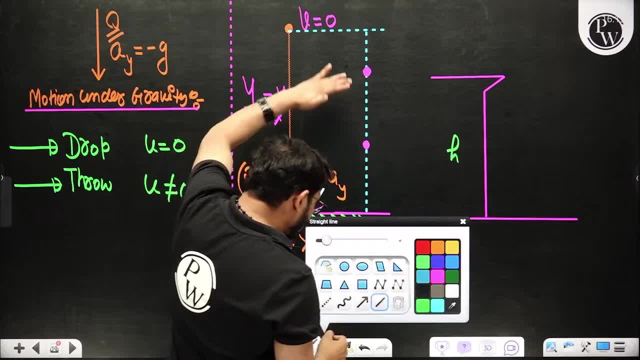 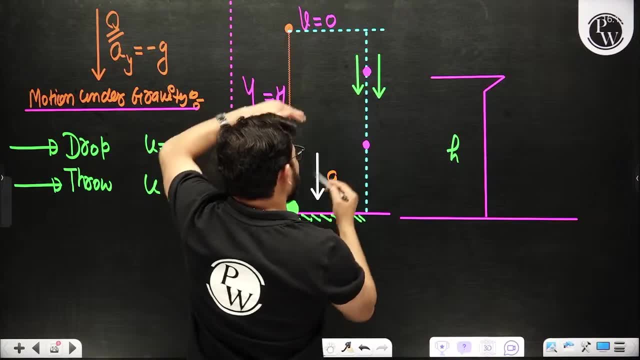 You tell me When that particle is coming down from here, Then where is the direction of motion? The direction of motion is going down from here And where is the acceleration? It is also going down. You are understanding right. What is the direction of motion? Where is the velocity? 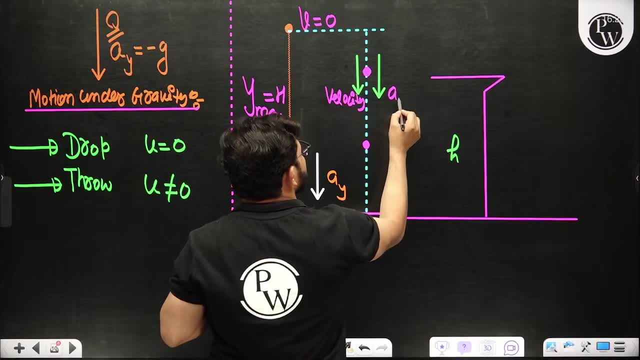 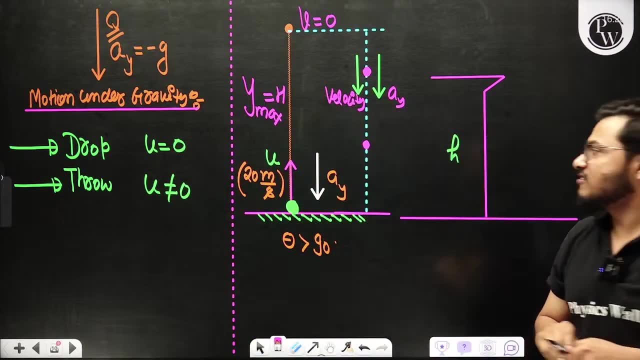 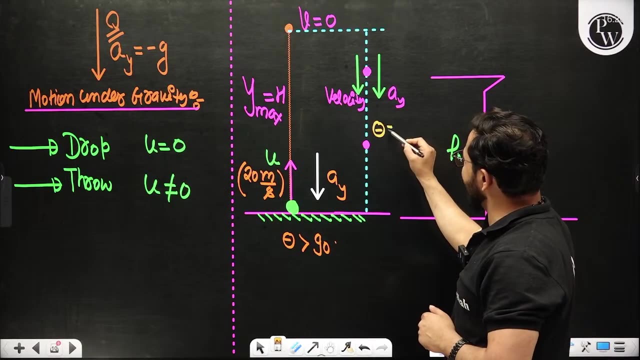 Downward. And where is the acceleration Downward? Why is acceleration going down Now? where is the velocity and acceleration? Quickly type the answer: Where is velocity and acceleration? They are in same direction Now. when they are in the same direction, then, what is the angle between them? 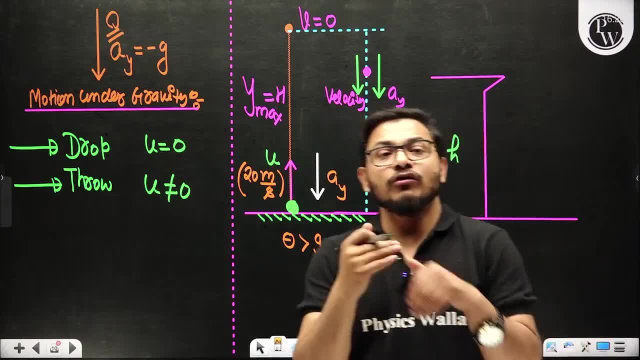 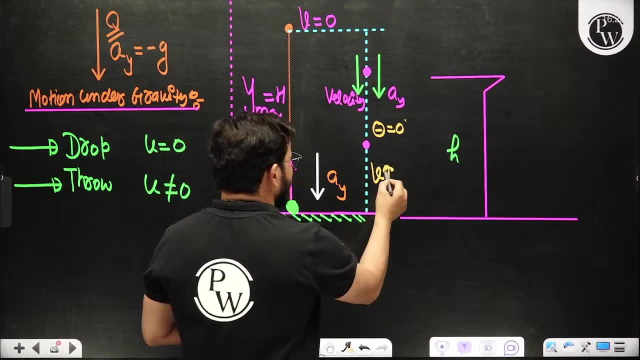 Zero degrees, Then if the angle is zero degrees, then what will be the Magnitude of velocity? It will be increase. What is the Magnitude of velocity? Its becoming increase. the magnitude of the velocity will be increased. so, please, you have to remember that I am explaining in which way. 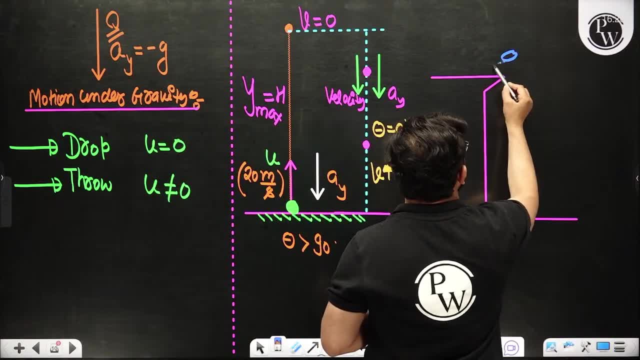 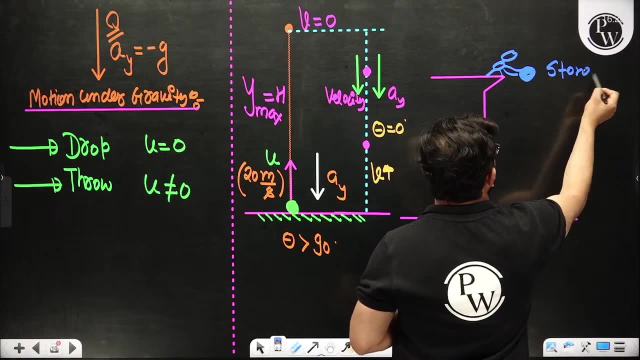 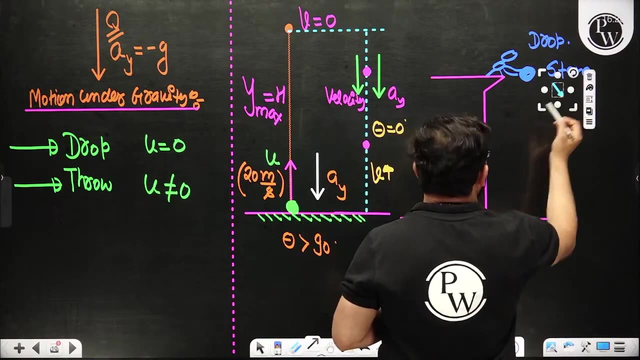 here also the same thing happens, like suppose there was a brother here and he was standing on the tower and he had a stone in his hand and he dropped the stone from here. when he dropped the stone, then what will be the velocity of the stone now? the original velocity will be 0, but you dropped the stone. 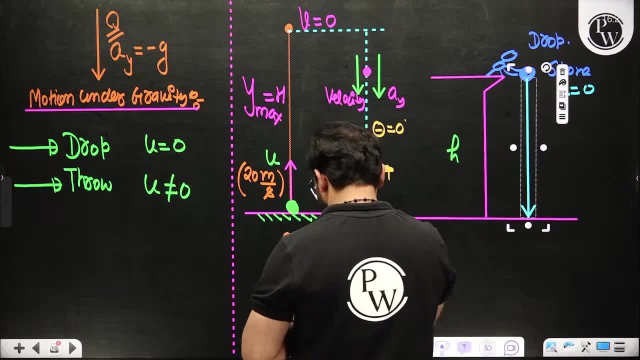 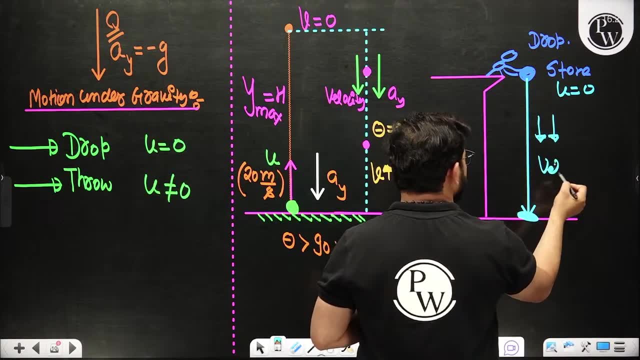 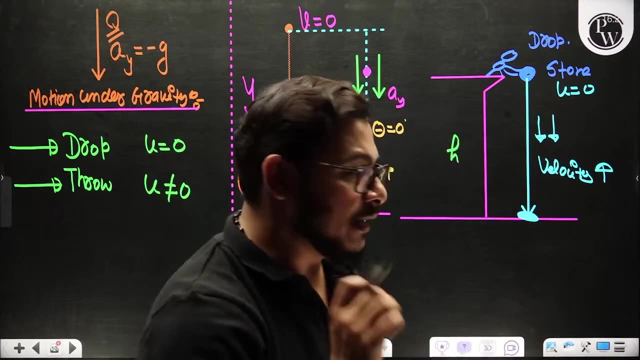 when you drop the stone, then the particle will come down and hit the ground, and when it comes down, then the velocity will come down and the acceleration will come down. so the magnitude of the velocity will be increased with the time. how many of you have understood the concept? 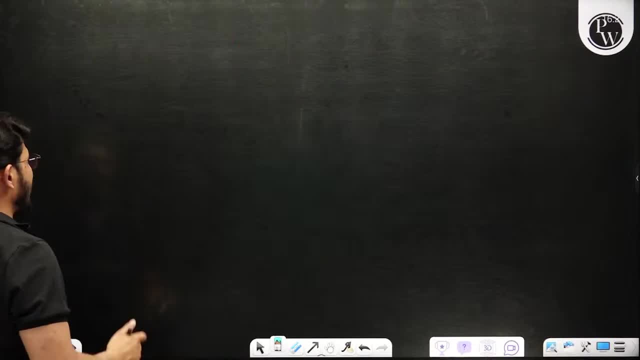 so this is called uniform acceleration. I am going to write one thing in the note. if I write any concept in the note, then you will understand the point which sir has written. it is a star point. if I write anything in the note, then you will understand the point which sir has written is a star point. 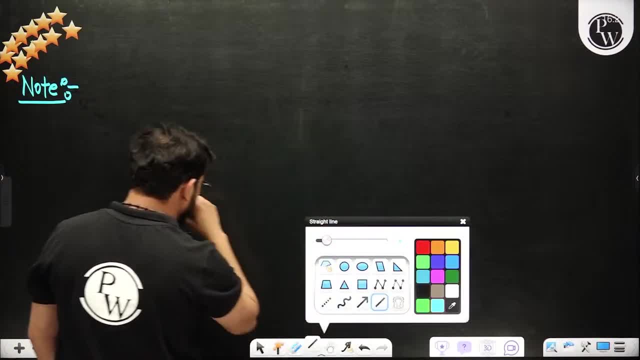 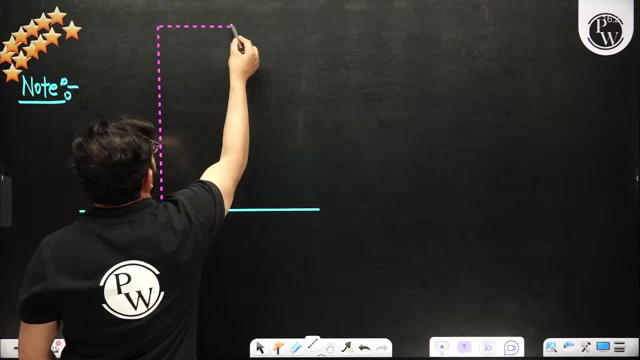 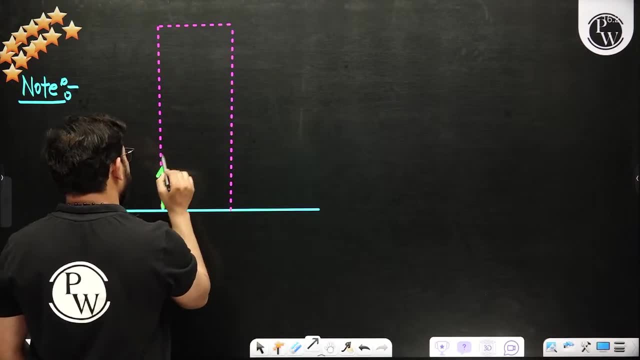 by the way, it will come down on this path, but I am making it down by doing it on the side. and then it came down. this is what happened first. where did that particle go to you? that particle first went up. then where did that particle come to you? 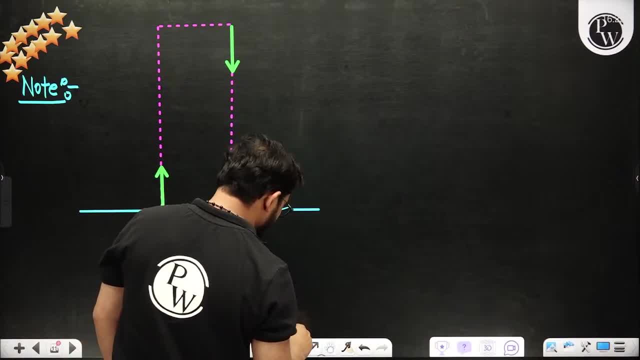 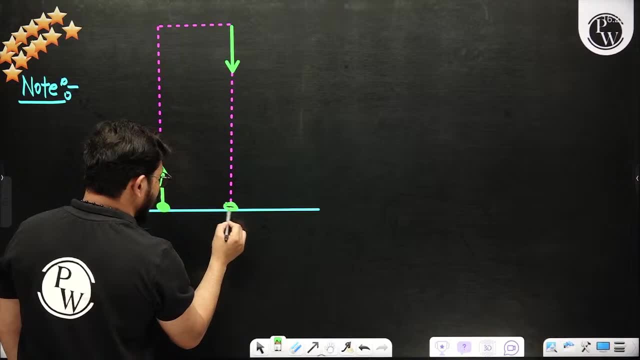 it came down. this is what happened. now I want to ask you one thing. please tell me one thing. listen first, that particle was here, went up from here, then it came down slowly and hit the ground here. suppose you gave the original velocity to the particle like this? 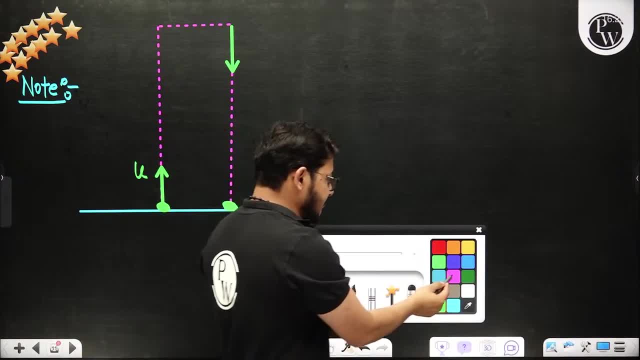 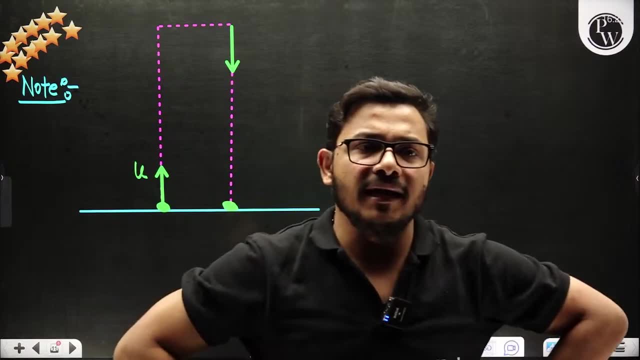 how much did you give? I will tell you one thing: please go back and see for one minute. ask me one thing. I will tell you one thing: when the particle is going up, when the particle is going up, then the velocity is decreasing. who is making the velocity decrease? 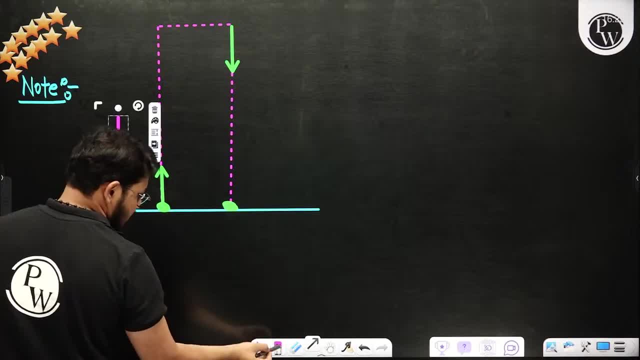 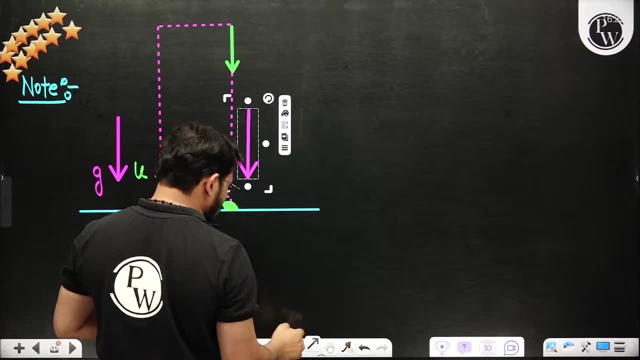 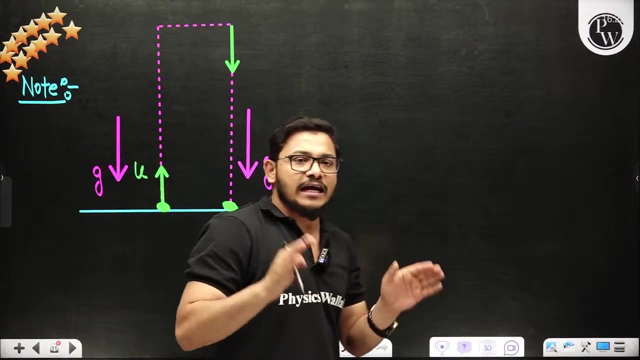 who is making the velocity decrease? acceleration? acceleration- how much is that small of g when that particle is coming down? then who is making the velocity increase? acceleration. so when the velocity is increasing and when the velocity is decreasing, are both the accelerations same. 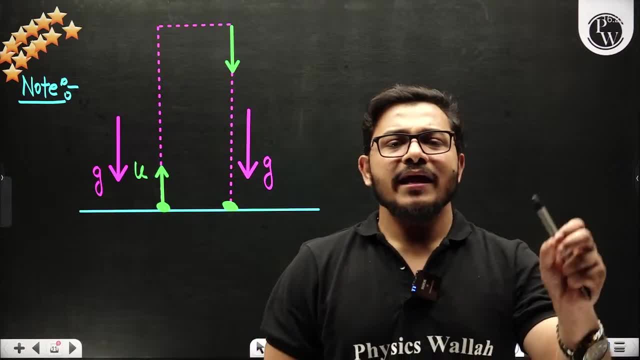 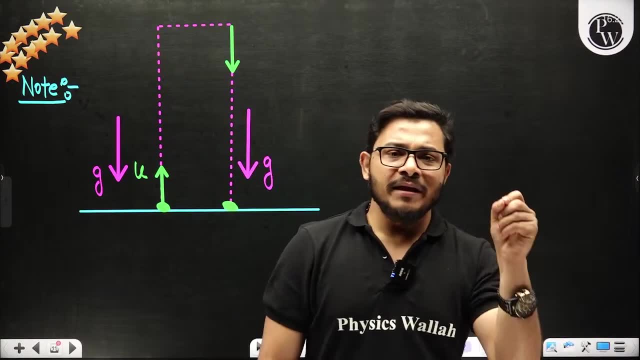 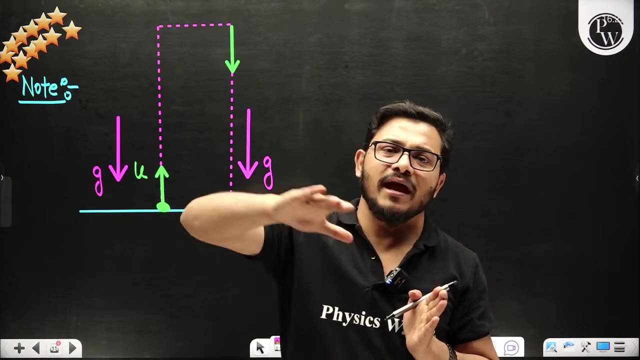 suppose let's understand a small example. you invested money in a company. suppose you work in a share market. you invested money in a company. when you invested money in a company, suppose the growth of your money, suppose it is increasing by 5% in an hour. so the money increased by 5% in an hour. 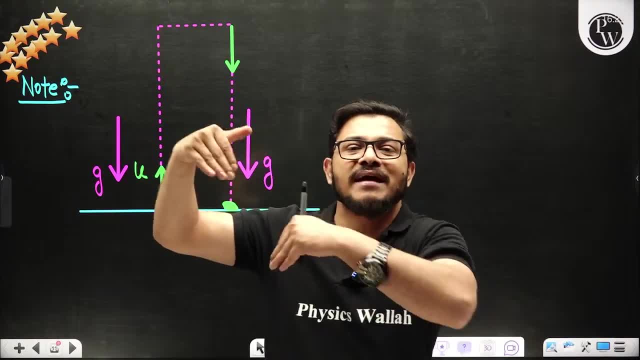 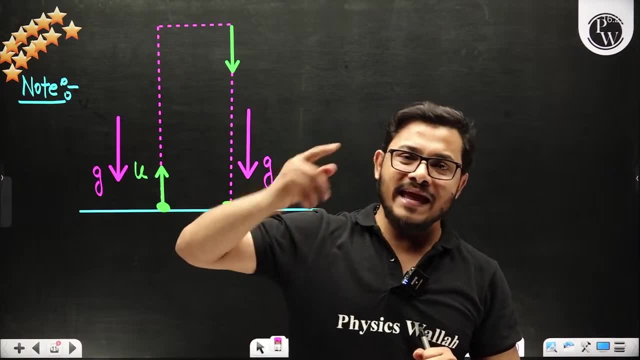 in the same rate means your money is increasing by 5%. suppose for an hour your money is increasing by 5% now, after some time, after an hour, for an hour then it is decreasing by 5% rate only. so what are you seeing? 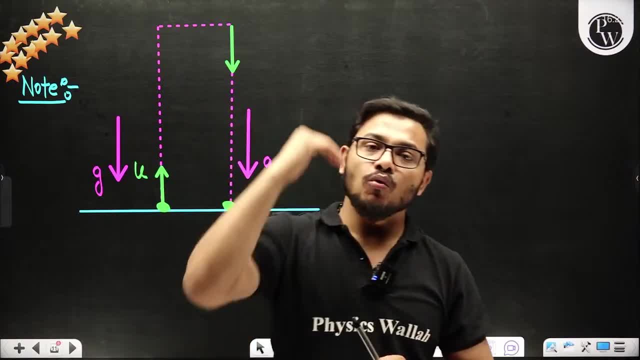 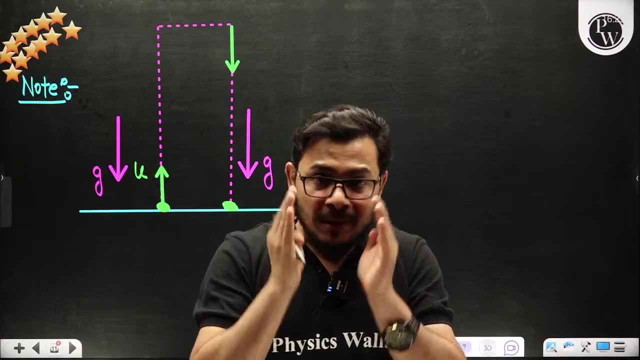 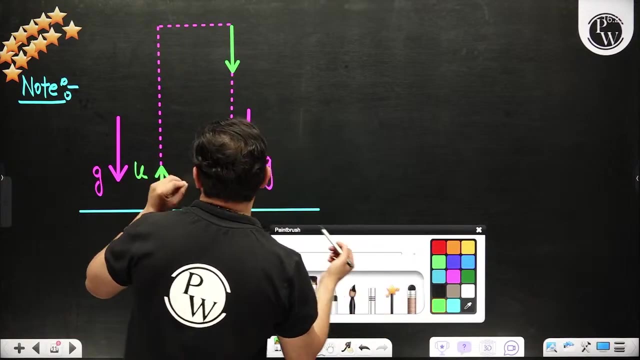 the rate at which your money increased, the rate at which your money decreased. what does it mean? it means that, at the same time, the value of your money will be same. I mean to say that when you, I mean to say that, at the same height, your velocity will be same. 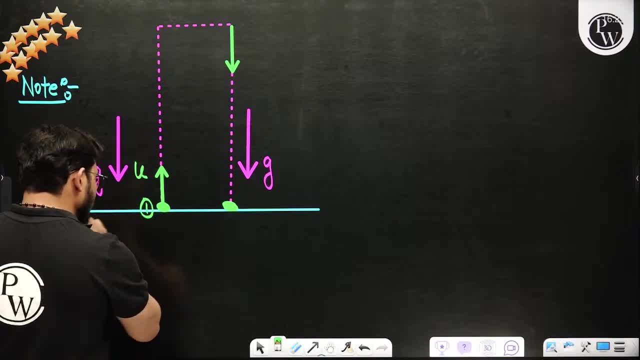 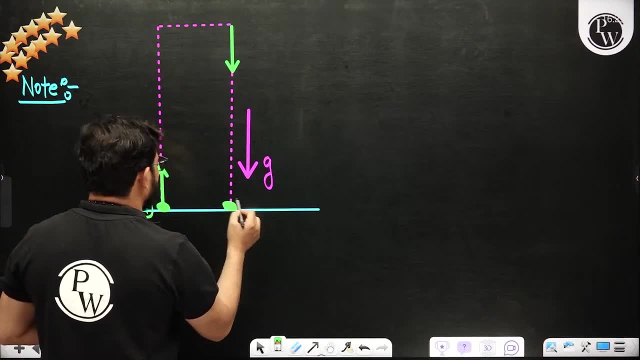 tell me at this point, if this is point no.1, I will ask you: what is the value of height here? here, the value of height is 0. now, suppose this is another point. suppose this is another point. suppose this is the number. this is the second point. 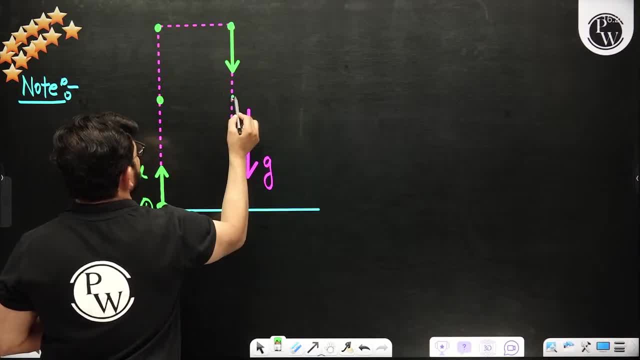 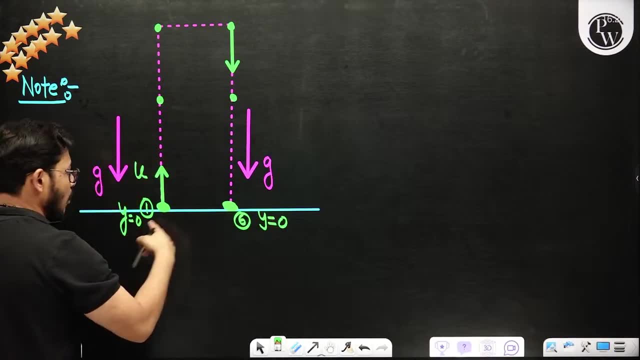 this is the third point, this is the fourth point, this is the fifth point and this is the sixth point. at the sixth point also, the value of height is 0. so at point no.1 and point no.6 the height is same on both. if the height is same on both, 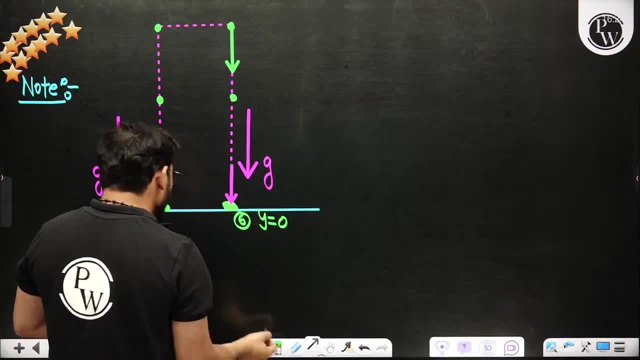 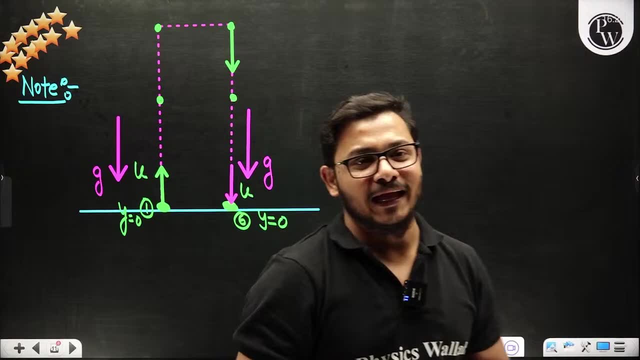 then remember, at the same height the same velocity will be there. so if you have thrown the velocity to the particle from U, then remember it will come to the ground and will collide with U. only what a wonderful thing you are saying means you said an amazing thing. 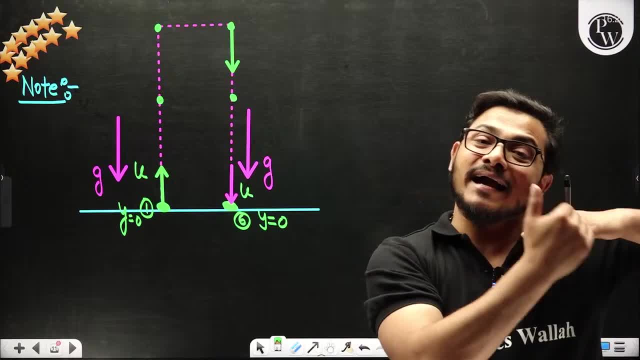 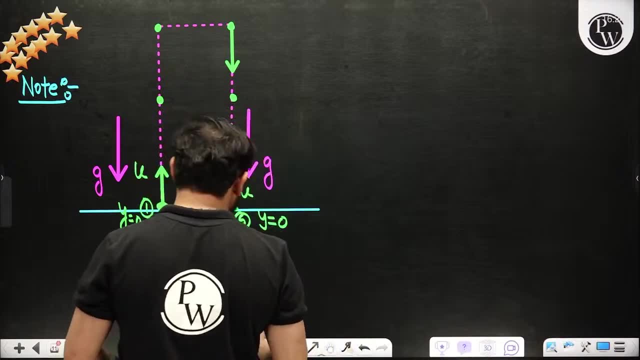 means at same height, same velocity. why? because the work of increasing velocity and decreasing the work, who is doing it, is same acceleration. velocity is increasing at same rate. velocity is decreasing at same rate. that means velocity will be same at same height if here the particle is going to the top. 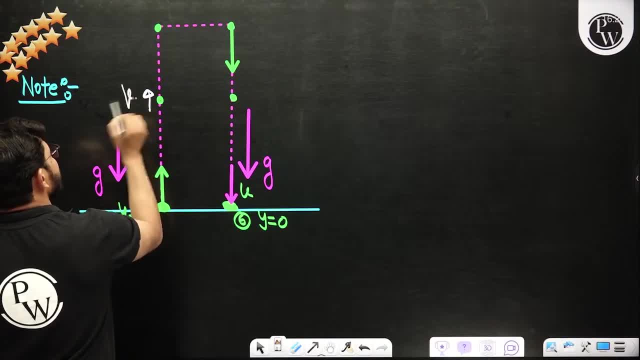 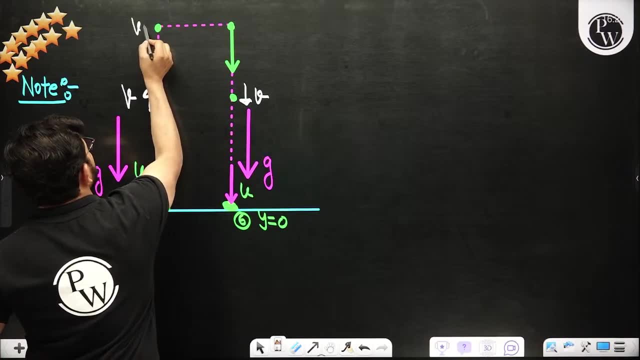 suppose if the velocity of particle is here, suppose it is V, then remember, at the same height I will see the velocity of particle at this point. suppose if the velocity of particle is here, then How much velocity of particle will I see? here I will see only zero. 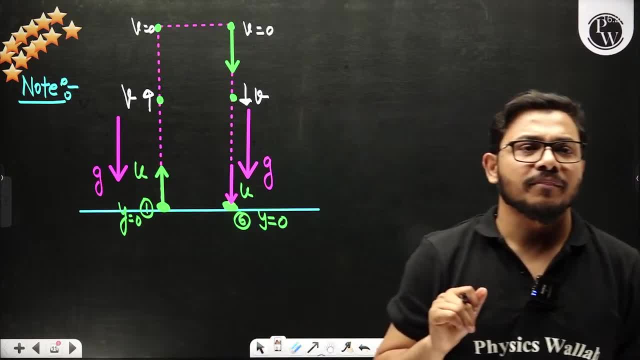 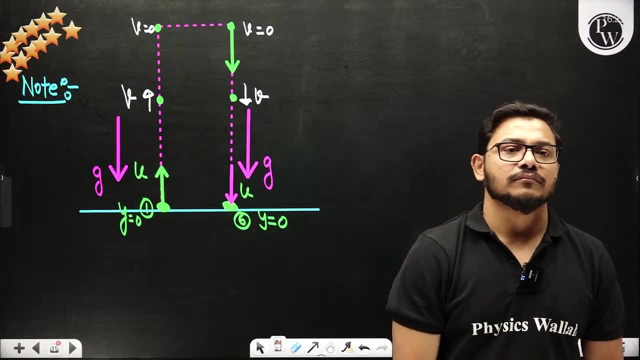 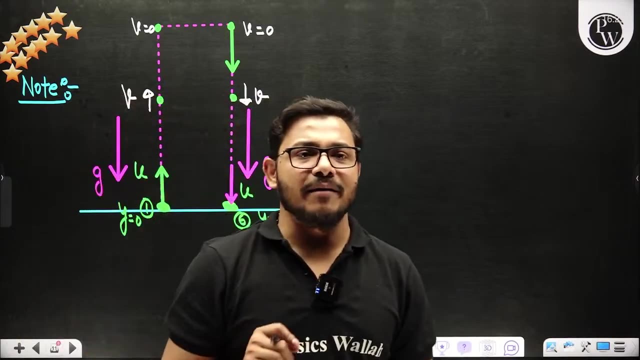 Same height, but same velocity, Did you understand? So, same height, but same velocity, Did you understand? Did you understand? I did not read anything wrong. Please listen carefully. Same height, but same velocity, Because of you know very well what is actually happening. 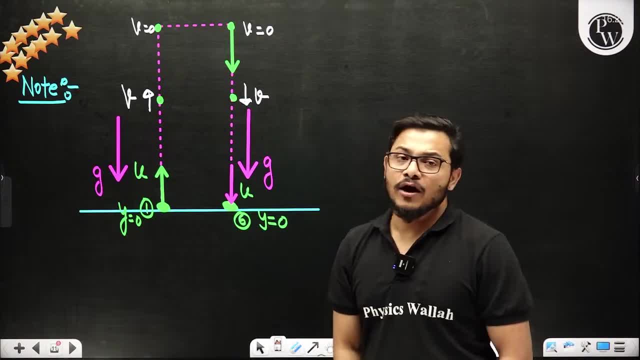 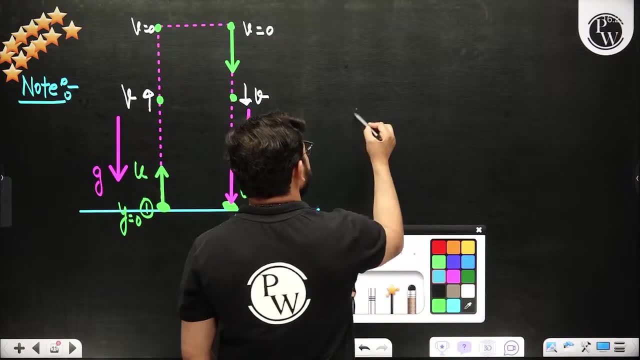 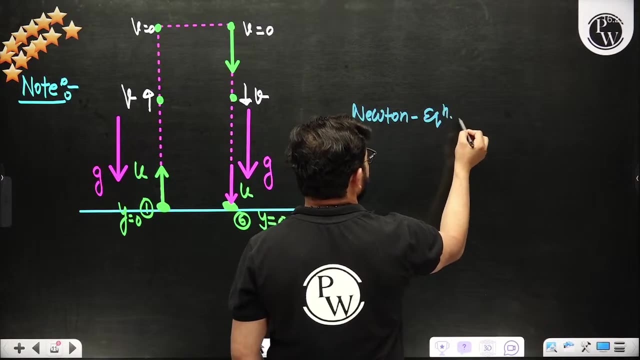 Increasing velocity and decreasing velocity is done by acceleration. And where will you get this story? Where will you get this story? I will prove it to you, Don't worry. It will be made by Newton's third equation of motion. Newton's equation of motion will be made from there. 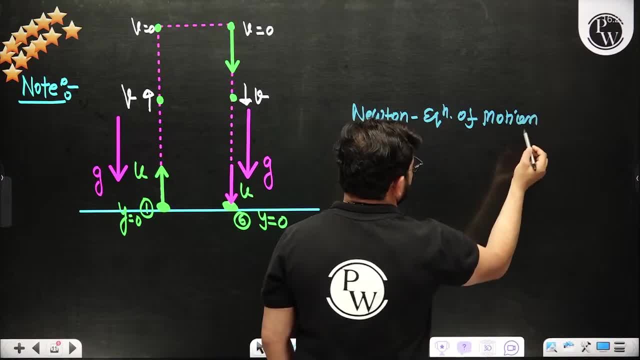 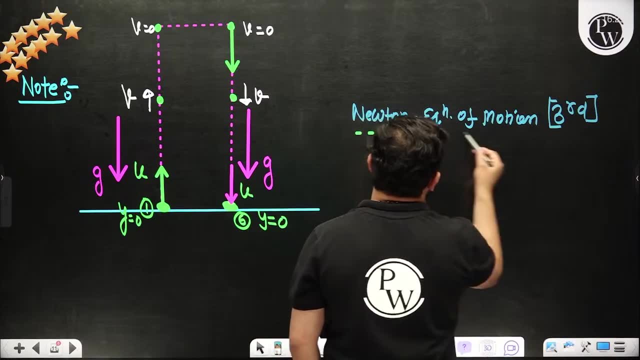 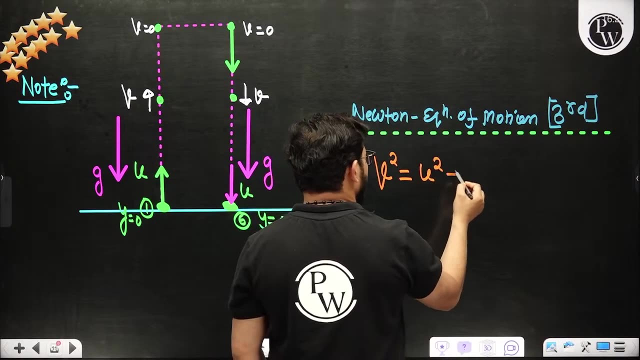 Newton's equation of motion. Third equation of motion. Third equation of motion. And what is that equation? Please listen carefully for one minute. What will be? that equation will be that equation: like final velocity square become is equal to u square plus of. 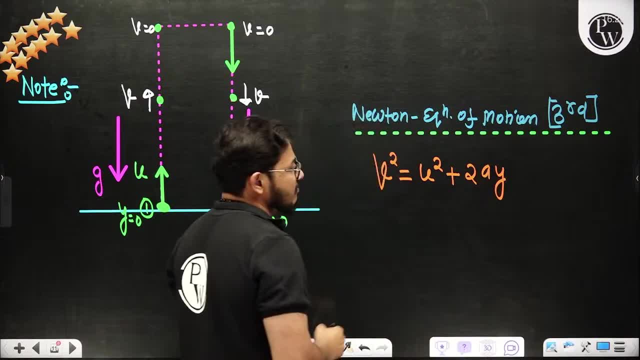 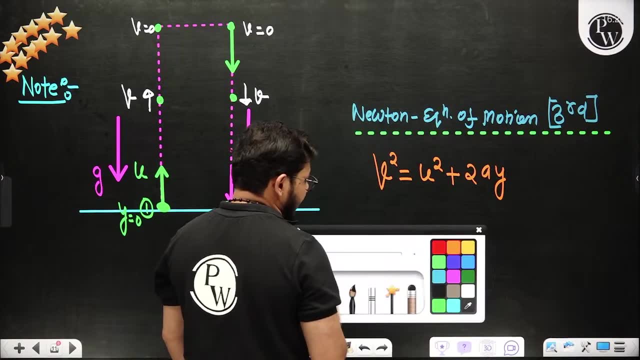 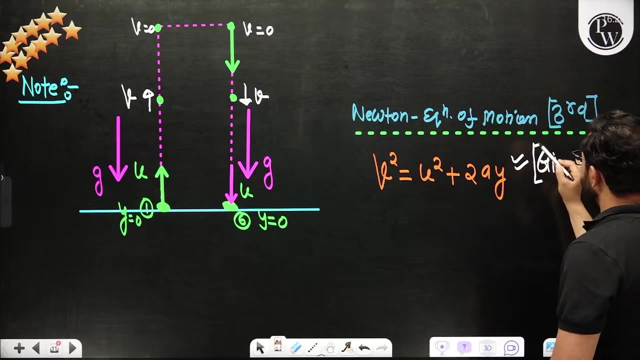 the 2 ay. this is what happens: v square is equal to u square plus of 2 ay. this is the third equation. if I ask you that, if you have any given height, if suppose, if you have any y given y, if you have any y given, then at any given height, if I ask you, tell me the. 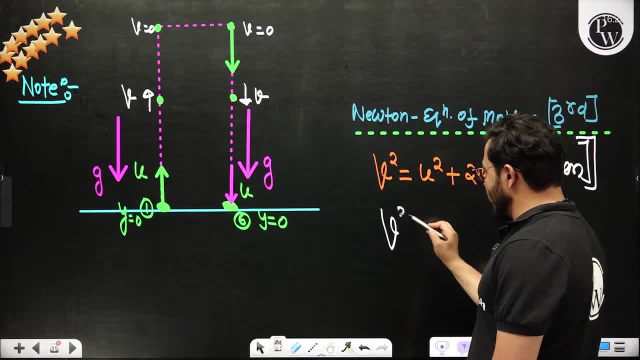 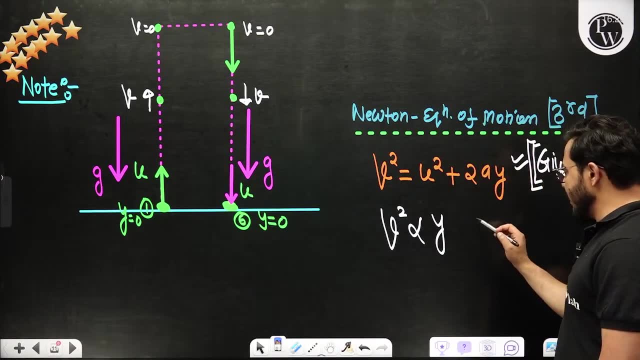 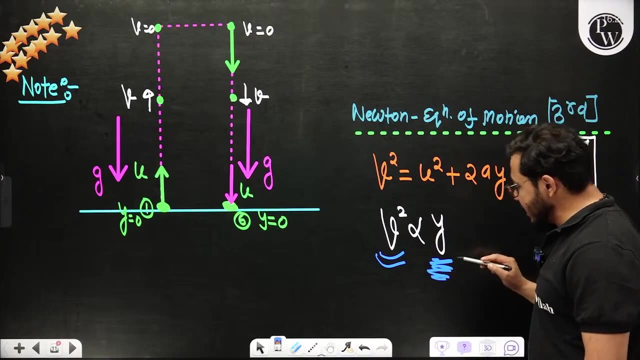 final velocity value of v, how much it will be. so v square is proportional to y. so this is a quadratic equation. what kind of equation is this? it is a quadratic equation. so quadratic means that for same y, same y. listen to me the one who told me that you told wrong mathematics. 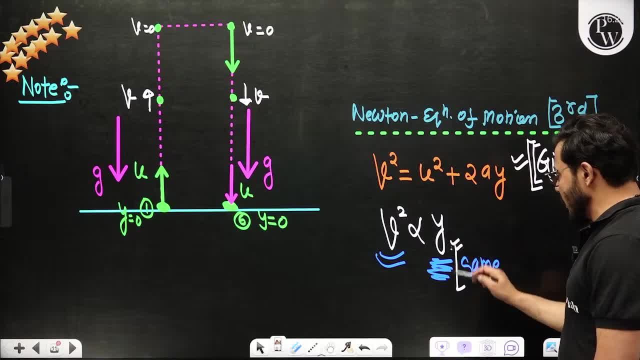 listen to me. I didn't want to get into mathematics, you told me, so I came in. same y same y. how much value of v will be same y same y. how much value of v will be same y same y. how much value of v will be. 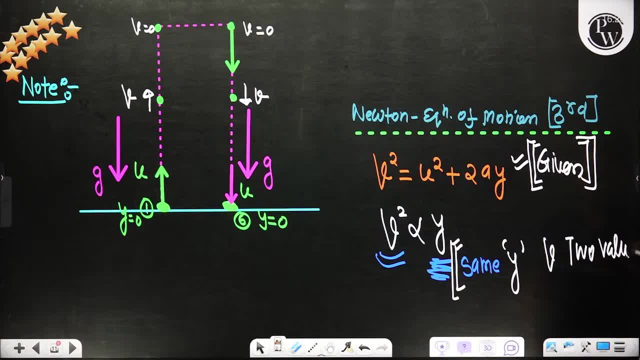 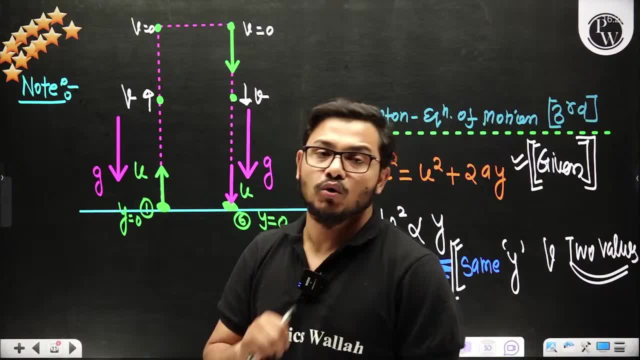 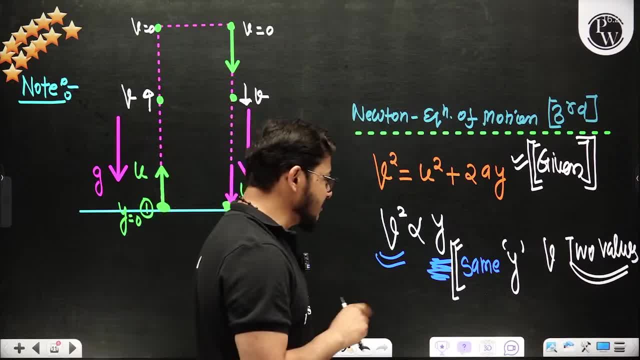 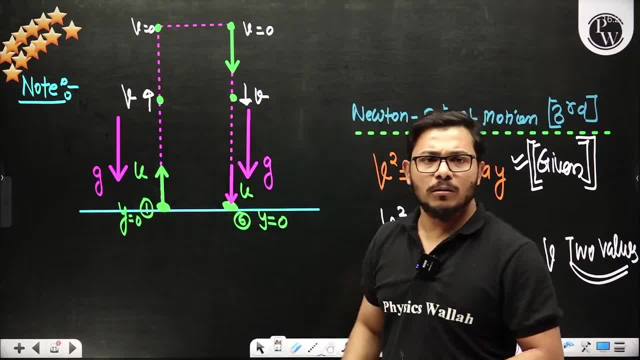 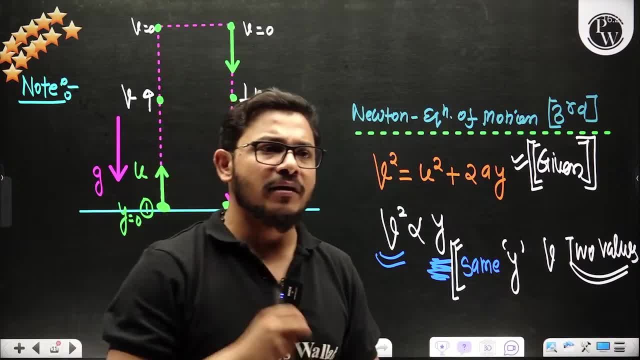 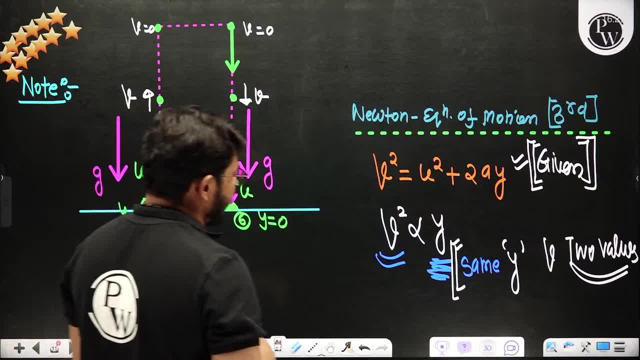 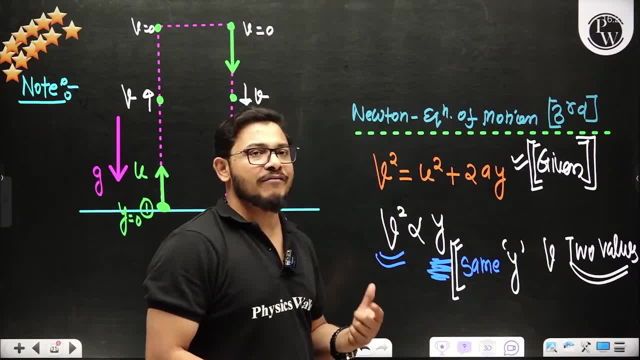 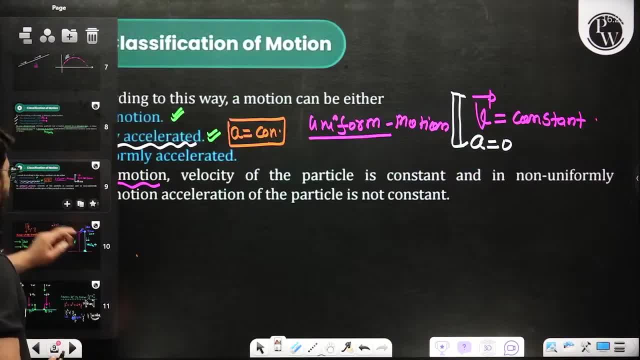 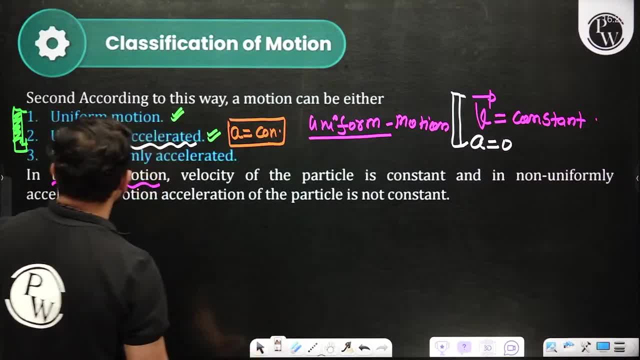 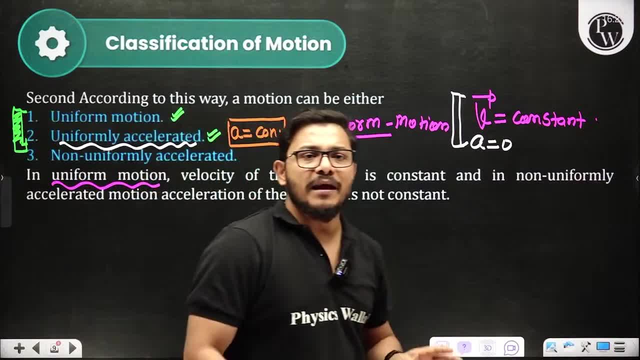 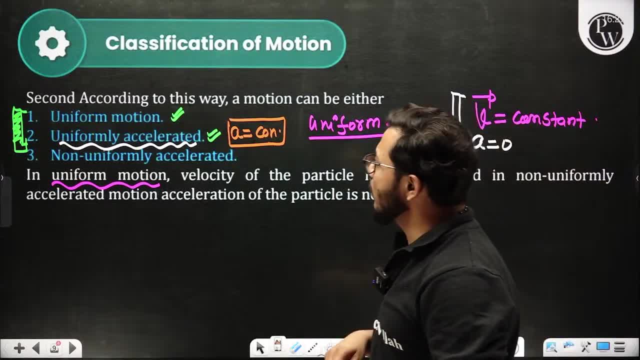 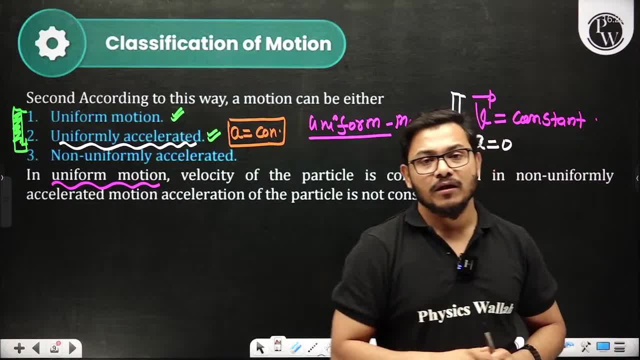 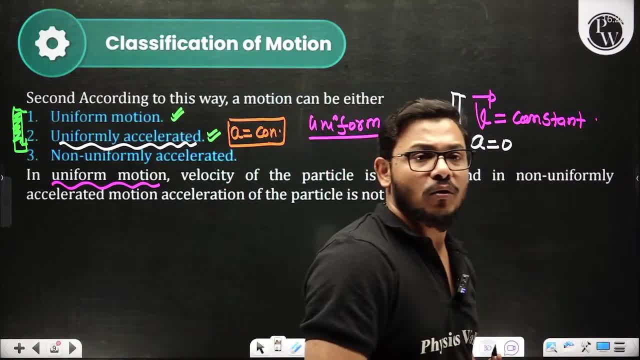 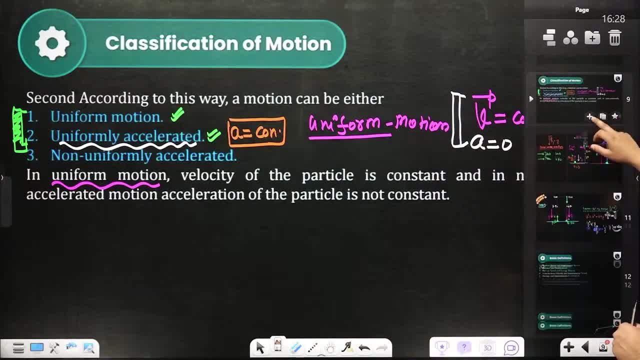 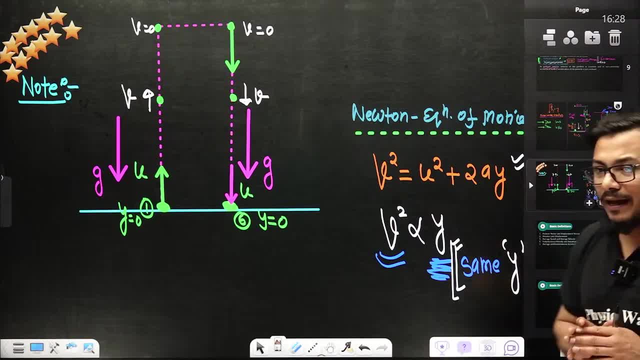 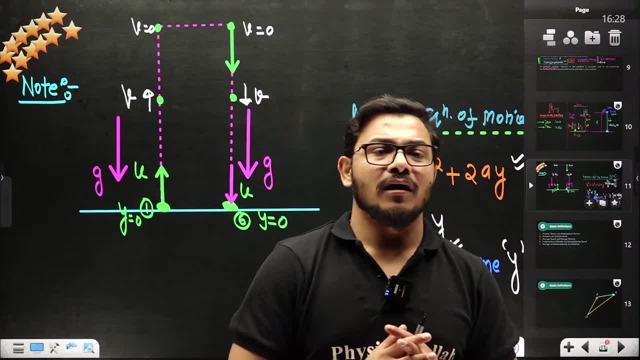 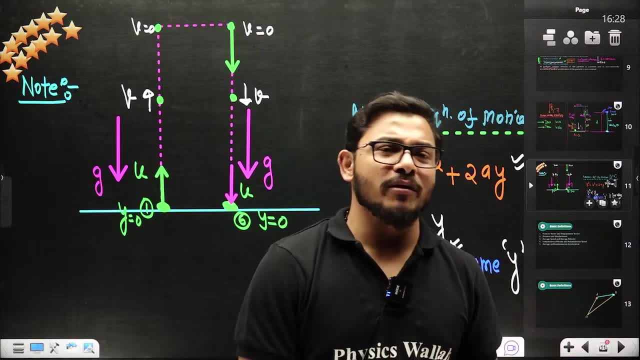 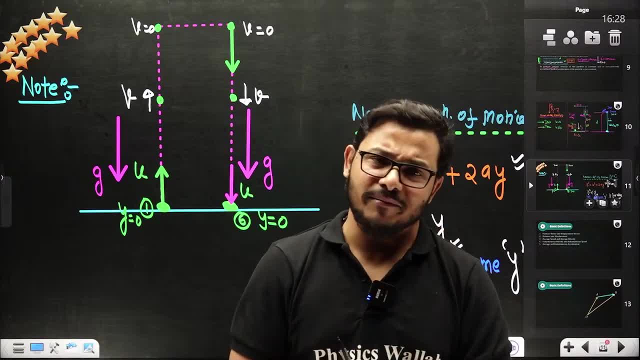 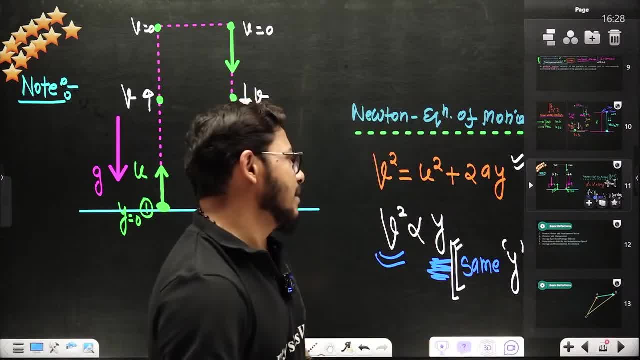 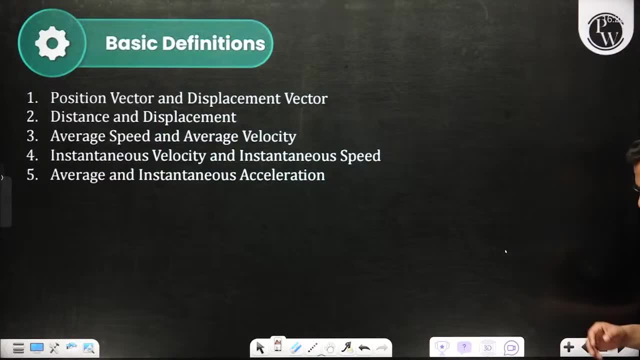 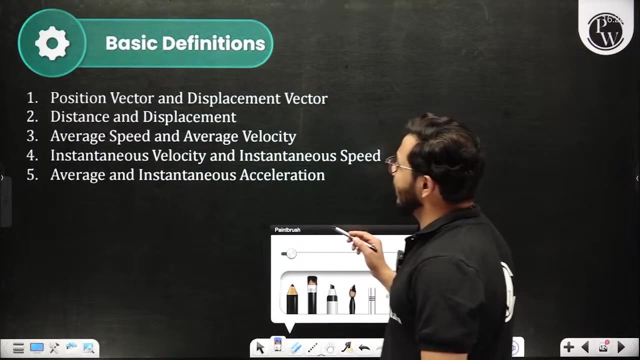 they will become different. don't go in aptitude now. what am I going to talk about? I am going to talk about basic definition now. actually, I am going to talk about motion, what I have to teach you in basic definition. first of all, I have to tell you: 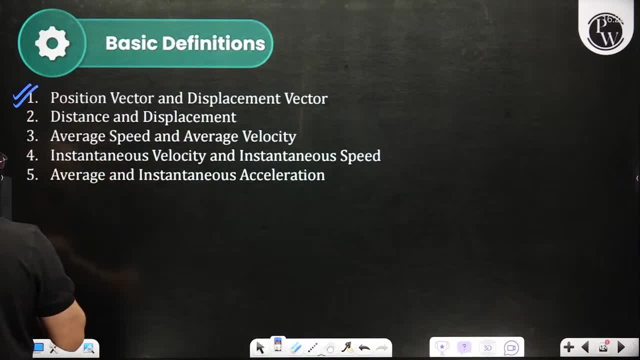 how to calculate position vector and displacement. then what is distance and displacement, average speed and average velocity? what is a particular instantaneous velocity and what is instantaneous speed? what is average acceleration and instantaneous acceleration? first, I have to tell you all these things one to one. first of all, I am going to talk about 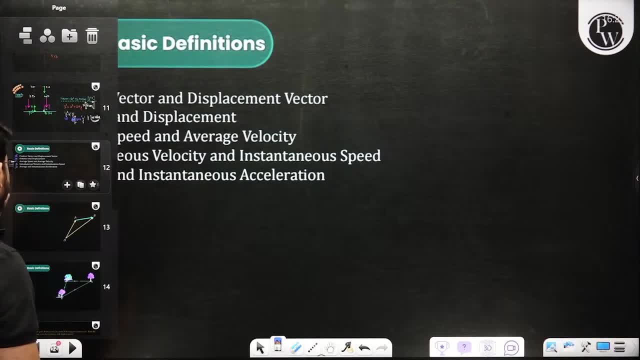 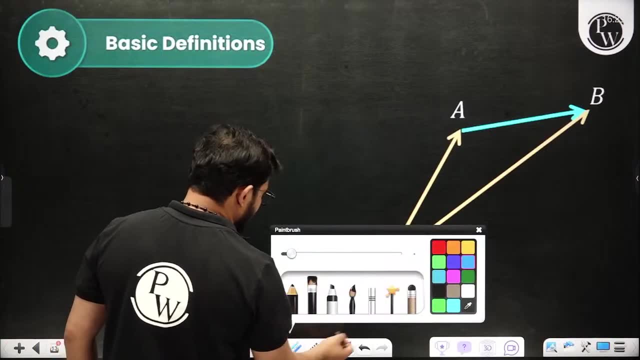 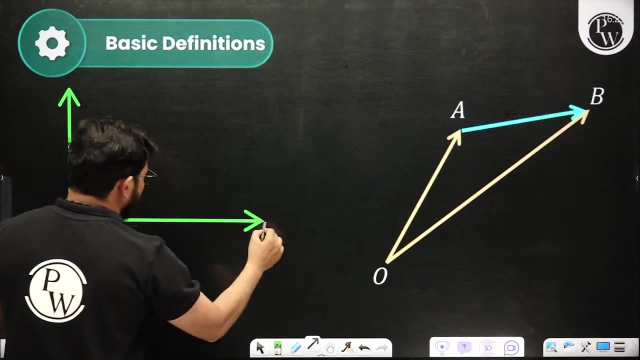 position vector and displacement vector. please understand all these things again. what is the position vector and what is the displacement vector? first of all, I am going to talk about position and displacement. listen carefully. suppose I have a plane. tell me once, son, if I tell you that my house is in xy plane. 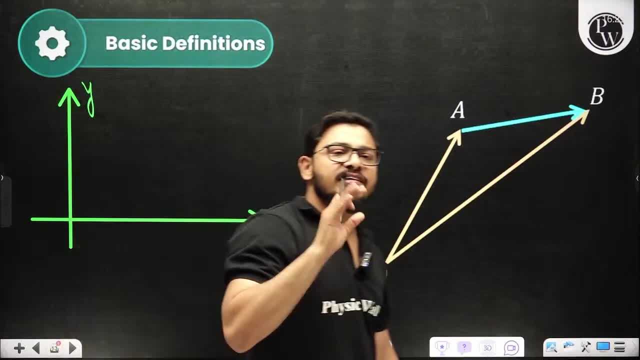 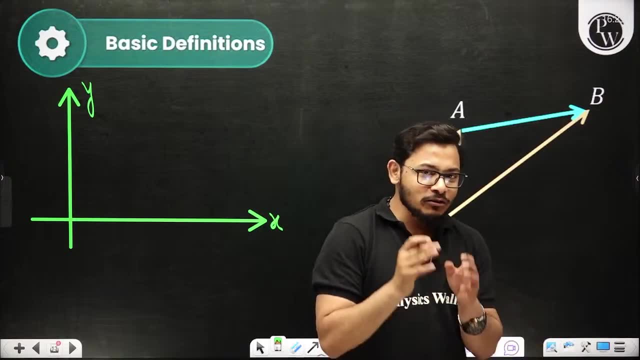 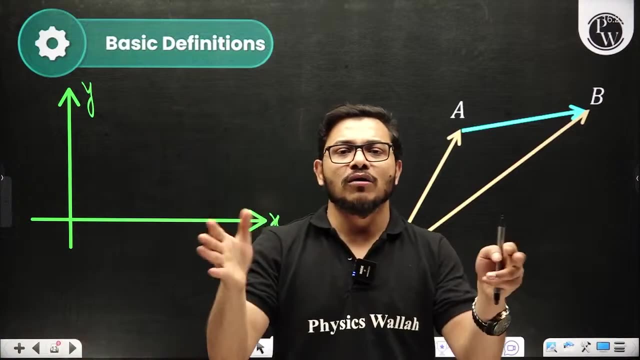 my house is in xy plane. someone told me that, brother, you do one thing. if my house is in xy plane, if my house is in xy plane, if I ask you this, tell me one thing. as you might have seen, some people study geography to study geography. when you see google map, 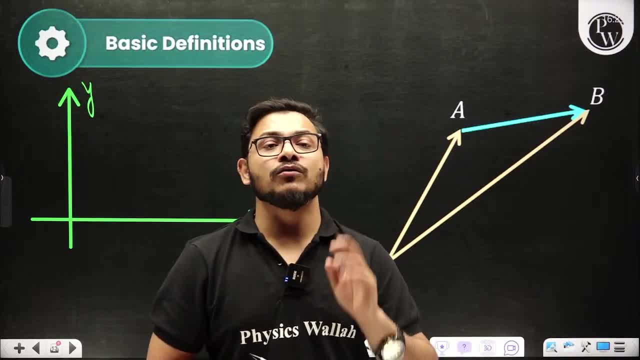 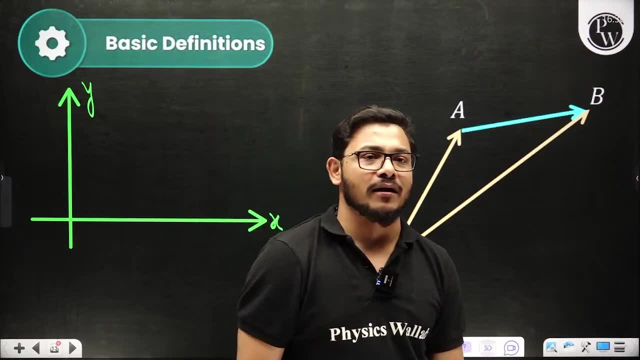 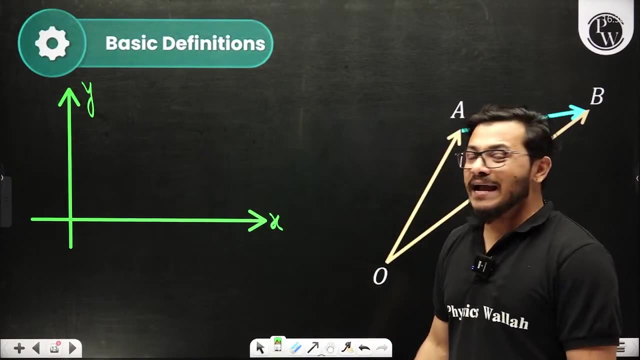 then you might have seen latitude and longitude in geography. do you know why it is studied? what is the need of all that? to identify a particular space? the same work I have here. listen to me carefully if this is my xy plane and if I ask you, where is my house? 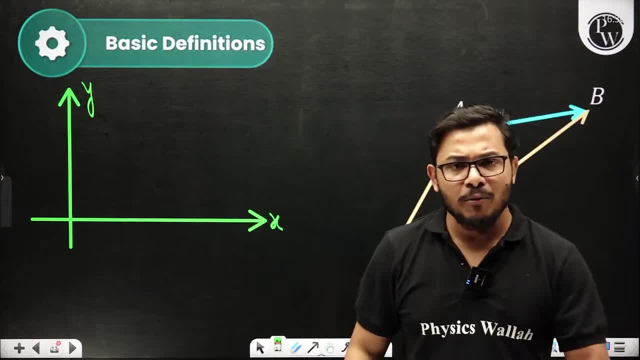 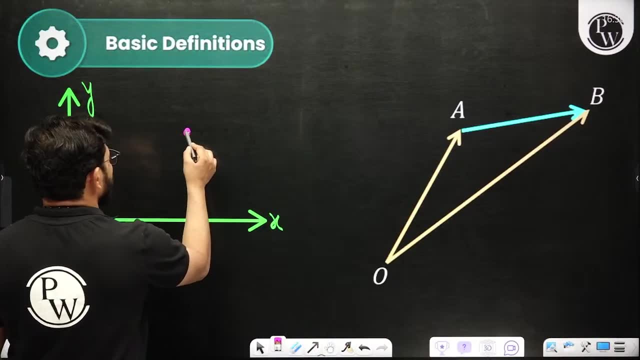 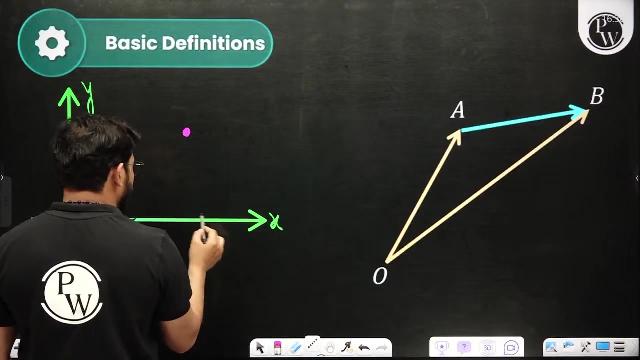 in which coordinate I lie. then you will tell me what is your position. to tell you the position, you need a coordinate. coordinate means you need x and y. so this is your position. how you are telling your position. this position tells you that you have to go in x. 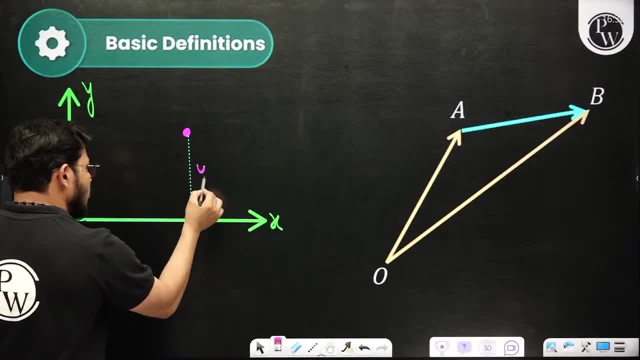 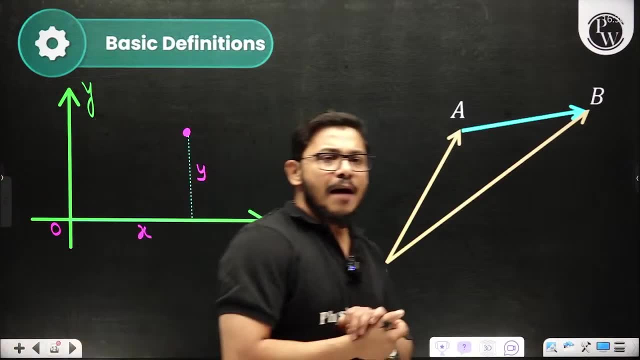 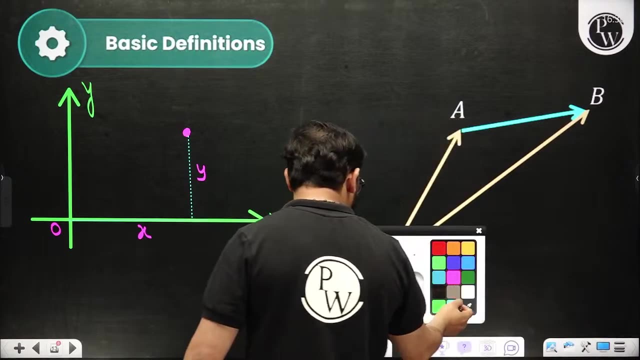 and y. what are you saying? this is your y coordinate, this is your x. so this is your position. now, to tell your position what you have to do, finally, where you have calculated your position, suppose a person was standing here. suppose a person is sitting here on a chair. 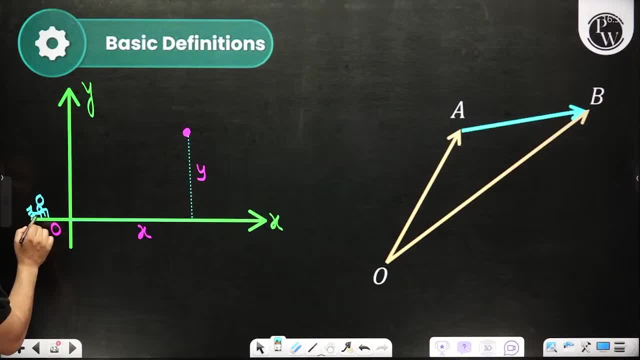 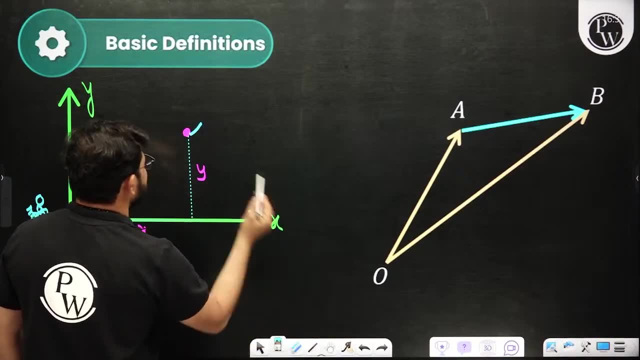 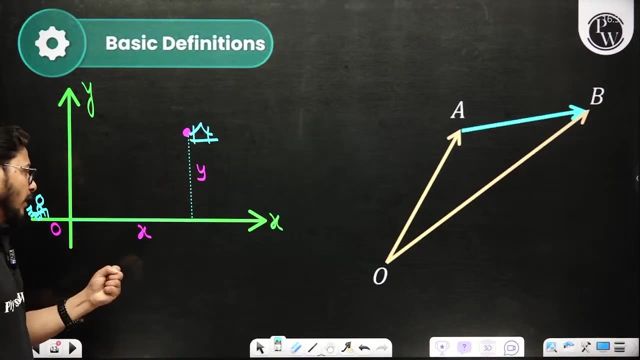 suppose sarukh bhai is sitting here. so he asked sarukh bhai, where is your house? so his home was here. so he is asking: where is my house, how far is my house from mine? if we ask sarukh bhai, how far is your house. 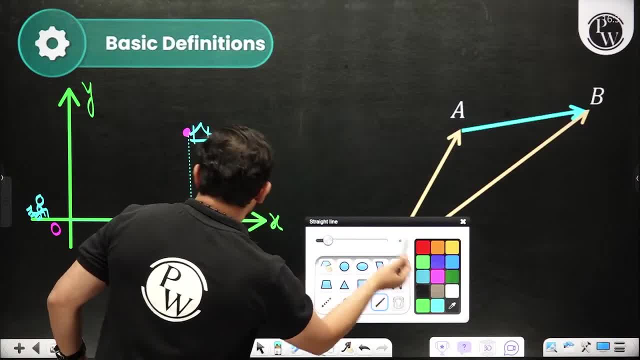 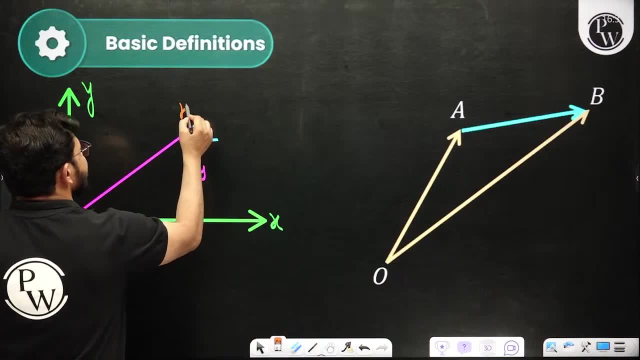 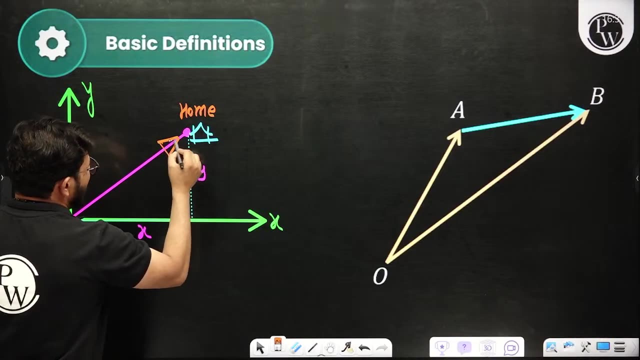 he will say x and y. so what will he do? he will tell you to connect your origin with this house and, after that, whose position you want to calculate, whose position is to be connected to this home and in which respect to which person. so remember this arrow. 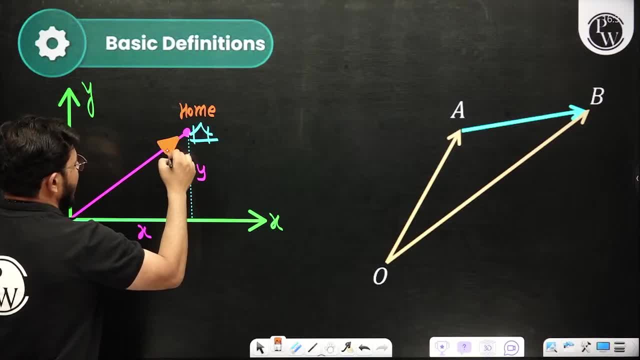 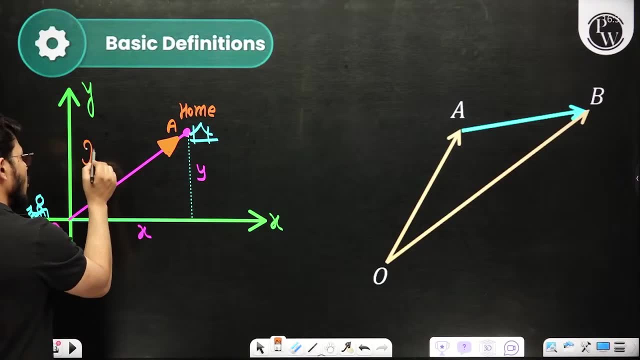 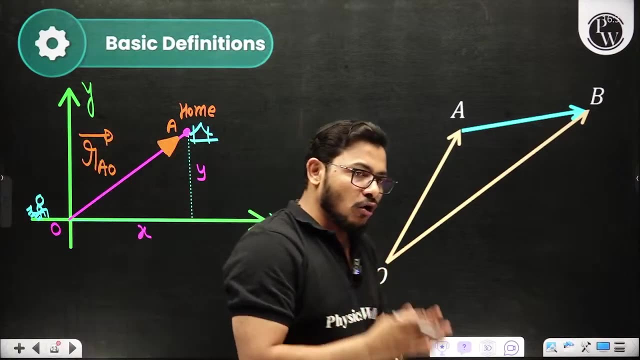 you have to install at house. please listen again whose shape you have put arrow at home. suppose you have written home at point a. so whose point is affection, whose point is Сегодня it? that is the position of point of a and with respect to point of o, 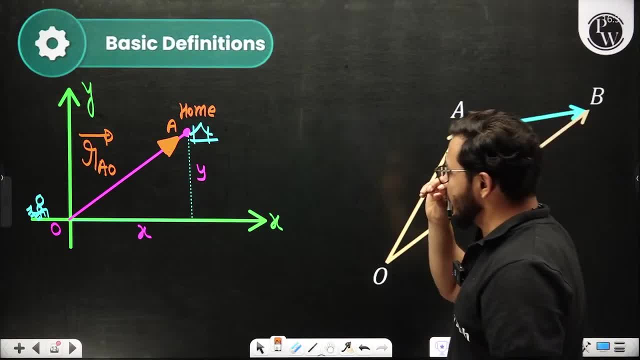 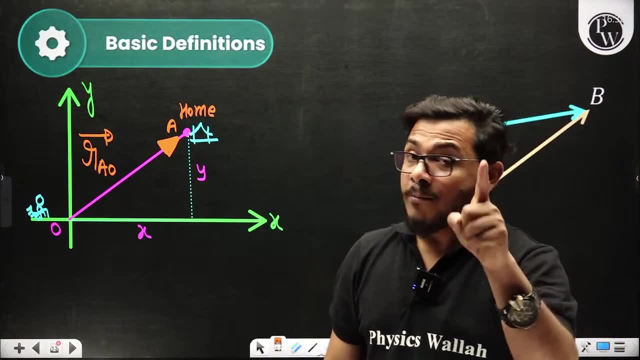 what a great saying you wrote. That one is called the position. See, always remember, in the whole fluid mechanics, in the complete fluid machinery. this is the work that is done. I am telling you again. people don't understand my dear. 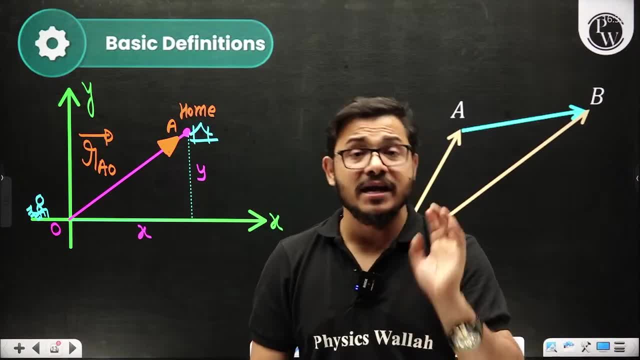 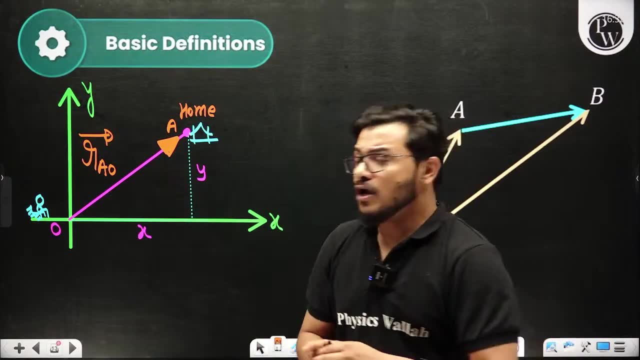 in the whole theory of machine. this concept is used In the whole theory of machine. this concept will work. Making the arrow, showing the arrow is very important to you. Whom did you put the arrow on? On point A? 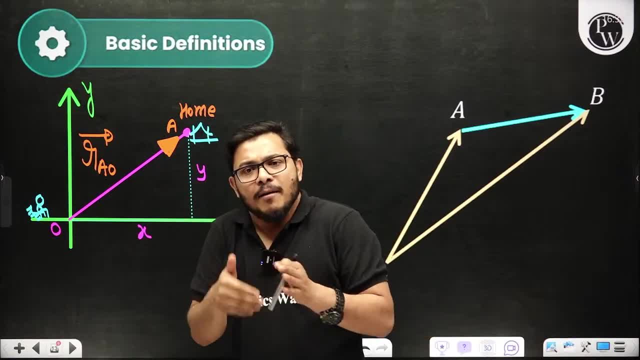 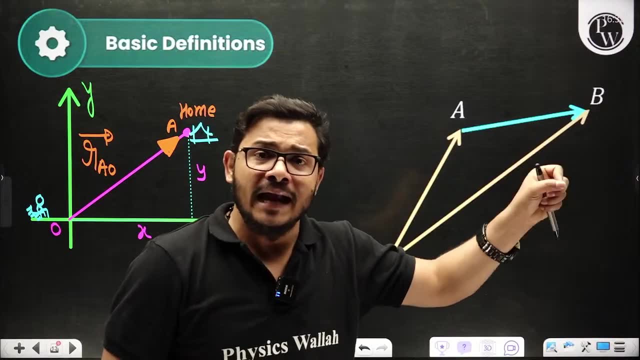 From where did the arrow pass? From point O, Which means which side is the arrow? Point O, Which means this position of point A is being shown in respect to point O, That one is called the position of point of A and with respect to point of O. 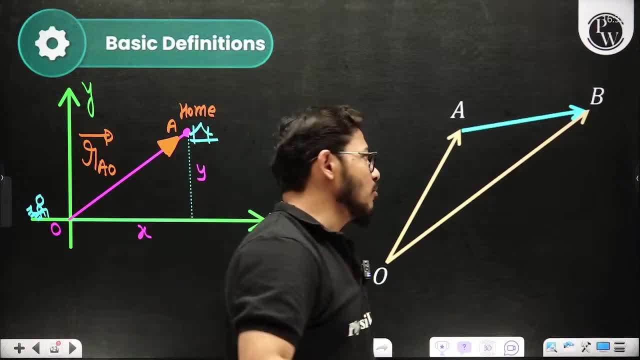 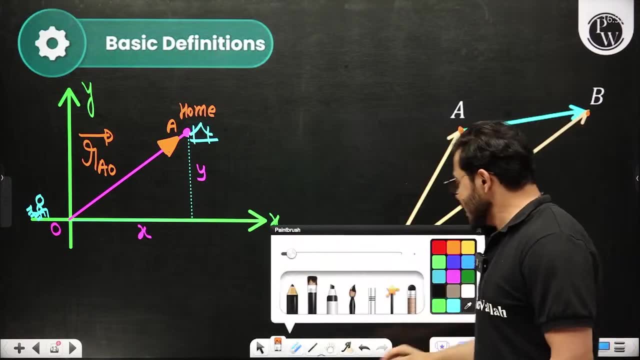 From where did you put the arrow? This is very important to understand. Like, let's assume I took the origin point here. This is point A for me. This is point B for me. What did I do? What did I do here? 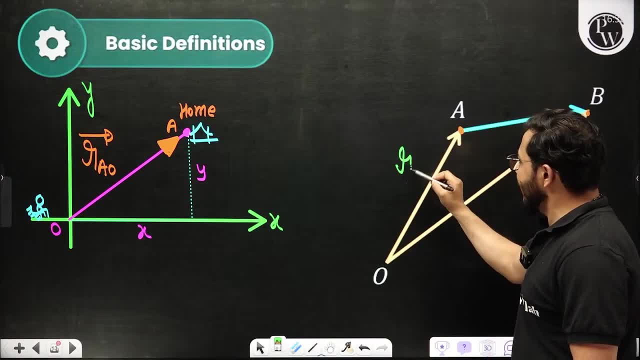 Please listen. I mixed this origin with A, So this is the position of A in respect to point O. Very good, And whose arrow did I put? Point B, Point B. So this is the position In respect to point B. 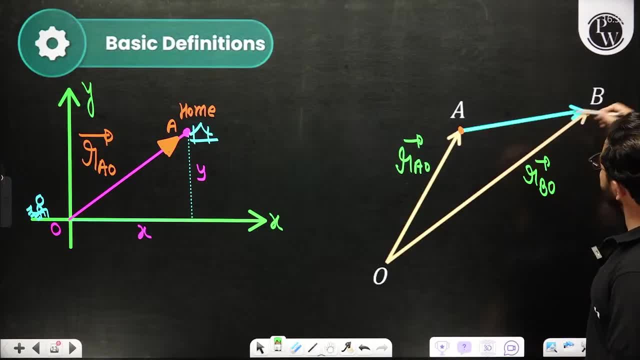 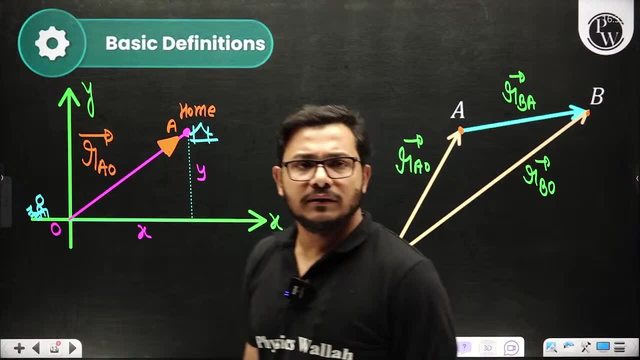 Very good. From where did your arrow pass From point A, And whose arrow did you put Point B? So this is the position In respect to point A. What a wonderful thing you have written. That one is called the position. 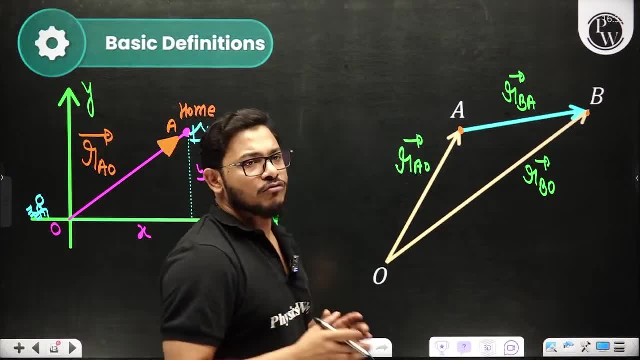 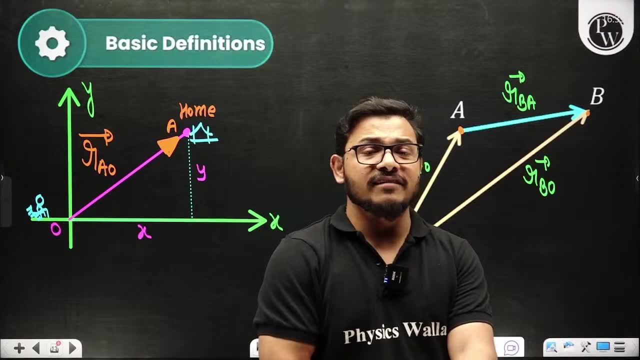 So how do you have to write the position? You have to understand this very well, And when I will teach you the theory of machine, then please listen to me, I will not revise all these things again. I will ask you all these things there. 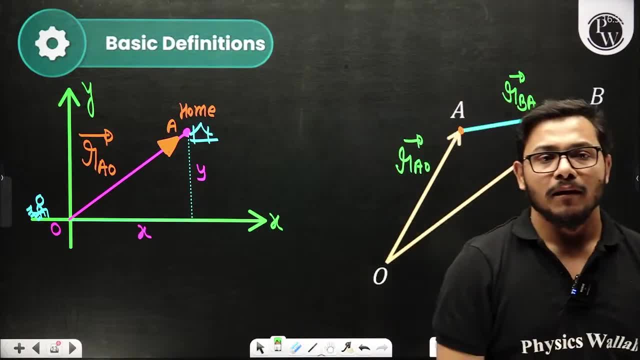 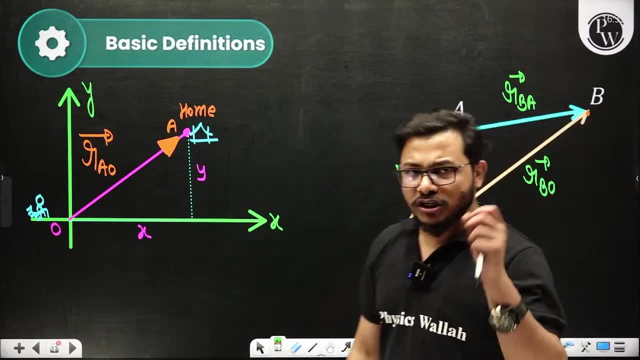 How did you write that position? That one is even concept That how we will write down the position. How did you write the position vector? It is very important for you to understand this: The position of point of A with respect to point of B. 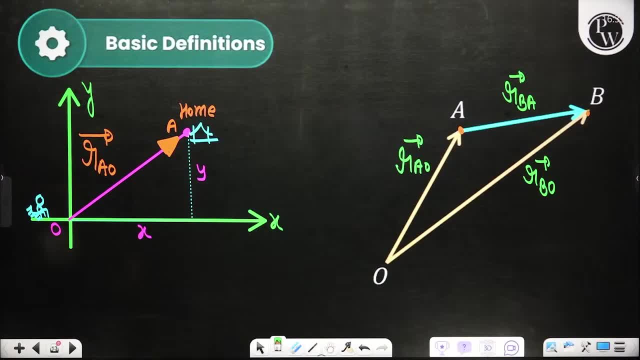 Did you understand the language. So I hope by doing 1 to 1, you must have understood all these things related to position, That how I have written and shown you this position. So I hope you got the concept of position. 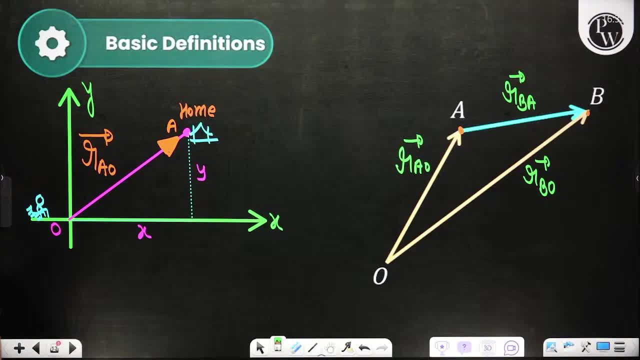 Now, as soon as you have talked about this position here, so now I am going to talk about the next point. The position is over with me. Now. who am I going to talk about? After the position, I had told you one thing. 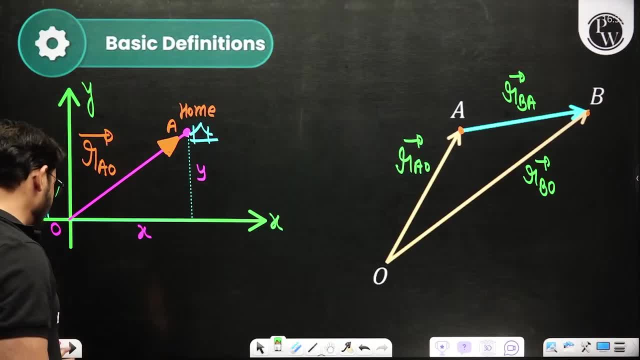 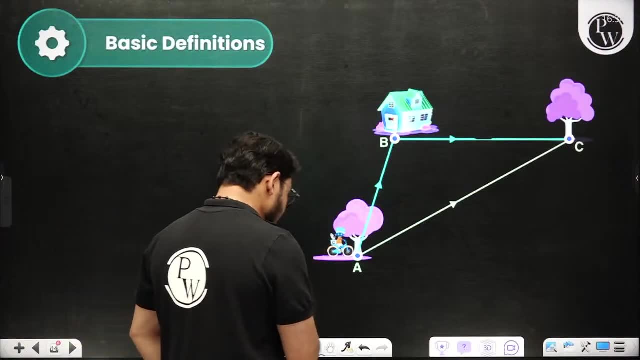 What is the distance and what is the displacement? I have taken the best example of distance and displacement. And what did I say to you? Please listen to me. Let's assume that this is a person, This is a man And he started walking from here. 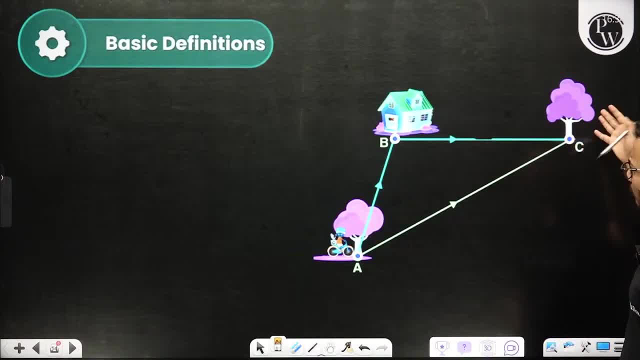 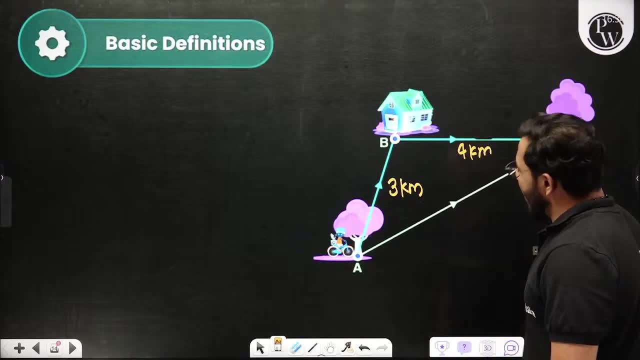 This is his house And here, whatever tree you have considered, let's assume that he walked 3 km in this direction And he walked 4 km in this direction. Okay, If someone tells you in the question that you tell me that, I want to ask a small example. 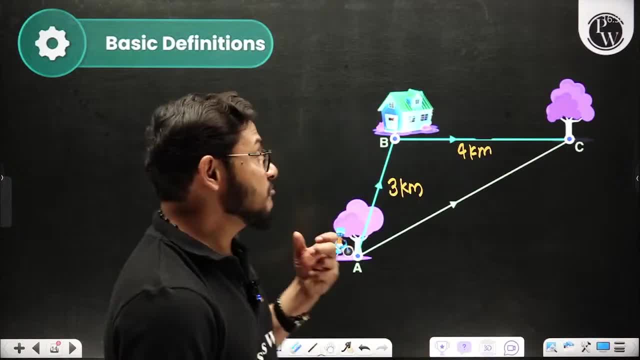 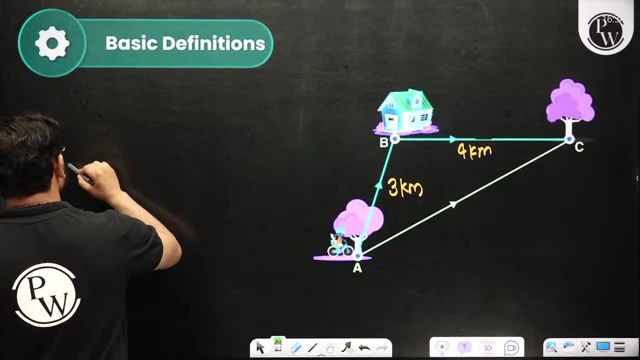 What is the distance And what is the displacement? What do you understand between distance and displacement? Please look at the word mirror. I will also explain this. Let's assume that you were here and after some time you were roaming around like this. 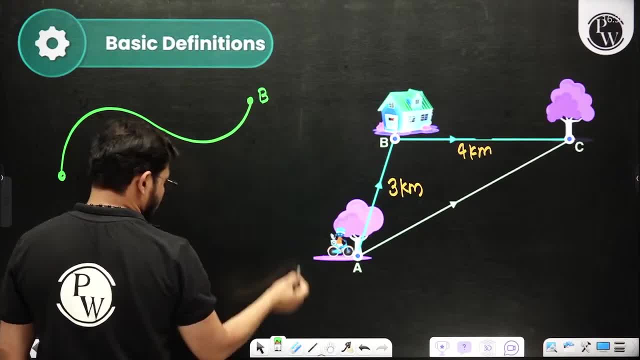 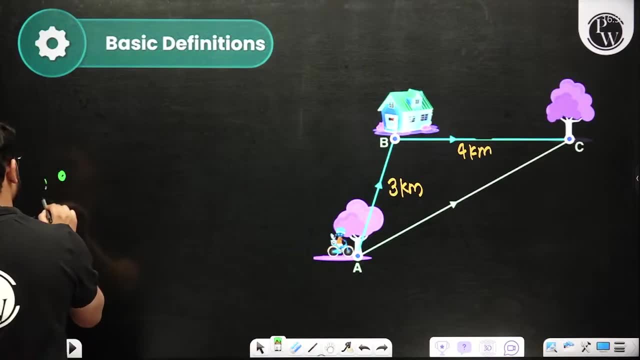 You were roaming around in the whole world and you reached here. Let's assume A to B. Okay, tell me one thing. Let me make it again. Wait a minute. You have to go from point A to B. Let's assume you have two points. 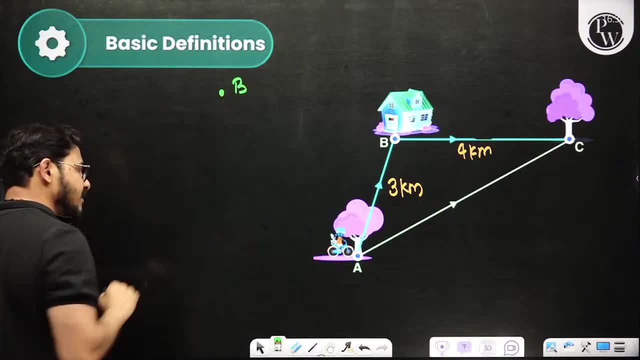 This is A and I have B. Tell me how many ways there will be to go from point A to B? Will there be only one way? No, There can be many ways to go from point A to B. Some kid is roaming around in the whole world like this: 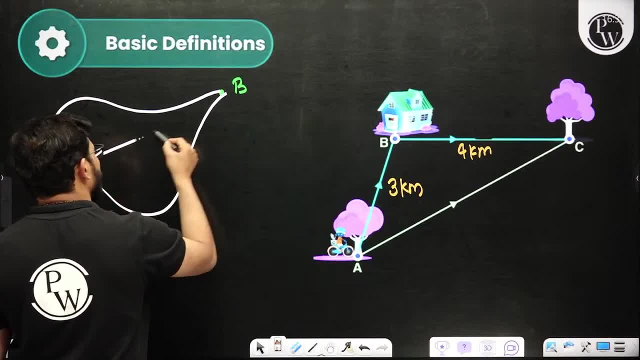 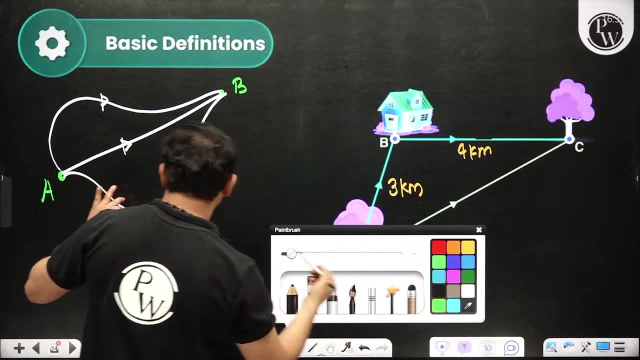 Some kid is roaming around in the whole world like this. Some kid is roaming around in the whole world like this. So what are you seeing? The length of the actual path alone is different, So it means that the distance between two points can be a lot. 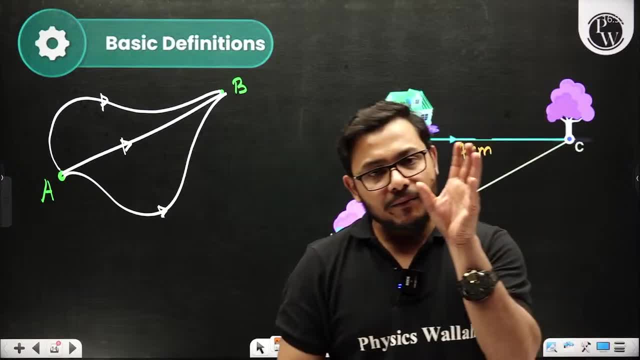 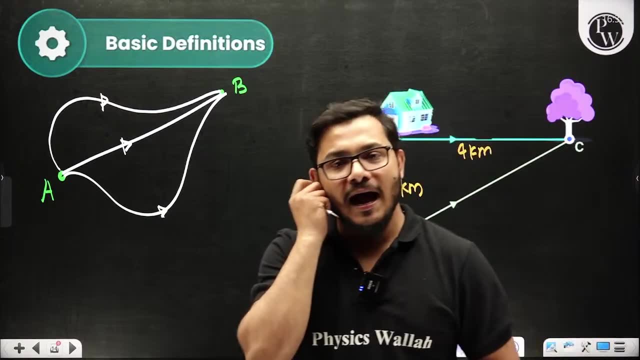 There is no fixed value of distance. It is an infinite value, But, but, but, but. but. The displacement between two points is unique. Do you understand what unique means? There is no fixed value. So let's say, if you want to marry, 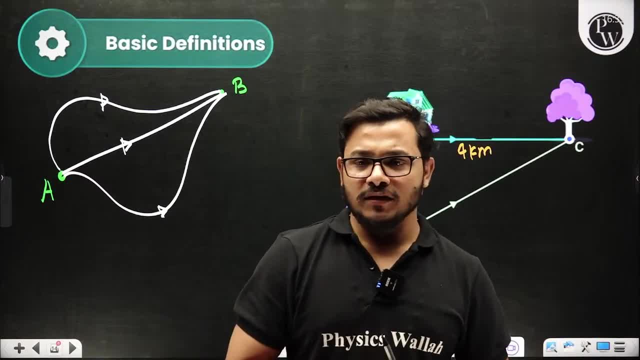 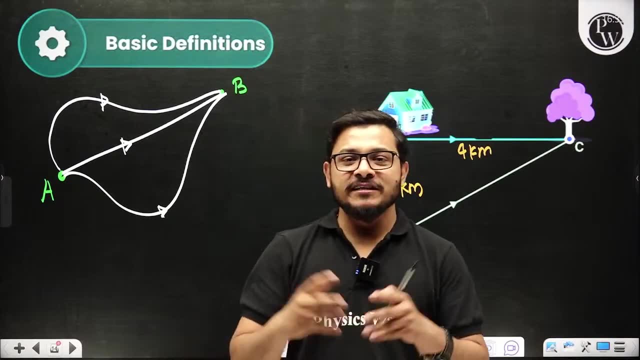 and your parents tell you that you want to marry. So when you go to marry, your parents ask you: what is your requirement? Which girl will you like to marry? So what is the demand of the child? A new child is about to get a new toy. 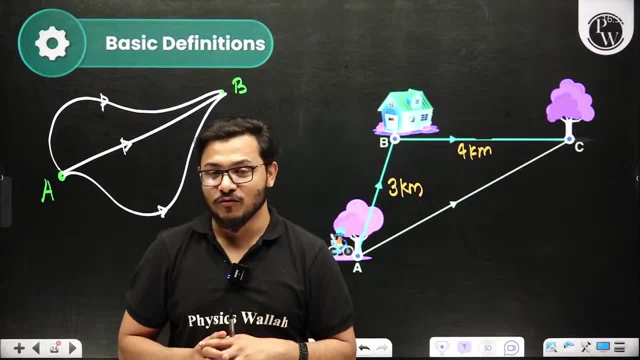 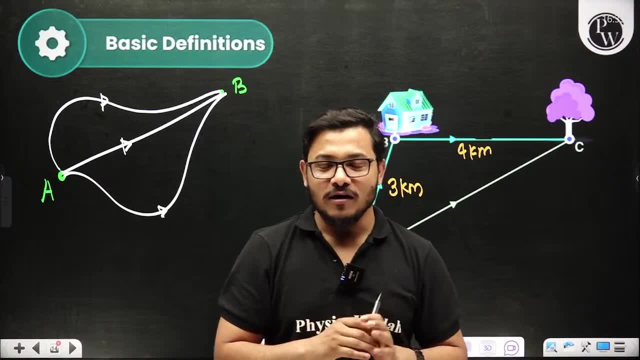 So what will be the demand That I will like to marry a girl whose hair is very beautiful and looks very good, The height is very good, The color of her hair should be very fair, she should have long eyes and she should be a very good girl. 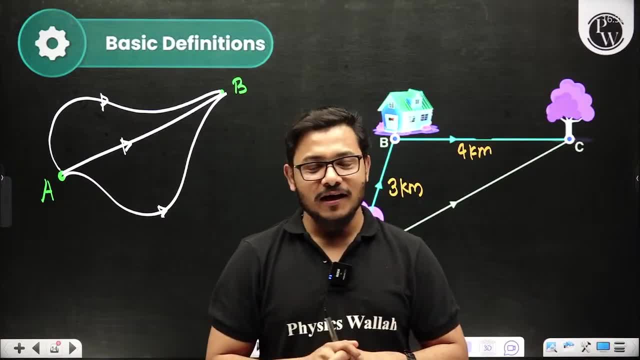 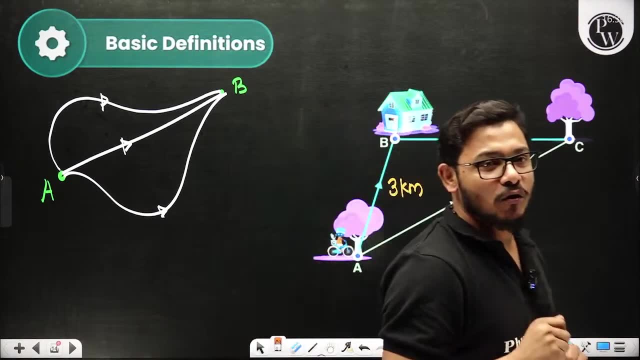 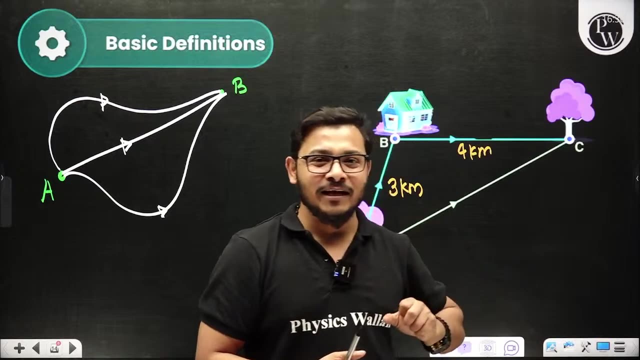 I will like to marry a girl like her. So you told me the whole quality, that I want this quality. So people said that this quality is unique. this quality is unique for you. What does unique mean? You told me the quality of such an antique piece that you will not get such a piece in the world. 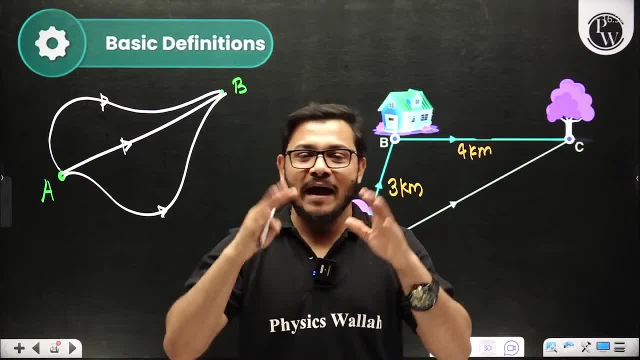 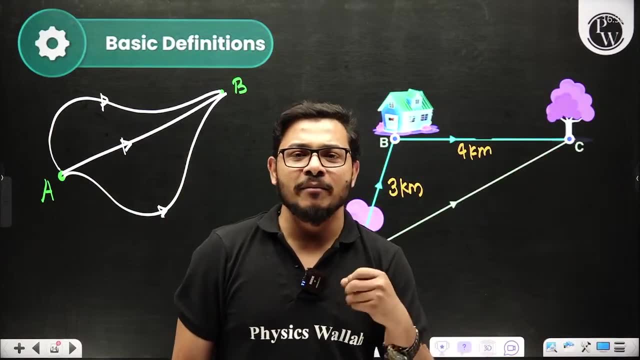 This is unique. You told me everything that you want. you want good hair, you want good eyes, you want a tall girl, you want beauty. you want everything in it. So God has made very few pieces like this in the world. 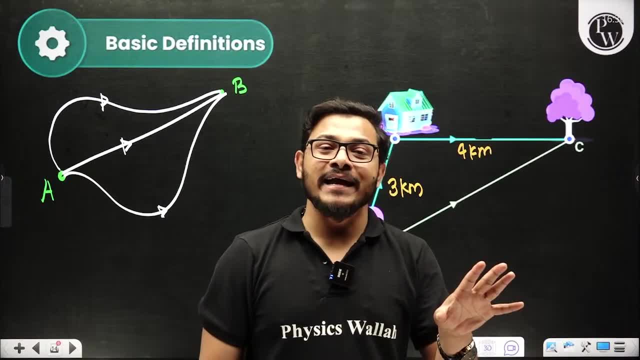 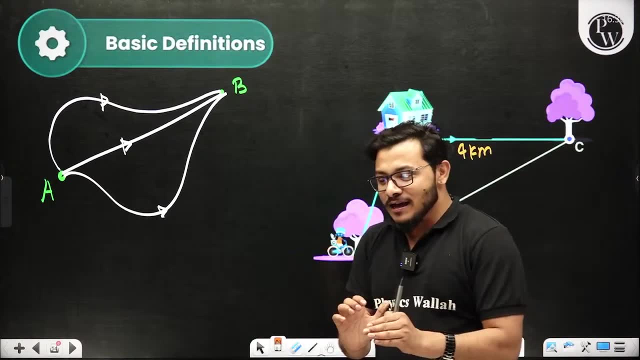 It has become unique. It is unique. So it is unique that there is no one like it. Is the language coming? It is unique. I am not sharing my feelings, So it has become unique. Unique means that there is no one like it. 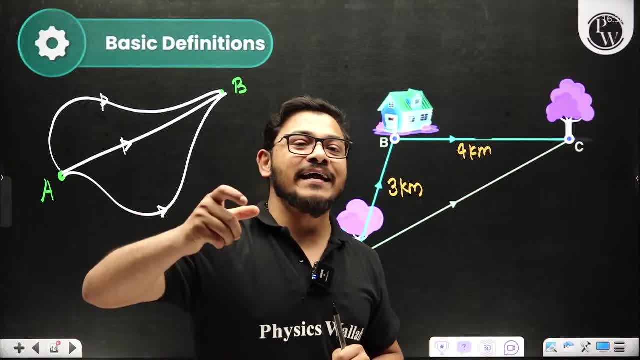 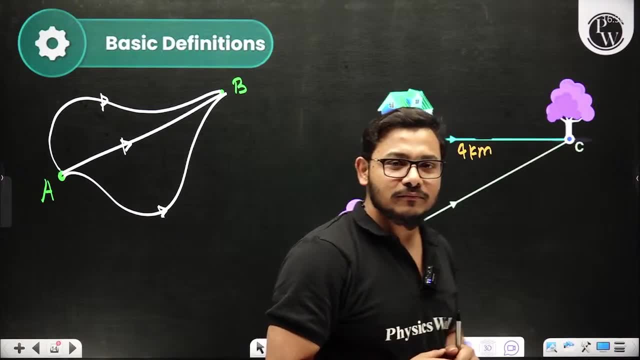 That one is unique. It has become unique. So unique means that there is no one like it. It has become unique. But now there is a story. Let me tell you one thing. You told me your demand. You are not even worthy of it. 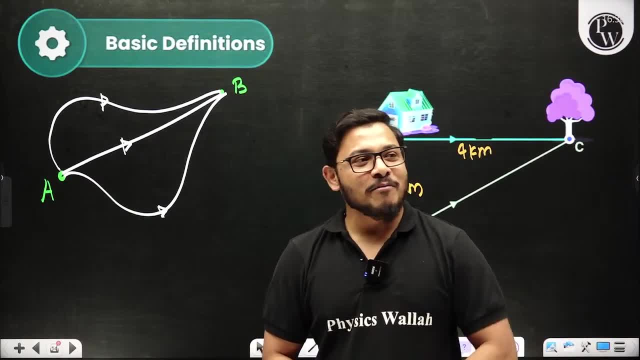 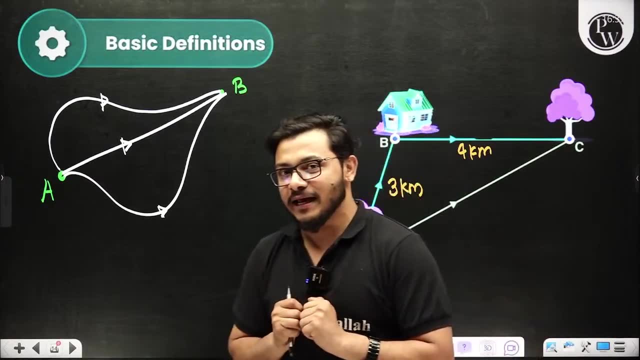 First of all you check the quality inside you. God has made such pieces very antique. It is not necessary that the antique piece is made for you. So I am going to say the same. This is distance and displacement. Distance can be a lot. 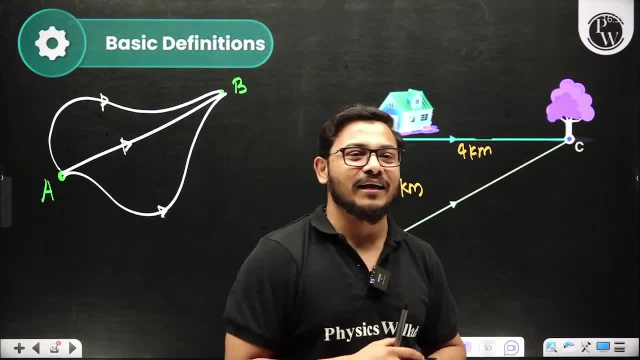 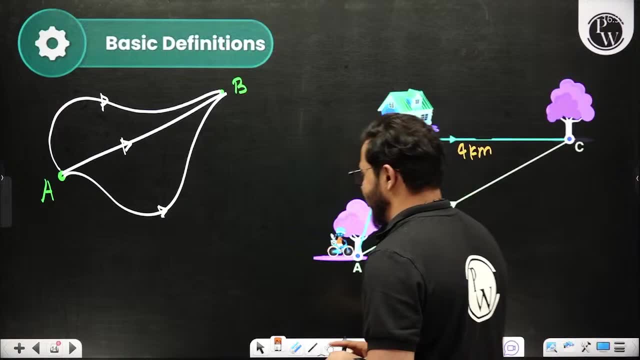 It will work wherever the marriage is done. But when it comes to displacement, then displacement is unique. There is no one like it. It is only one. There is only one in the world. It is an antique piece, So that one is called displacement. 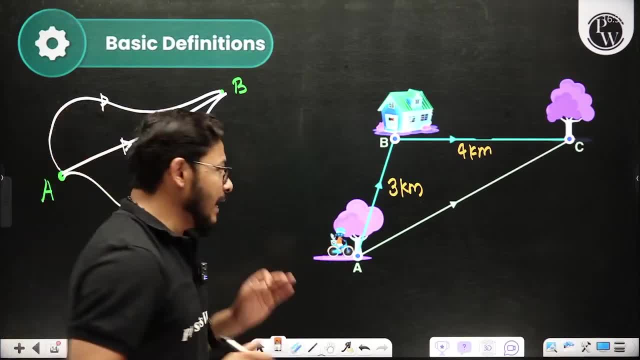 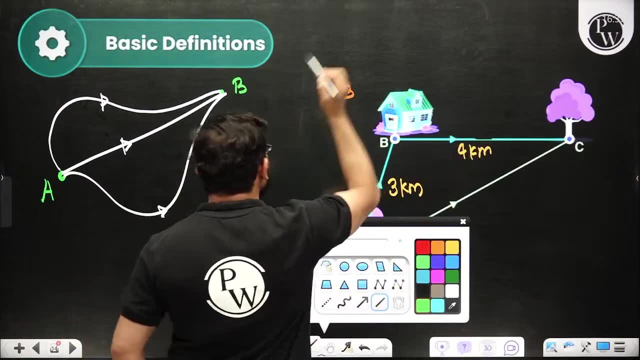 Displacement is unique. There is no one like it, Because it can be only one. That means between two points. If between two points, If someone talks about displacement with you, Then you say that it is unique. Unique is what is minimum. 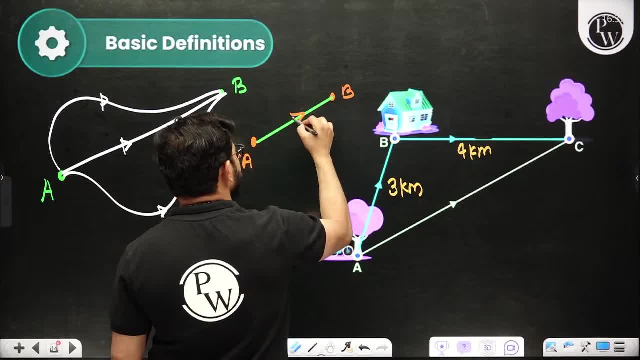 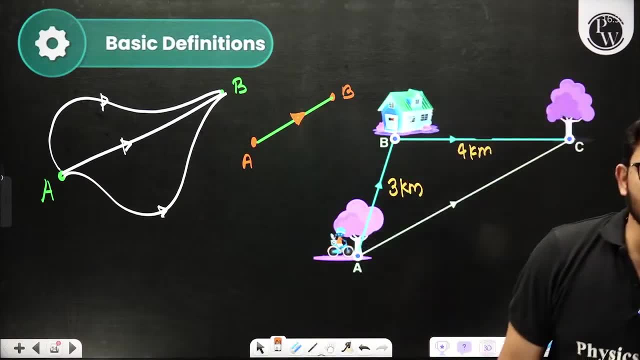 The matter is over. Just combine these two points with a straight line: That one is called displacement, That one is called displacement. Have you understood the amazing thing? So this is my example: What is distance and what is displacement? So you had to tell. 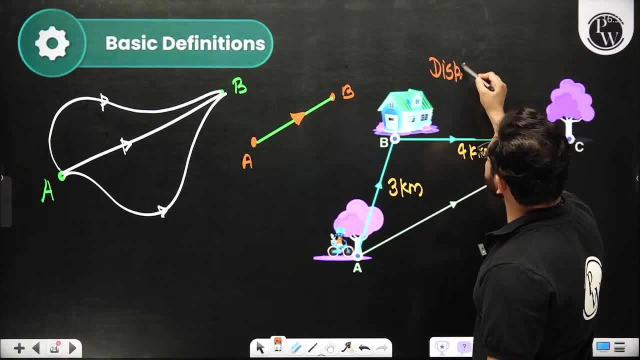 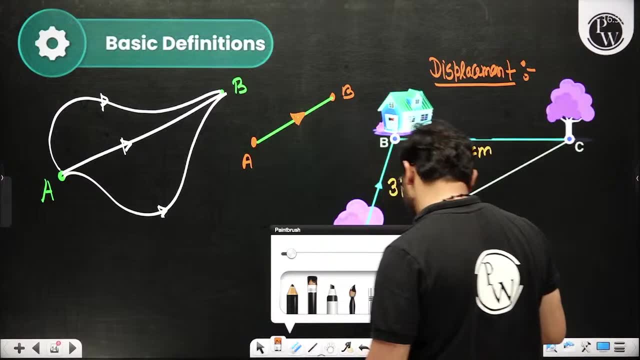 Brother, the displacement is unique. What is displacement? Displacement is unique. This is given to the guys with good luck. Understand what I am saying. Those who are very lucky will get it. This is unique. This is unique, Okay. 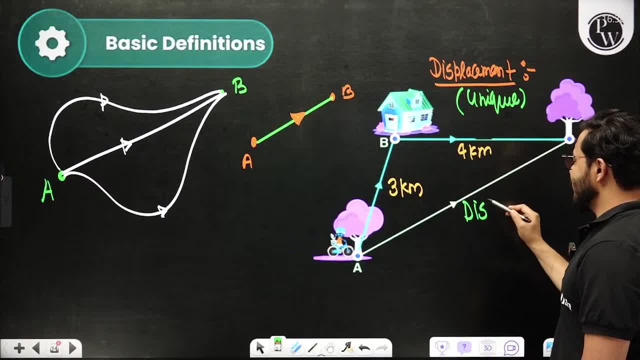 And everyone gets distance. Distance is everywhere. You will get it somewhere, Because it is infinite. Marriage is for everyone, Whether it is from anywhere, Isn't it? It is infinite, It is infinite, It is infinite. Okay, brother, So that one is infinite. 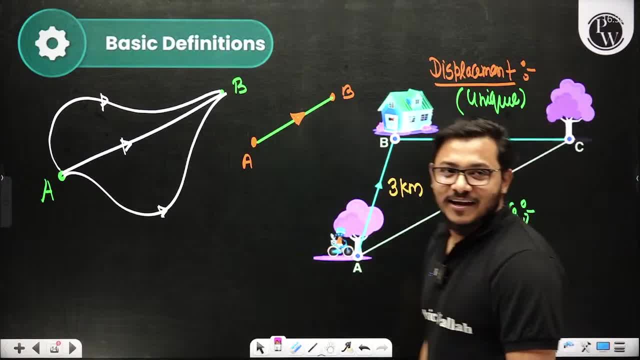 That one is infinite. So I hope you got it: The concept of distance and displacement. So I hope you got it: The concept of distance and displacement. So I hope you got it. So I hope you got it. So we have understood the concept of distance and displacement. 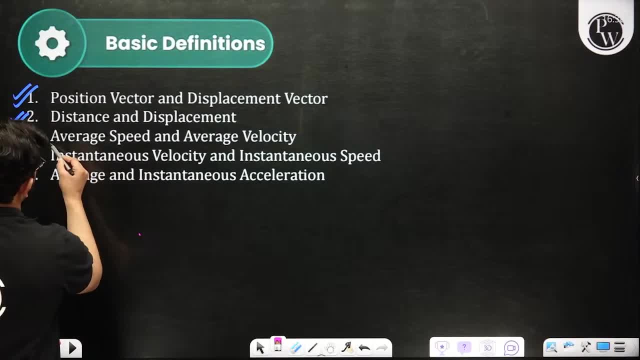 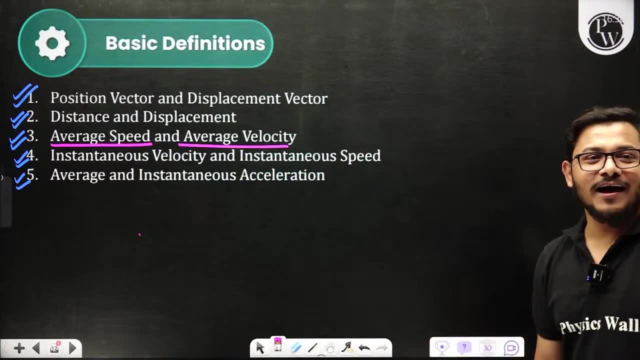 Then after that, we people have written a funda here: Average speed and average velocity. Average speed and average velocity. What is it called? Ha ha ha. No, this is one thing. Let me tell you one thing: Displacement is equal to Gulabo. 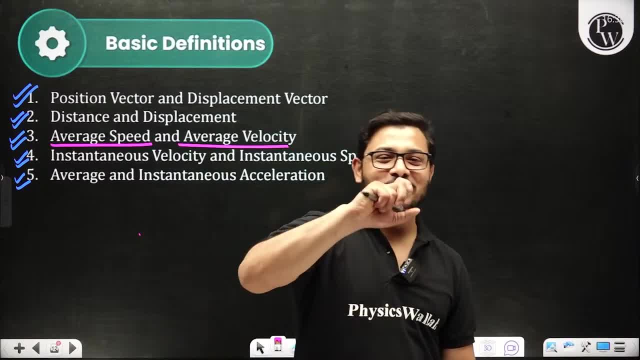 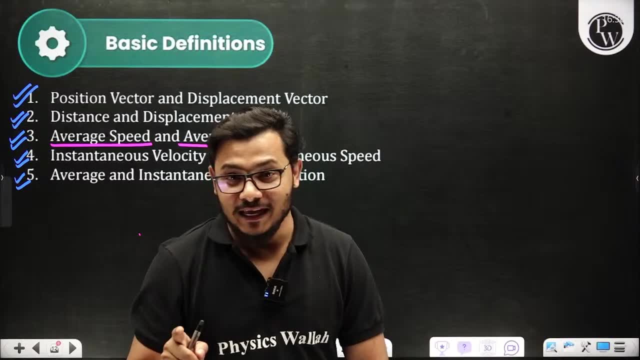 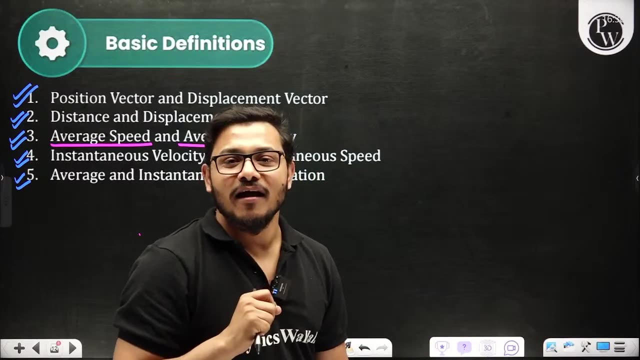 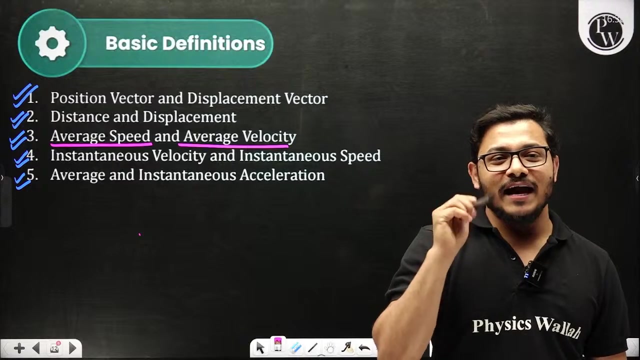 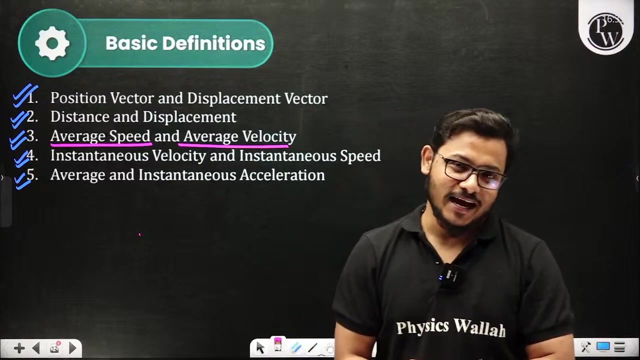 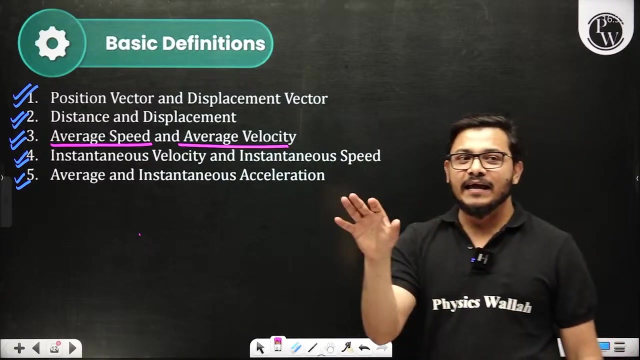 Yes, it is true. Let me tell you one thing. Listen to me, This is the truth, And the task for you is very important. If the boy's government doesn't work, Then the government will not work. If the girl is married, the chance of getting a unique piece is less. it is said that it is very important for the boy to have a government job. then only he will get a unique piece. so now you think that you have to take a distance by doing a government job or you have to take a displacement. if you do a government job, then you will get a displacement. if you go to a private job, then you will get a distance. decide what to do on you. it is being said so. that's why I am saying: study, study, break the examination once, prepare once. when the level is ready, then you can do it, then you can do it, then you can do it. 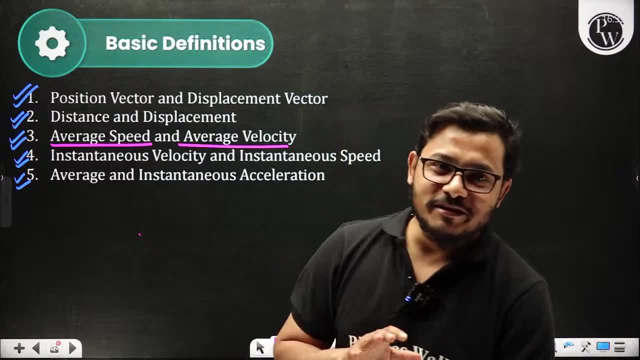 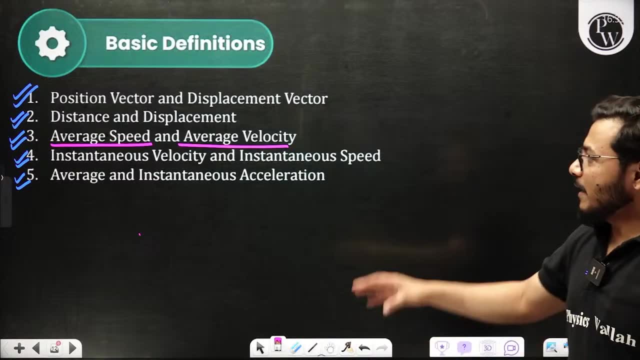 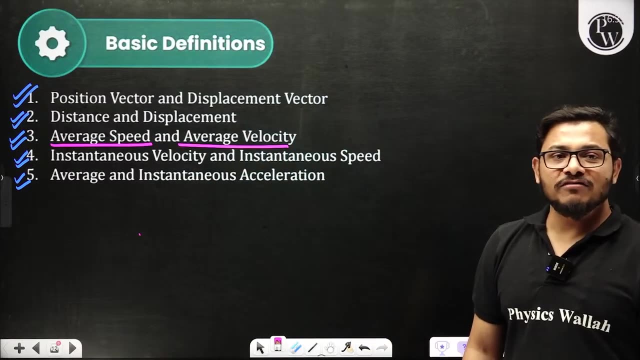 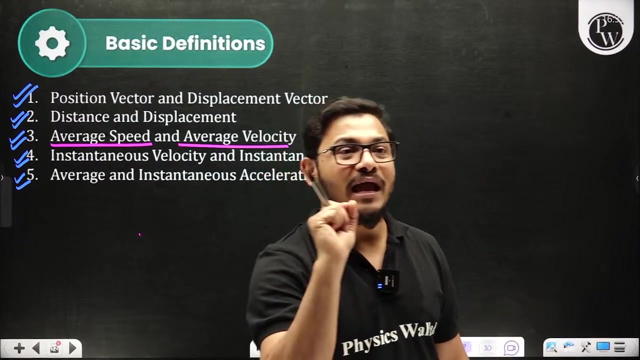 So I can say with guarantee that you will get everything. there is no need to worry about anything. okay, yes, so sir, what is the displacement position? the displacement position is this, son, that where is the displacement written? that position has to be told. that how that position is told. okay, now listen to me please. what am I going to say in one minute? now? I am talking about an average speed and average velocity. what is the average speed and what is the average velocity? let's understand a little about this now. I will come back a little. average speed and average velocity. 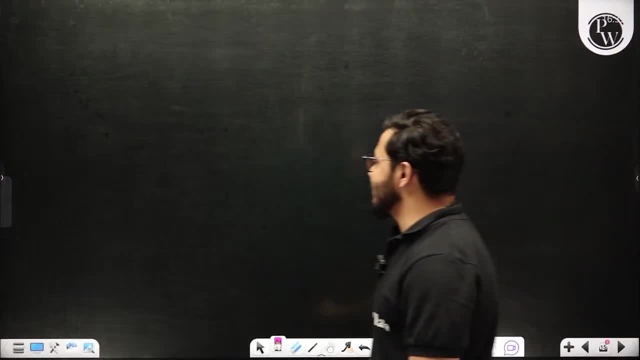 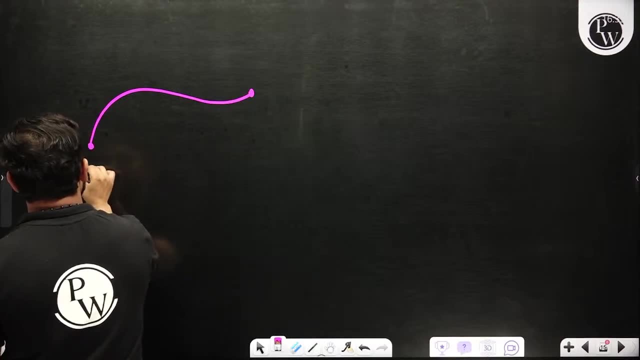 let's talk about the velocity. please see just one minute what I am saying. if you follow a path, you reach from here to here. if you reach from point a to point b, then the actual path alone, the length that you have traveled, the length that you have traveled along the actual path, you calculate it. it will take you some time to reach from here to here. 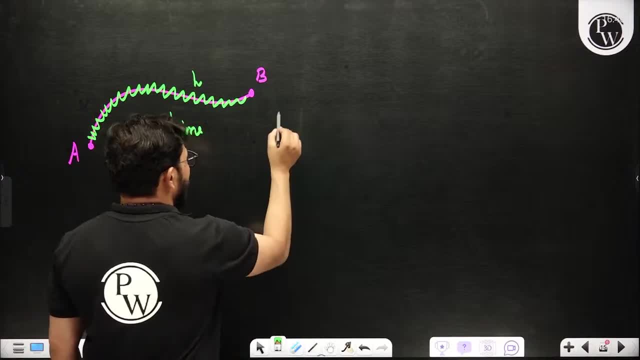 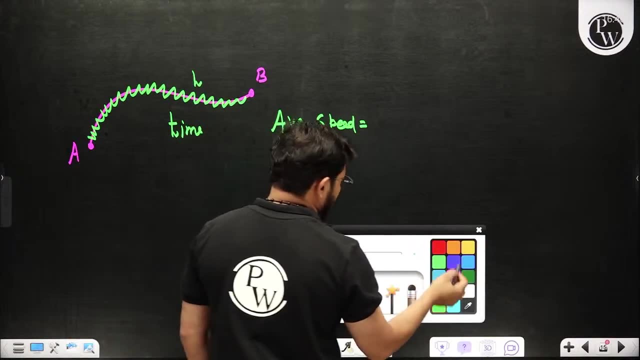 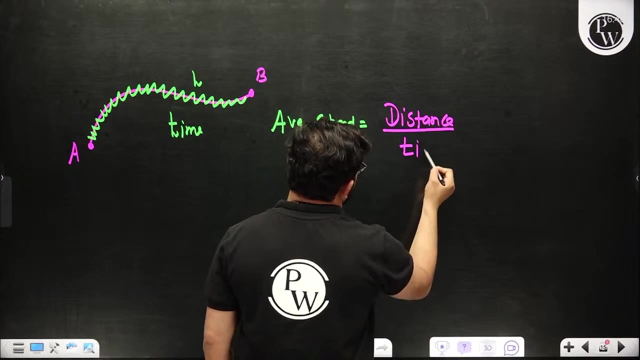 Let's assume for some time. then name the constant after talk about the average speed. jati hai toh, wo barabar hoti hai distance upon me time ke. wo kya hoti hai distance upon me time ke that one is average speed. agar koi tumse pooch le ke average velocity kya. 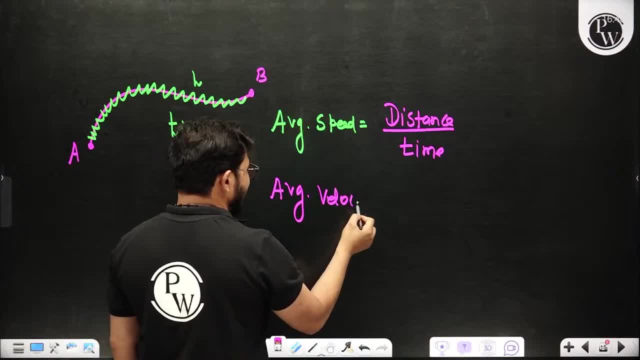 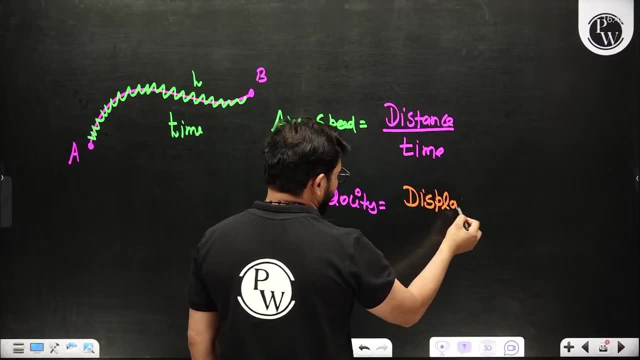 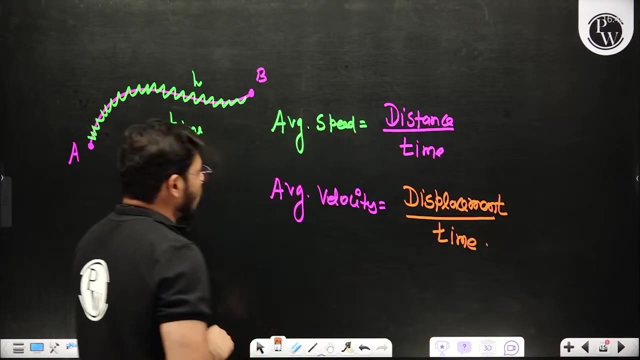 hoti hai average velocity, toh velocity kaise calculate karenge, jo aapne distance likha hai, bas uski jaga tumhe displacement kar dena hai, toh displacement, and upon me time, displacement men time is called average speed. toh average velocity aur average speed dono. 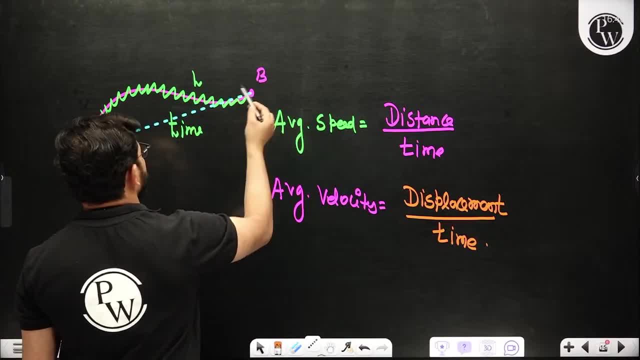 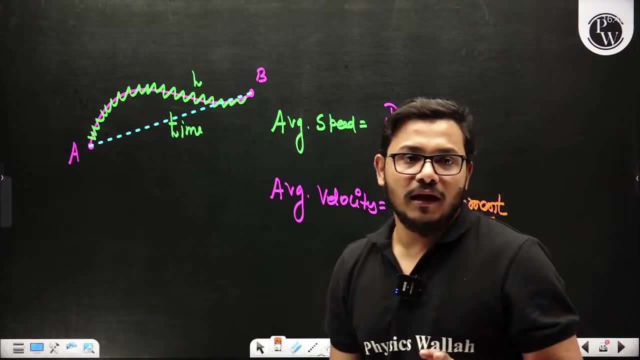 ek dusrey ke respect mein in dono ko men ek line se milaya hai toh misplacement, hai toh average speed aur average velocity dono alag alag hoti hai, dono says alag alag hoti hai. college, sir, ek minute abhi batata hai, sul nijega beta please average speed aur average. 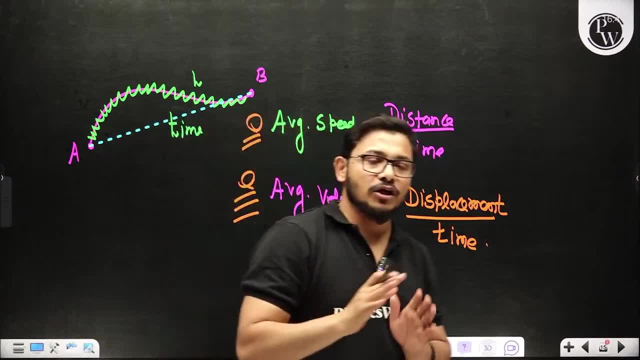 velocity dono kya hoti hai different hoti hai. both are different dono kaise hai different hai dono same hi hoti hai. signifika same咁 misra hai same nullah biri kti aap askaji Lolle aur aappa bast abhi ek aap proper fajni hai. sameurers, here, aap, ex IU of you may say the 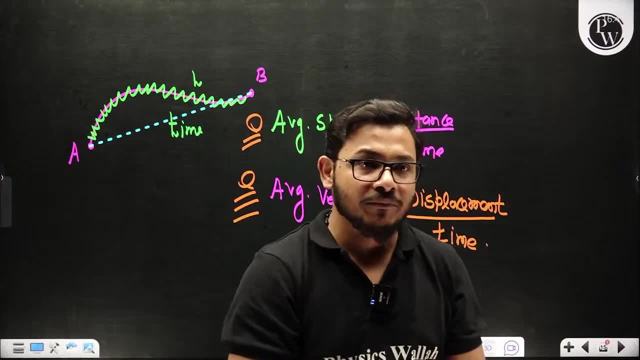 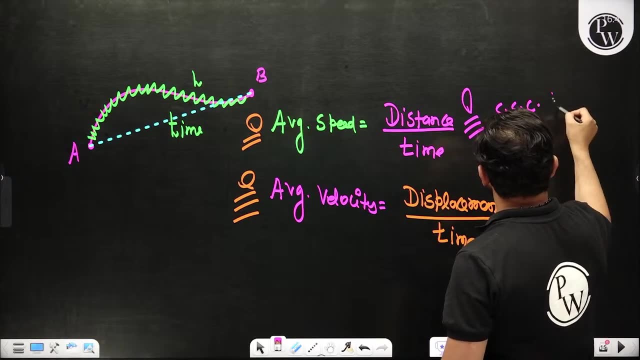 Please remember the total distance upon my total time. and let me tell you one thing: the formula I have written here, this formula, is a star formula. From this formula, many questions have already been asked in SSC, JEE. Average speed becomes equal to the total distance upon my total time. 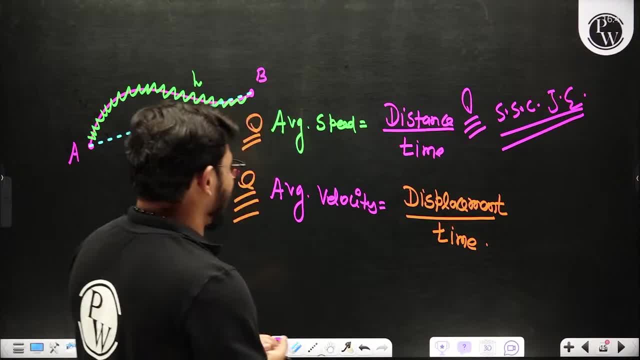 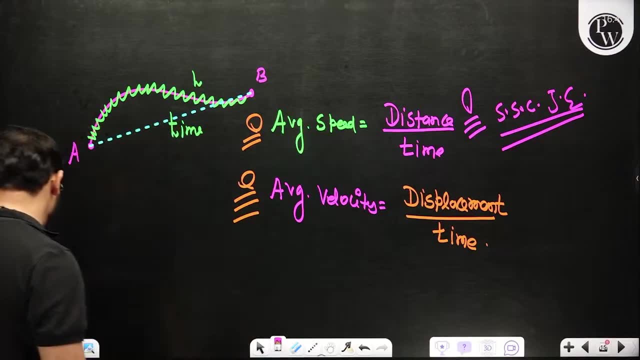 I will also show you the question. Have some patience. I will also explain the question to you. In what way Sir has talked about the average speed, The total distance upon my total time and average velocity. I hope you got it, the concept. 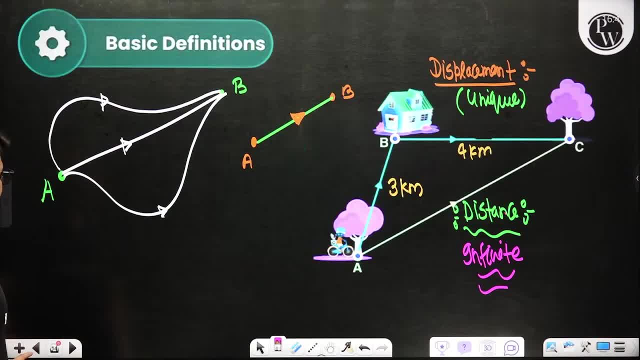 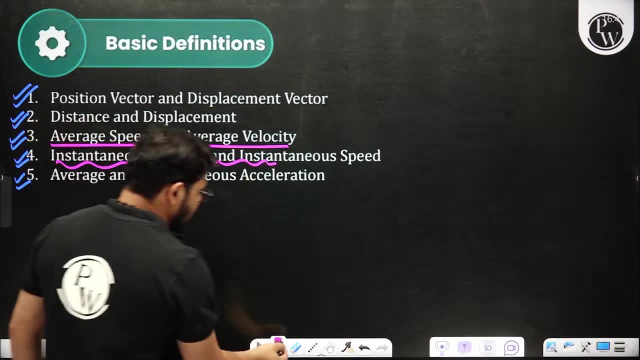 I have told you these two things one to one. After that, I come to the next point, And that is the next point: Instantaneous velocity and instantaneous speed. Listen to me, Look, the names of these two are different, But actually they both are same. 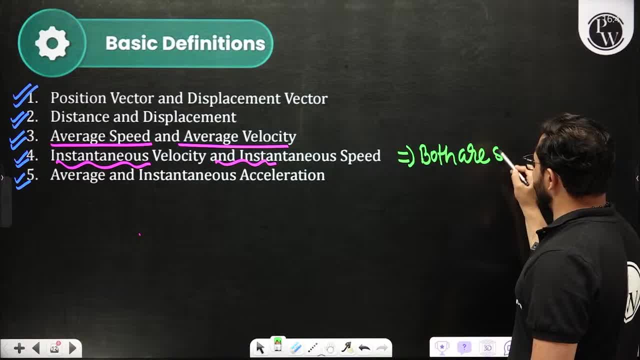 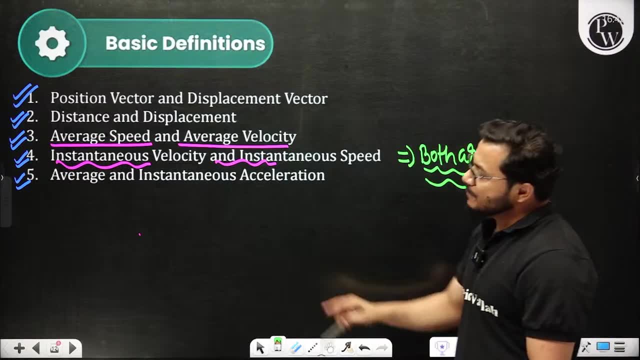 These two are same. Both are same. These two are same: Instantaneous velocity and instantaneous speed. How are these two? They are same, Whereas average speed and average velocity are different. These two are different. Both are different. These two are different. 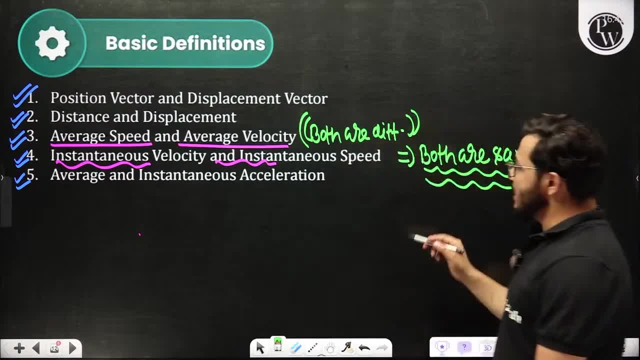 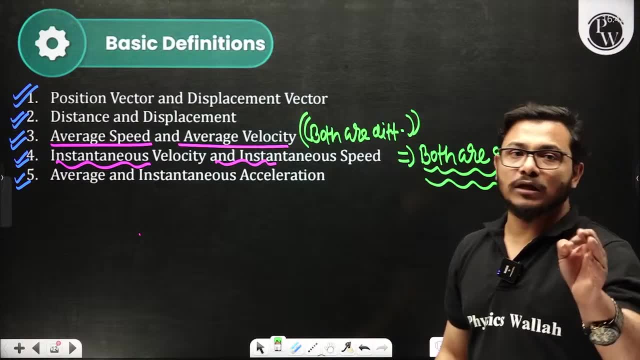 Please remember, These two are different, Whereas average velocity and average speed are different, Whereas instantaneous velocity and instantaneous speed are both same. These two are same. How are these two? If you ask me why I am saying this, Please look at this for a minute. 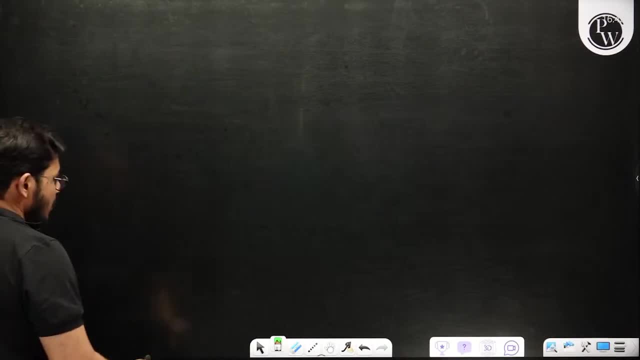 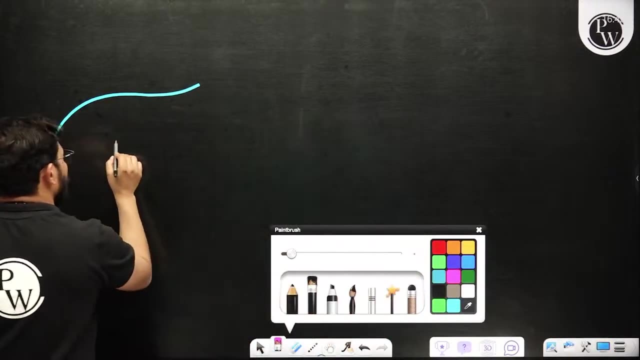 I will tell you the reason why I am saying this. Please listen to me for a minute. Suppose there was a particle. It may be moving along any path. Suppose I am saying a particular reason. I am talking about an instant. You are going to talk about a particular instant. 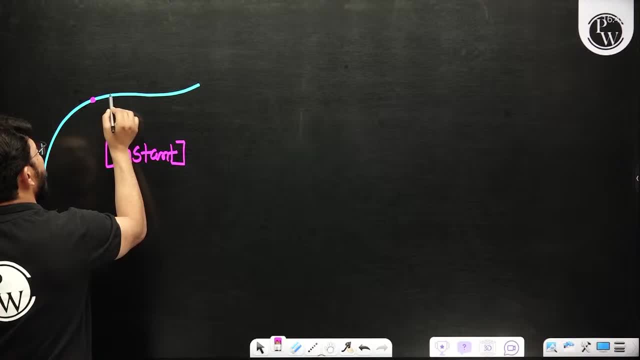 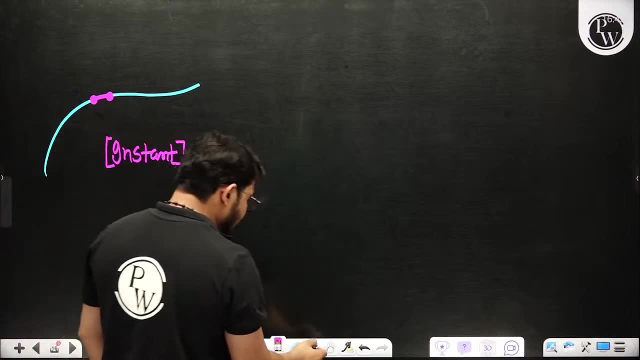 So for a particular instant, If you assume The length that you have run, A small length must have run, You must have run a small length It must have run. So this small length of yours, A small length that you have run, 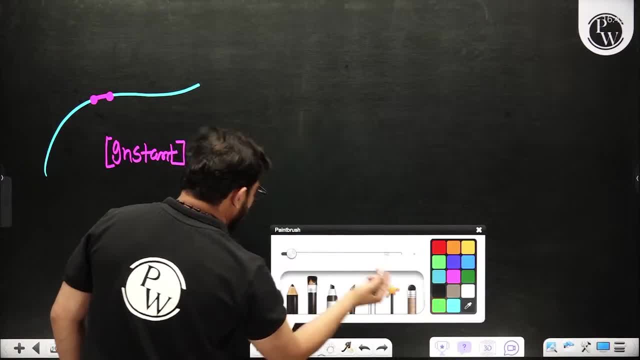 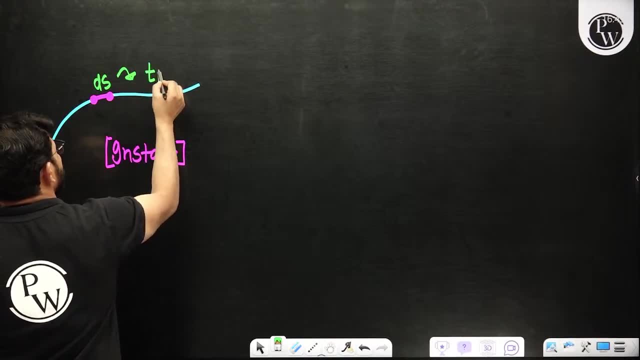 Suppose this small length is ds for you. What is this small length? for you, It is ds. Now, the time you took to run this small length, The time you took here. Suppose how much time did you take You took dt. How much time did you take? 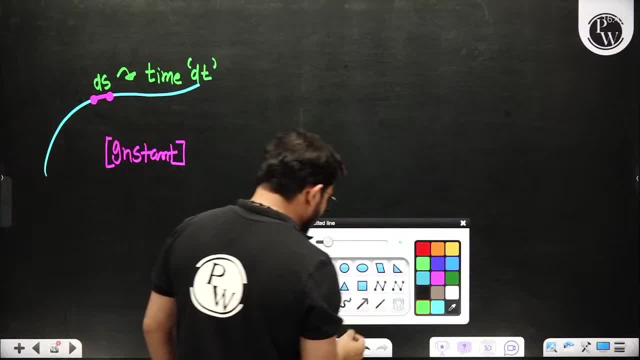 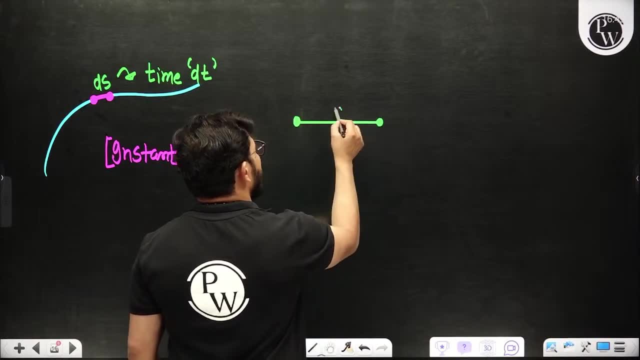 You took dt, So this small line became a straight line. How did this small line become a straight line? It did not become a straight line. Tell me one thing: If the path of any particle, If it is a straight line, Then the distance and 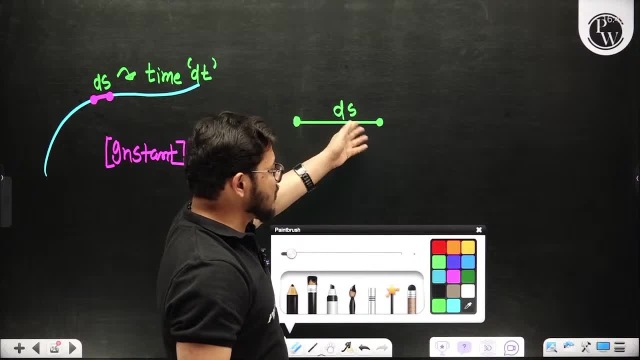 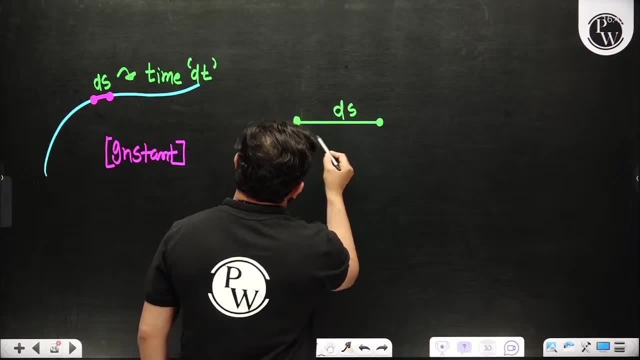 For a particular instant. The distance and the displacement are not equal, Absolutely. What is the length that has run from here to here? What is this? What is the length from here to here? What is the distance? It is a line. 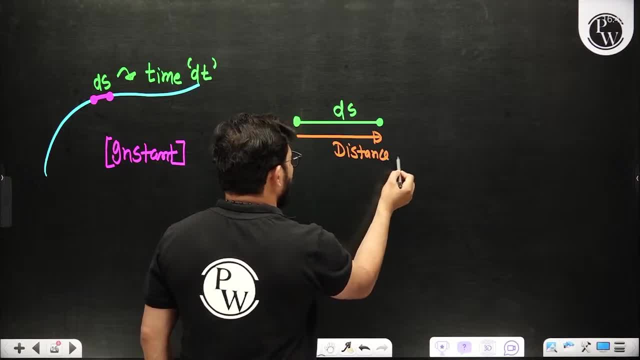 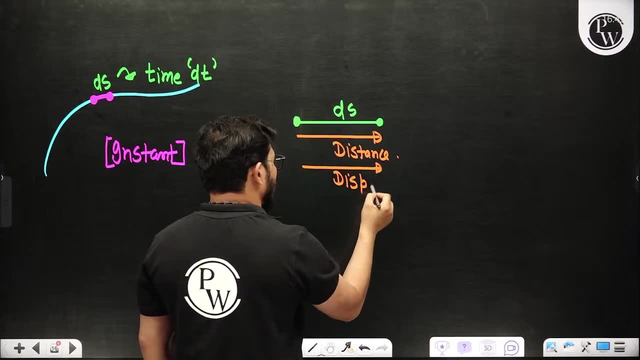 It is a straight line, This is the distance, And if you combine these two points with a straight line, Then this line is also your displacement. So here the distance and displacement are not equal. Yes, both are equal When these two 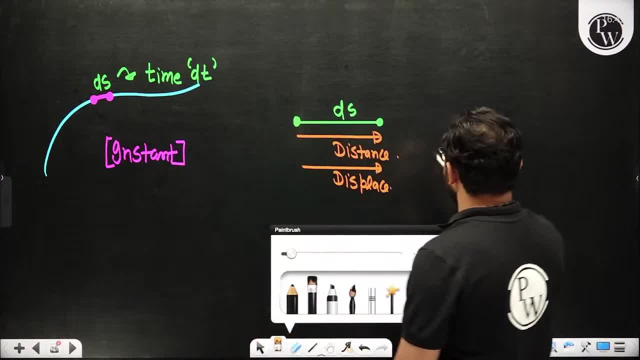 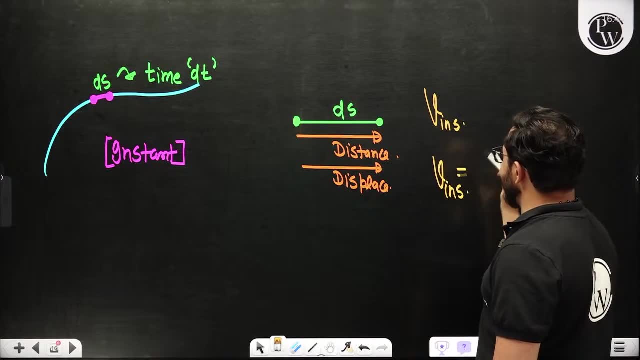 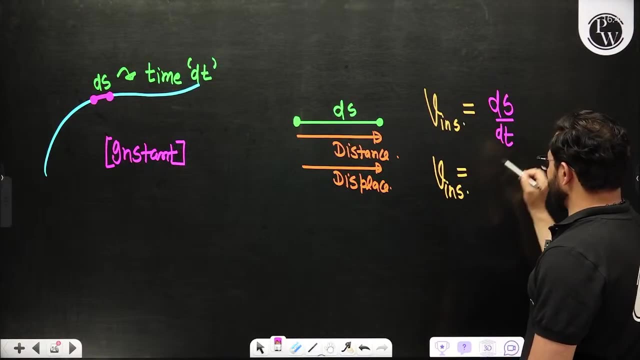 Distance and displacement, When both are equal. So remember, For a particular instant And for a particular instant, Your speed and velocity. The magnitude of both is same. And what happens? Total distance is gone. Total distance upon my time. Total distance is gone upon my time. 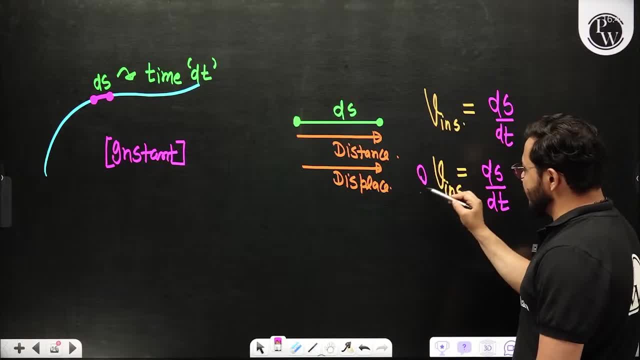 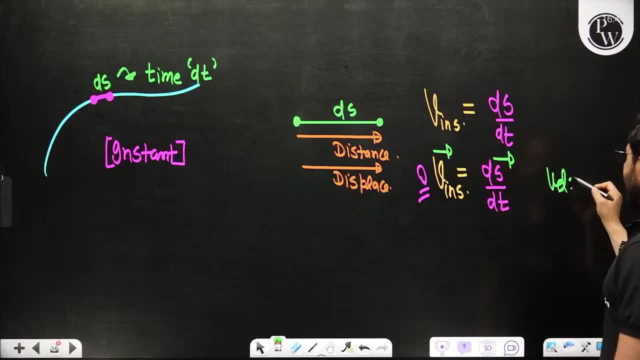 When you talk about instantaneous, Instantaneous Velocity, Then you just don't forget to put the vector sign above, Because velocity is vector quantity. So this is instantaneous velocity, Whereas the magnitude of both is same. And this is the speed for me. 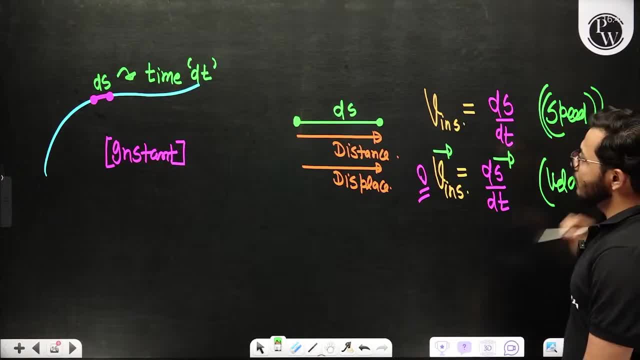 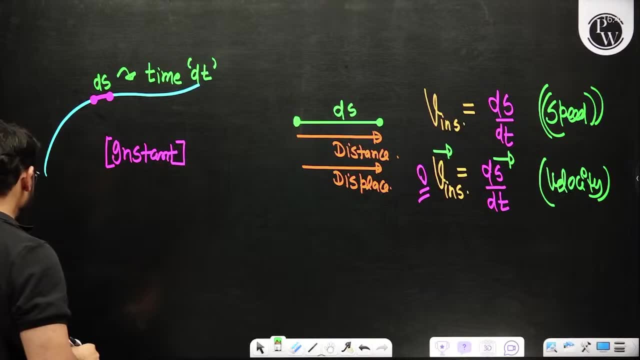 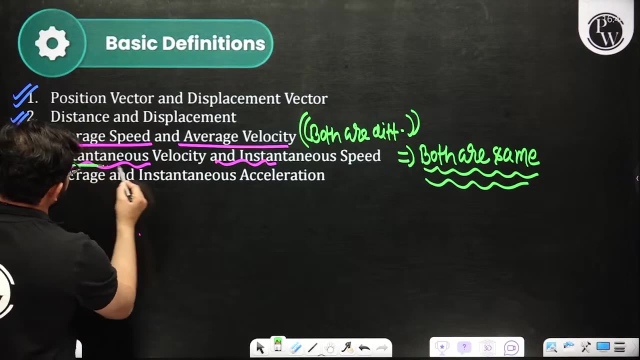 So I hope you got it. the concept: Did you understand the concept of instantaneous speed and instantaneous velocity? Tell me quickly, please. Both of you understood All the students. tell me quickly What I want to say. Did you understand that instantaneous velocity and instantaneous speed are both same? 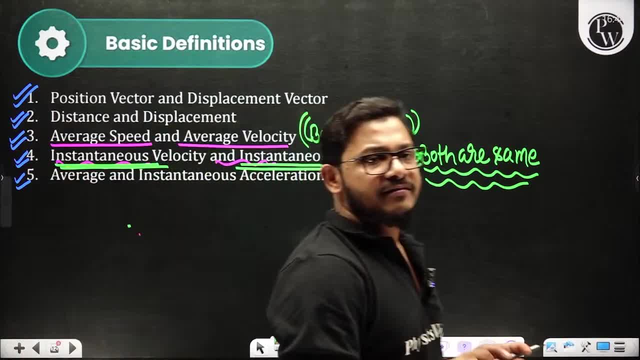 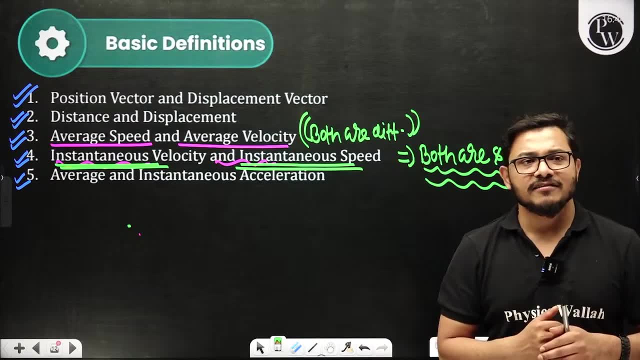 Both are same. There is no big difference between the two. Please tell me quickly. All the students message me quickly. 82 students are watching the lecture. All the students message that. all of you understood the concept. I hope you got it, the concept. 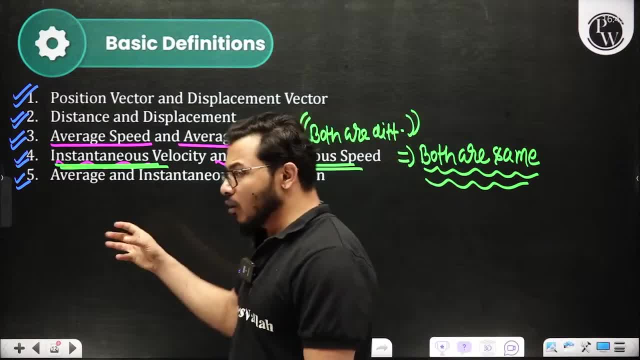 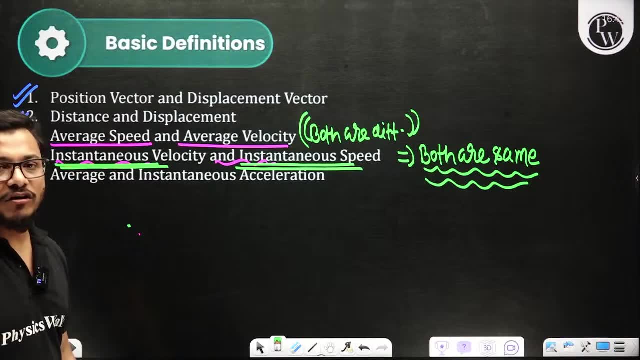 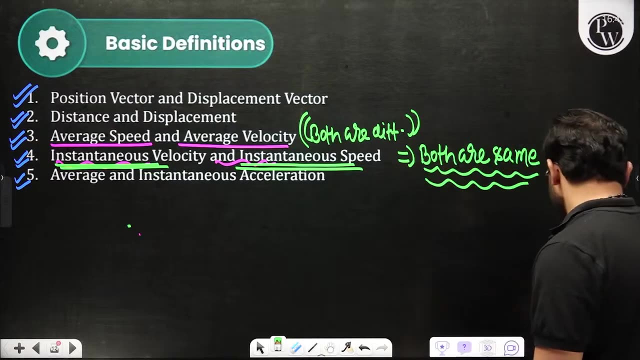 All of you understood So: instantaneous velocity and instantaneous speed. you have understood all the things here, How I have written all these things to you very good, very good. Now I will talk about the next point. The next point is average and instantaneous acceleration for me. 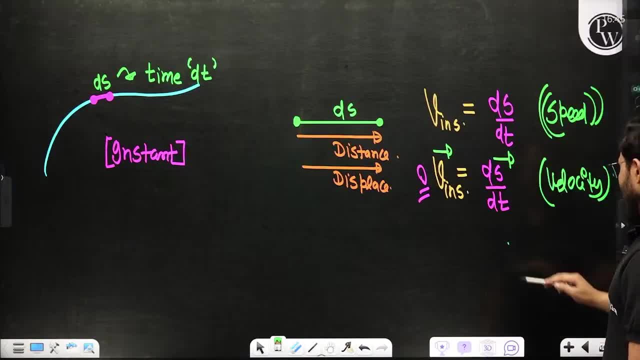 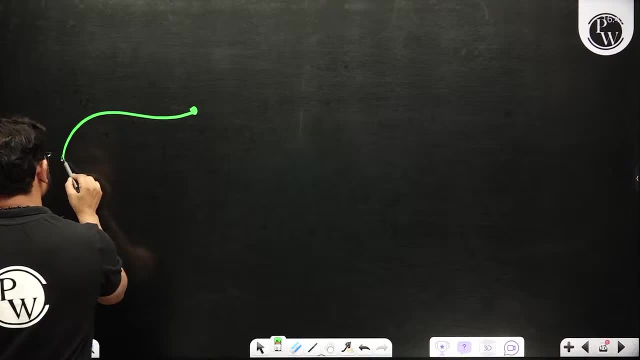 So I also talk about average and instantaneous acceleration. Let's understand a little about what that is. Suppose you have made a path here And, after making the path, suppose this is the starting point for me. Suppose, at the starting point, your original velocity is Vi. 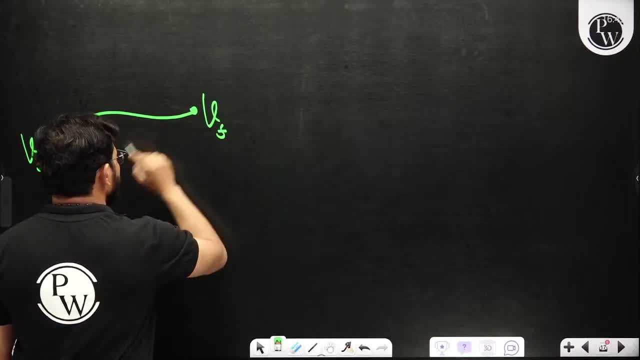 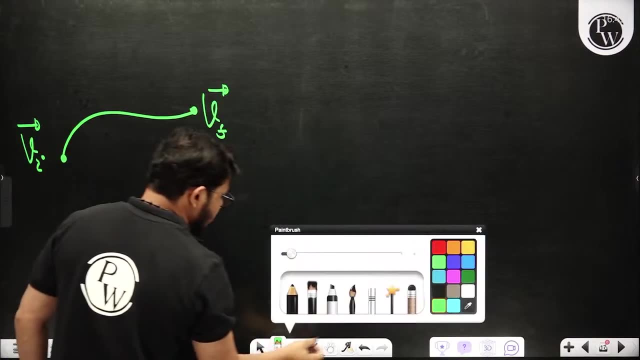 And after some time you have the final velocity Vf. So you had one total velocity Vi and one total velocity Vf From here to here, from the starting point to the ending point. the time you have taken- suppose that time is T for you. 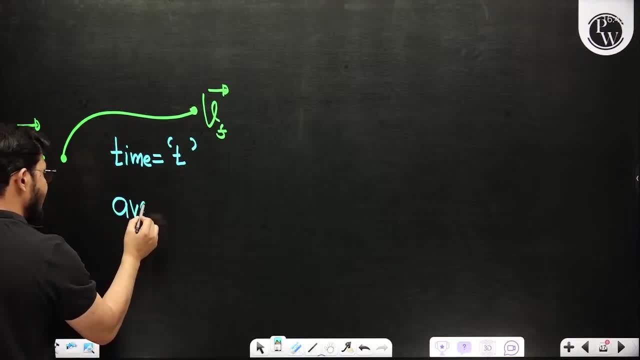 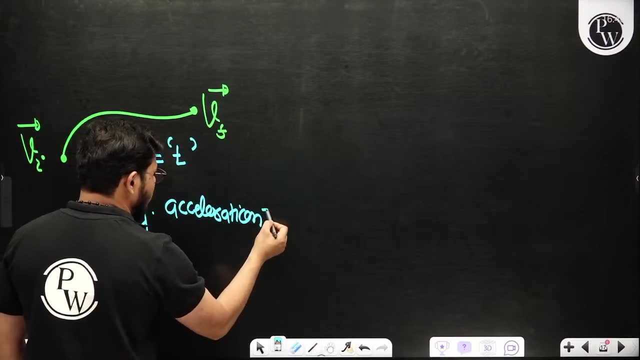 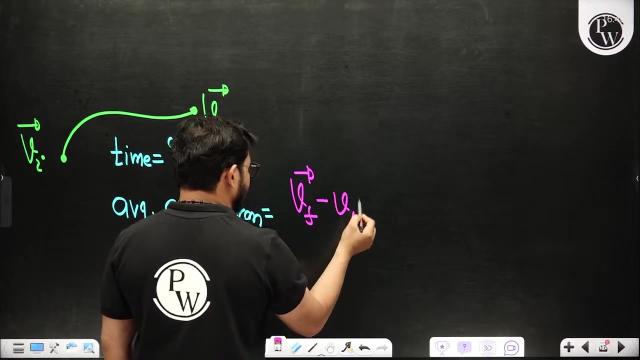 If someone asks you tell me the value of the average acceleration, What will be the value of the average acceleration? So the value of the average acceleration is the change in a velocity. So that will be Vf and minus Vi, Vf minus Vi and total time in upon. 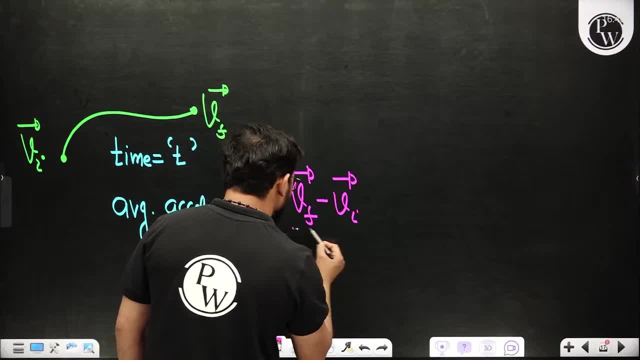 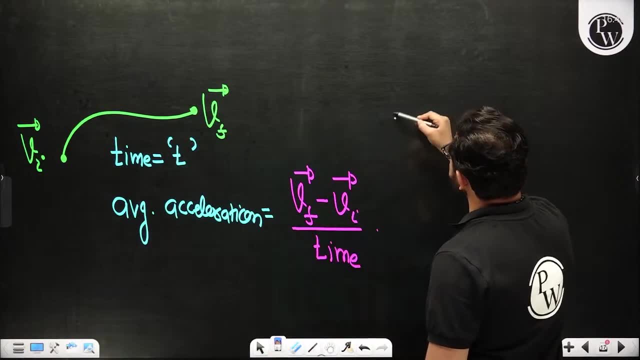 What will be in upon? It will be total time, So that one is called average acceleration, That one is called average acceleration. If we talk about instantaneous, So suppose you have reached from here to here, So instantaneous is calculated for a short time. 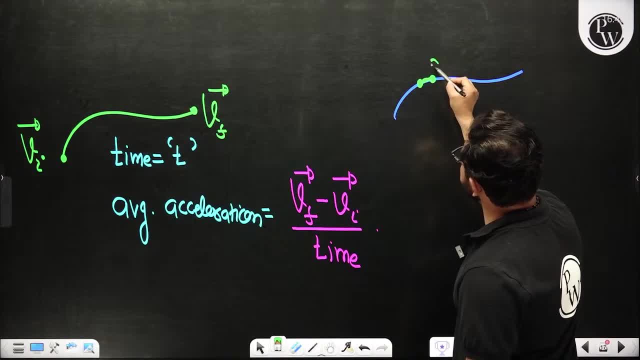 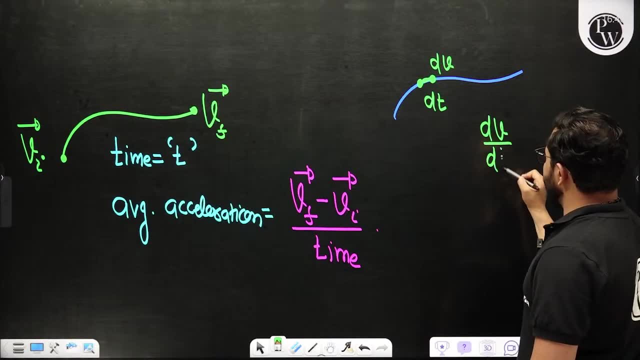 Suppose, in a short time the change in your velocity is dV And in a short time your dT is made. So change in a velocity dV and upon dT And that one is become is equal to instantaneous acceleration. I am talking about a particular instant. 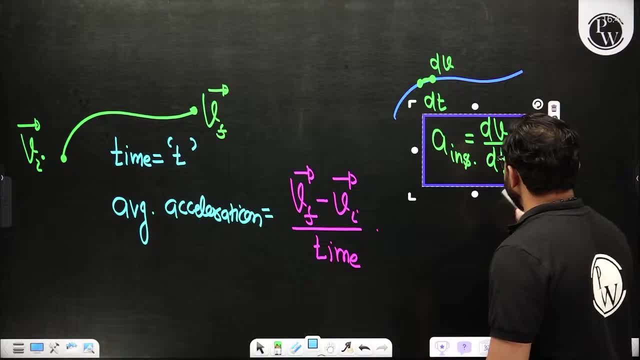 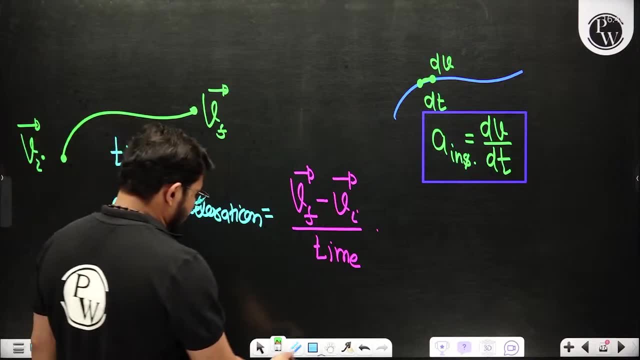 Instant means for a short time, So that one is called dV upon dT acceleration. So you have two ways to write acceleration. One is average and the other is instantaneous acceleration. So I hope you got the concept. How many of you have understood about these two? 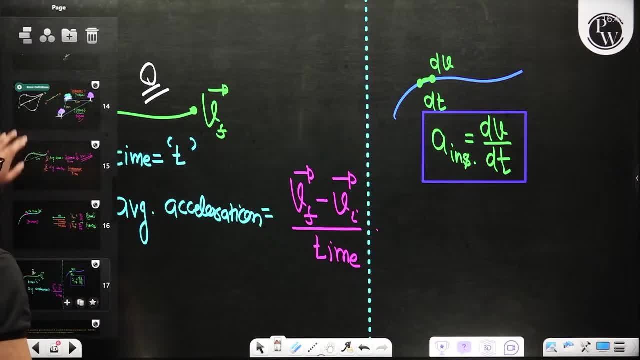 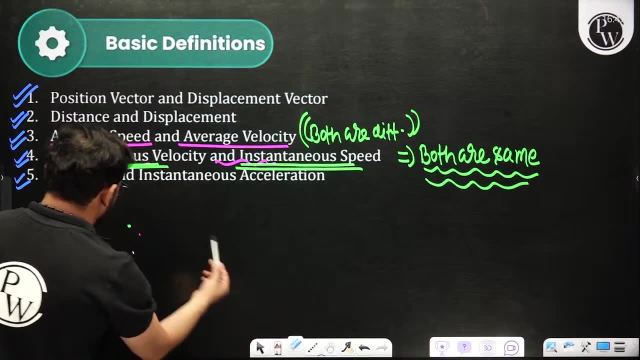 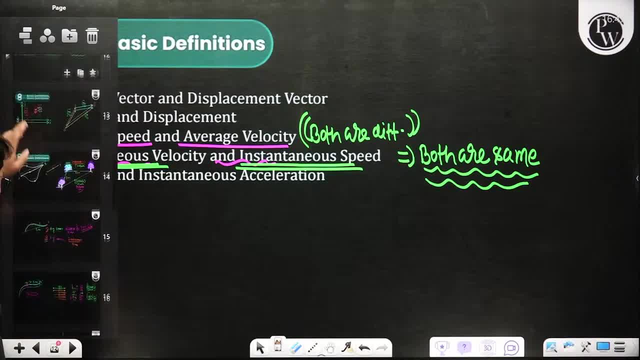 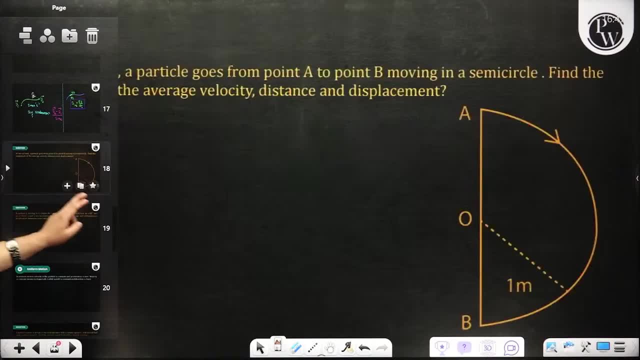 So everything is clear, isn't it Very good? Now I will do one thing: I will solve some numerical questions on them And after that I will move ahead. Not now. First, we will solve the question, After that we will move ahead. 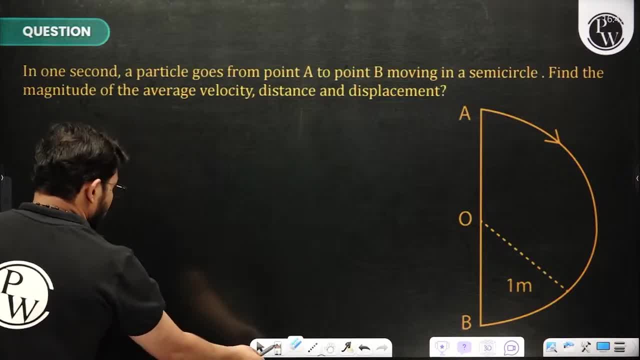 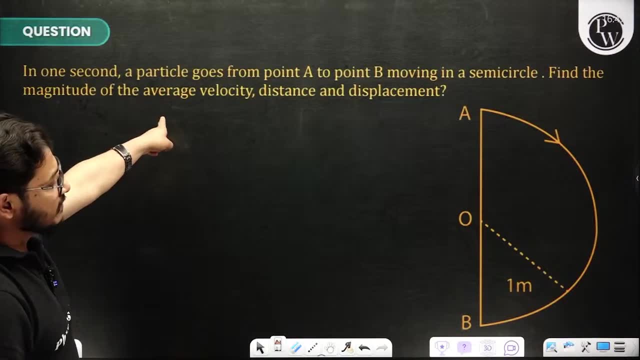 Read the first question. Look at the question. What is it asking in the question? Please look at it. It is asking one second. In one second Means: what did you do In one second? one particle went from point A to point B. 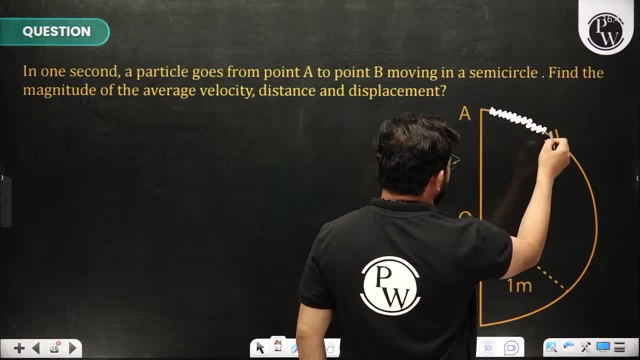 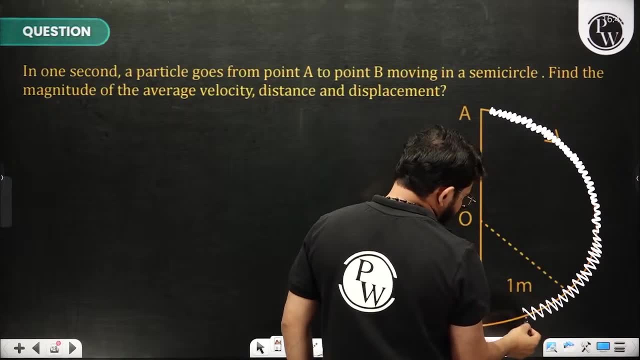 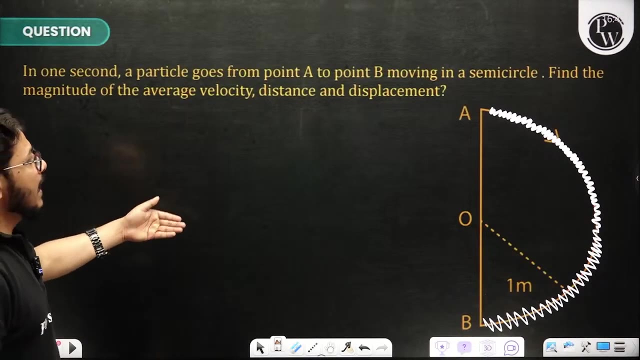 So to go- it is following this path- And to go from A to B, the time that the particle is taking is one second And the path on which it is moving, the radius of that circle, is one meter. Very good, Find out the magnitude of the average velocity and distance and displacement. 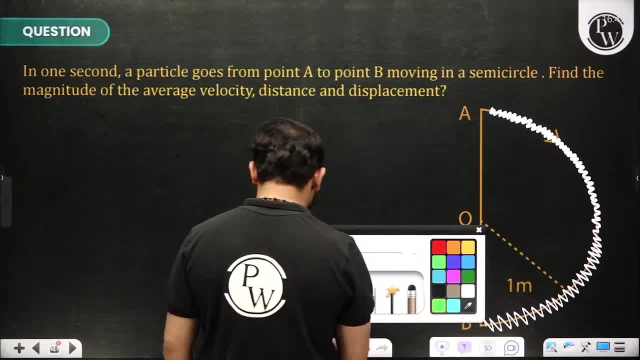 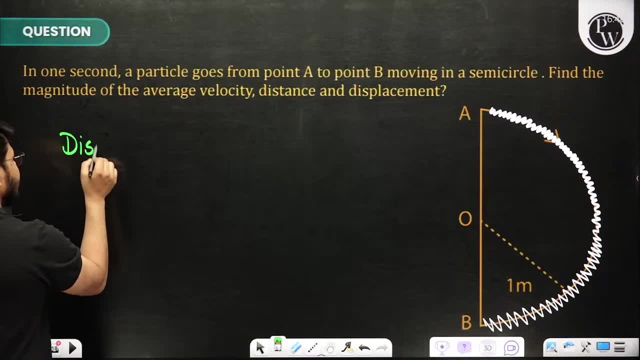 How much distance and displacement you have. How much displacement and distance you have, The distance gone alone from the actual path. what will you get? What will be the distance? So how much distance will it be? This is the periphery of the circle. 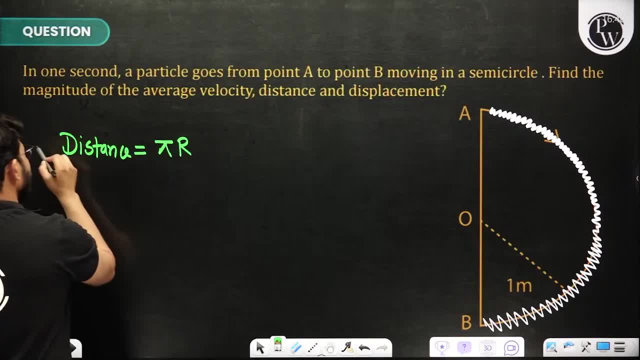 So the length of the periphery of the circle is pi r. How much is the length of r Pi r? How much will it be Pi r? So if I talk about the distance here, then what is the value of pi in the periphery of the circle? 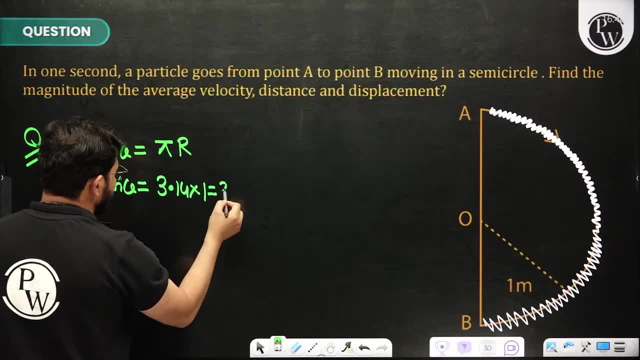 3.14.. And the value of r is 1.. So that one is becoming 0., That one is becoming equal to 3.14 meter. So this is the answer of the question. for me, This is the answer of the question. 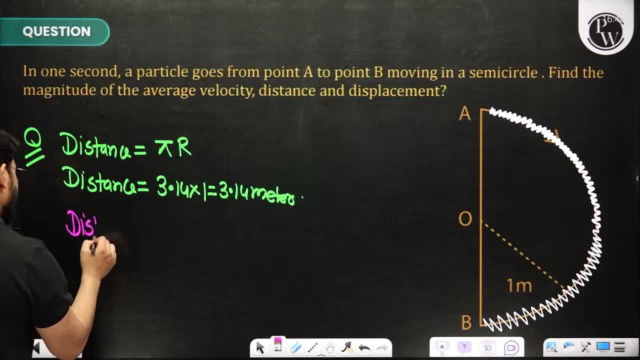 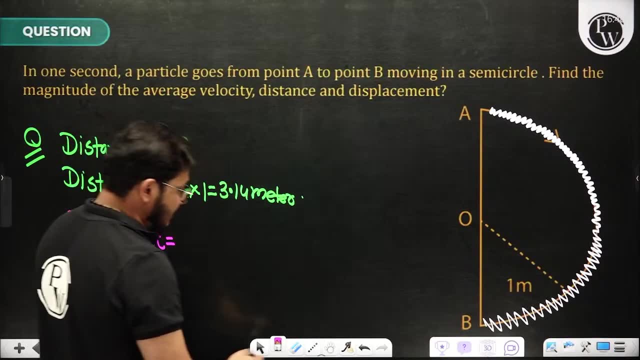 If someone asks you about displacement, what is the value of displacement? What is the meaning of displacement? What is the meaning of displacement? Displacement means that you add the starting point to the ending point. So I added the starting point to the ending point. 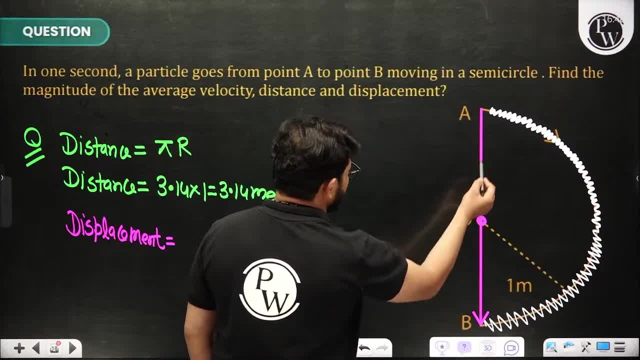 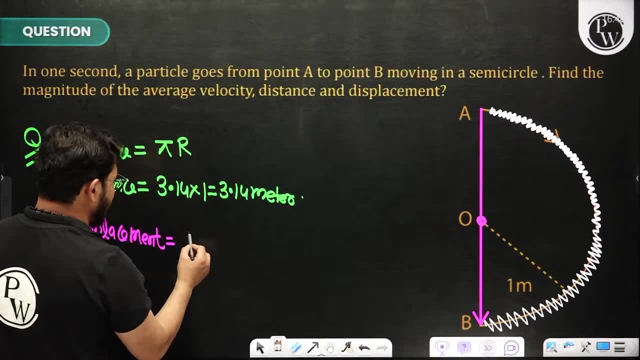 This is the diameter of it. Now, this is the diameter because this is 1 and this is 2.. So 1 over 1 is 2.. So this is the diameter. This is the diameter of the entire semicircle. So the gap between A to B is 2 meters. 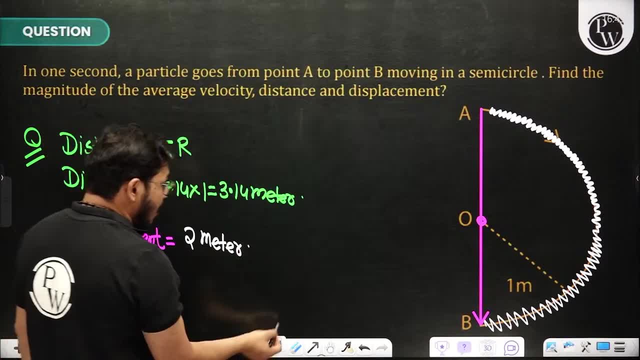 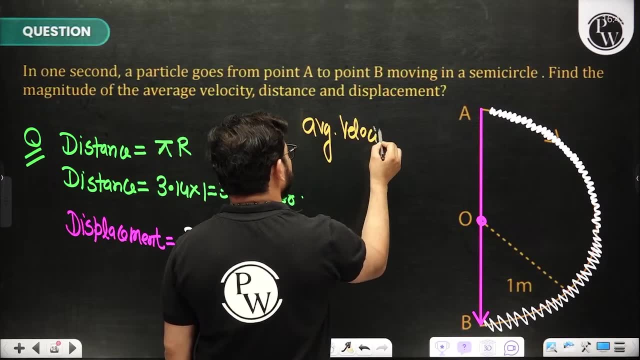 That is directly 2 meters, So displacement is 2 meters. Now, if someone asks you to tell me the average velocity, So if someone asks you to tell me the average velocity, Average velocity means displacement, So displacement is 2.. Time in the upon. 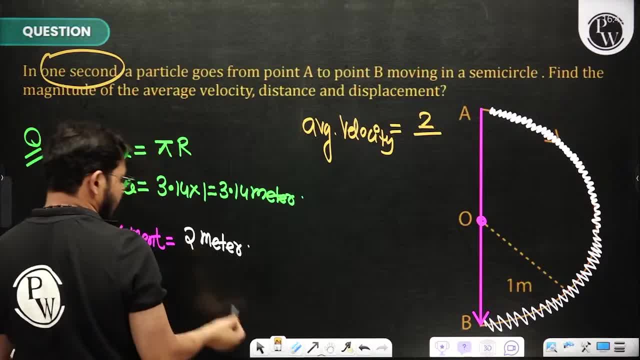 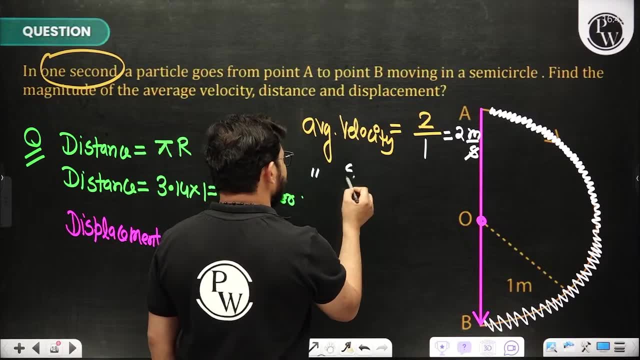 And how much time is taking In a 1 second? It takes time of 1 second. So do 1 in the upon, Do 1 in the upon, So the answer is 2 meters per second. Very good If someone talks to you about the average speed. 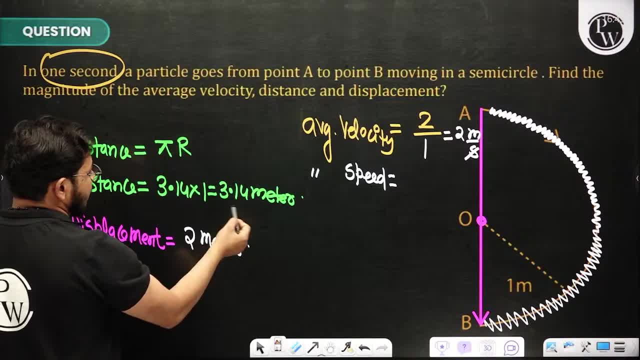 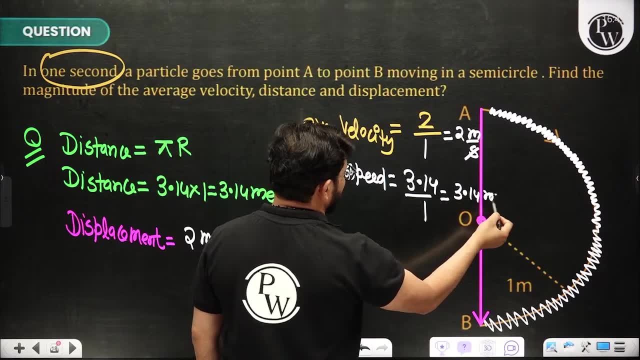 So the average speed becomes equal to. So the total distance is 3.14.. And the time in the upon And the value of time is 1.. So the time in the upon is 3.14 meters per second. So I hope you got the concept. 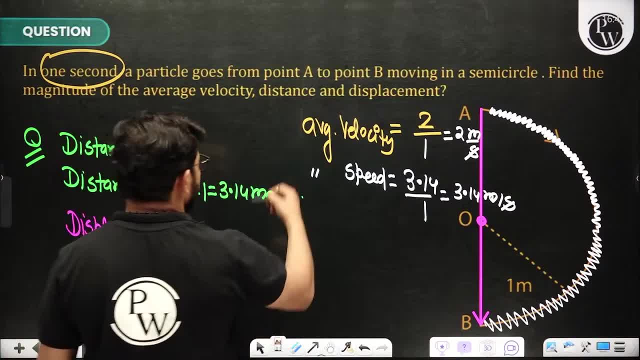 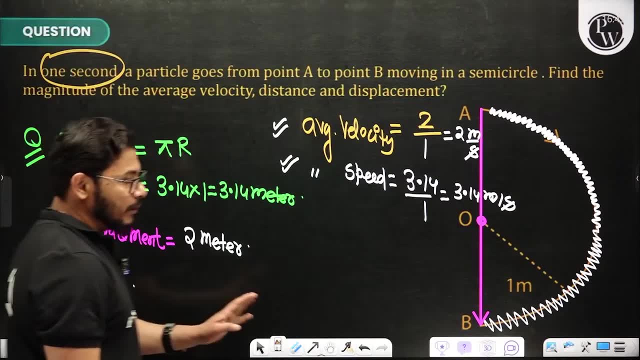 You have understood both the things here, That how much is the average velocity And how much is the formula of the average speed. So everyone understood what I said. Any child has any problem in this numerical question? Tell me quickly. Everyone got the question clear. 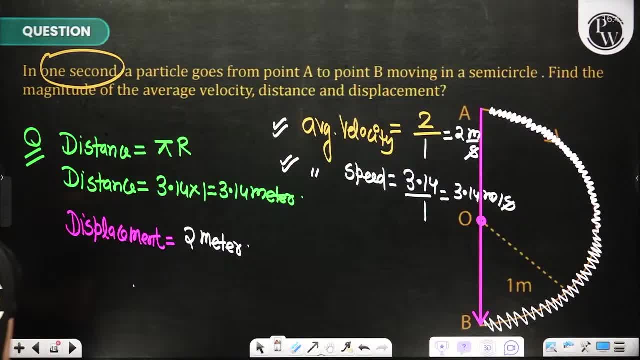 Quickly. Everyone understood the question. Any doubt, Any child? No, The question is clear. Very good Now. everything is ok. Very good, Now we will move on to the next question. Please, let's talk about the next question. We will read the question carefully. 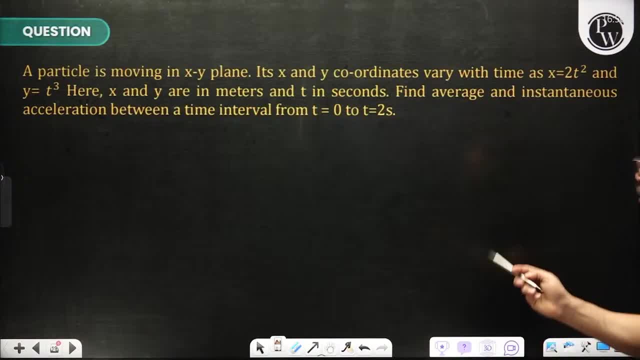 What is written in the question? First read the question. It says there is a particle, It is moving in some xy plane. So first make the xy plane So that one is the xy plane. So there is a particle moving in the xy plane. 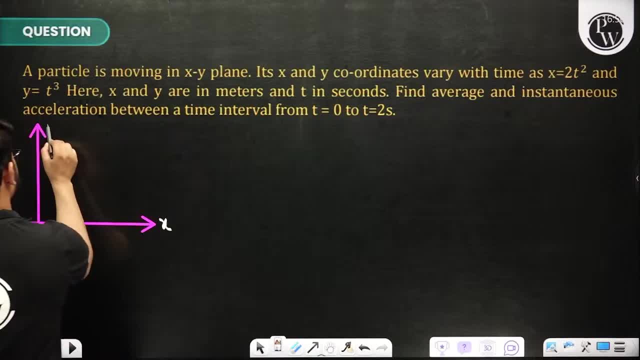 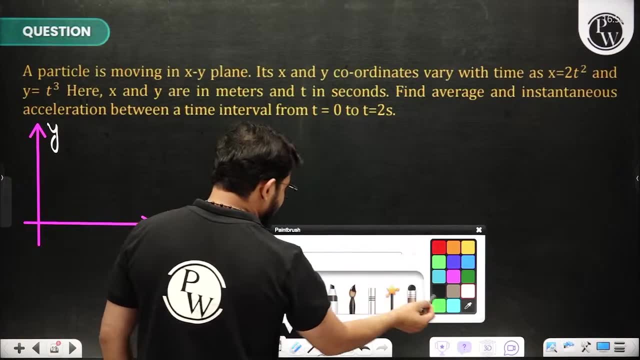 So here it is: A particle is moving in the xy plane. I made it. It says that its x and y coordinates are varying with time. So in the question you have given the value of x. That how much is the value of x? 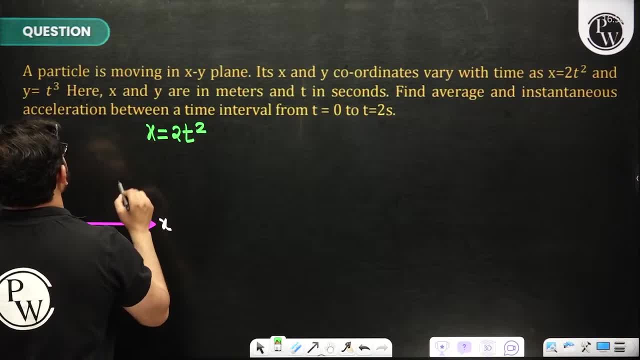 That 2 t square? Very good. And what is the value of y T power 3.. This is given in the data. Ok, It says that x and y are in meter and time is in t second. Find out the average and instantaneous acceleration. 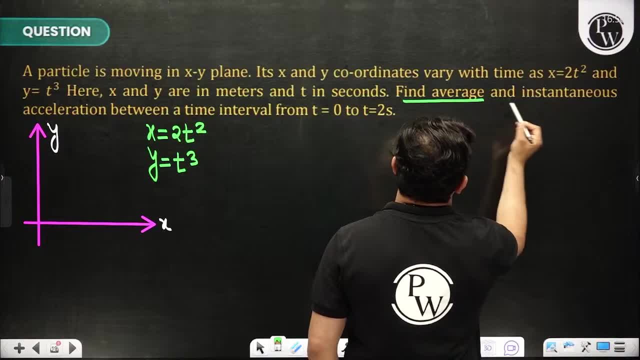 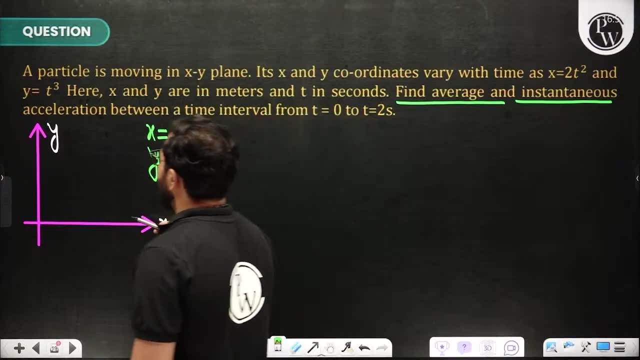 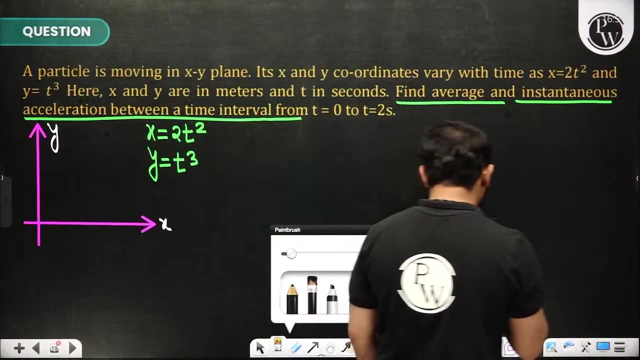 You have to talk about the average and instantaneous acceleration. You have to tell that how much is the average and instantaneous acceleration? So first I will talk about how you will calculate acceleration. First you tell me once that, how will you calculate acceleration? First thing: 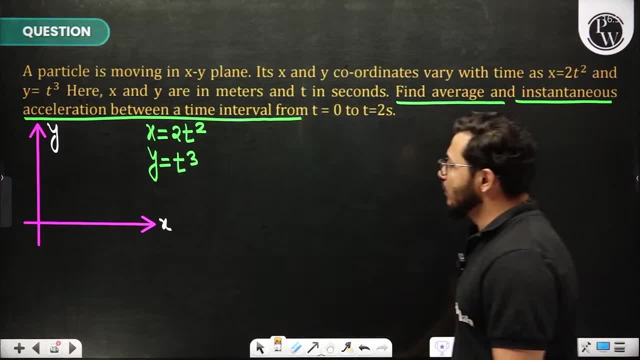 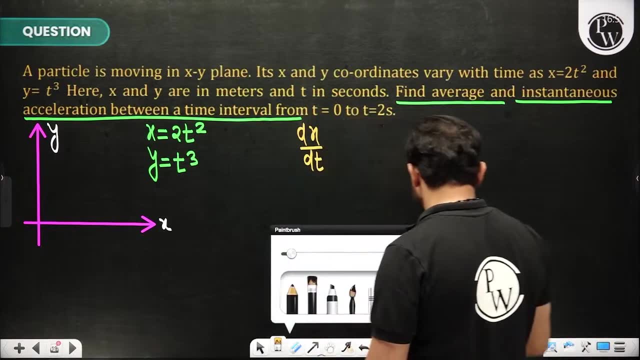 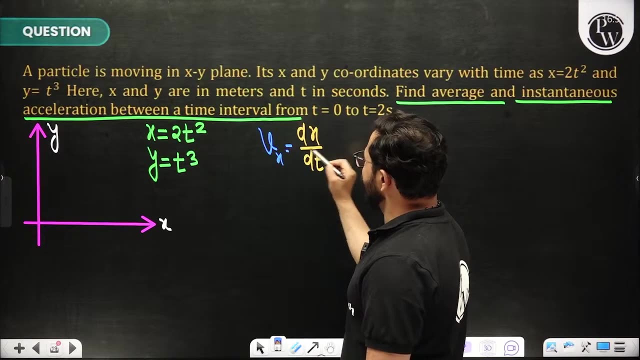 Tell me once, how will the velocity be calculated? What is the velocity? So if I make this velocity as dx upon dt, then tell me, what is dx upon dt. If dx upon dt becomes the velocity in an x direction, then how much is the velocity in an x direction? 40.. 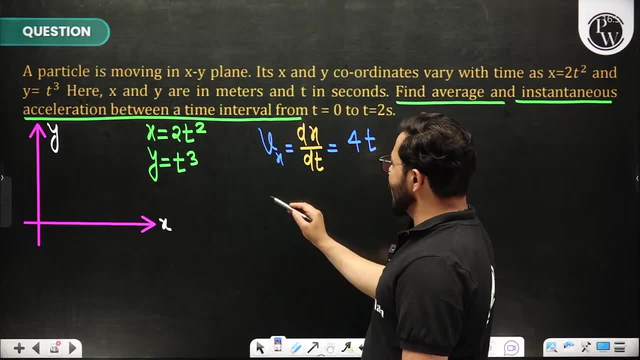 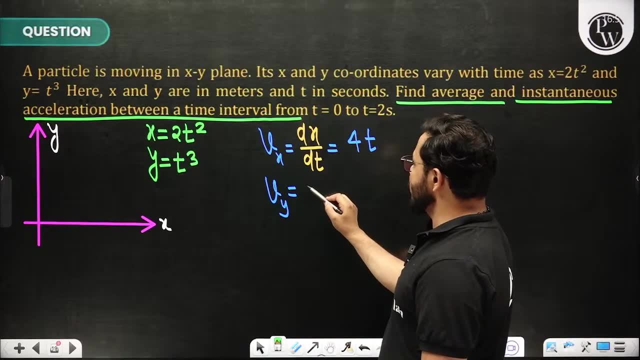 You can make the differentiation as 40.. If I ask you to tell me the velocity in a y direction, then how much is the velocity in a y direction? Velocity in y direction that one is become is equal to dy upon dt. When you solve it, then it becomes 3t square. 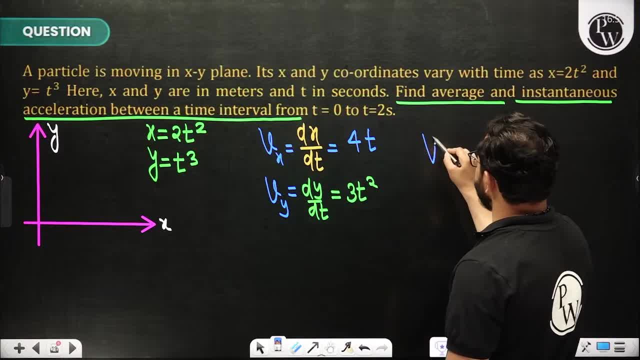 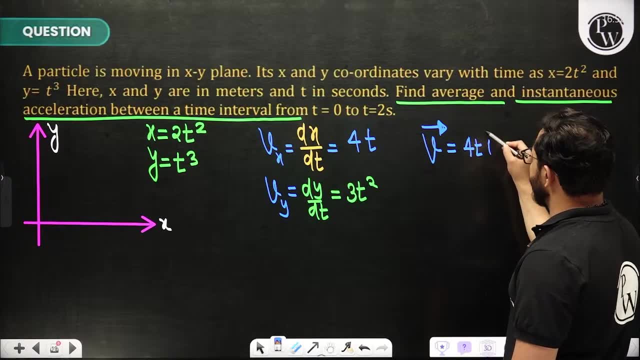 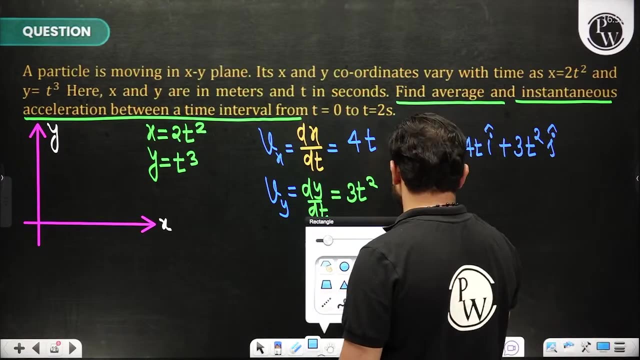 If someone asks you to tell me the total velocity of a particle, how much is it? The total velocity becomes is equal to how much is the total velocity? 4t i cap and plus of the 3t square j cap, This is the total velocity that you have. 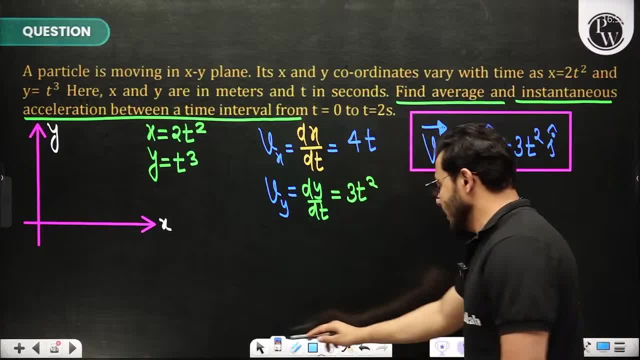 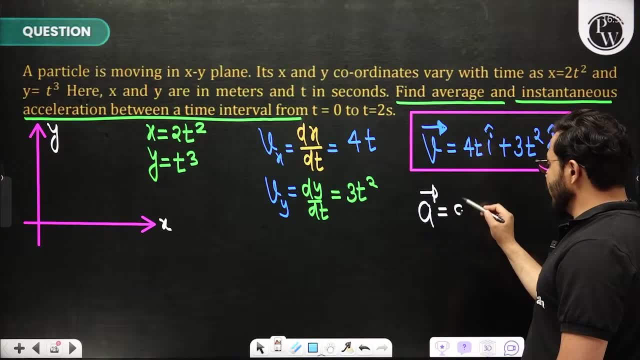 This is the total velocity. If someone asks me in a question that how much is the velocity in a y direction, Tell me the total acceleration. that too instantaneous. So do you know what is instantaneous acceleration? Total instantaneous acceleration becomes is equal to the dv upon dt. 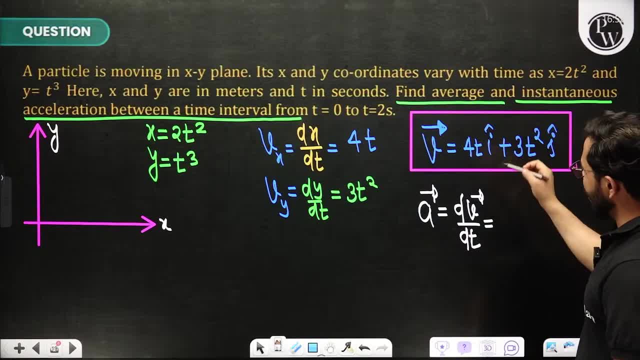 By instantaneous means to differentiate. So you differentiate it. See, if I want, then I can do it here also. If I want, then I can do it here also. When I will differentiate 4t, then it will become 4.. 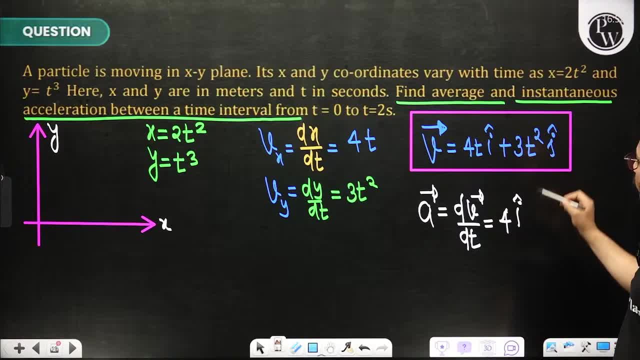 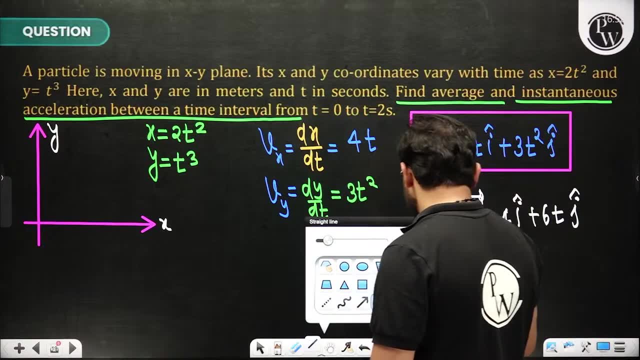 So that one is 4i cap. When I will do 3t square of this, then it will become 6t and j cap. That one is called Any particular instant. You have found the value of acceleration. So what you have written here. 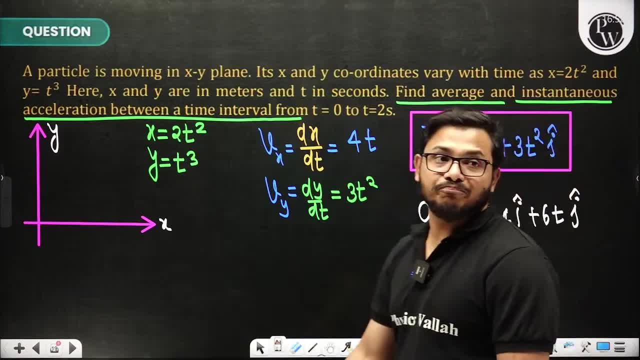 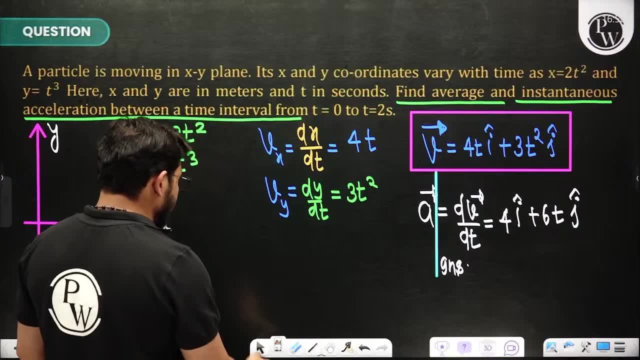 it has become the acceleration of any particular instant, Did you understand? Did you understand So that one is called the instantaneous acceleration? If someone asks me, this question has already been asked in SSE JEE. This question is of SSE JEE. 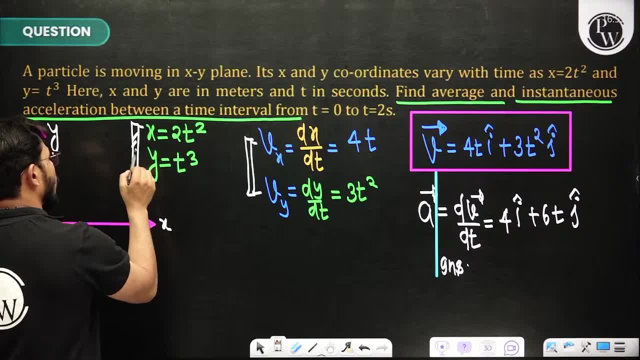 Exactly same problem. when you solve PYQ, you see this type of question in examination. You put the question of PYQ, you will see this type of question. You will see this type of question. You will see this type of question in SSE JEE. 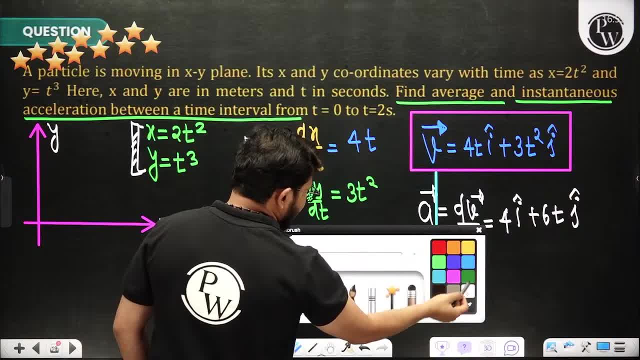 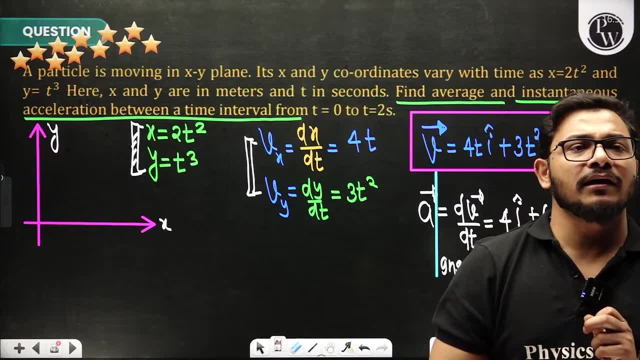 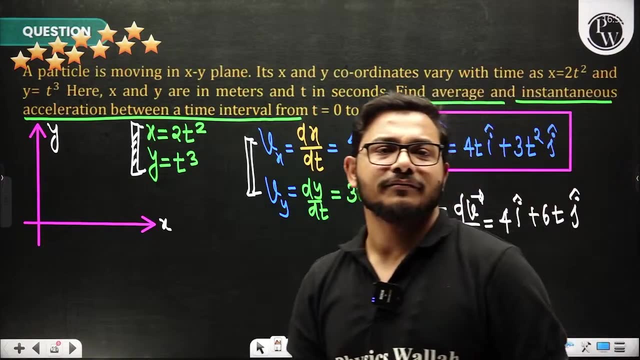 You put the question of PYQ. you will see it. You will definitely see such questions there. If I had told you that now I particularly Sir, I am Mechanics, Mechatronics Engineer, JEE. What are you talking? I can't understand what you are asking. 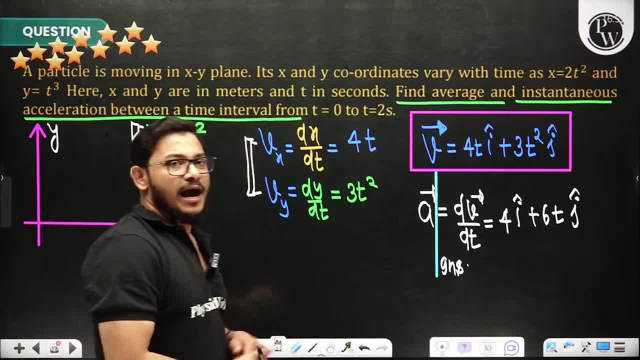 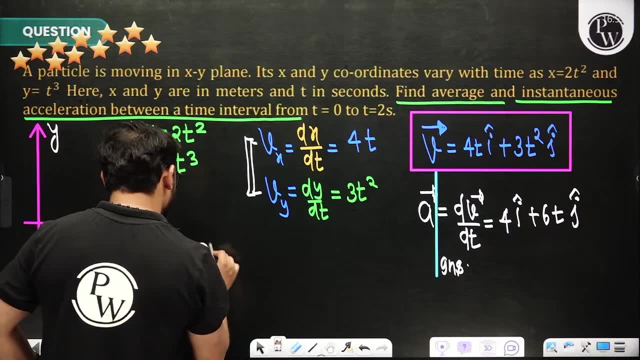 Read it, brother. You have got the value of acceleration. Now, what am I going to do here? Now, what I have to do here is, if I had asked, you, tell me the average acceleration. So what will be the value of the average acceleration? 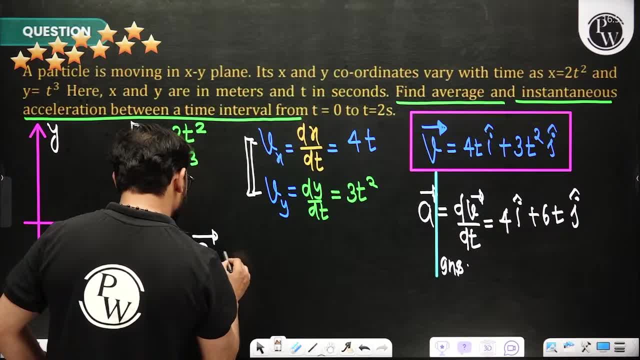 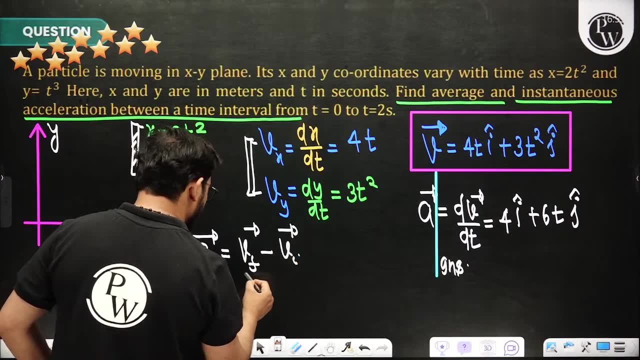 Average. What is average Average? Average means V final and minus Vi. What are you talking? You are writing absolutely right: V final minus Vi, And upon that total time, Total time. This will be the average acceleration. Now, what am I asking you in the question? 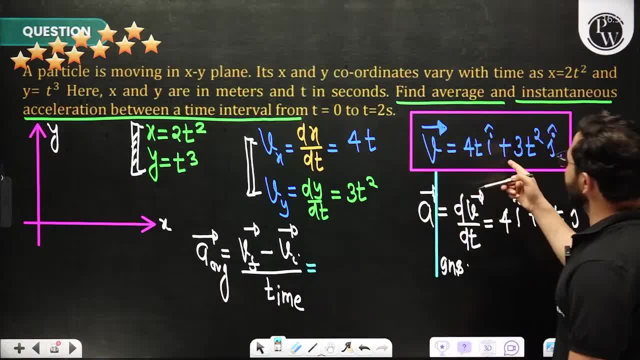 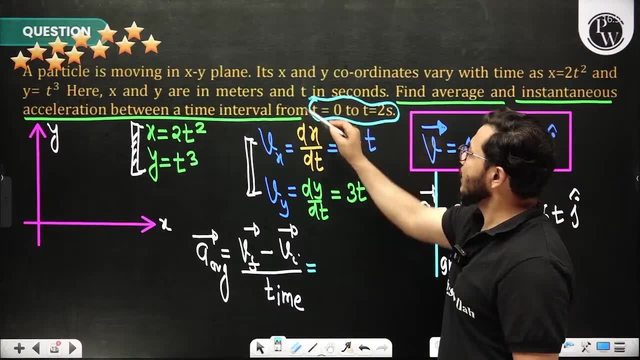 Tell me Average, Tell me, See V is this? At what time? you have to calculate this? Now you have to calculate from 0 to 2 seconds. So tell me the final velocity. time t is equal to 2 seconds. 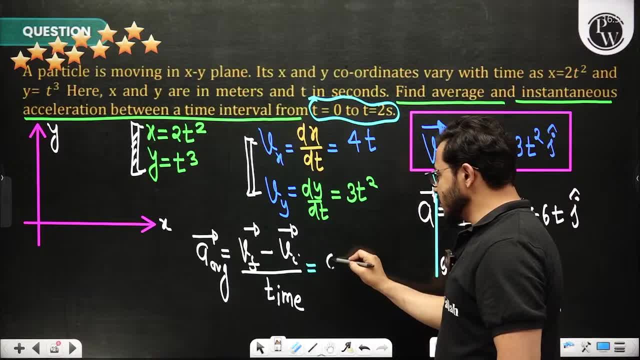 So put 2 instead of t. So how much is 4 times 2? 8.. 4 times 2 is 8.. 8, i cap, But put 2 instead of t. So 2 times 2 is 4 and 4 times 3 is 12.. 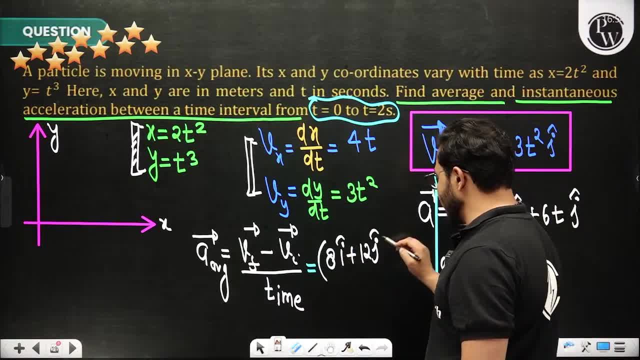 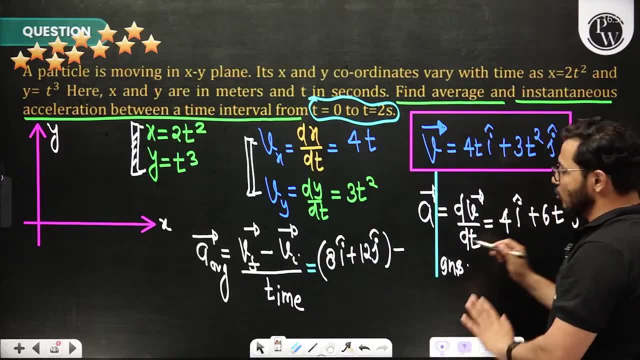 So 12 j cap. So final velocity is this much: at 2 seconds Minus Initial velocity, Time t is equal to 0.. Put 0.. 0, i cap 0.. So it went to 0.. 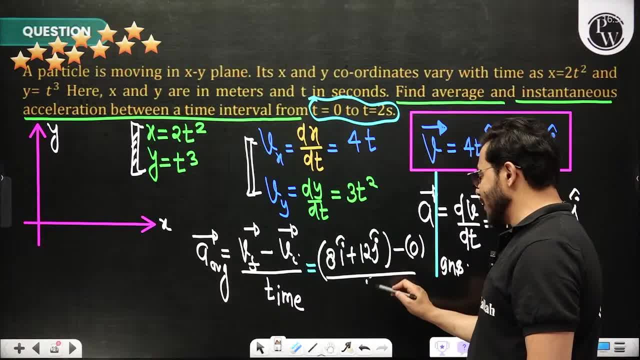 It went to 0.. It went to 0.. And upon From whom do I divide From total time? Upon me 2. When you solve it? So when you cut it from 2.. So it became 4, i cap. 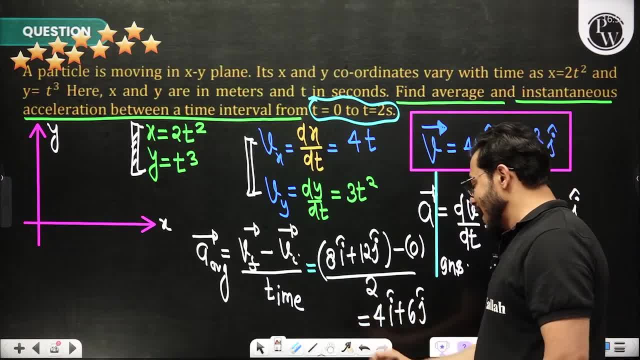 And 6 j cap. So I got this Average acceleration. That one is called average acceleration. In average acceleration you don't have to differentiate the velocity For average acceleration. what do you have to do? Direct velocity Final. 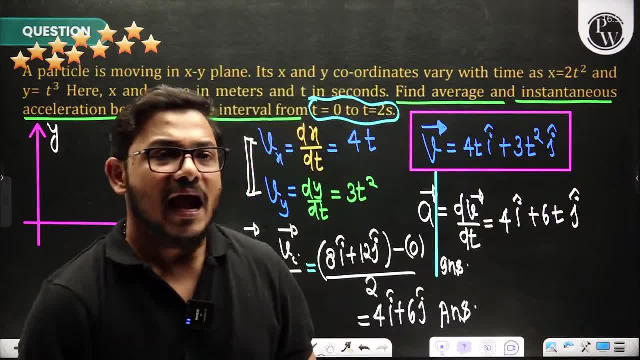 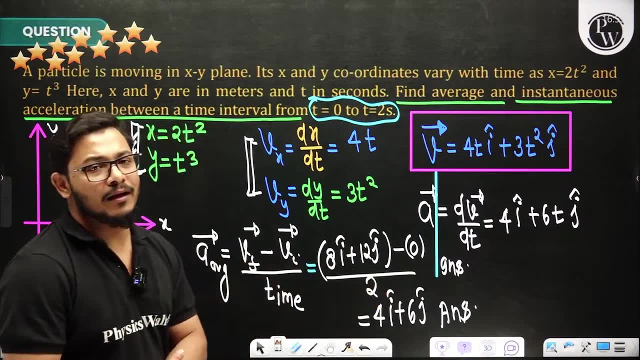 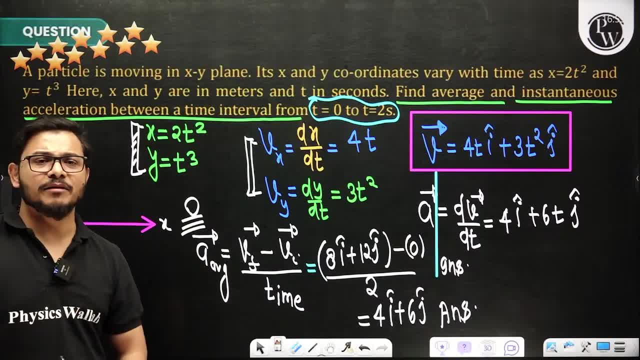 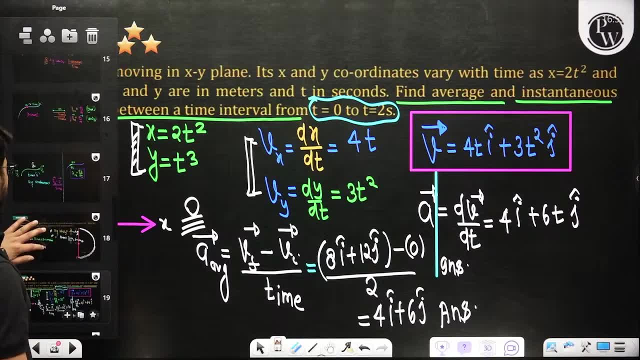 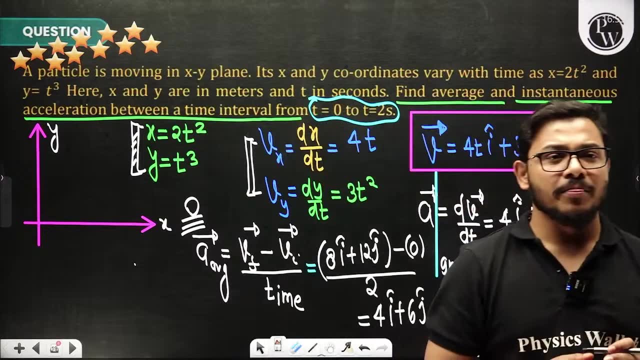 Tell me quickly How many others came to know this question. Please tell me quickly. Have you understood this question or not? Average acceleration or instantaneous acceleration? Have you understood both the things? I hope you got it: The concept: Average velocity and average acceleration. 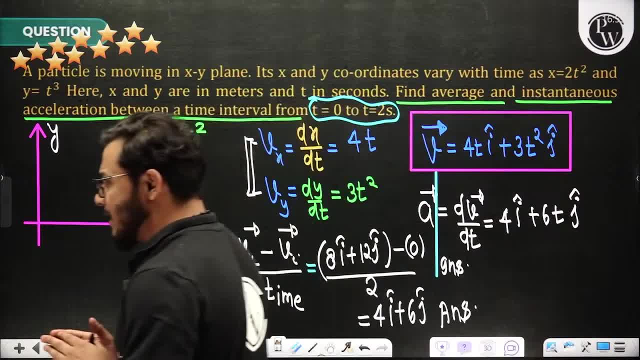 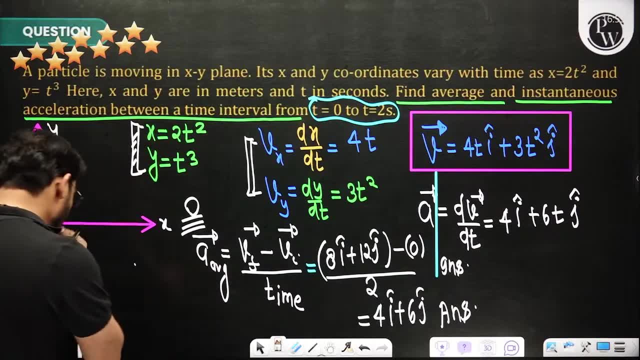 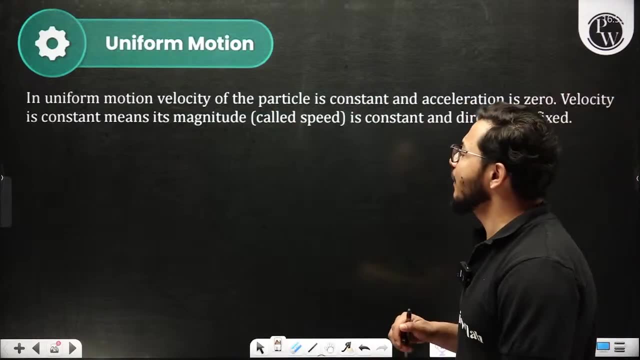 Have you got both? So I take it. So Both are clear, Both are clear. Very good. Now I am going to talk about the next point of uniform motion. What is uniform motion? Let's talk about it. Uniform motion- is that motion? 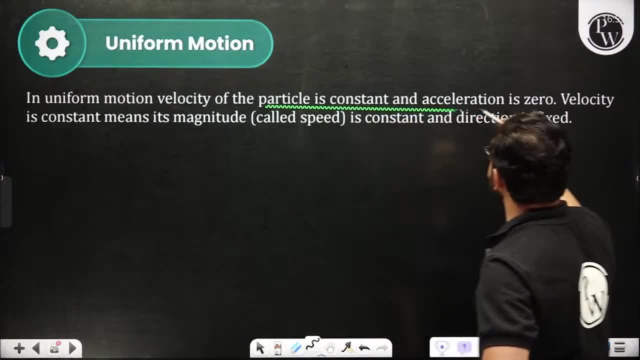 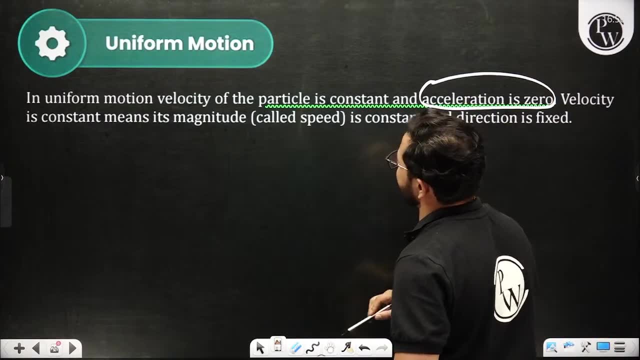 where the particle does not have any acceleration. Particle does not have acceleration. It means velocity is constant. It means in this motion, acceleration of the particle is zero. If we talk about uniform motion, then what should be the acceleration? It should be zero. 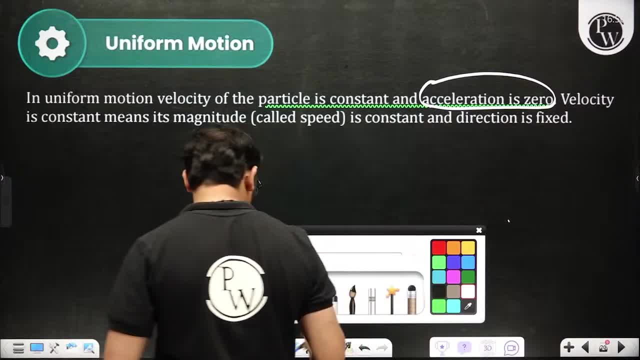 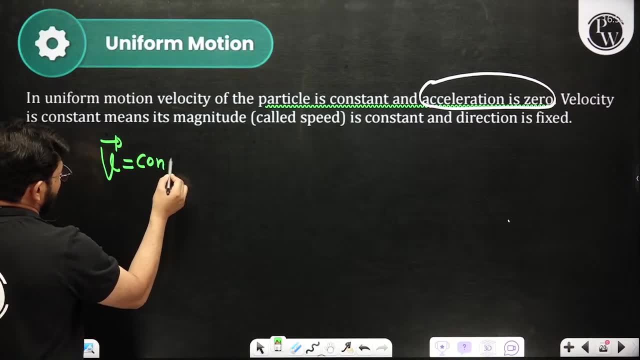 What should be the acceleration? It should be zero. Now look at the velocity. Velocity is the vector quantity. Velocity should be constant. When will the velocity be constant? When will the velocity be constant When its magnitude and direction should not change? 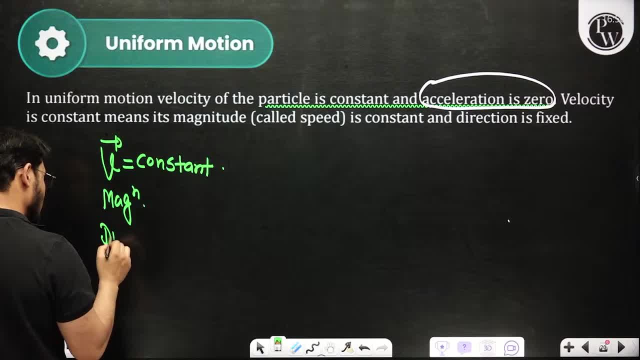 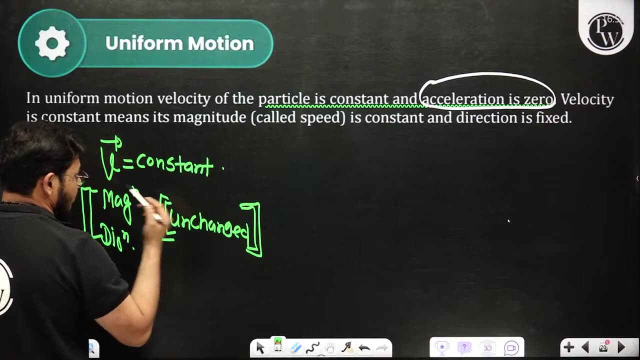 Magnitude and direction should be constant. How should both be? These two should be unchanged, Unchangeable. If they are unchanged, then the velocity will be constant. So that one is the one idea: that when, the velocity will be constant. So if the velocity is constant, 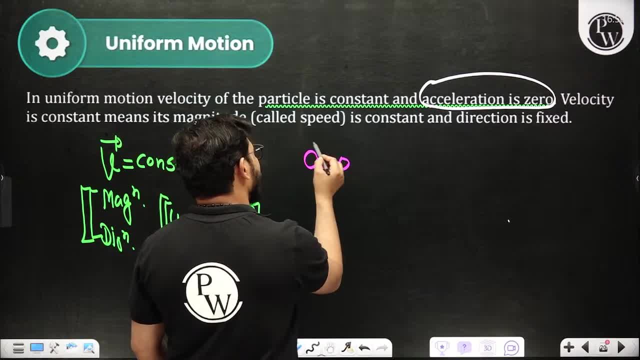 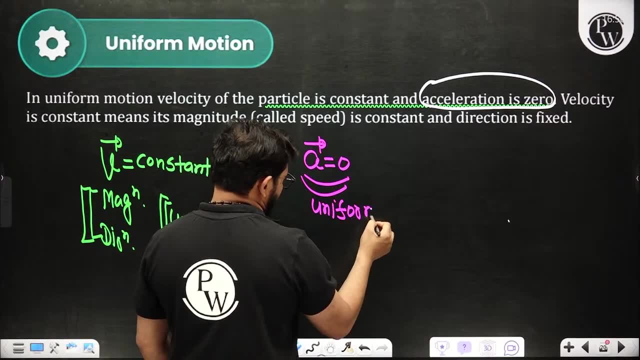 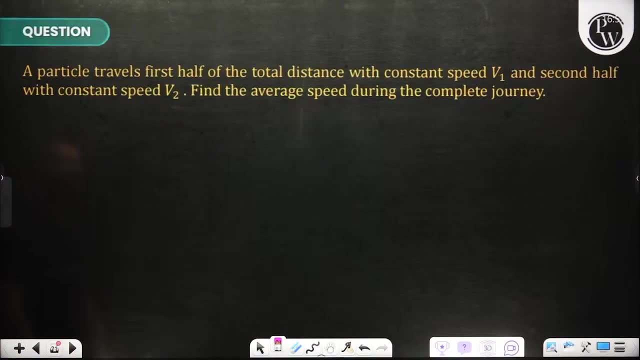 then remember that acceleration is zero. So what do you call this story of acceleration being zero? You call it uniform motion. This is what I call uniform motion. Let's look at a question on this. Now we will take another question. Here is a question. 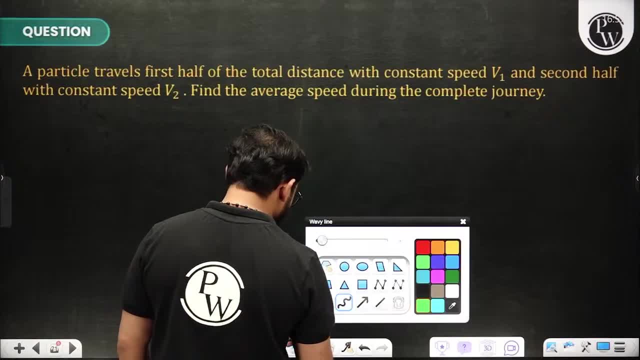 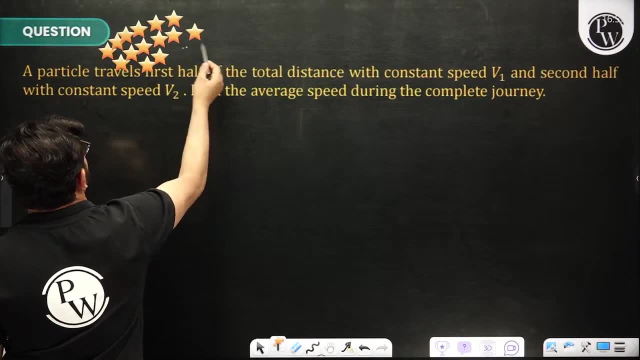 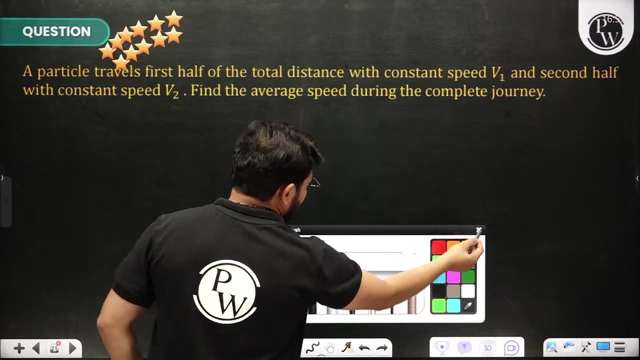 Please listen that point. Make this question a star. Make this question a star. This is a very important question. I will make this question a star. This is a very good question. Solve this question. Solve it. Read the question. In the question it says: 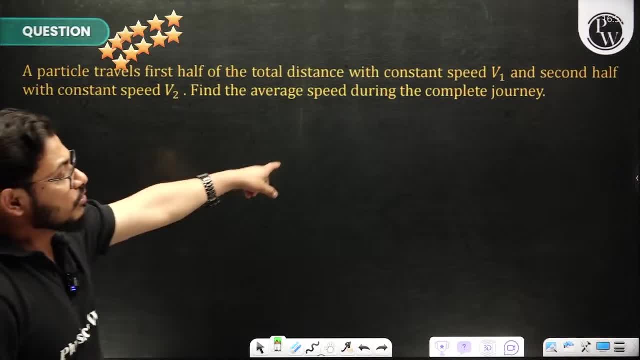 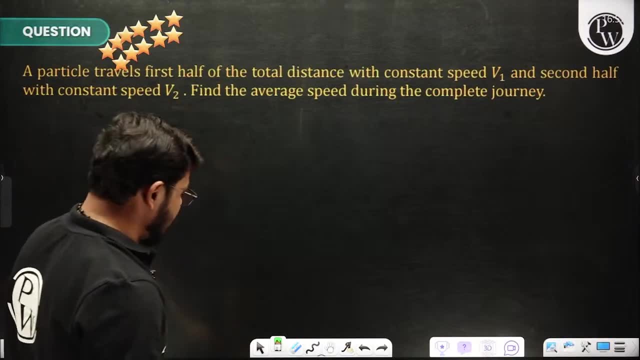 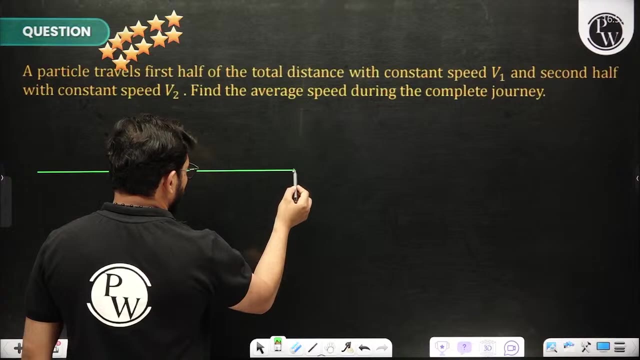 A particle travels first half of the total distance with constant speed of V1 and second half with constant speed of V2.. Find out the average speed. That means. let's assume that this is a total length. This is a total length And I have to divide this total length. 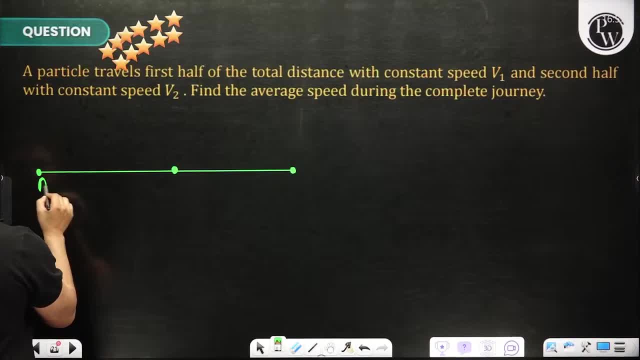 into two parts. Let's assume that you go from A to B and then from B to C, So divide it in half. From A to B you go L by 2 length, and from B to C you go L by 2 length. 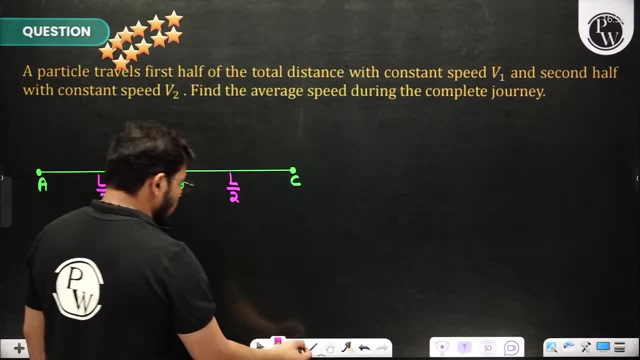 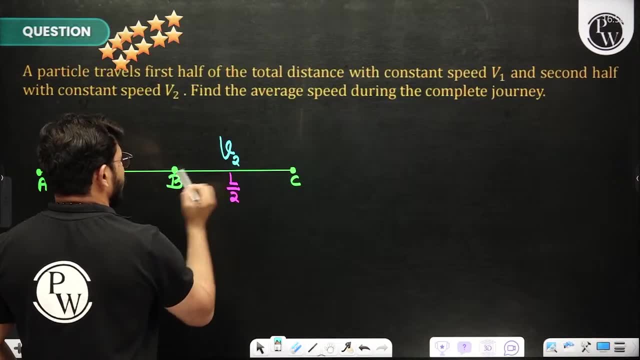 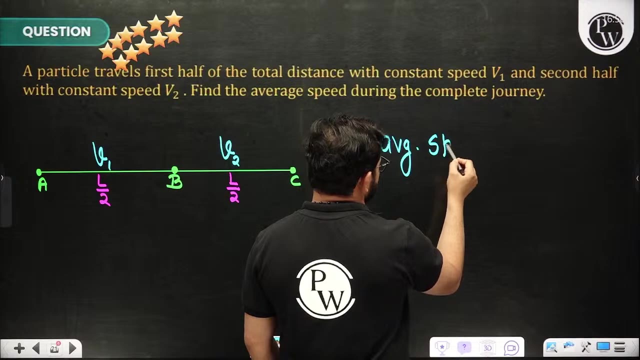 And when you go from A to B, then you go with velocity of V1. And from B to C you go with velocity of V2.. Do you know the formula of average speed? Let me tell you the formula. Average speed becomes equal to. 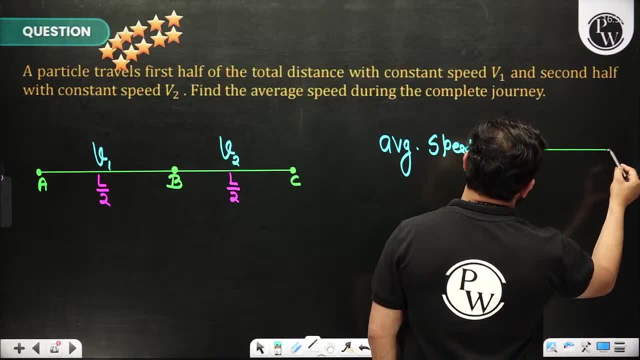 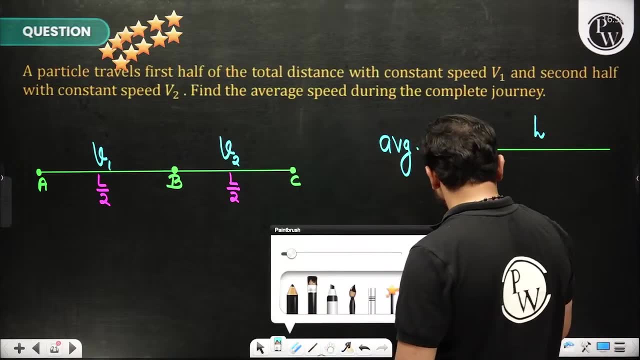 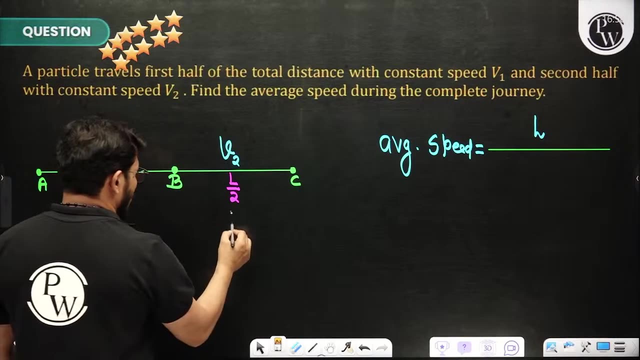 total distance. You tell me how much total distance do you go Upon total time. You don't know the total time. Let's do one thing: Let's take total time from A to B as T1 and from B to C as T2.. 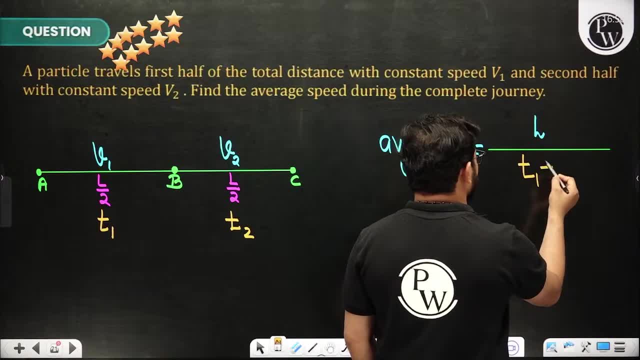 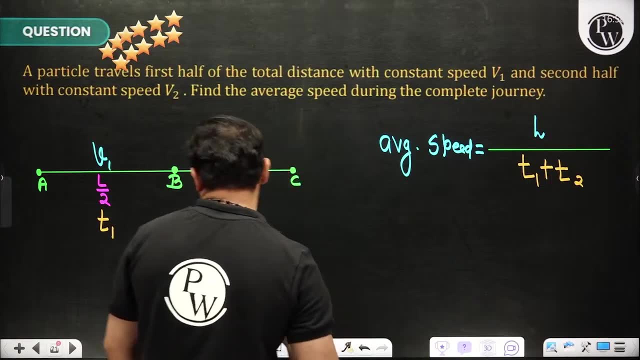 If I talk about total time, then I will call total time as T1 plus of T2.. So the question is finished. How will you calculate the value of T1?? Do you know how to calculate the value of T1?? You know how to find out the value of T1.? 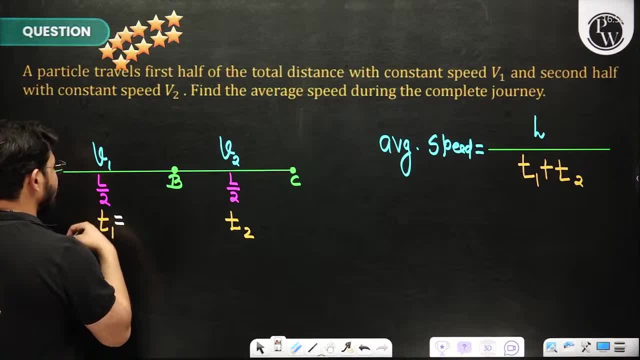 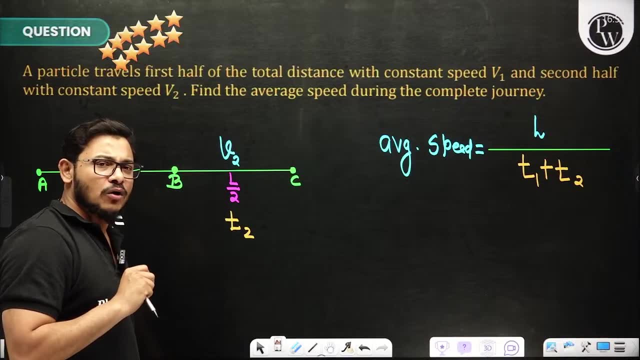 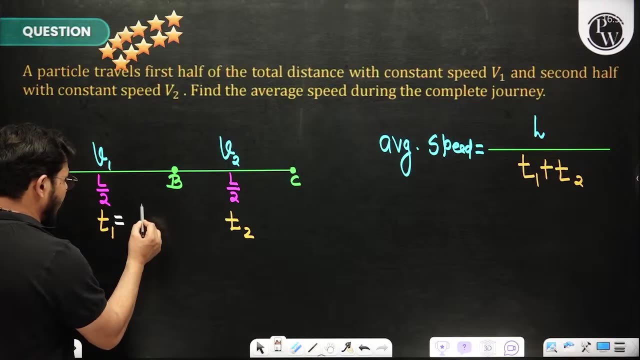 T1 becomes equal to. How do we calculate time? Speed becomes equal to distance divided by time. You must have studied a formula in your childhood. So time becomes equal to distance divided by time. So when you have to calculate distance and talk about time, 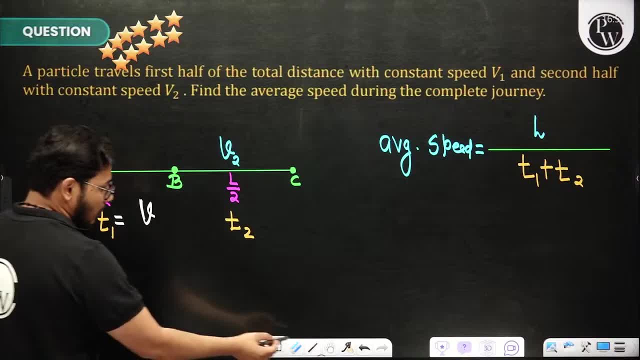 then you don't read. speed upon. Do you understand what I am trying to say? So let's do one thing: Time becomes equal to L by 2 and upon V1.. So how much is T1?? T1 becomes equal to. 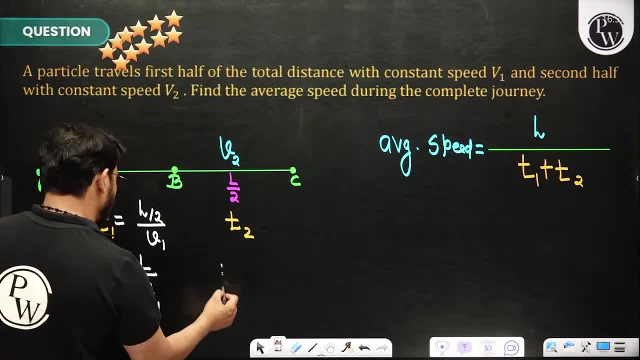 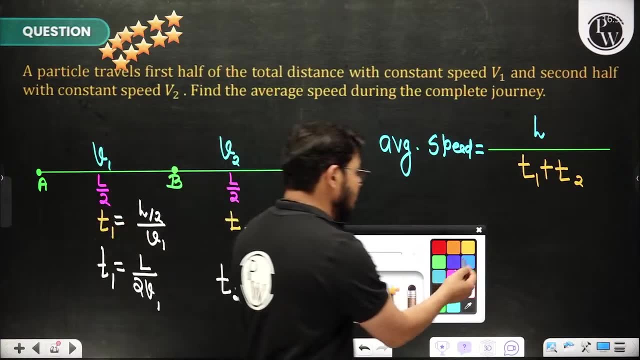 L upon 2 V1.. Similarly, you will write T2. here T2 becomes equal to L upon 2 V2.. You put the value of these. When you put the value of T1 and T2, then the average speed becomes. 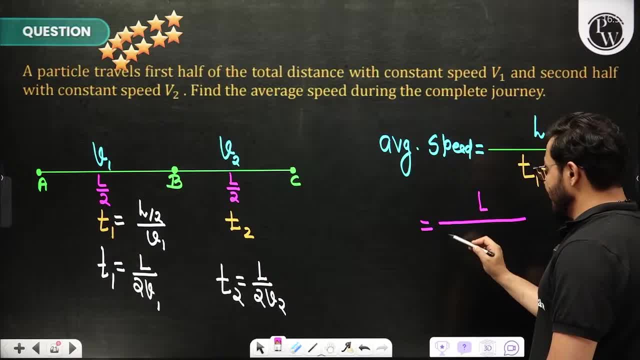 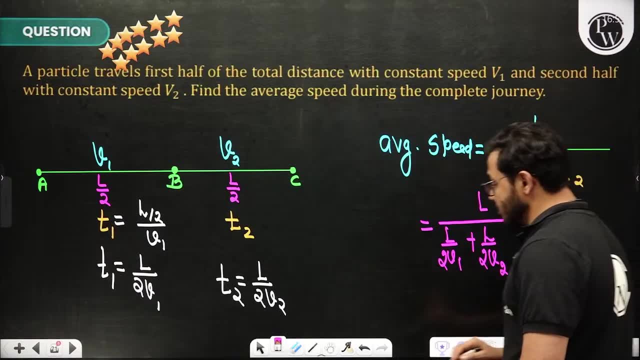 equal to L upon 2 V1, plus L upon 2 V2.. L upon 2 V1 plus L upon 2 V2.. L upon 2 V1 plus L upon 2 V2.. Solve this equation. What will you get after solving? 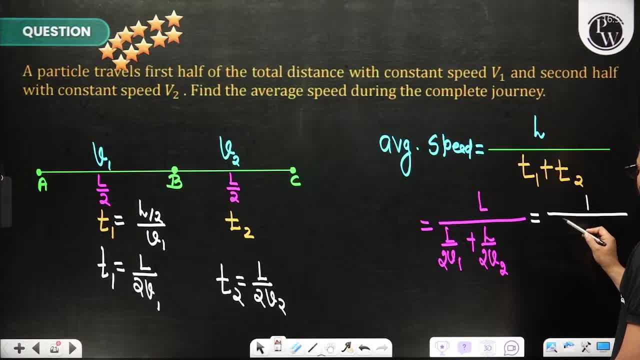 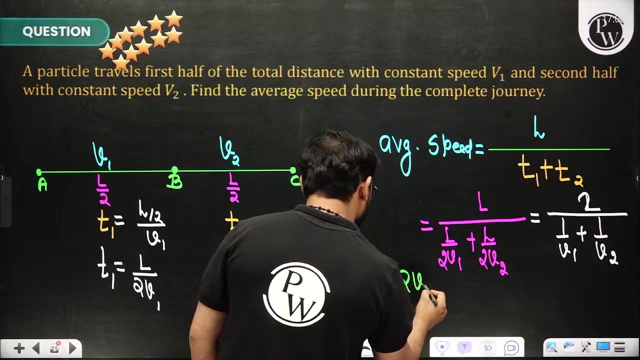 That one is 1 upon 1 upon 1 upon V1 plus 1 upon V2.. I took this 2 upward and cut the L cell. Solve this whole equation. When you solve this, then the formula of average speed will be. 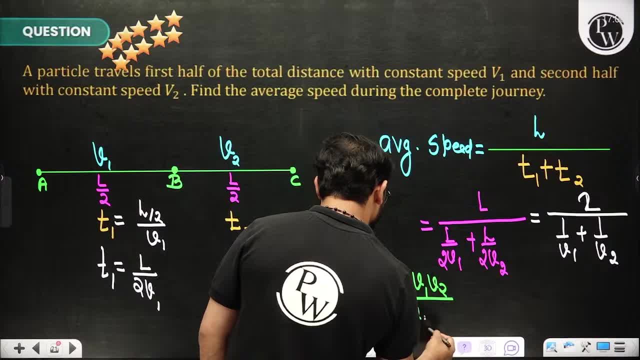 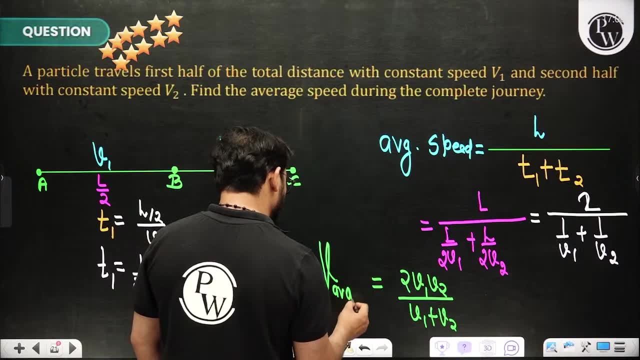 2, V1, V2 and upon me the V1 plus of V2.. So that one is called average speed. So this became the average for me, So that one is called average speed. So I hope you got the concept of. 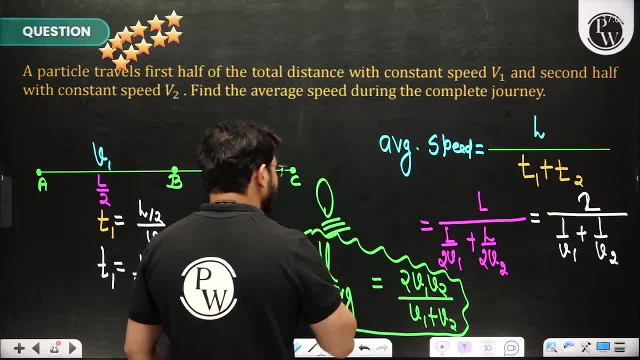 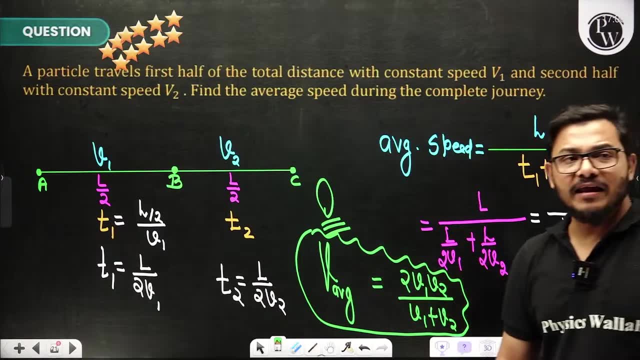 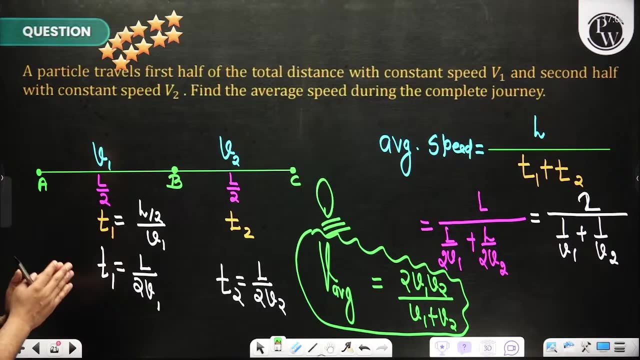 the average speed. So for every question you can find out the formula. So how many students understood this? Please tell me quickly. Did you clear this question? What is the value of the average speed? Did you understand about the value of the average speed? 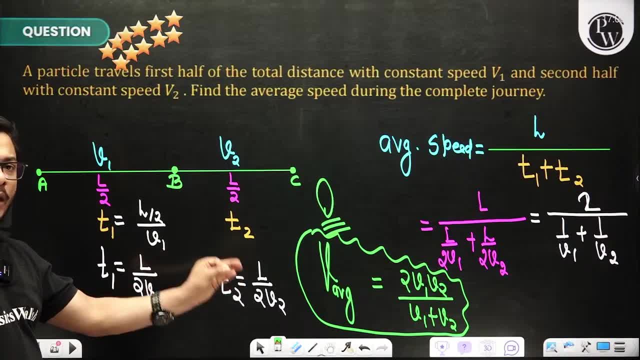 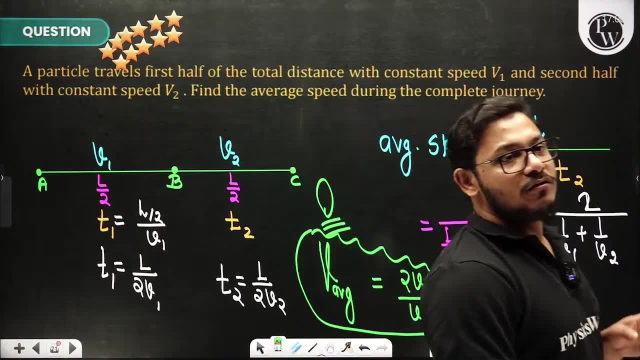 Average speed becomes equal to the two time of V1 into V2, and upon me the V1 plus of V2.. Did you understand, Is it clear? Whenever I solve a numerical question, the formula disappears. Why? Because people don't solve. 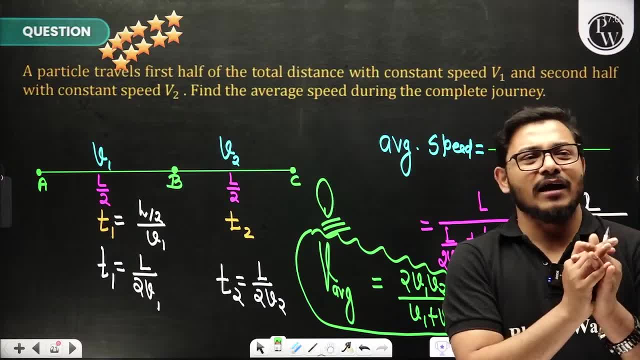 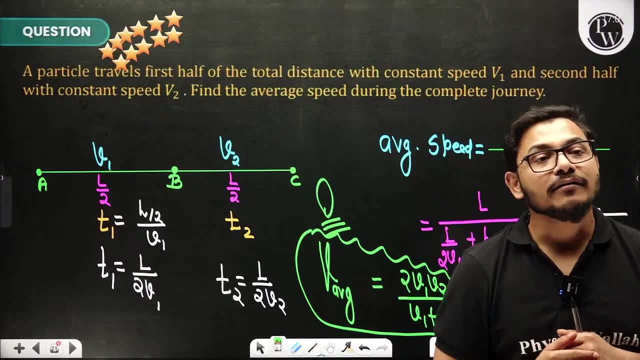 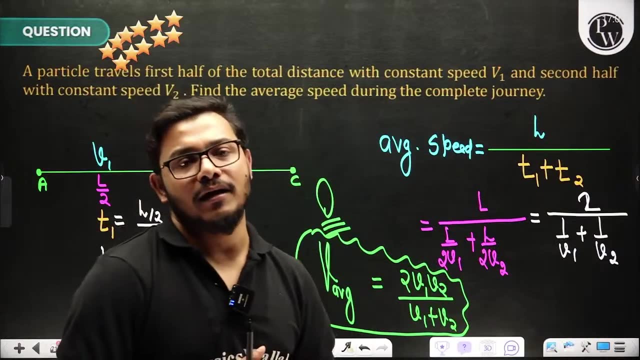 numerical questions. If you keep studying the theory, then it will remain the same. When I solve a numerical question, then it disappears. Brother, it is also important to solve a numerical question. Question is asked in the exam. How will it work? 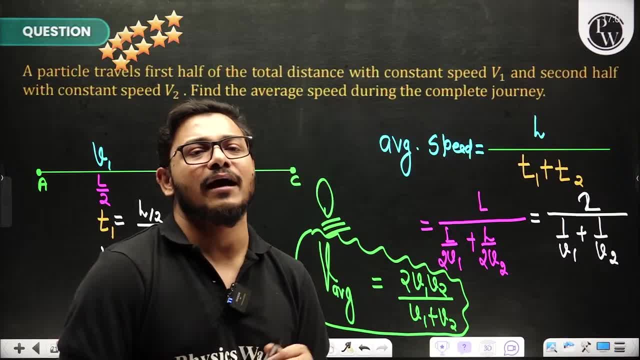 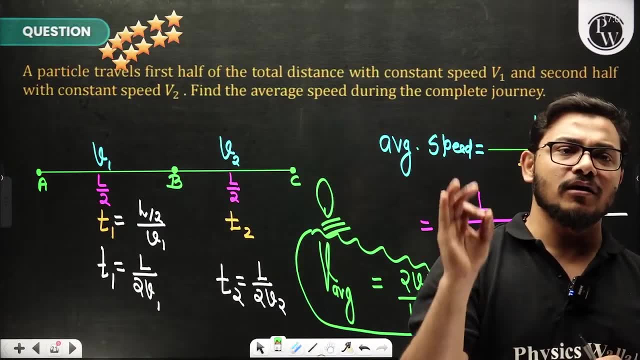 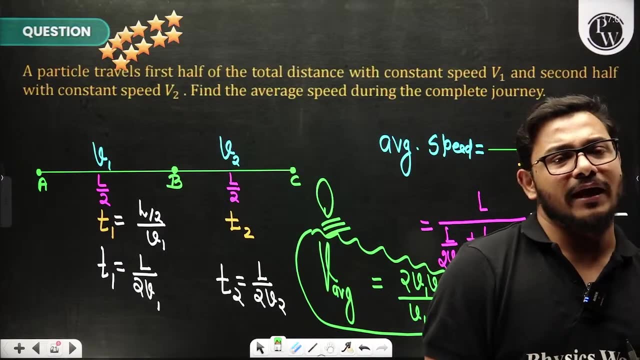 Brother, it is also important to solve a numerical question. If you don't solve a numerical question, then how will it work? Just understand one thing: Average speed becomes equal to. Why do you have to remember? This is a question. Question can be anything. 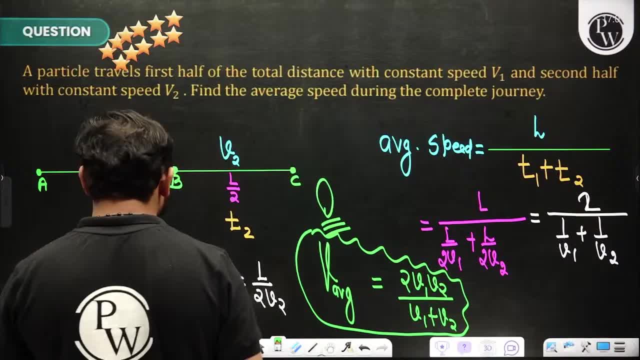 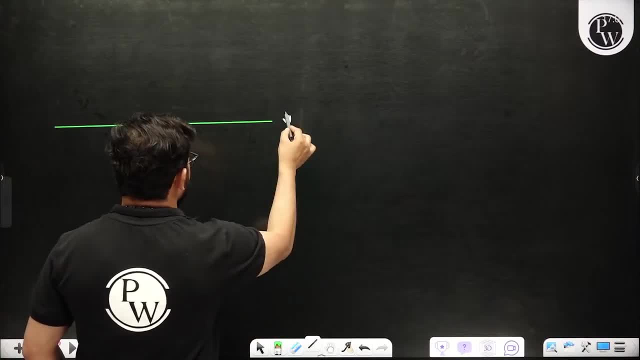 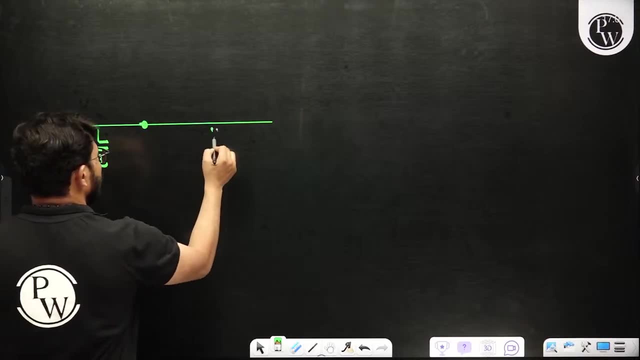 Question can be anything. Question means: whatever you say, You will tell the answer of the question. Solve it. I am changing the question. Calculate the average speed. Total length of 1 by 3rd portion and remaining 2 by 3rd portion. 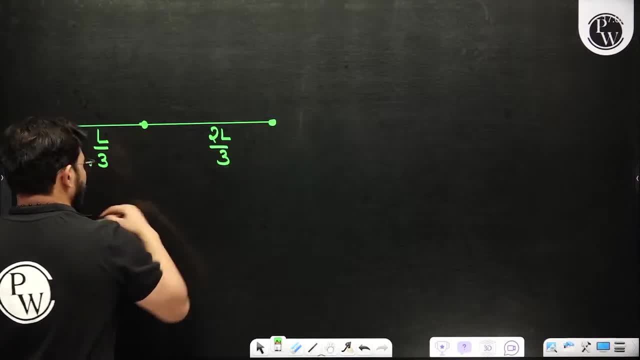 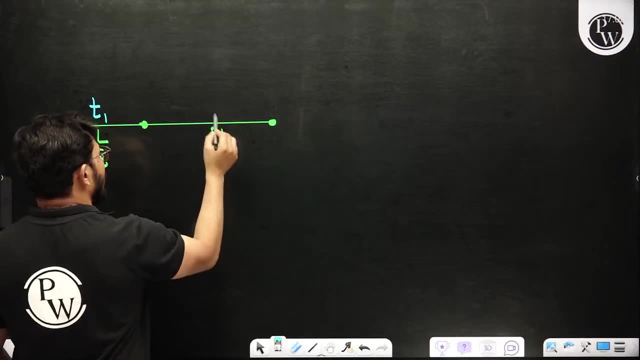 Keep listening. Total length of 1 by 3rd portion is equal to t1 and 12 by 3rd portion is equal to t2.. Here, t1 and t2 are given. What is given to you? t1 and t2 are given. 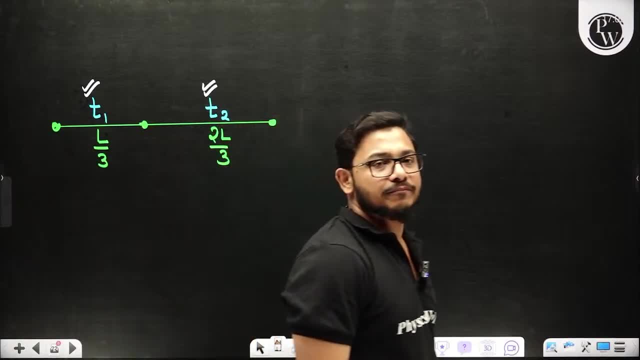 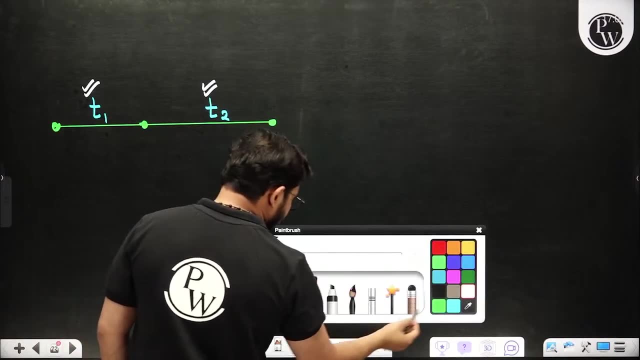 Tell me the average speed. What is the average speed? Sorry, I didn't have to do this. I had to do this. Please listen for one minute. Please listen for one minute For one distance. you moved some portion in t1. 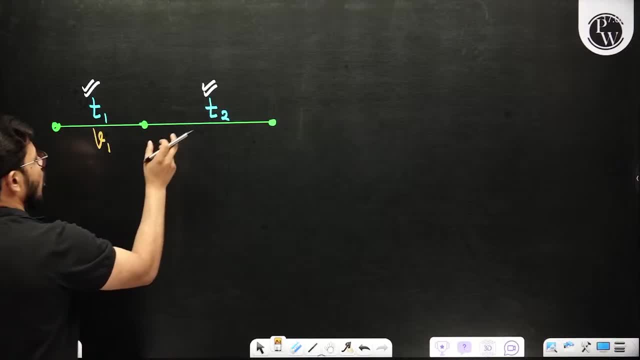 and moved some portion in t1 with a velocity of v1 and moved some portion in t2 with a velocity of v2.. Suppose this. There will be some distance. Do this Now see, any data can be anything. Now tell me what you do. 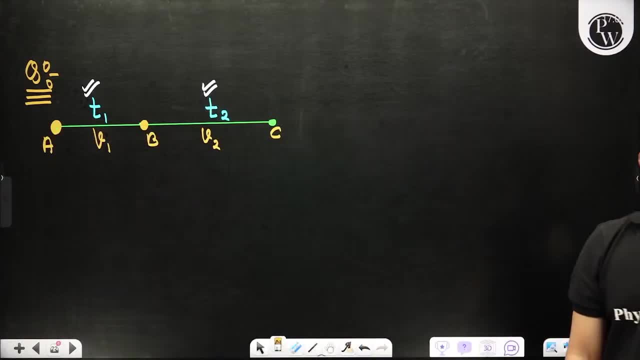 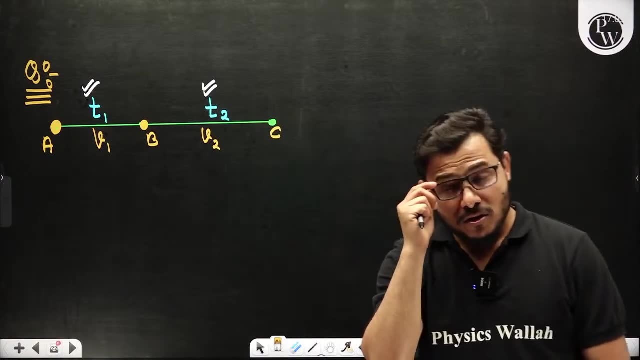 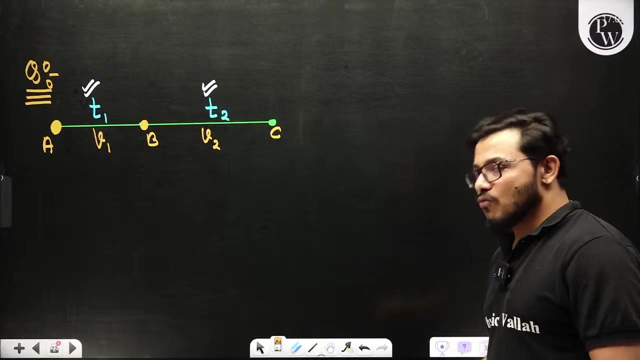 How will you solve it? Tell me quickly, What have you been told in this question? You are being told to move ab with a velocity of v1 for t1.. Then he is saying that you move bc with a velocity of v2 and for t2.. 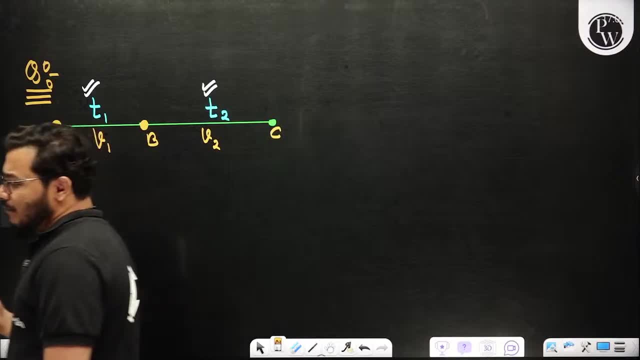 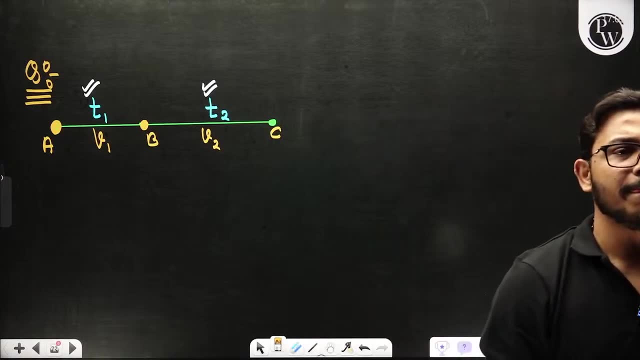 So he is asking you in the question that: how much velocity, how much is the average speed here? So tell me what will be the answer. All the students quickly type the message. Solve this question again. What am I saying, Dear Business Guru? 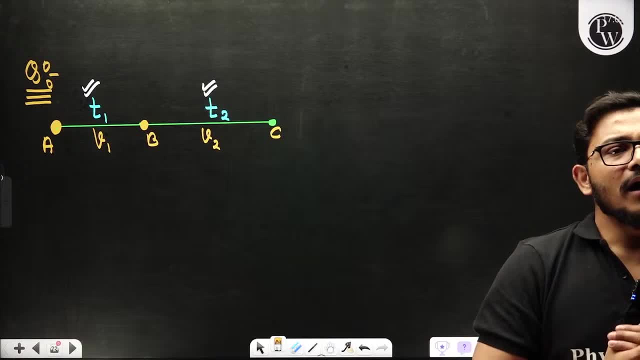 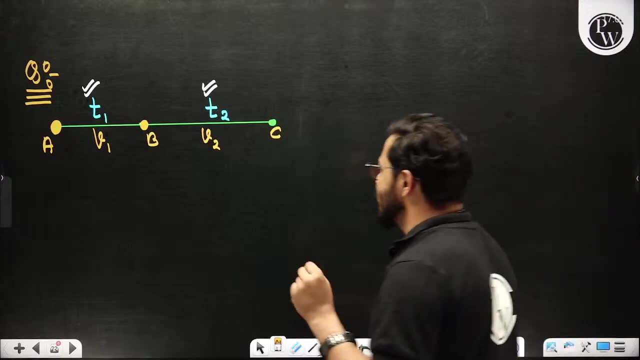 we will answer in the same way as we did earlier. You will solve this question. What is the formula of average speed? Chandra Prakash Sharma Ji? Chandra Prakash Sharma Ji, tell me what is the average speed, Say total distance. 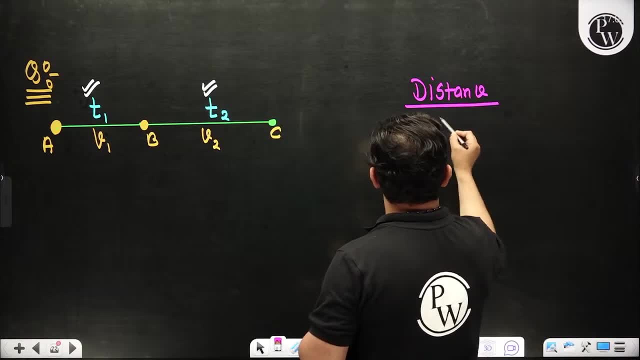 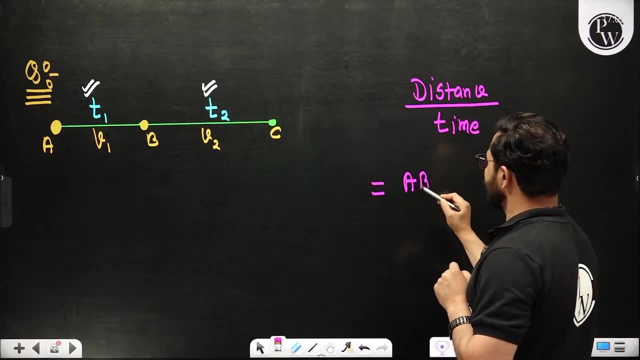 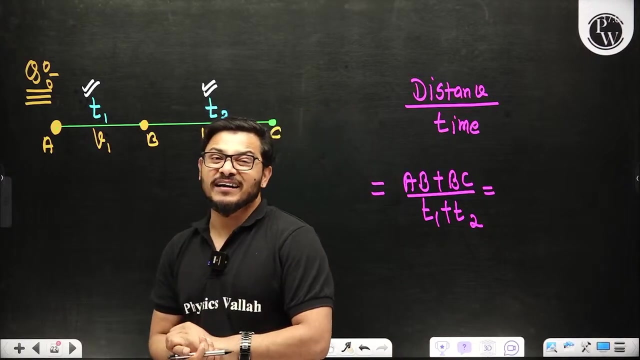 Total distance upon total time. This is what happens. Very good, ab plus bc, and what is the total time? t1 plus d2? You do not know ab. You do not know ab. How will we calculate ab? How to find out the value of ab? 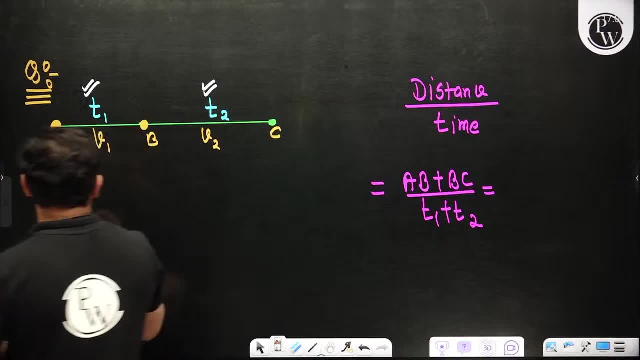 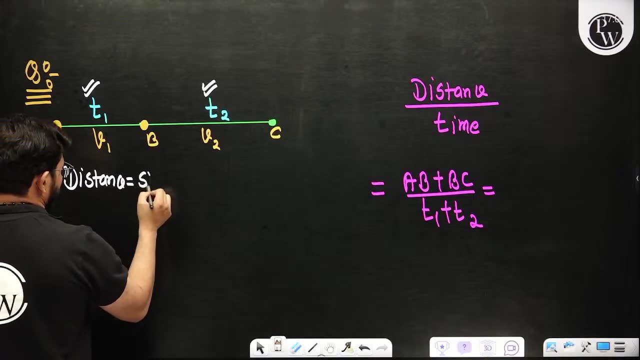 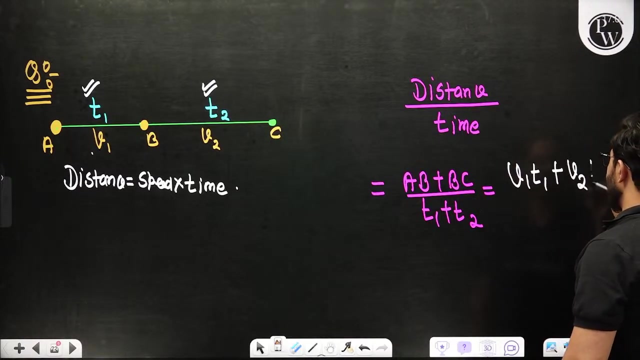 How to calculate ab. Tell me what is ab. What is the distance? Speed into time? Speed into time Ab is equal to v1 into t1.. What is ab v1 into t1 and how much is bc v2 into t2? 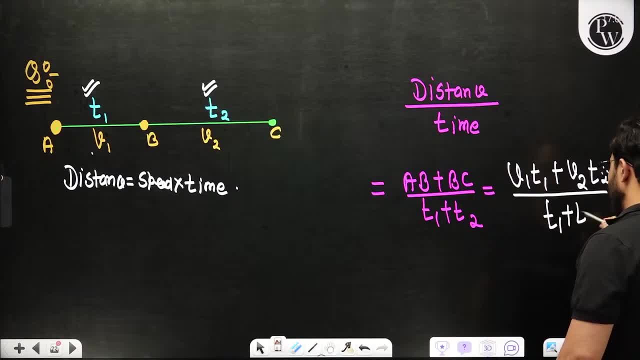 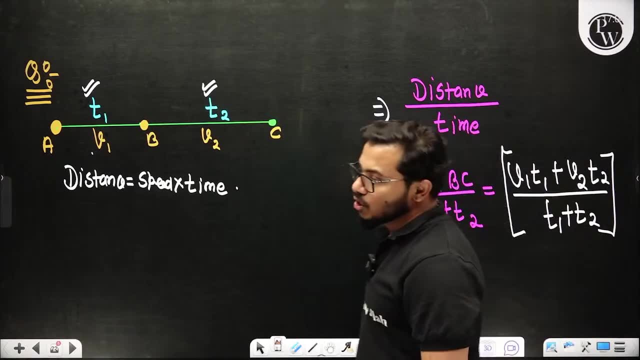 upon total time t1 plus of t2. This one is called average speed. The answer is here. This was the answer of average speed. The question is finished. You can write anything in the question. Please do not think what is given to you in the data. 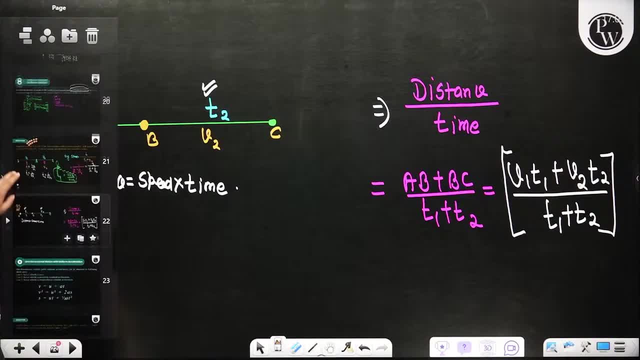 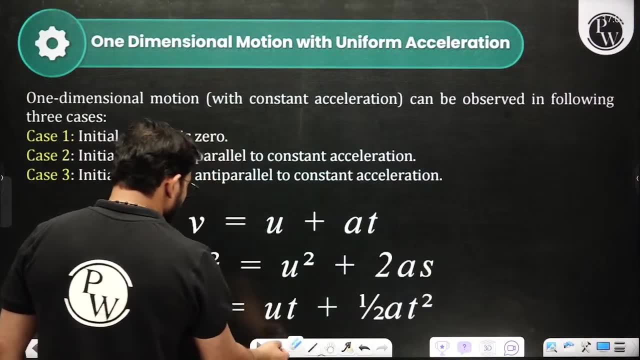 That one is called average speed. That one is called average speed. What is this called Average speed? Now I am talking about the next point. Please listen carefully for one minute. Now I am going to talk to you about Newton's equation of motion. 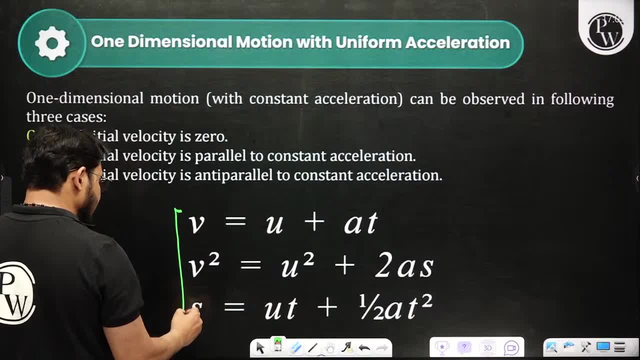 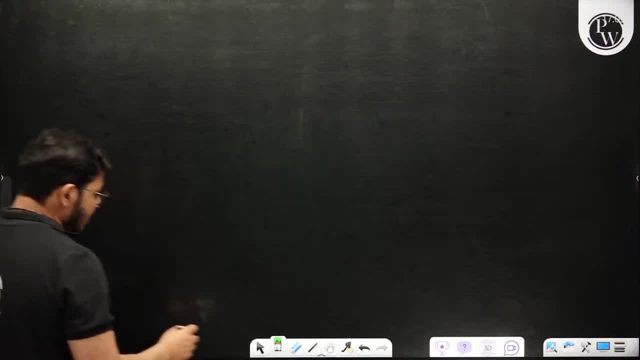 So Newton's equation of motion is three. Now, how are these three equations written? Listen carefully for one minute. I am telling you that you had explained me some things. First thing, you had told me that the value of velocity is ds upon dt. 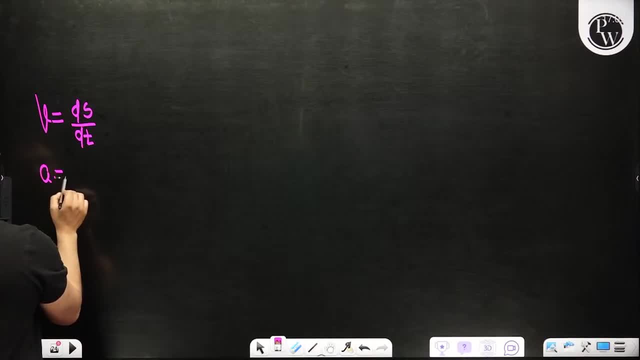 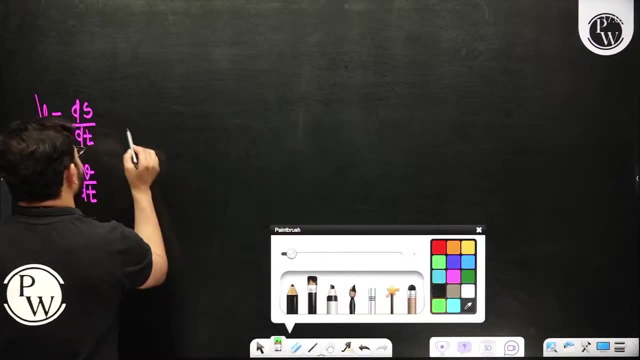 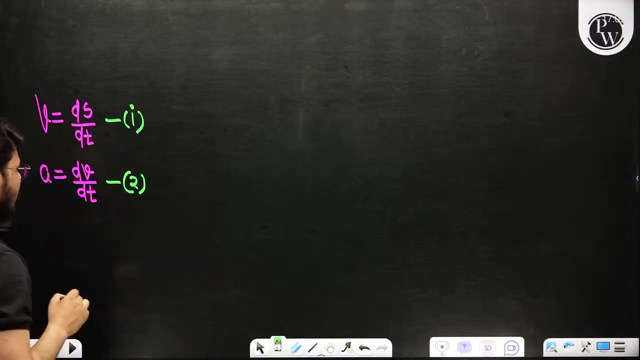 Rate change of displacement and the value of acceleration is the rate change of velocity, dv upon dt. Let's assume this is equation number one for me. This is equation number two for me. Now let me listen carefully for one minute. Let's assume that you have 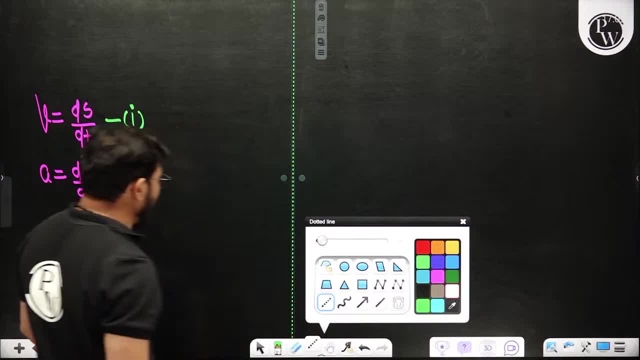 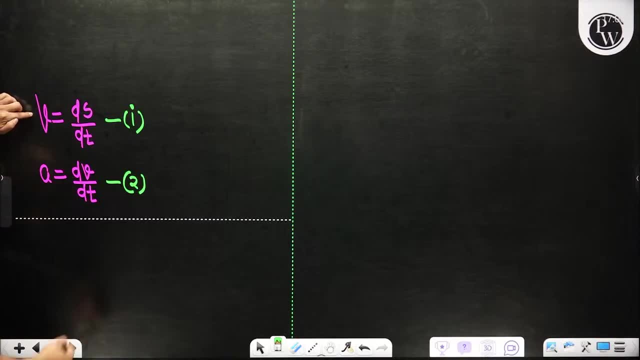 some numerical question given to you and in that numerical question if you have, in that numerical question, if you have velocity, displacement and time, then you will apply equation number one. If you have velocity, acceleration and time, then you will apply equation number two. If you have velocity, 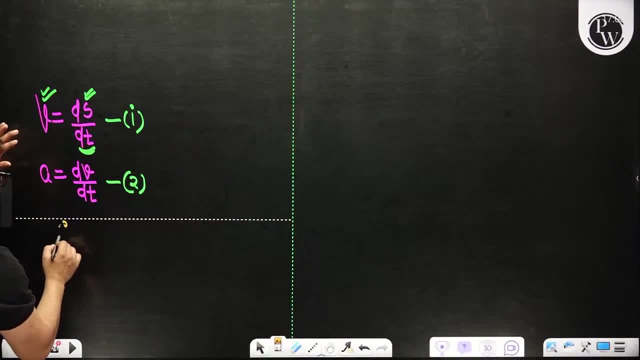 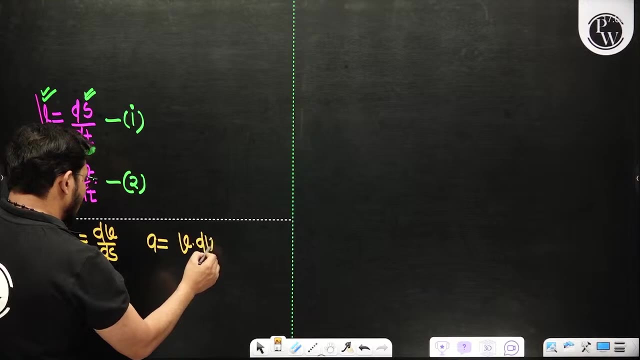 and time, then you will divide these two equations, So a upon v becomes equal to dv upon ds. By doing this, what happened is dt to dt is cut, so a becomes equal to v into dv upon ds. This value came to you: dv upon ds. 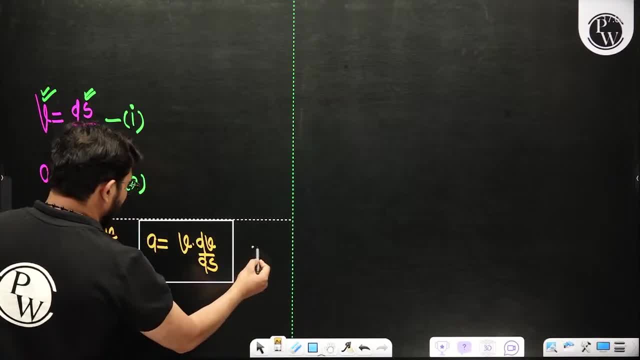 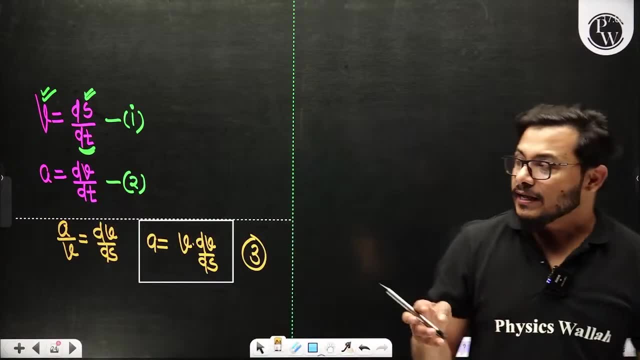 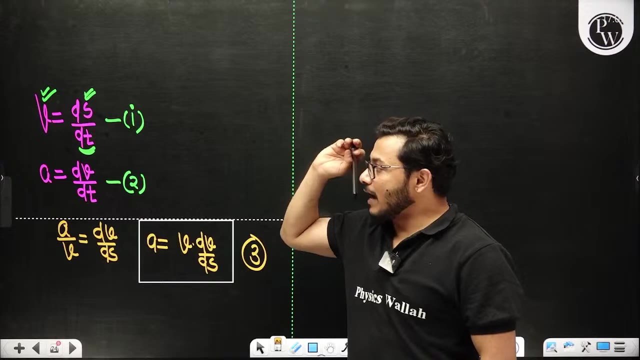 So you must be understanding what I have written. This is equation number third. So you have written three equations here. The first equation: you have written that velocity becomes equal to rate change of displacement ds upon dt. Then you have told me what is the acceleration. 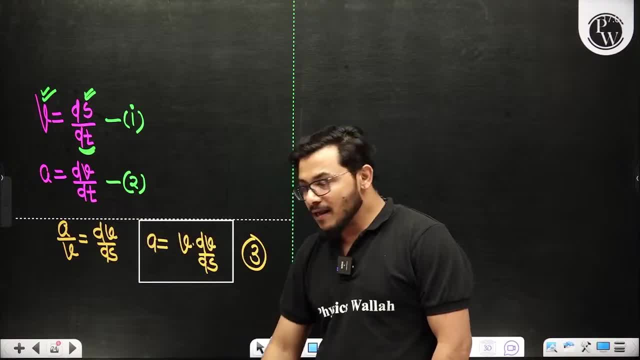 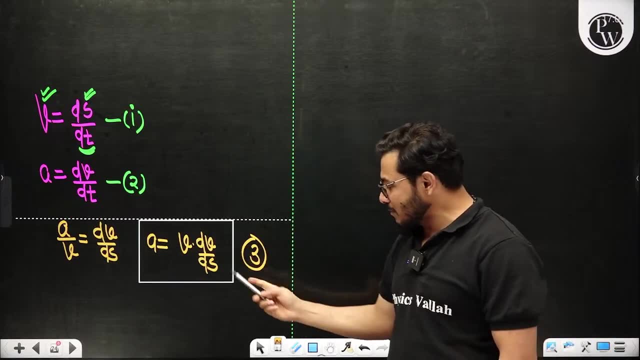 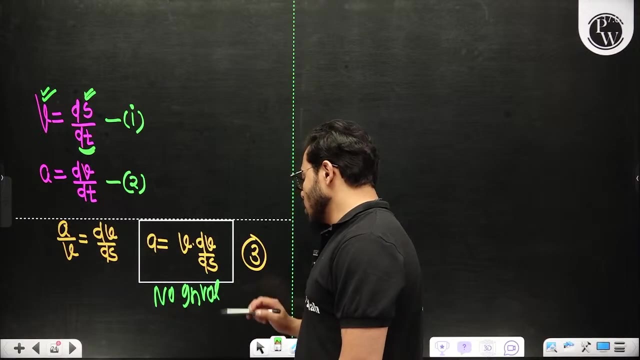 Acceleration becomes equal to rate change of velocity. Then you have told me that acceleration becomes equal to v into dv upon ds. This is the equation in which time is not involved. No involvement, No involvement, No involvement of time. There is no involvement of time here. 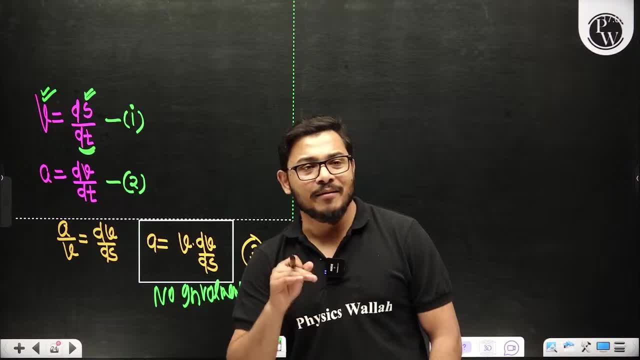 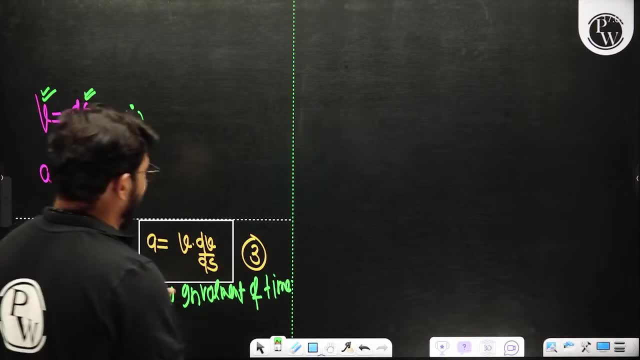 There is no involvement of time here. So if there is no time in any numerical question, then you will apply this equation. Very good, Now I will go a little further. I have to go a little further in this way. Now, suppose if someone talks to you about a special case. 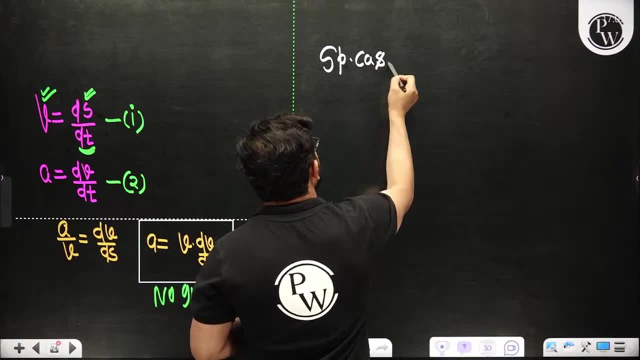 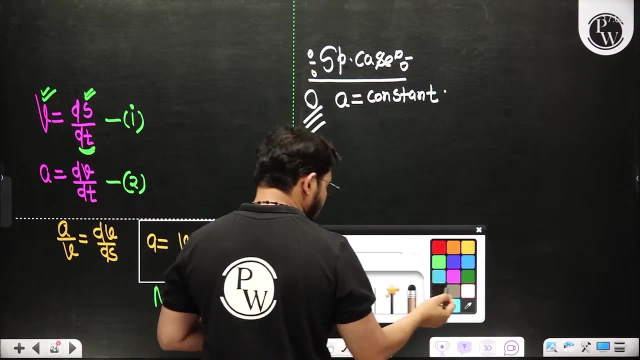 Special case And tell you that you have to solve this differential equation. And someone is telling you that if the magnitude of acceleration is constant, What are you saying? Absolutely right, If the magnitude of acceleration becomes constant, then what are you seeing here? 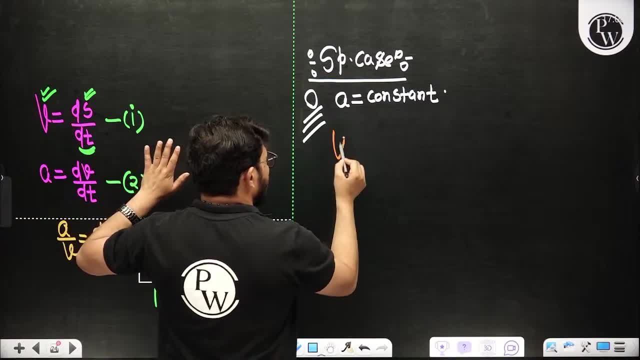 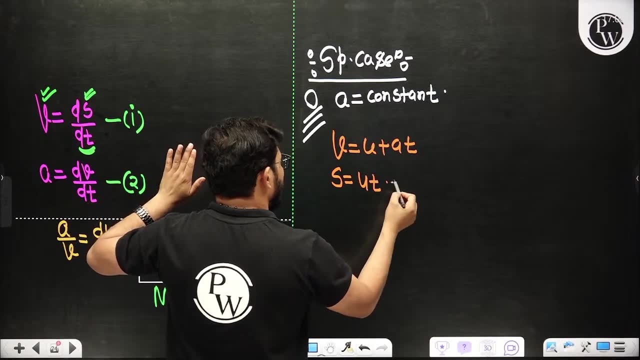 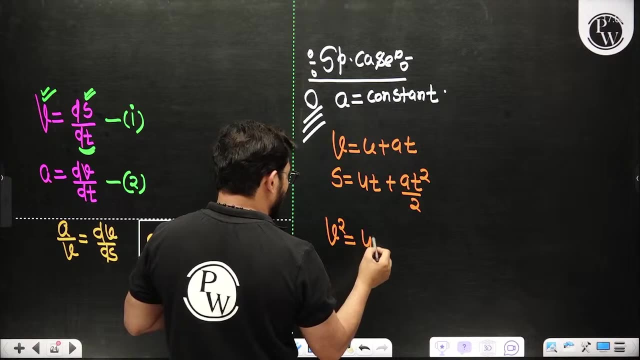 If the magnitude of acceleration is constant, then what will this equation become? v becomes equal to the u plus of at, and s becomes equal to the ut and plus of at square by 2.. And the third equation: you know how it comes. After terminating the time. 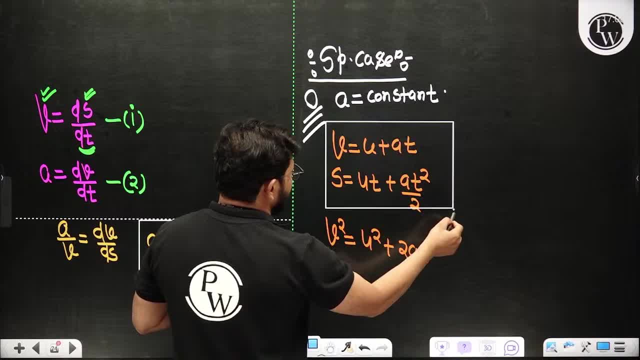 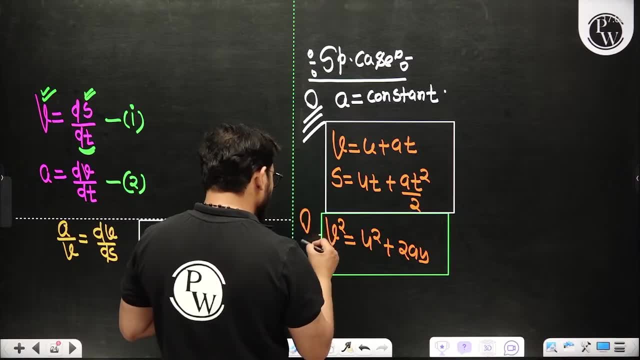 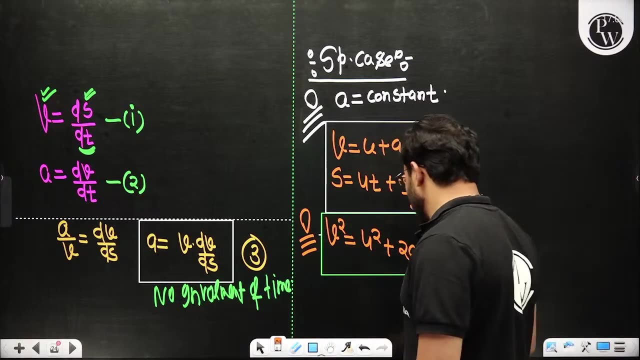 v, square u, square plus of the 2 ay. So here you have written three equations of motion. First you have written two and then you have written the third equation. And please remember, these three equations you call Newton's equation of motion, You call them: 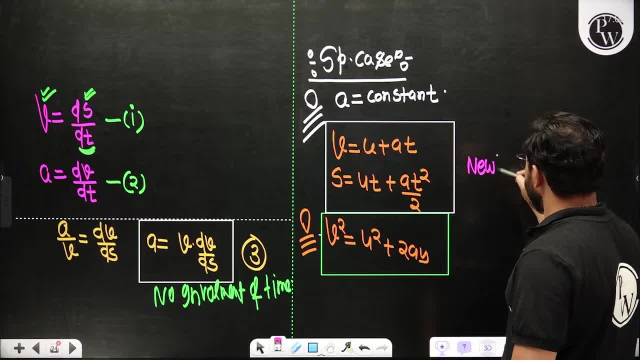 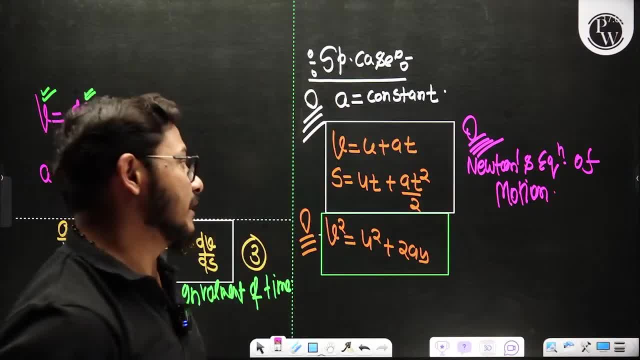 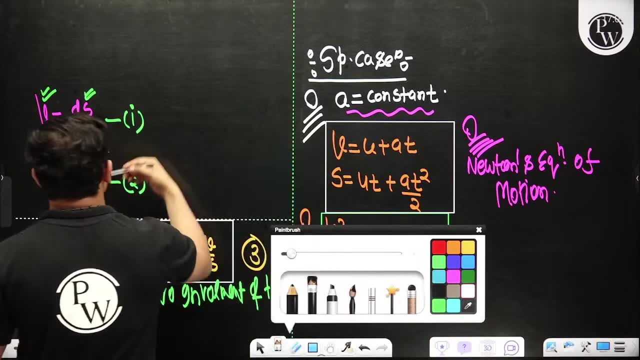 This is called Newton's equation of motion. This is called Newton's equation of motion. And when these three equations are valid, When the magnitude of acceleration is constant And when these three equations are valid In any case, In any case, In any case. 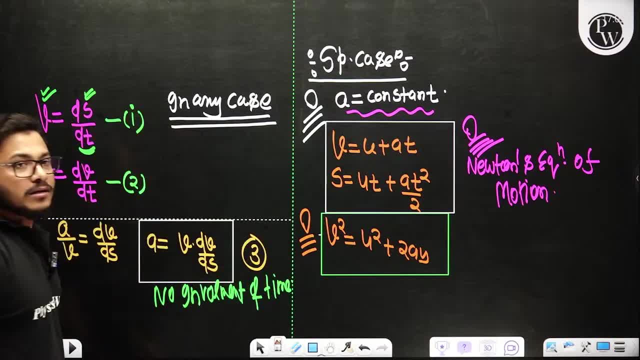 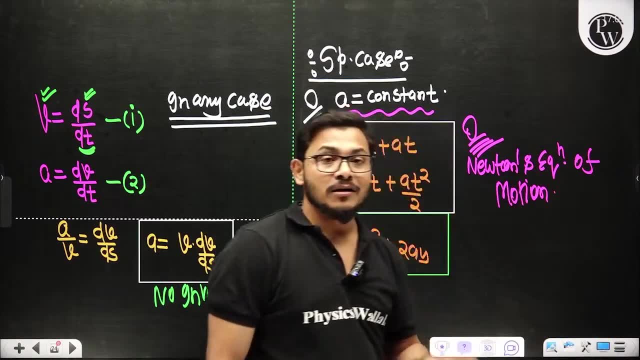 Whether the magnitude of acceleration is constant or not. I don't care about that. This is valid in any case. And when these three equations are valid, When you have Newton's equation of motion, When the magnitude of acceleration is constant. When the magnitude of acceleration is constant. 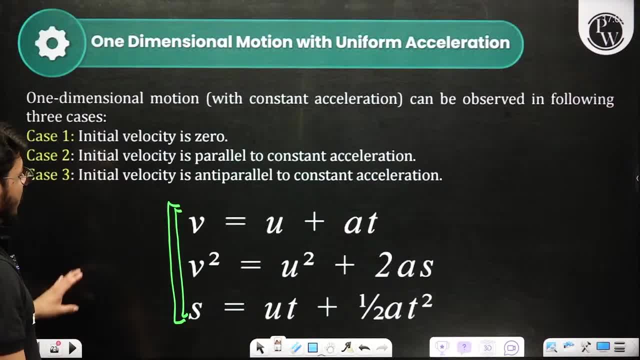 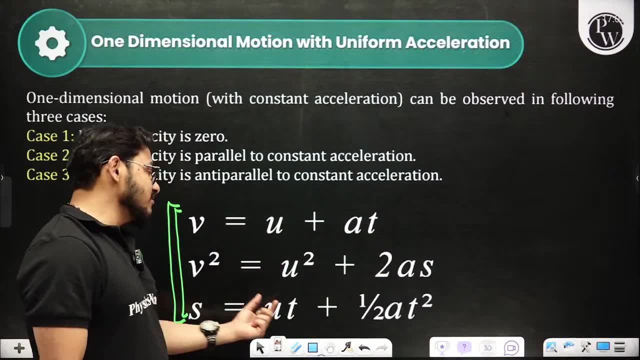 When the magnitude of acceleration is constant. So please, let's see here once. See, I have written and shown. v becomes equal to u plus of 80 v. square becomes equal to u square plus of 2 ay. s becomes equal to ut plus of half at square. 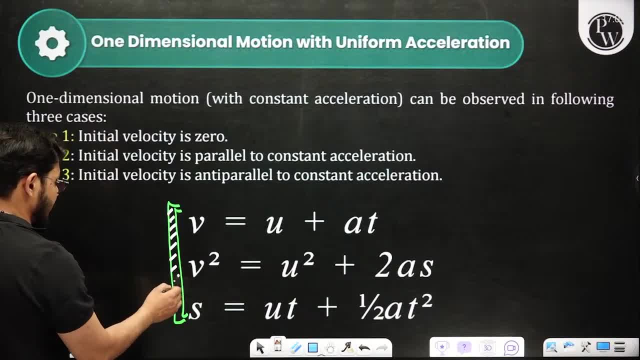 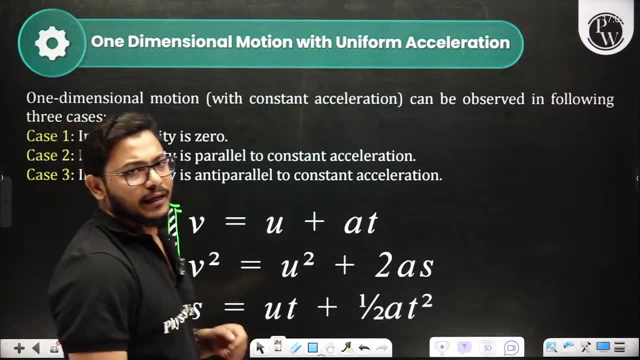 s becomes equal to ut plus of half at square. That only the one idea, please, written and shown. So I hope you understood the things And see when you solve such questions. then, while solving such questions, you, Sir, tell me the relation. 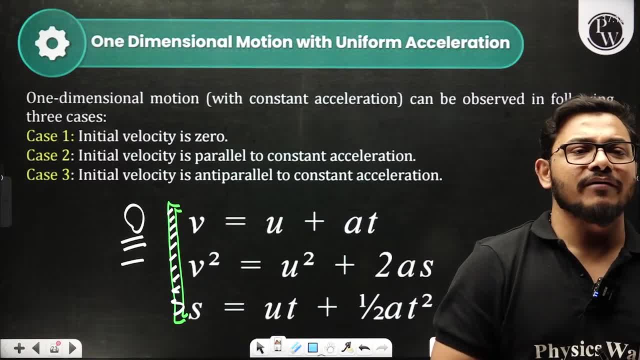 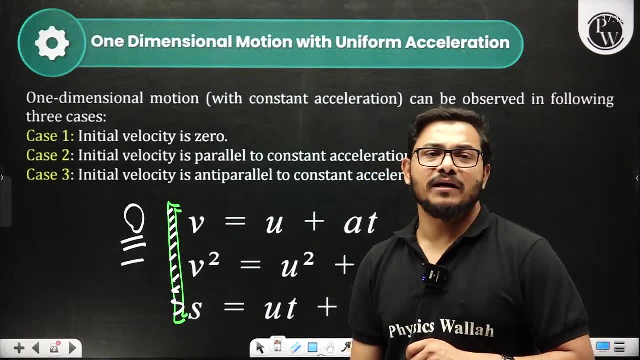 V of the first equation and speed and time of all three. Sir, tell me the relation V of the first equation and speed and time of all three. Sir, tell me the relation V of the first equation. Yes, so now listen to me. 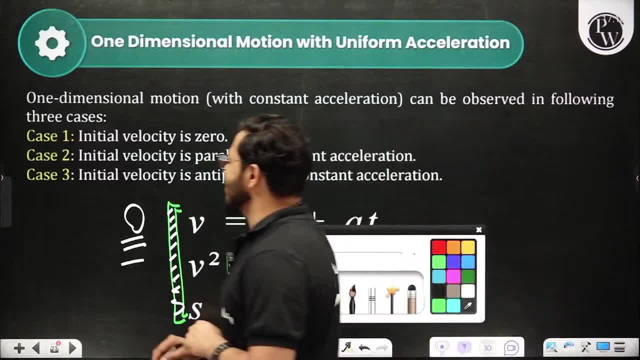 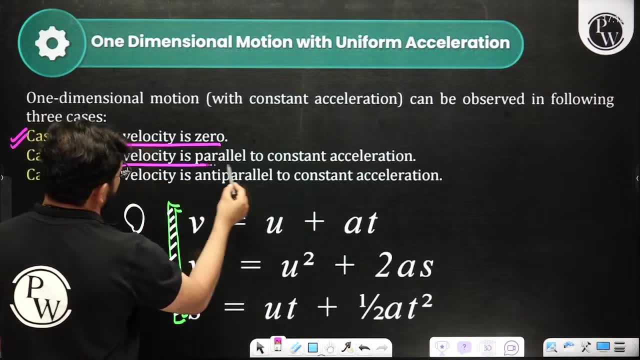 Here there are three cases. Here there are three cases. What is the first case? What is the first case? That either the initial velocity becomes zero for you, or the initial velocity is parallel to the constant acceleration for you, or the initial velocity. 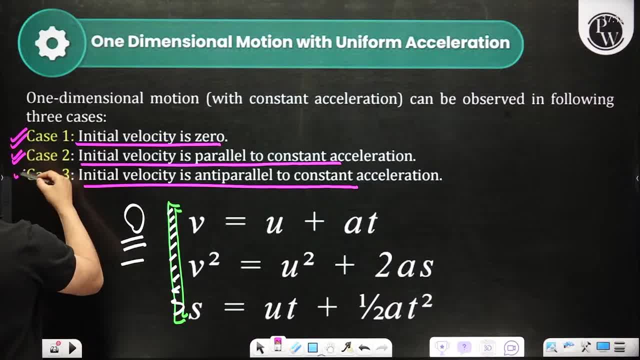 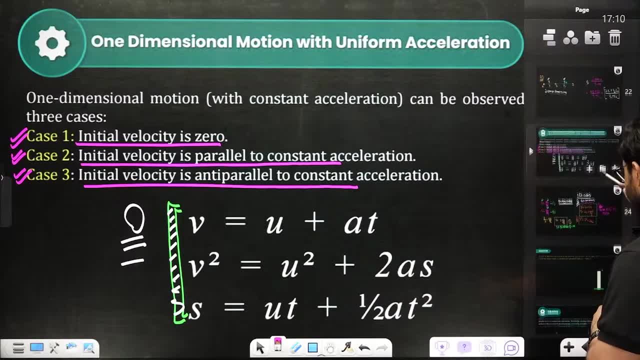 is anti-parallel to the constant acceleration. for you, There are three cases, And when I mean this is how the story goes. You are understanding what I am trying to say. So now I am here, Newton's equation of motion. I mean, if I ask you, 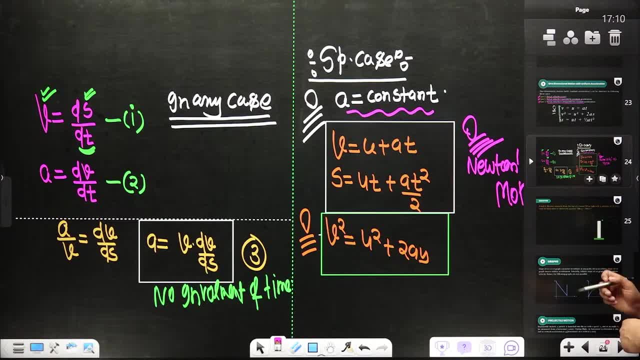 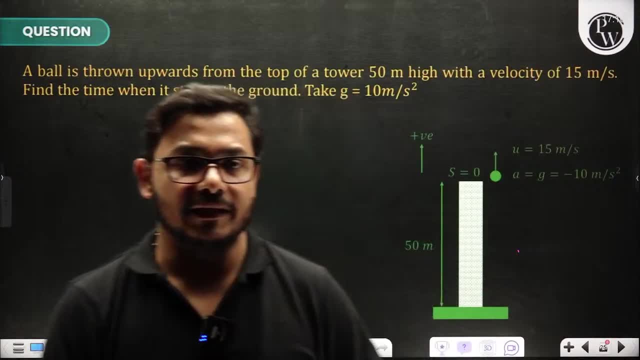 a question, then it is very intense. There will be ten questions And please see the question. What is it? Let's see a question. You will clear all the concepts. Please see the question for one minute. What is the answer to the question? 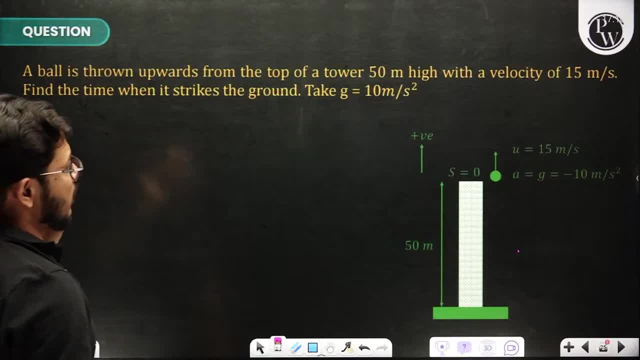 It says that you have thrown a ball from 15 meters per second from a tower whose height was 50 meters. He is asking in the question that: tell me the time when this ball will hit from the ground. Listen to me a little carefully. 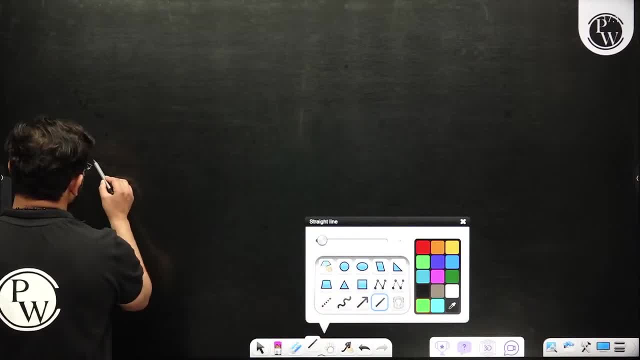 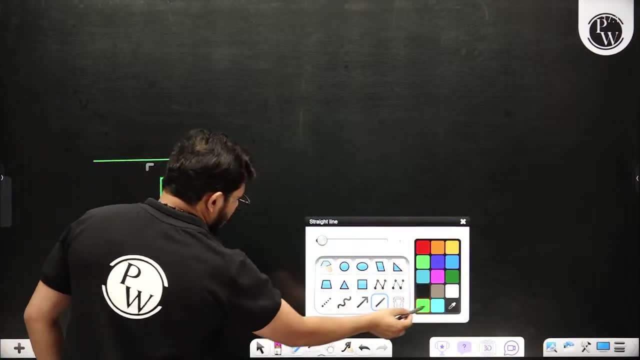 What am I saying? You have a tower, You had a tower. Please listen to me for one minute. You had a tower, You have a tower, And this is the ground for me. This is the ground for me. What is this? 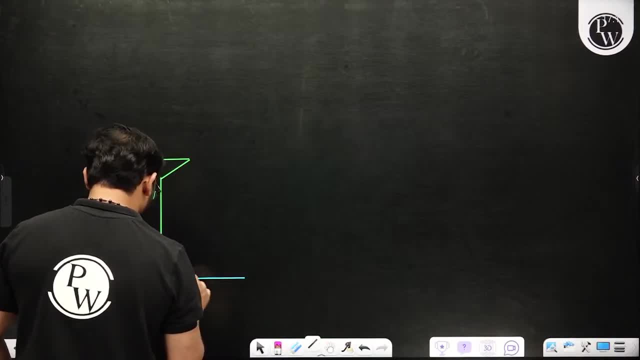 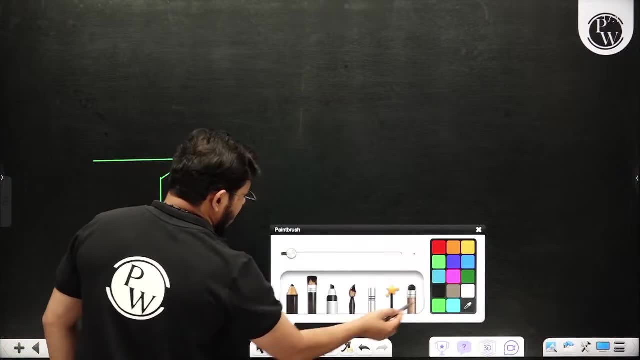 This is the ground for me. What are you doing here? Listen to me a little carefully. You are a ground for me. What are you doing here? Let's understand that for a moment. You took a ball here. You took a ball here. 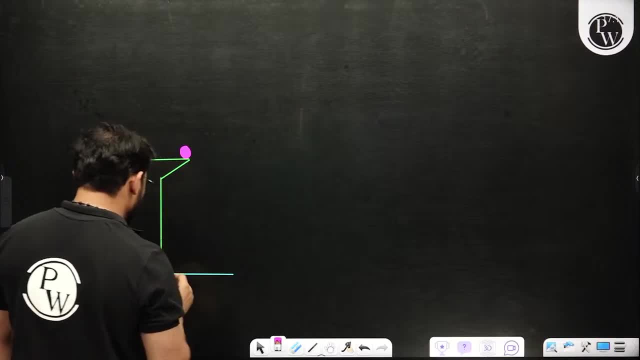 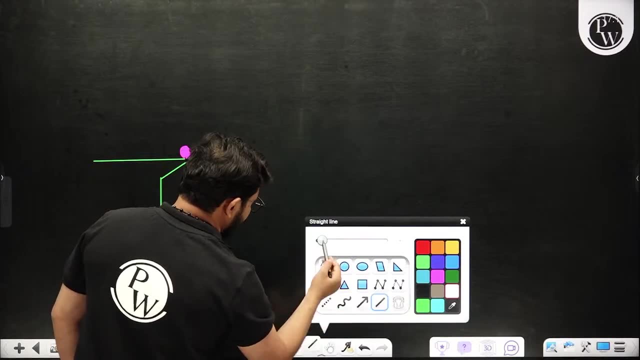 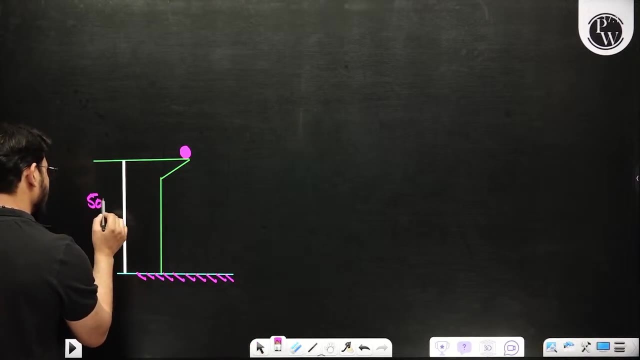 Here is a ball. OK, please keep listening. You took a ball here And I am here. I am looking from here and the total height of this tower is 50 meters. Please listen carefully. the height is 50 meters. What did you do? You threw this ball upwards from here. 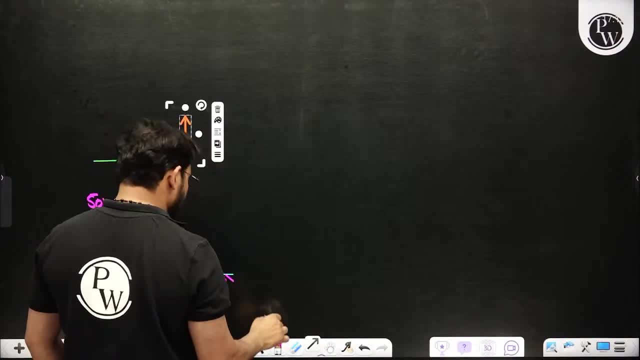 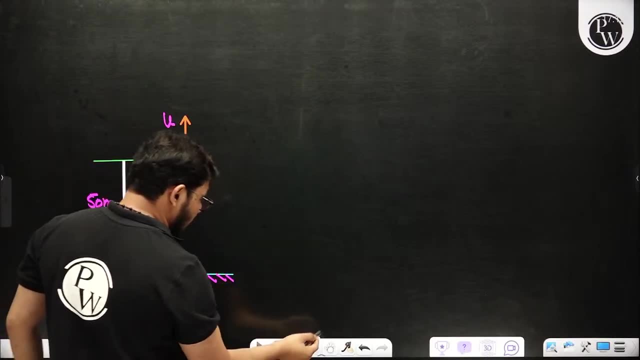 You threw the ball upwards. When you threw the ball upwards, let's assume that you had original velocity U. When the ball is going upwards, then the velocity will decrease slowly, Because gravity acceleration is always going downwards, So the ball is going upwards. 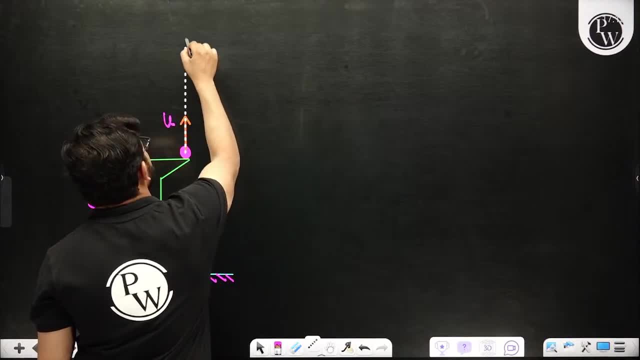 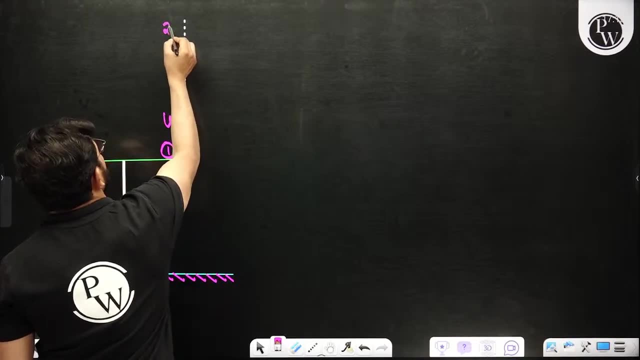 Let's move the ball upwards. The ball is going upwards. Assume that you have reached here. Let's assume that this position number is 1.. And this position number is 2 for you. And after going to position number 2,, what is the final velocity of the ball? 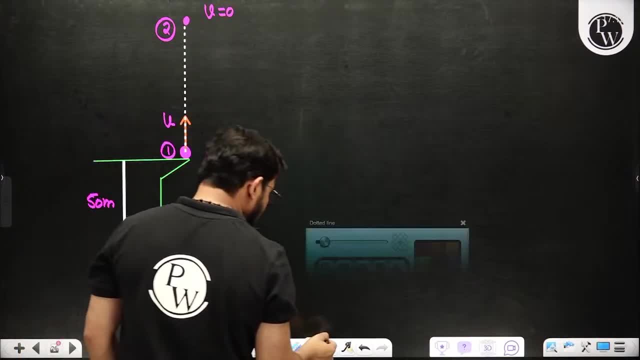 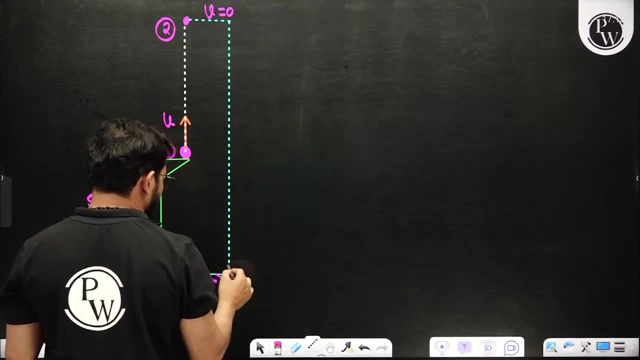 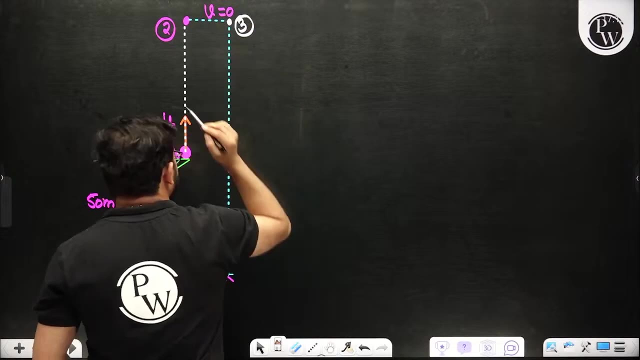 It became zero. After the final velocity is zero, this particle is coming down from here to here. Let's assume that this position is yours. Here the position number is 2, but I write it here. Assume that this position number is 3.. 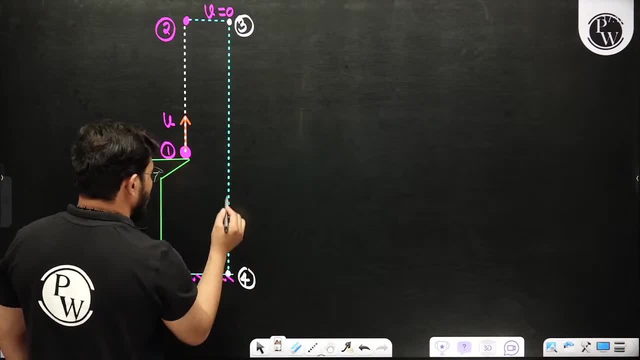 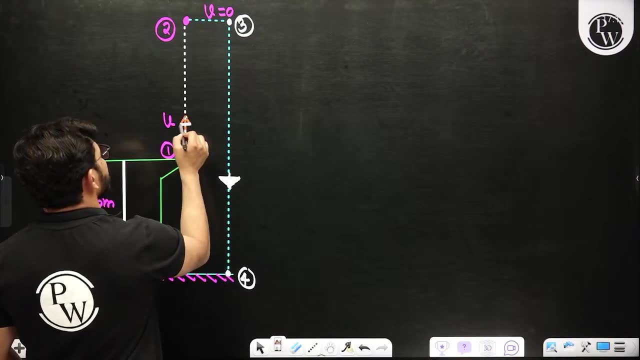 Now this position number is 4 for you, This position number is 4.. And I made it like this. So did you understand what I told you? Like this, So you can see this story like this. So let's do one thing. 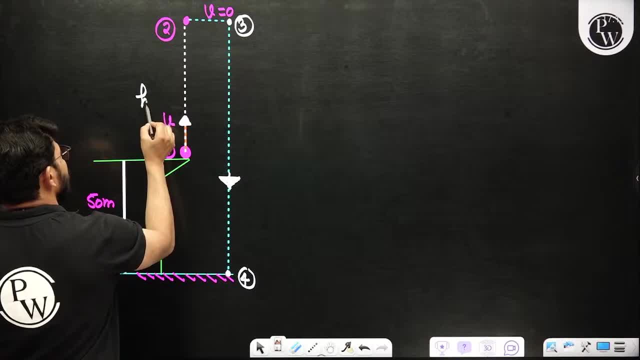 When you go from 1 to 2, what is the height- Assume that it is h- And when you go from 1 to 2, what is the time you took? It took t1.. How much time did it take? 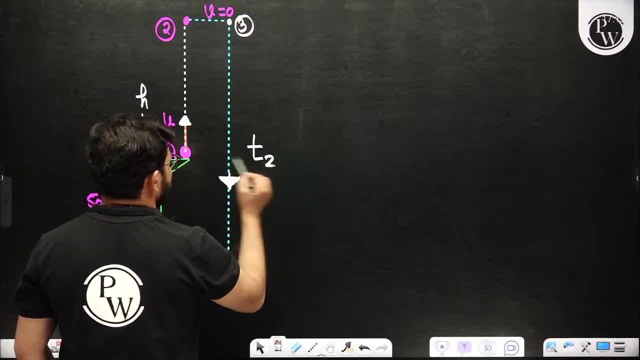 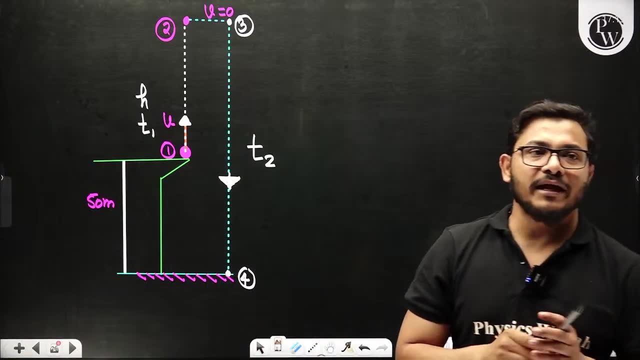 And when you go from 3 to 4, what is the time you took? Assume that you took t2.. I am asking you, tell me how much is the total time? Total time, What will be the meaning of total time? 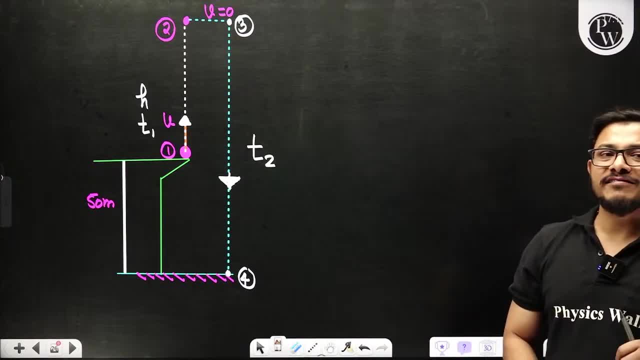 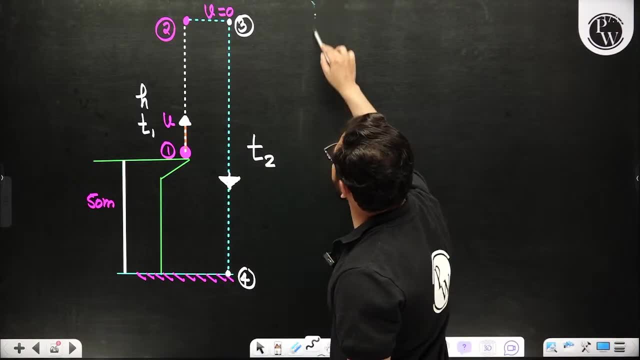 How to find out the value of the total time. Will any child tell you how to calculate the total time? The meaning of total time is t1 plus of t2.. Now how will you calculate this total time? Do one thing When you solve the numerical question. 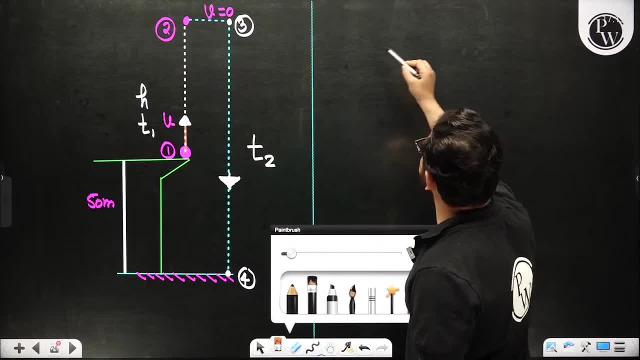 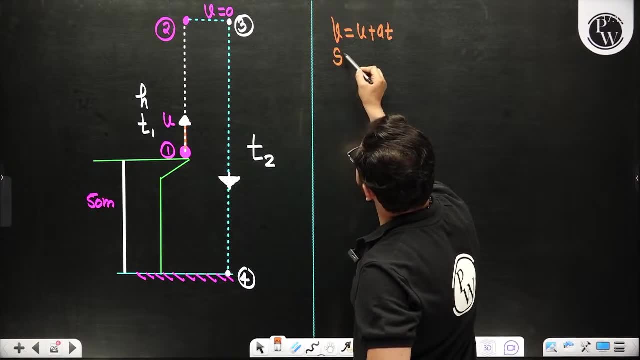 then, first of all, write Newton's three equations of motion. Write it somewhere on the side. What was the first equation v become is equal to u plus of at. And what was the second one s become is equal to and ut plus of at square by 2.. 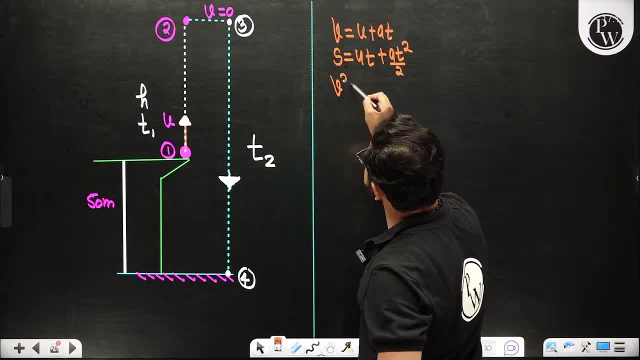 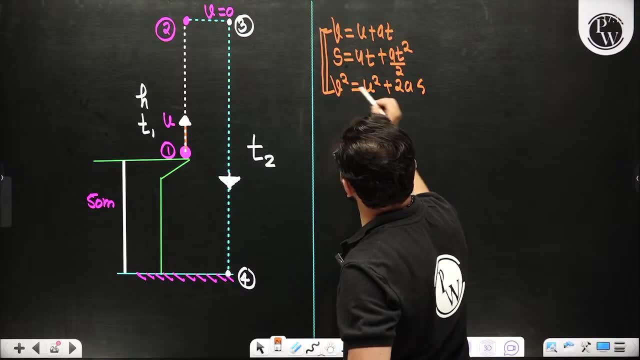 And what was the third equation? The v square become is equal to the u square, n plus k2. as These are Newton's three equations of motion, Never forget these three in your life, Please. just one minute Now. let's do one thing. 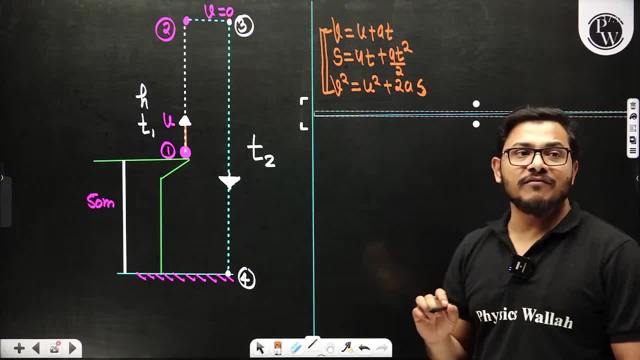 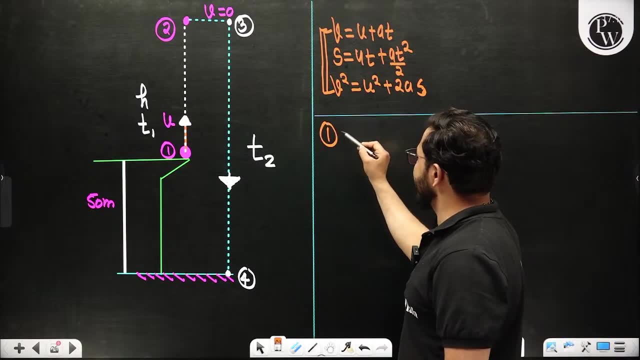 Now you apply Newton's equation of motion from the first position, from 1 to 2.. The public will tell me what I am saying. First of all, let's apply from 1 to 2.. From where? From 1.. 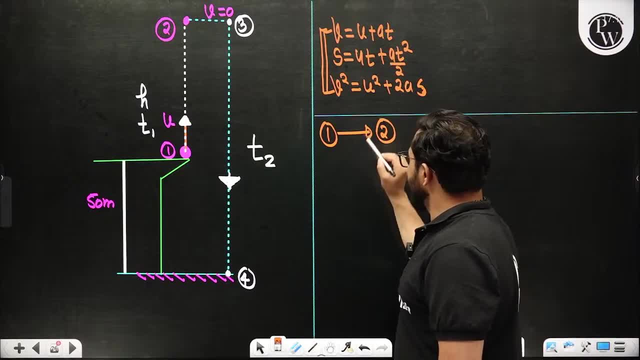 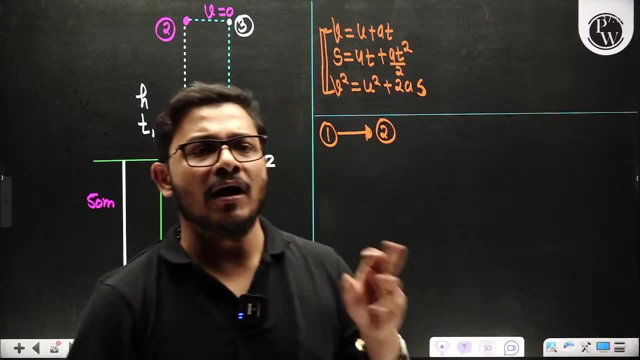 And to where? To 2.. From 1 to 2.. So 1 is my original position. Please listen to that point, All children. tell me which equation you would like to apply here. Tell me quickly. I want to calculate the time. 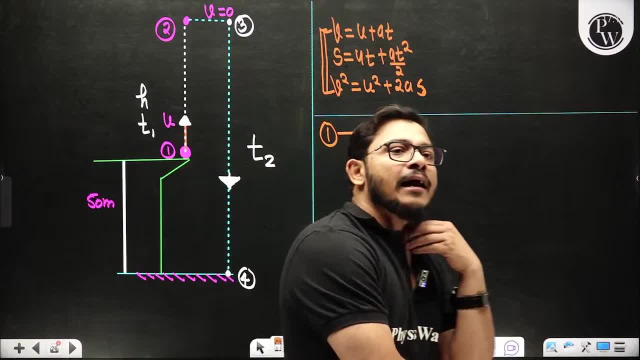 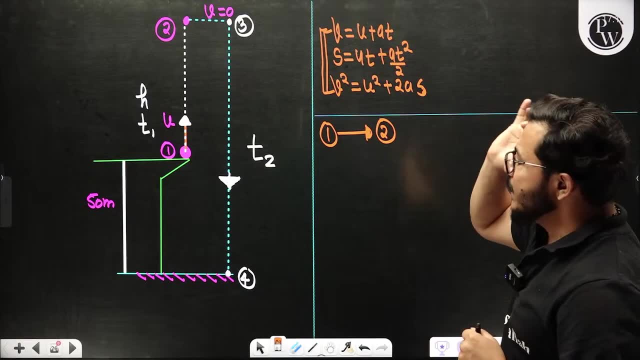 I want to calculate the time to go from 1 to 2.. Which equation would you like to apply? Tell me quickly. Type a good message. Which equation would you like to apply To go from 1 to 2,? you have to calculate the time. 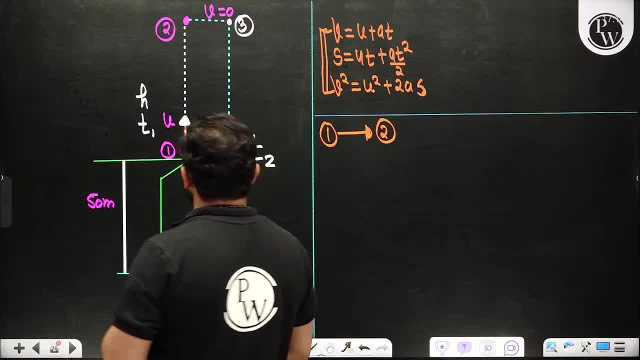 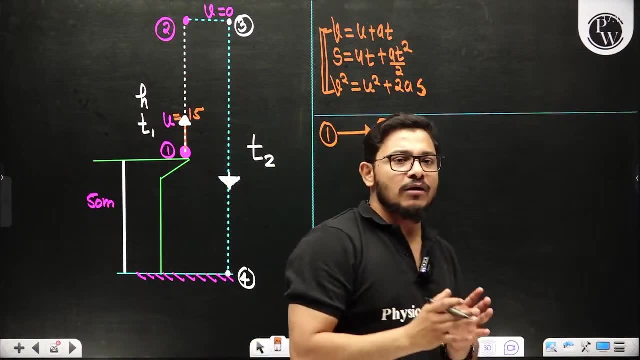 You have to calculate the time. You don't know the height, Whereas you know U. What is the value of U 15. Whereas the final velocity here has become 0. You know the velocity. You have to calculate the time. 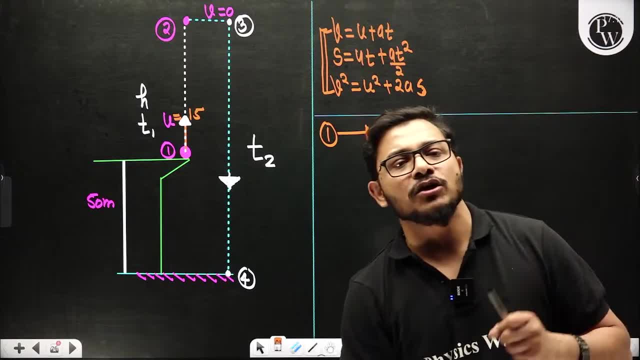 Why would you apply the second? Subham Sahoo, tell me one thing: Why would you apply the second equation? To apply the second equation you need, the value of height S becomes equal to UT. Subham, listen to me. 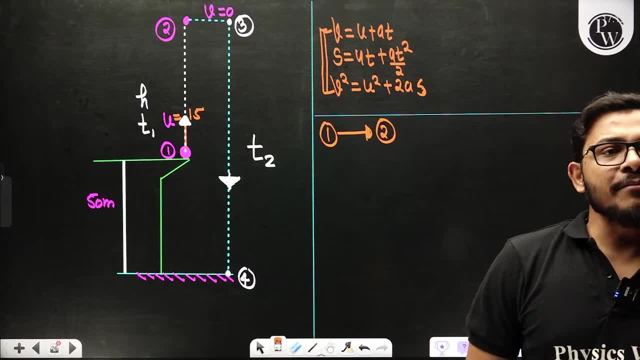 Why would you apply the second equation, Subham? please, Mr Chaudhary, listen to me. Why would you apply the second equation? You apply that equation in which you have all the data. Subham, listen to me. 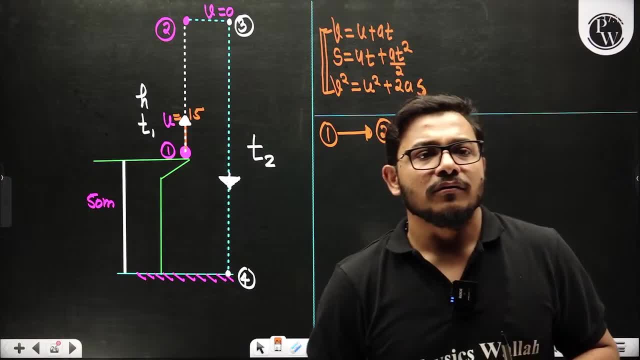 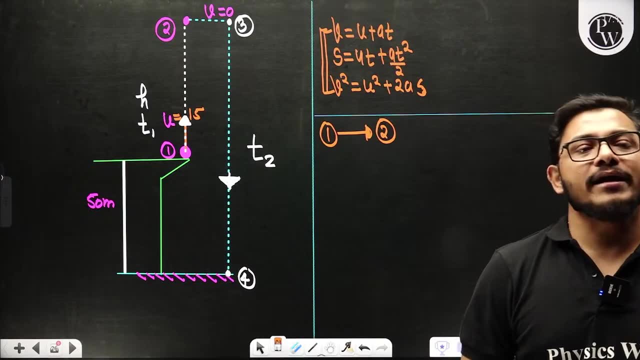 All the data is known. All the data is known. Some have come, Some have come. Which equation would you apply? Tell me quickly. We will apply the first equation Because we know the velocity and have to calculate the time, So apply the first equation. 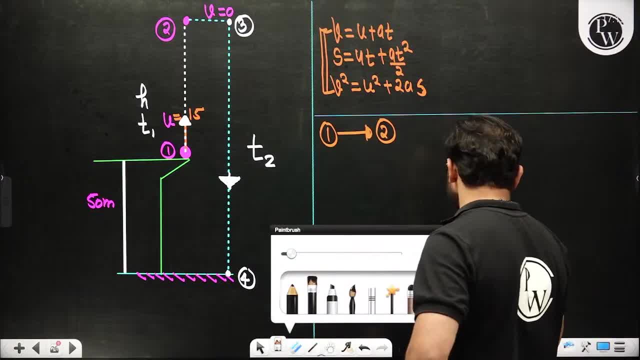 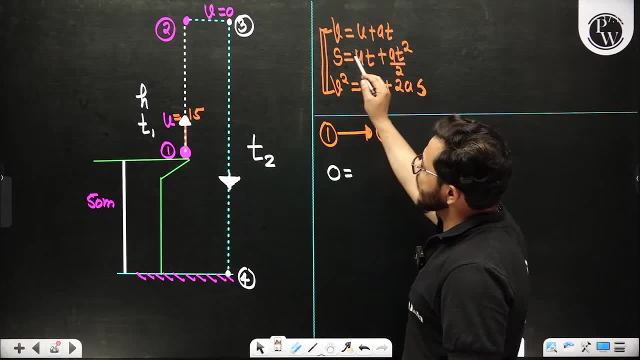 The first one. So write down the first equation: V becomes equal to UT U plus of AT. So what is the final velocity? It is 0.. The final velocity is 0.. What is U Tell me? Tell me U. 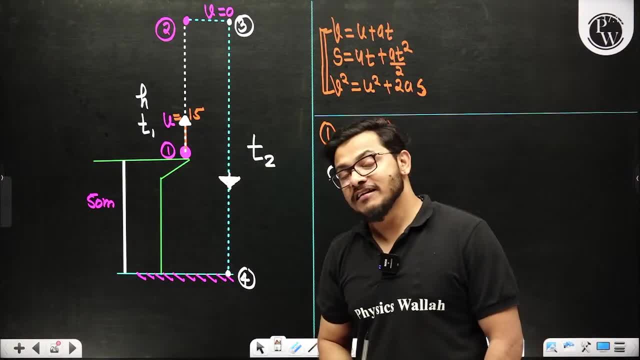 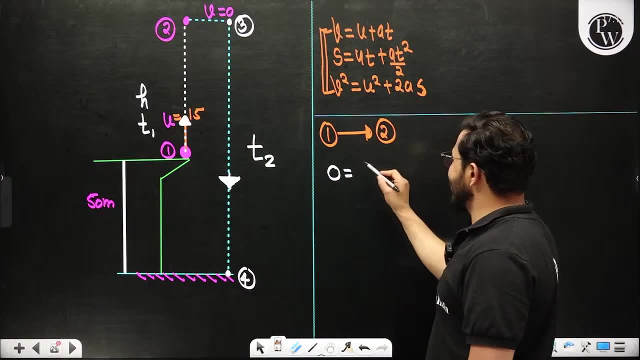 Positive or negative? Tell me quickly What is U Positive or negative? Tell me quickly. U is positive. Why is U positive? Because it is going up. It is going up, So plus 15.. Plus 15.. Plus 15.. 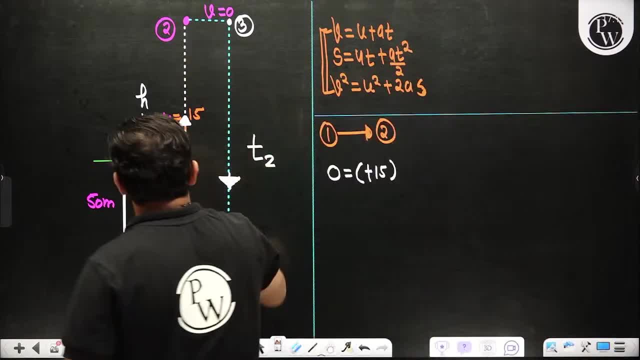 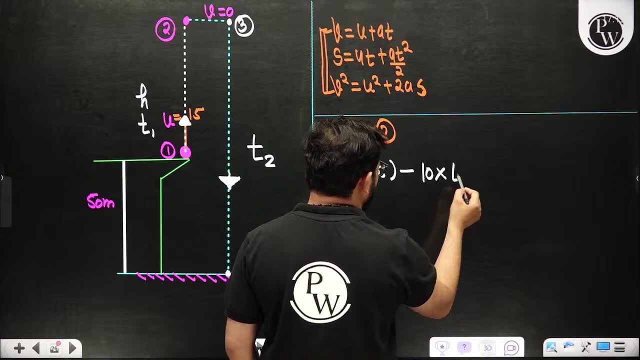 And 80. Acceleration. See, acceleration always goes down, So acceleration due to gravity will be negative. Come on, do one thing: Acceleration due to gravity: take 10. And consider into time as T1.. Listen to me. 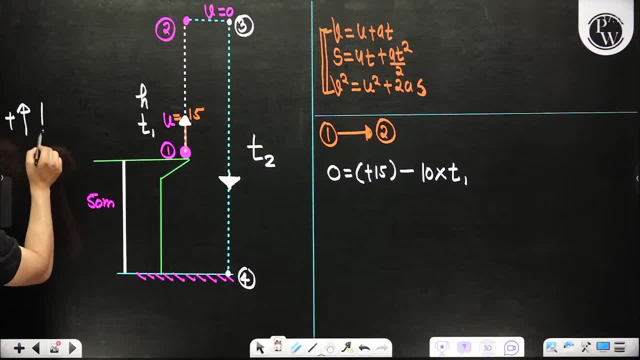 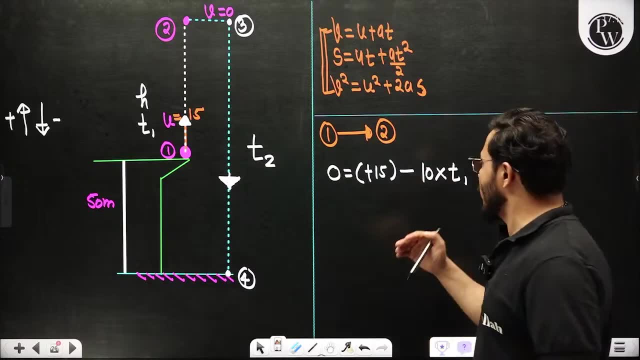 Whatever terms you take up, say it positive. Whatever you take down, say it negative. The talk is over. So why did acceleration due to gravity become negative? Because it is always going down. Solve it. So what is the value of T1?? 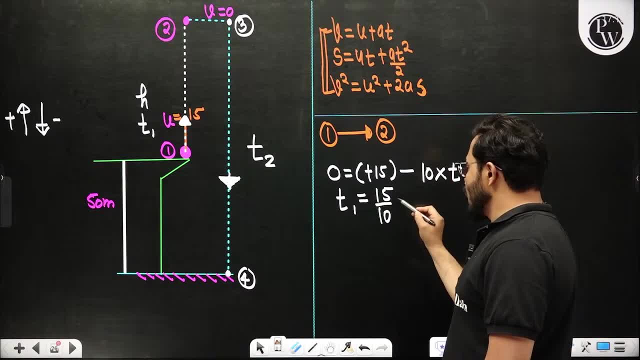 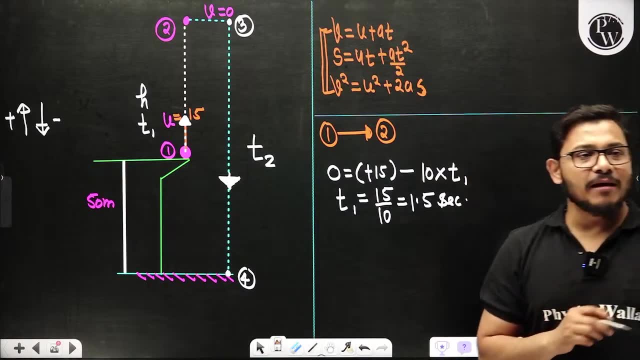 15 divided by 10.. So 15 divided by 10 means 1.5 seconds Means it took you 1.5 seconds to go from 0.1 to 2.. Now let me ask you one more thing. 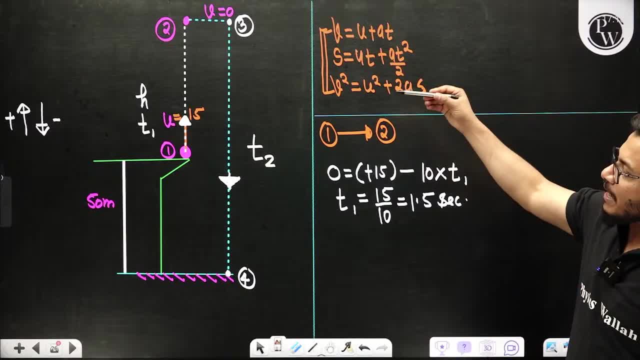 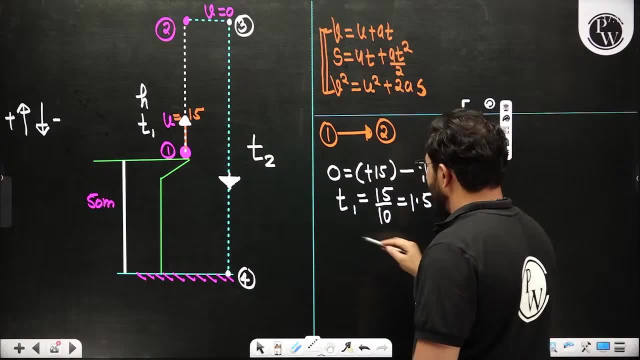 One more thing: Tell me quickly How much height did you go from 1 to 2? Height, Height, Height, Height. Tell me which equation do you like to write to calculate height To go from 1 to 2,? 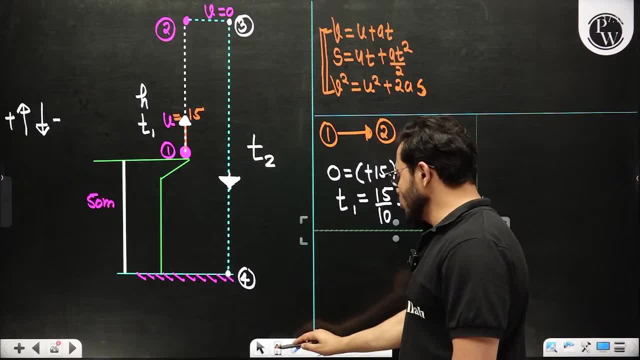 which equation do you like to write to calculate height To go from 1 to 2, now think about this: If I calculate the height directly, which equation do you like to write to calculate height to go from 1 to 2?? 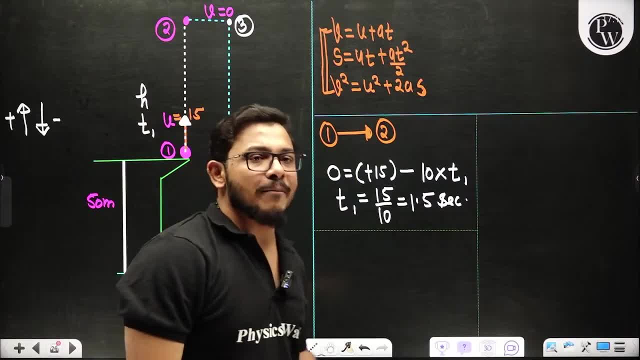 The third one. Very good, If you go from 1 to 2, you can also apply the second one. I am not saying that you can't do the second one. You can do the second one because you have calculated the time. 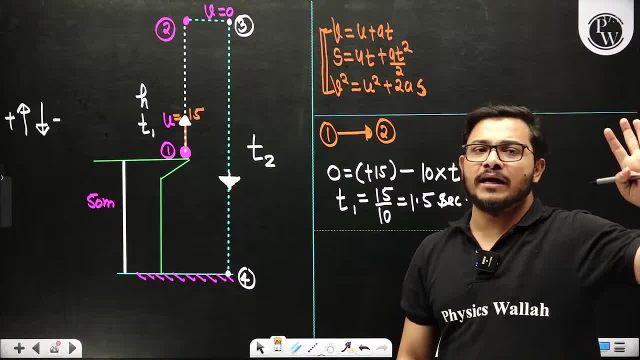 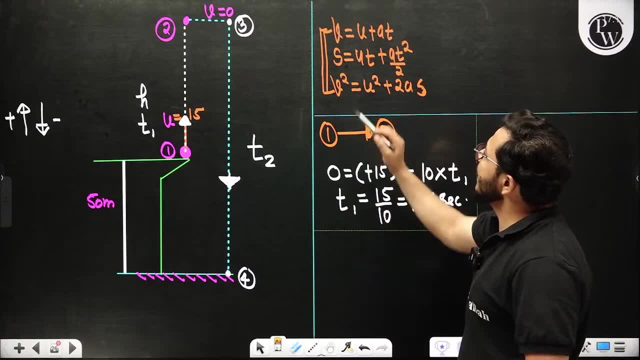 If you want to calculate the height directly- I just want to calculate the height, nothing else- Then I will apply the equation number 3.. So what is the equation number 3 for 1 to 2?? The final velocity square means 0 square becomes equal to u square. 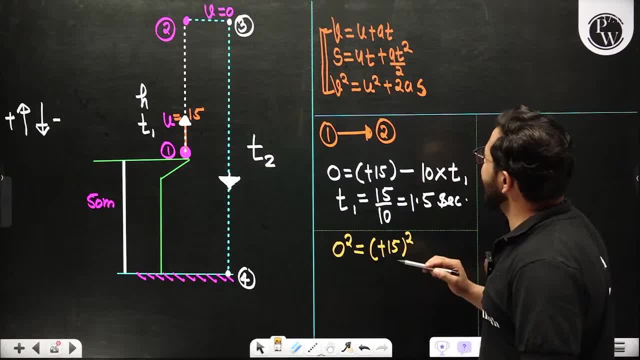 So u is 15 plus k, So 15 square. Did you understand? n plus of plus of the 2a. So the value of a is minus k 10.. And how much is the height? It is h. 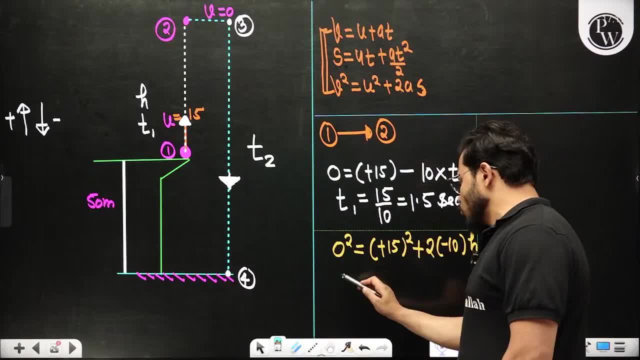 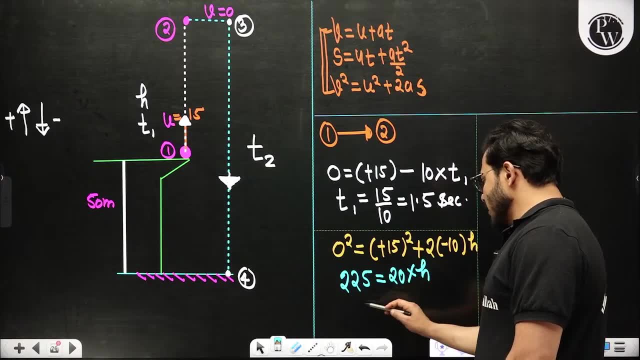 The value of a is minus k 10.. So when we did 15 square, how much did it become 225.. Didn't it become 225?? 225 becomes equal to 20 and into h. This is done When you wrote the value of h, how much did it become? 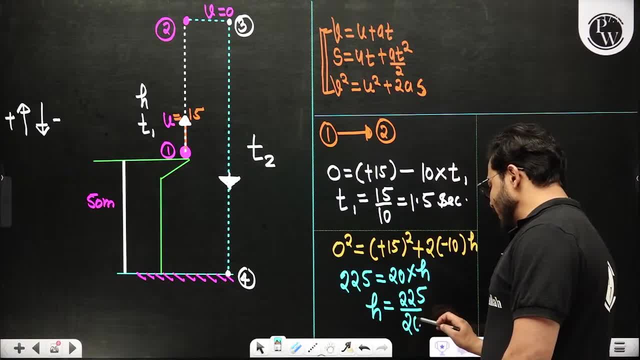 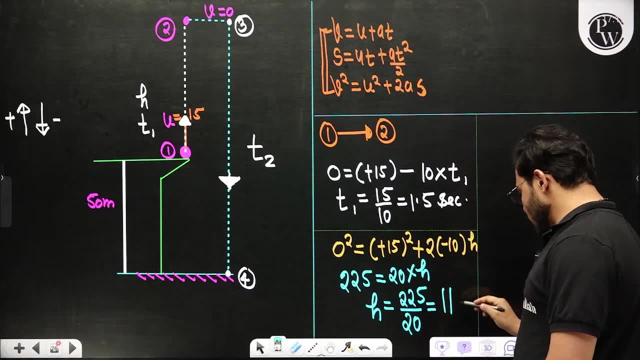 225 upon 20.. So when you solve 225 divided by 20, how much will it become? 2 minus 1 is 2.. 2 minus 1 is 2. And 2 minus 1 is 2.. 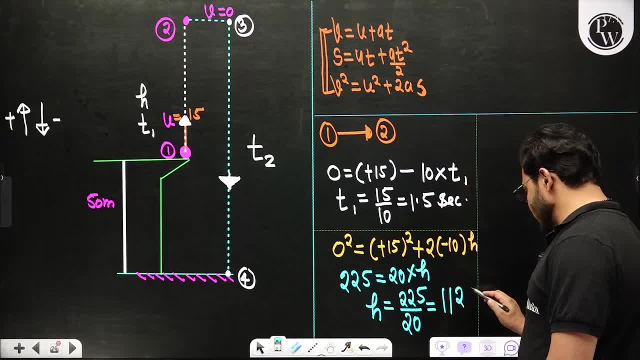 2 minus 1 is 2. And 2 divided by 2 is 4. And 2 divided by 5 is 10.. So will it become 112.5?. Will it become 112.5?? 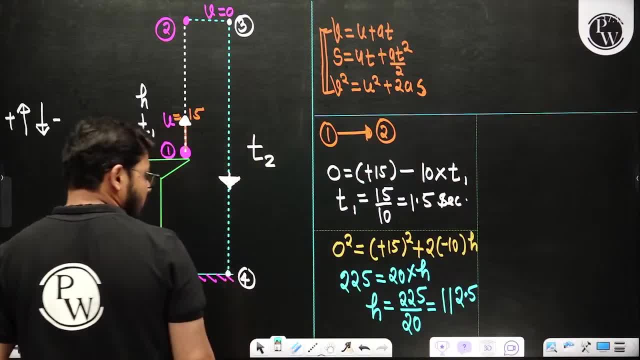 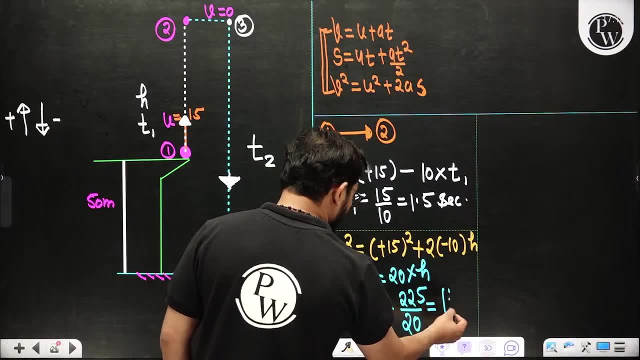 See, is this what is coming? 225, no, no, It will probably become 11.2.. Not 112.. It will probably become 11.25.. It will probably become this 11.25. Because upon is 20, right. 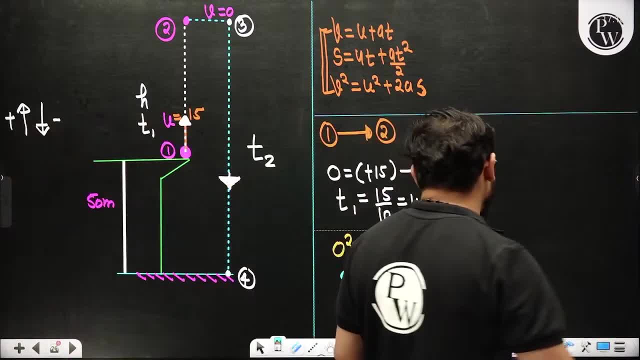 Will it become 11.25 or not? Very good, 11.25 has come. Very good. The answer of all the children has come. Okay, Now listen to me Now. for whom will you like to apply the equation? 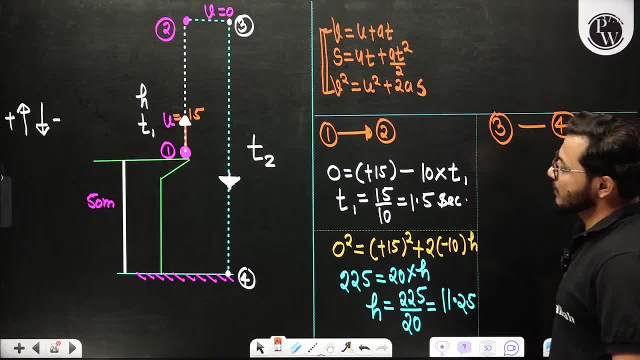 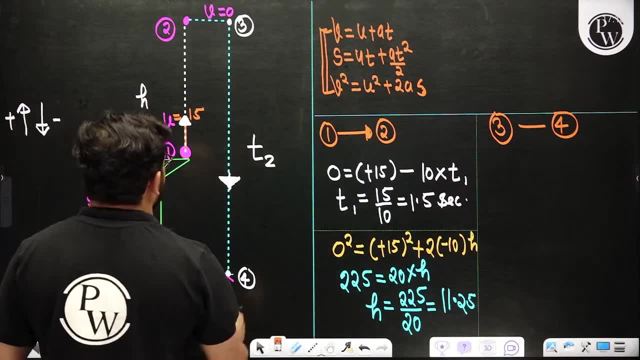 Between 3 to 4.. Between 3 to 4.. Listen carefully, Come on, tell me Which equation will you like to apply between 3 to 4?? I want to calculate the time. Tell me how much will be t2?? 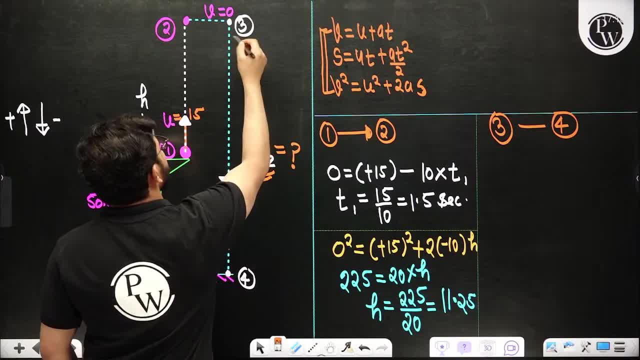 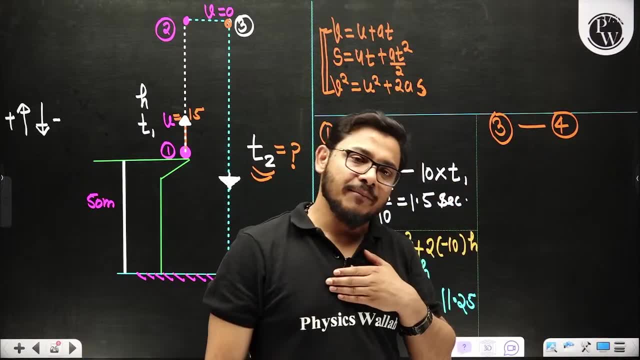 Tell me which equation will you apply. See, you know the original velocity here. Listen to me When you are going from 3 to 4, So from where do you go From point 3.. So point 3 is the initial position for me. 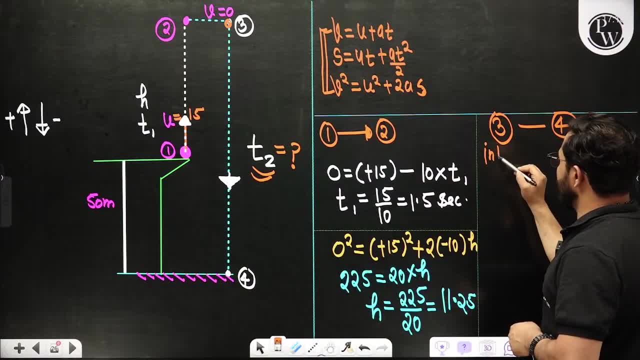 Point 3 is the first initial position for me. It is initial And point 4 is final for me. Remember: wherever you go, it becomes initial for you And wherever you reach, it becomes final for you. You tell me which equation will you like to write? 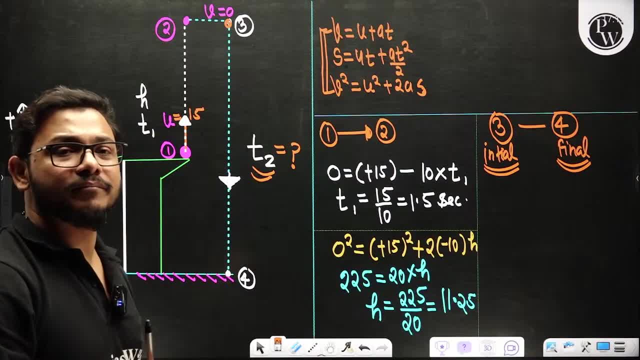 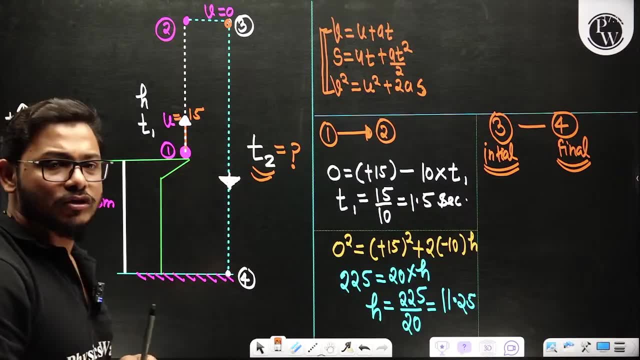 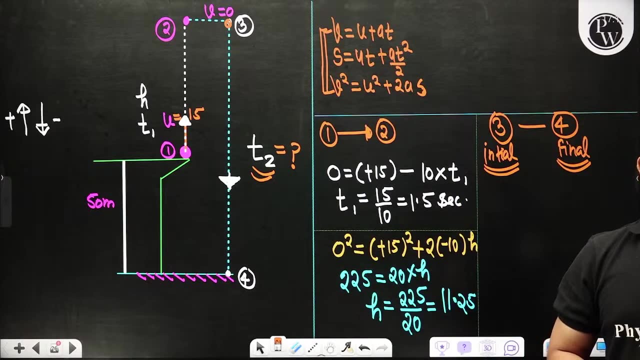 The second one. Very good, Will you like to write the second one? Is it 11.2?? Did I write 11.25?? Did I write something wrong? 11.25?? Is it 11.25?? Okay, now listen to me please. 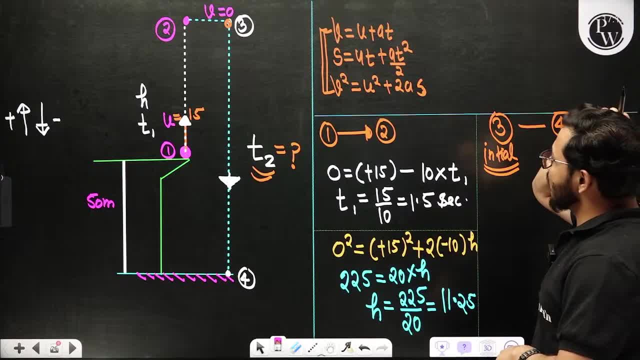 Now, what am I going to write here between 3 to 4?? Tell me one thing: what is the value of s? Please, please, please, please. Now see there is a problem here. There is a problem here. 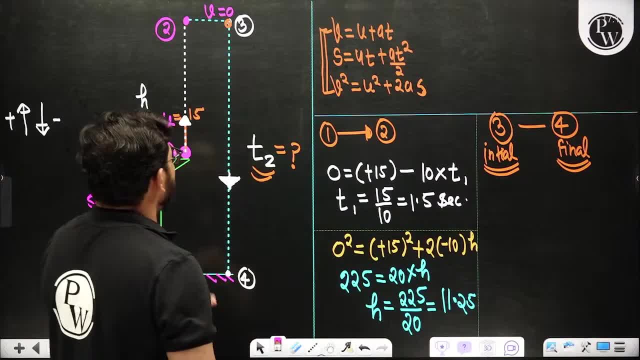 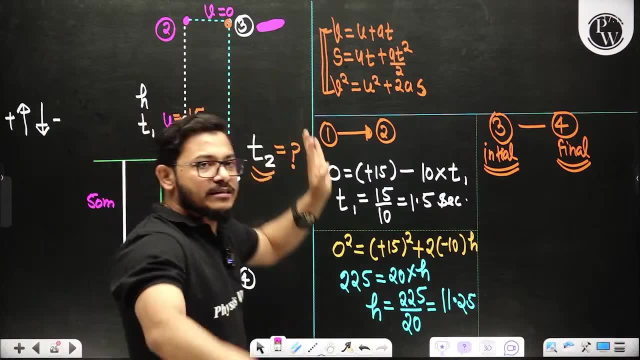 There is a problem here. Wherever you go, I am talking about that. Where do you go? Point 3. So this is the reference for you. Make it a star. Now listen to me. Some kid will say the height will be positive or negative. 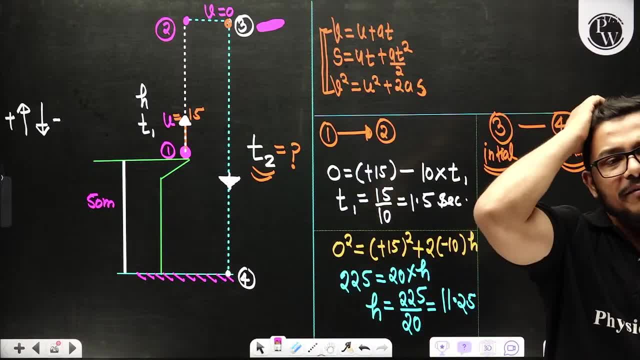 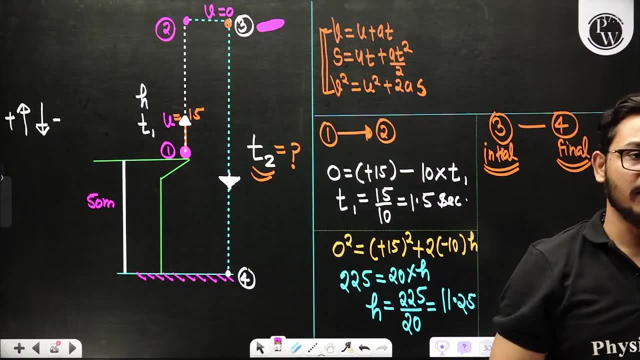 Tell me quickly The height will be positive or negative. Some kid will say the height will be positive or negative. The height will be positive or negative. Wherever you go, it is the initial position You go from. there Is the height positive or negative for you? 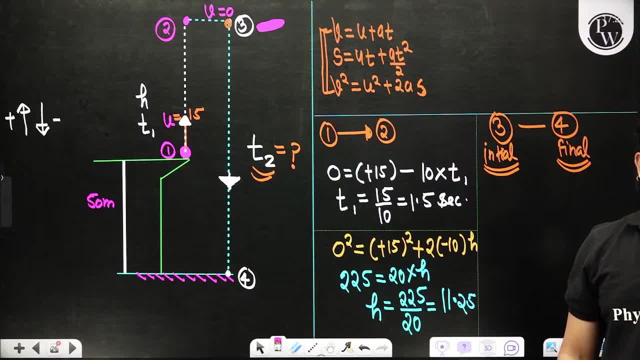 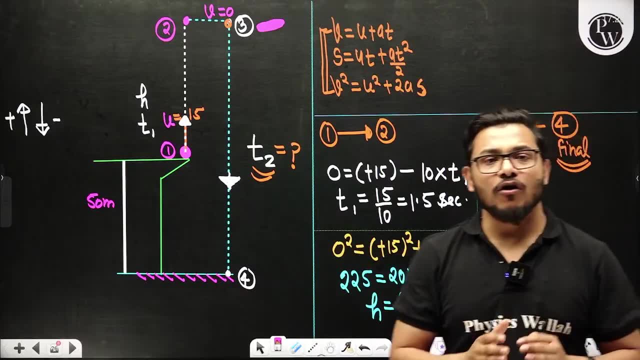 Tell me quickly: Is the height positive or negative? Is the height positive or negative? You can't put the first one because you don't know the final velocity at point 4.. You don't know the final velocity at point 4.. See, you are making a mistake. 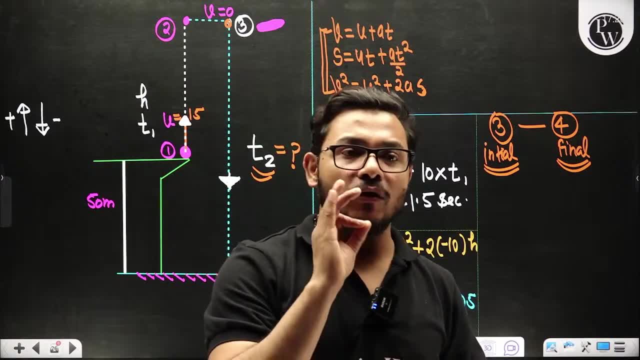 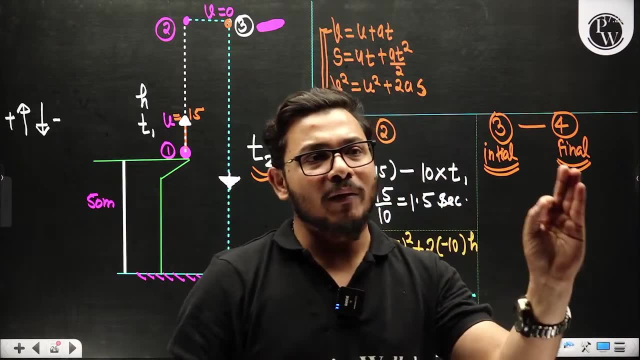 Listen to me again. The height will be negative. Why will it be negative? See, all the kids are telling wrong. You don't understand what I am saying. When I apply Newton's equation of motion from where you go, it is called point 1 for you. 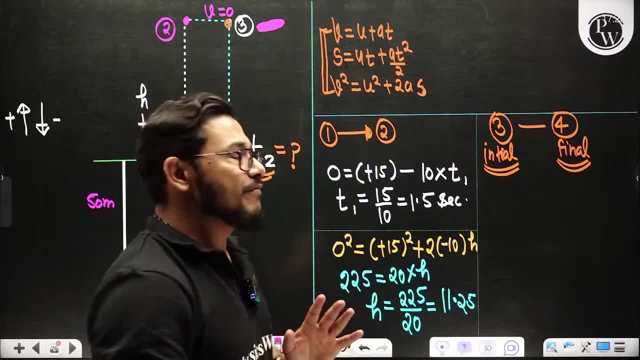 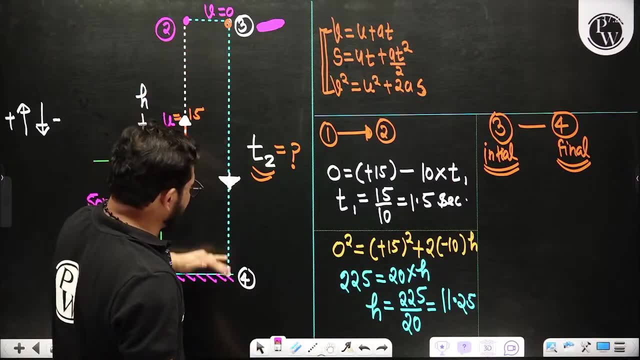 And from where you reach. it is called point 1 for you. Please try to understand again. The point where you go is initial And the point where you reach is final When you are going from point 3 to 4,. 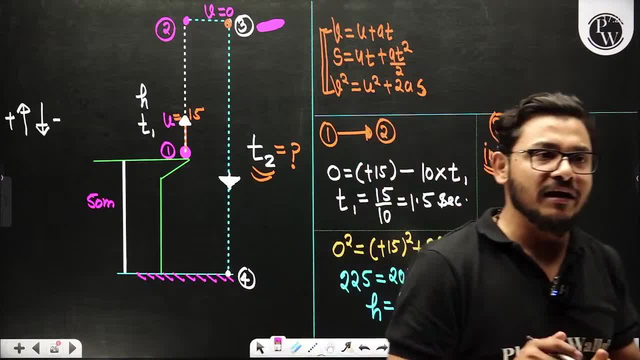 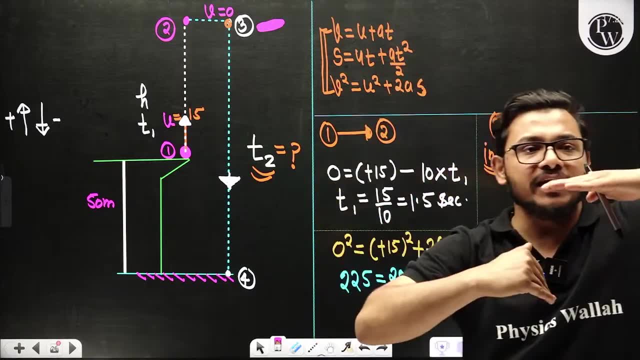 then you are going down, so the height will be negative. You don't understand what I am saying. The point where you go is your initial position. In respect to that, see if you go up or down. When you go down from point 3,. 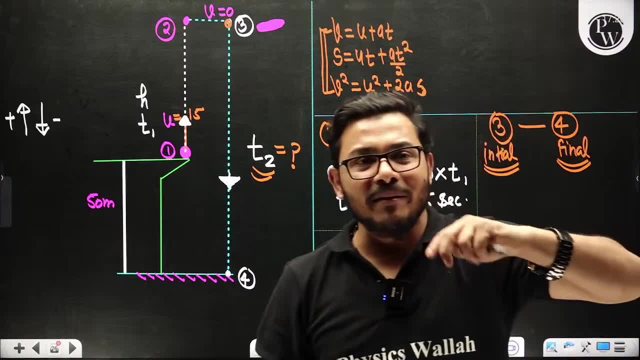 when you go down from point 3,. you don't understand what I am saying. Please message me quickly. Do you understand what I said? Where you go from From point 3.. When you are going down from point 3,. 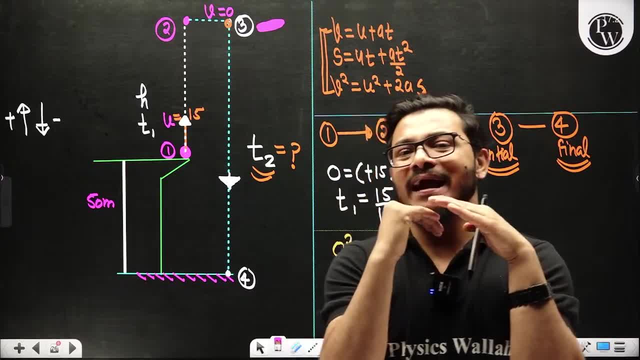 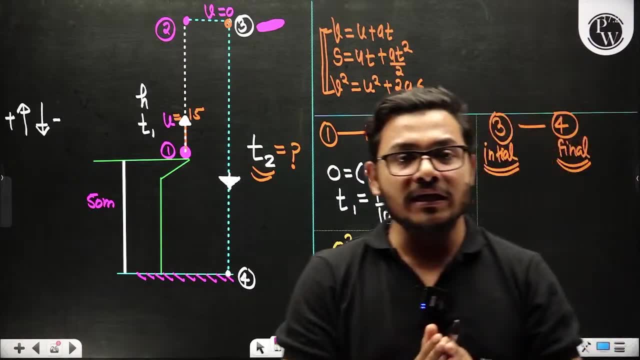 then the height, what is going to be? What is going to be the height of point 3? for you See that height from point 3.. If you go down, then that height will be the negative. Before applying Newton's equation of motion. 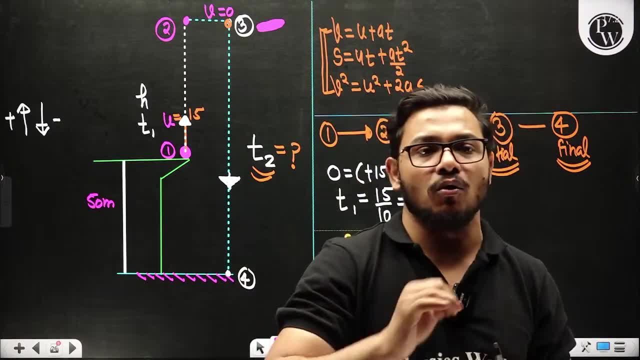 you have to keep one thing in mind: You have to see from where you are going. So if you are going from point 3, then if you are going from point 3, then if you go down, then it is negative. 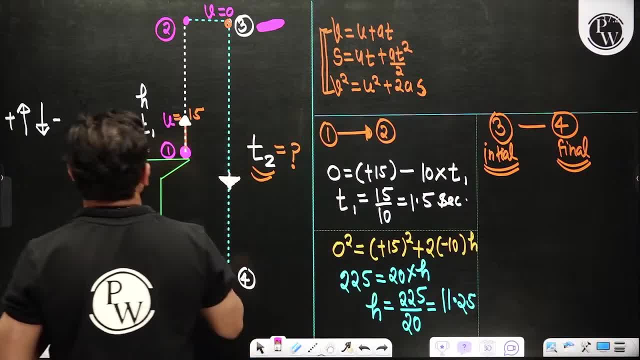 And how much should be the total. How much should be the total? How much should be the total? See how much was this: 11.25.. Add 60 more to this. If you add 60 more, how much should it be? 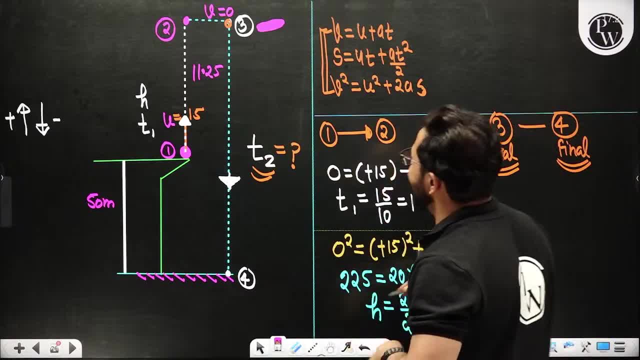 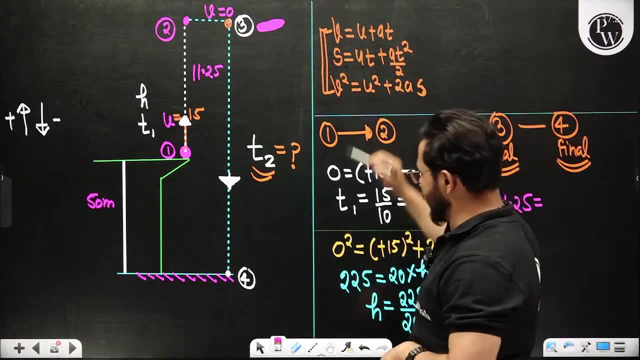 If you add 60 more then 50. So adding 50 more it becomes 61 minus So 61.25.. And become is equal to S's value. And u t What is u? Original velocity. 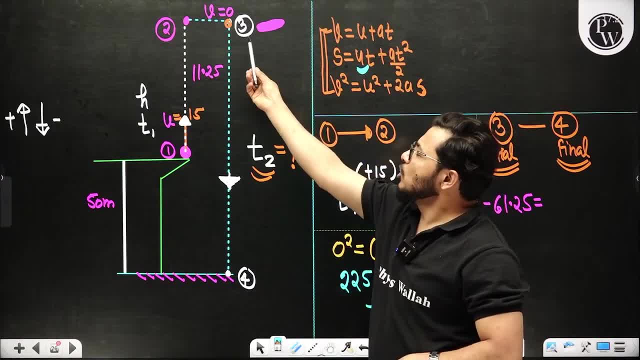 And what is the original velocity From where it goes? So if it goes from point 3, then the original velocity of point 3 is 0. So 0 into t And plus of 1 by 2.. 1 by 2.. 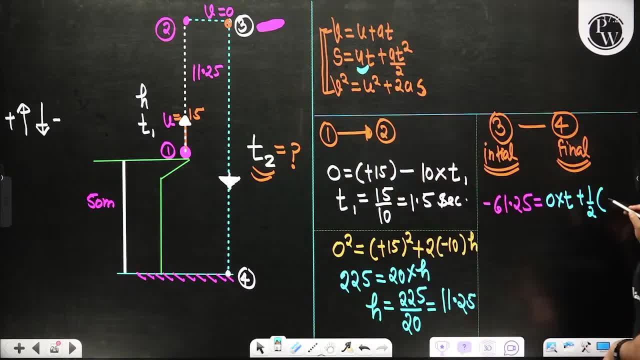 And where is the acceleration? Acceleration is always on the lower side, So minus 10.. Minus 10.. And into t square: Minus 10 t square. So how much Minus k, 61.25.. 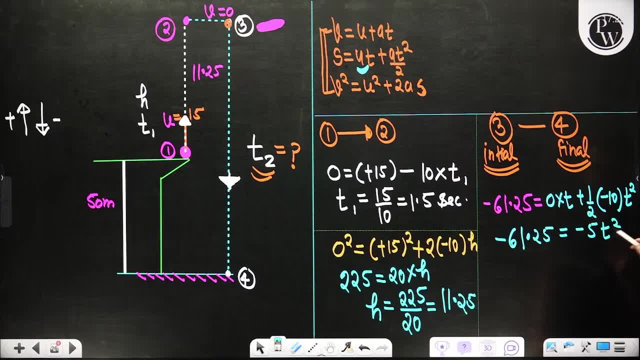 And become is equal to Minus k 5 into t square, So you will solve this. So this is t2.. t2 square, Because I have taken t2 as the time. So what is the value of t2?? 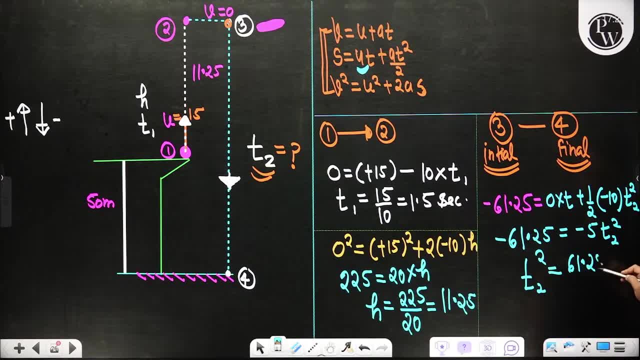 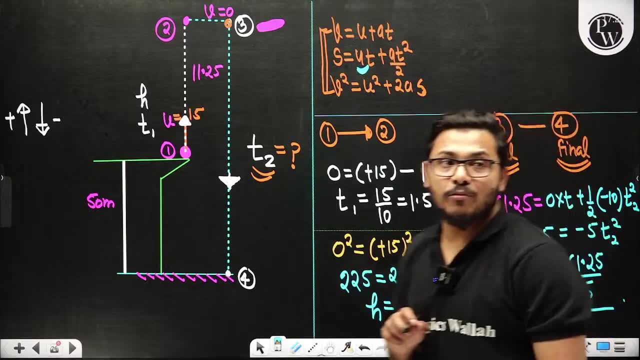 The value of t2 square 61.5.. And upon me 5.. If you solve this, then the value of t2 will come. If you solve this, then the value of t2 will come. So I was asking you that question. 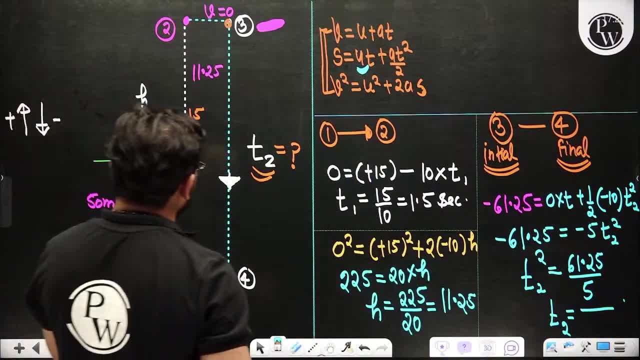 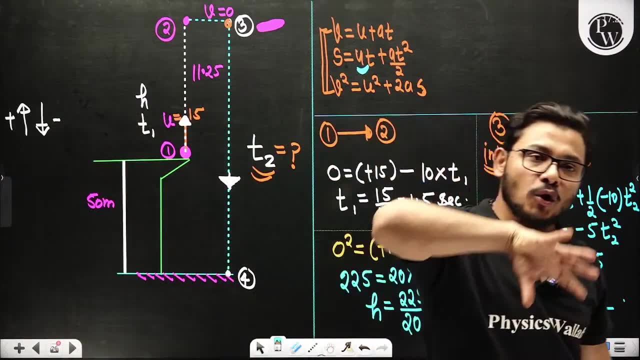 After how much time in total? After how much time in total that ball will hit the ground. So the time will be t1 plus of t2.. So see, do you know why I took this question? Both the concepts are involved in this question. 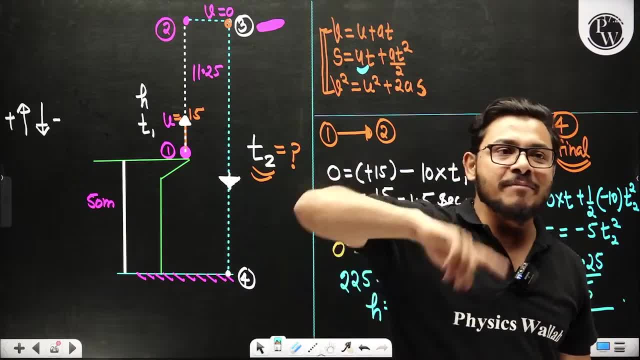 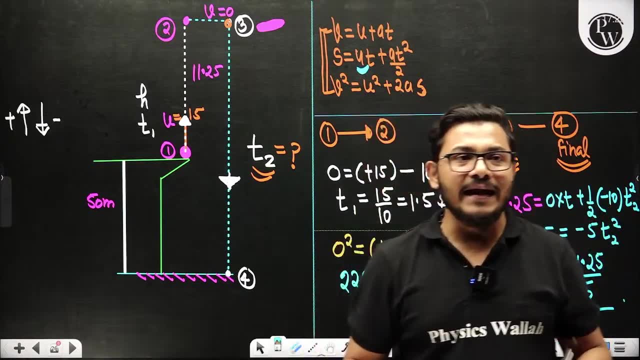 Newton's equation of motion is complete. You also got to know when to take terms positive and when to take negative. You also got to know when it will be positive and when it will be negative. So that only gave one idea that how many children are there. 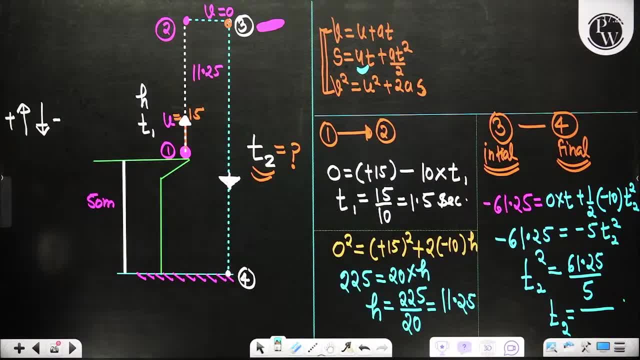 who have understood this whole concept? Please tell me quickly, All of them. The negative of height did not come in the sun. Listen to me again, Mr Adil. Remember one thing, son. Remember one thing, son, When you apply Newton's equation of motion. 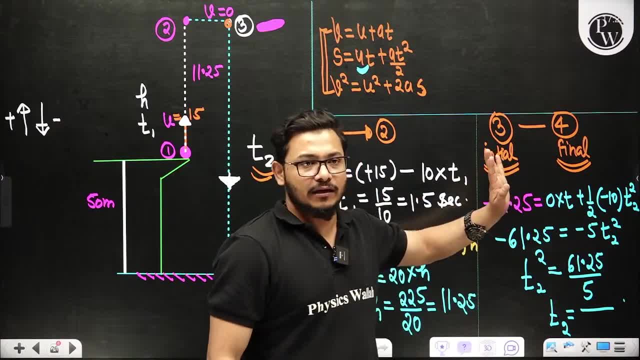 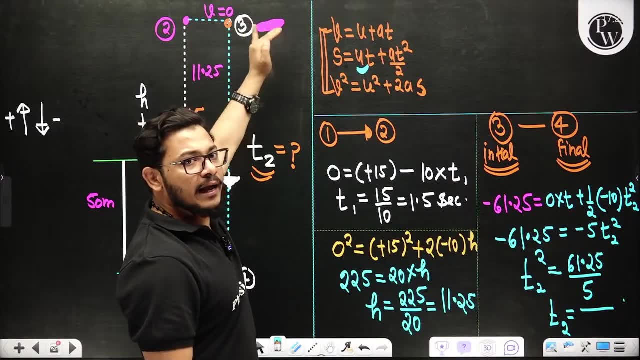 so, like you have to apply the equation from 3 to 4, Adil, So for you the original is 0.3.. You see everything in respect of 0.3.. So 0.3 is now original for you. 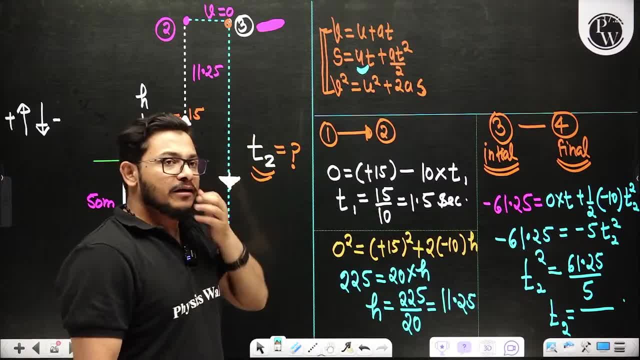 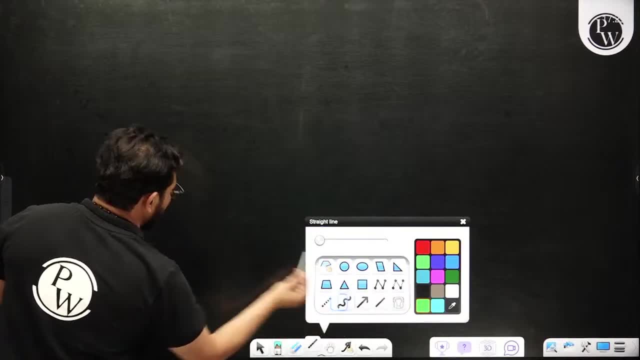 If you go down from here, then it is negative. If you go up from here, then it is positive. Did you understand? As I explain again, listen to me. When you called it 0.1 in the starting, you called it 0.1, right. 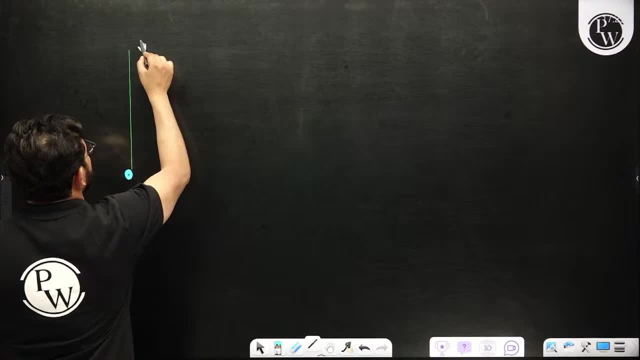 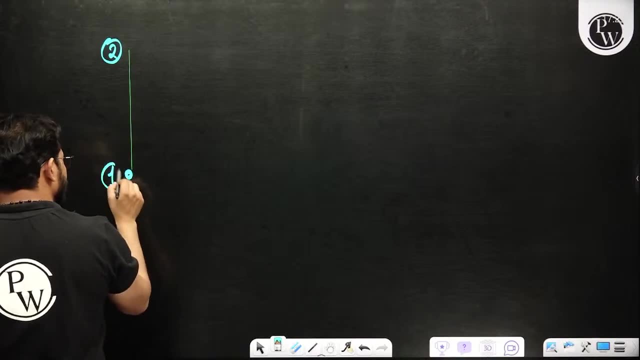 You went from 0.1 to 2.. You went from 0.1 to 2, right. So when you applied the equation in the starting, then I applied the equation between 1 to 2.. So what did I believe? 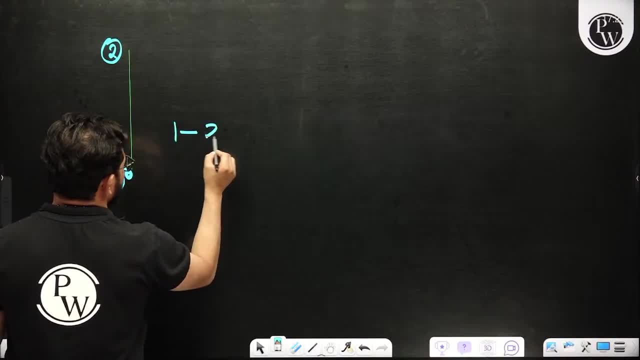 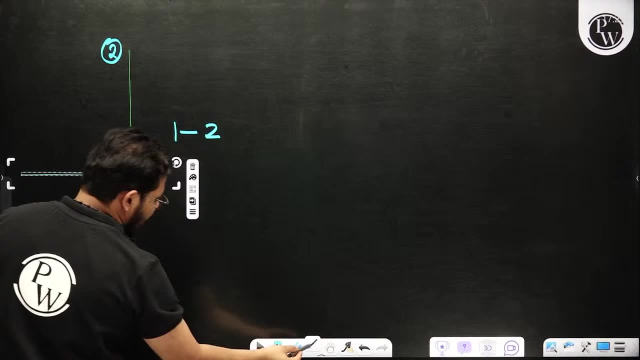 I believed that let's go from 1 to 2.. You go from 1 to 2.. Now you will see everything in respect of 1.. Remember my words. Now you have to see everything in respect of 1.. If you go up from here, 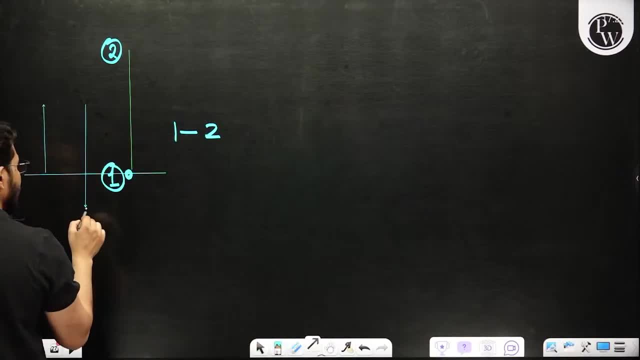 if you go up from here, then it is positive. If you take anything from here, then it is negative. That's it. This is positive and this is negative. That's it. Like in the story, I wrote the same thing. 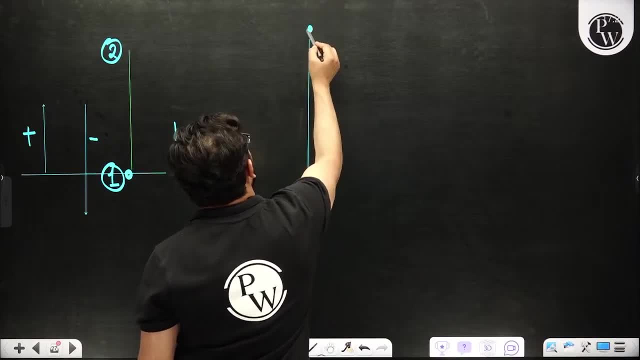 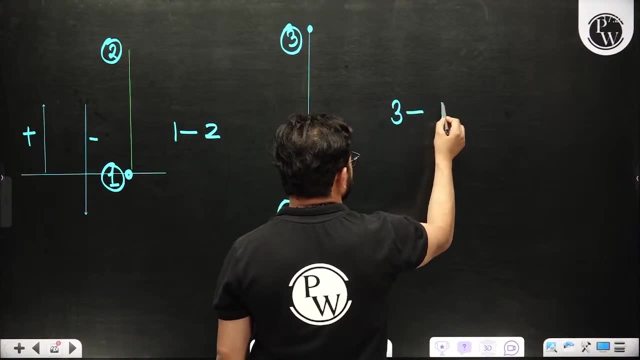 When you are talking from 3 to 4, where do you go from? You go from 0.3 to 4.. Between whom do you want to apply the equation? I want to say between 3 to 4.. So 3 is original for me. 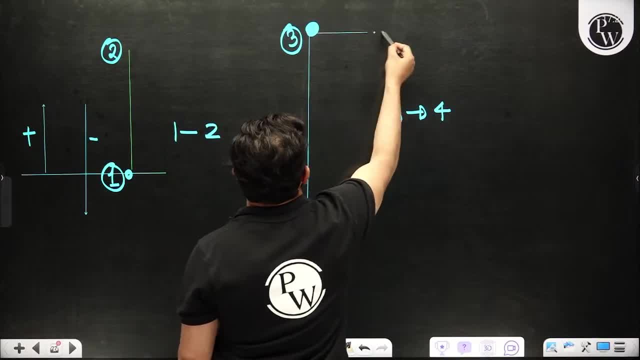 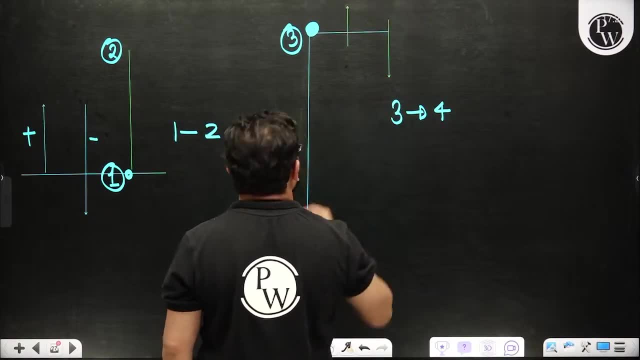 If you go from 0.3, from here in respect of this line, if you take any distance from here, if you take it up from here, then it is positive. If you take it down from here, then it is negative. 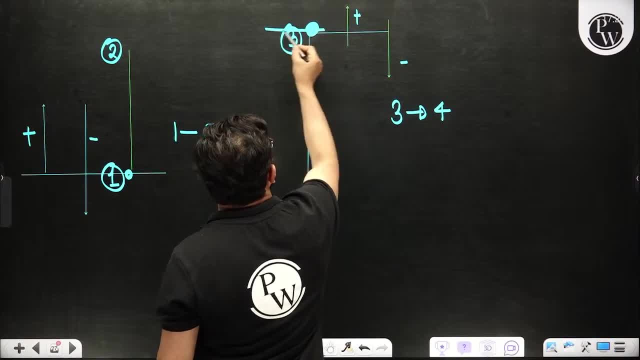 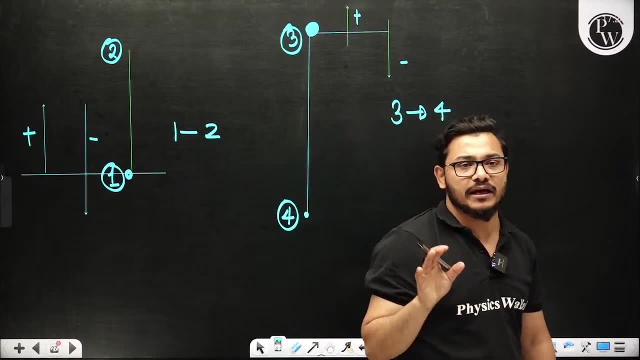 That's it, Because this is a way for you to understand. This is an origin point for you. If it is up from origin, then it is positive, It is negative for you. That one is the one idea, please. This is the way I have explained this story to you. 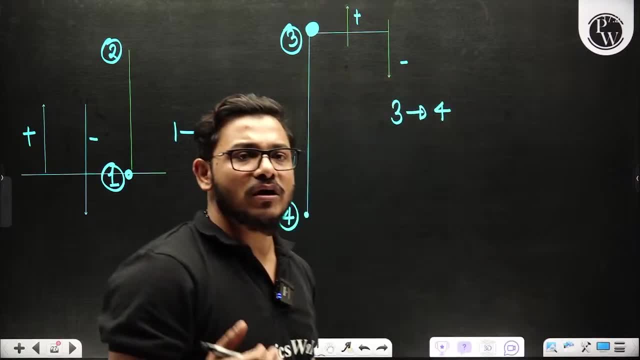 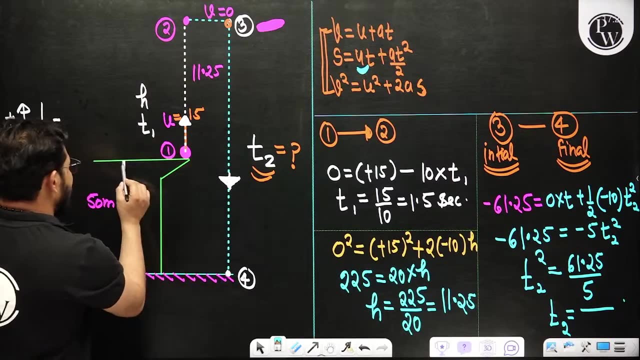 I hope you got the concept. You must have understood something. Okay, how did you take 61.5?? Son, tell me one thing: Between 3 to 4, what will be the total length? 50 meters is the height of the tower. 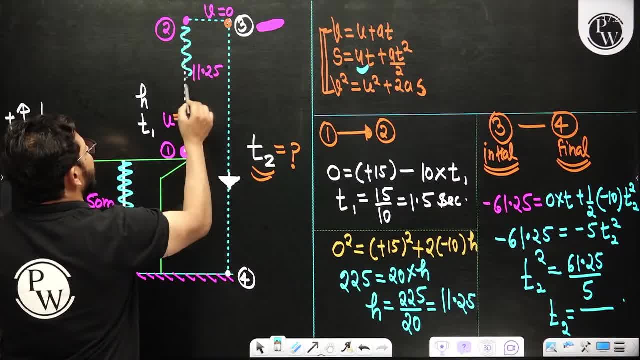 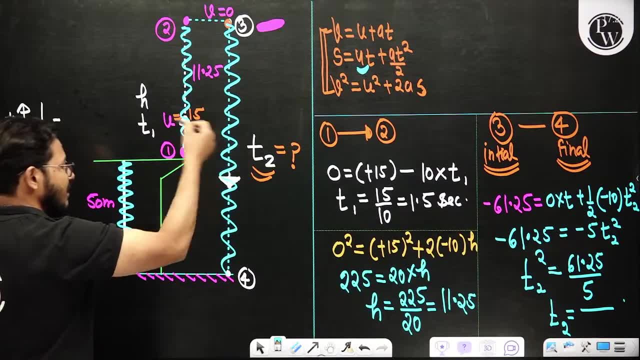 50 meters is the height of the tower And 11.25, you have calculated this. So, from here to here, what will be the total distance? Tell me, 50 plus 11.25, in total, will it be 61.25 or not? 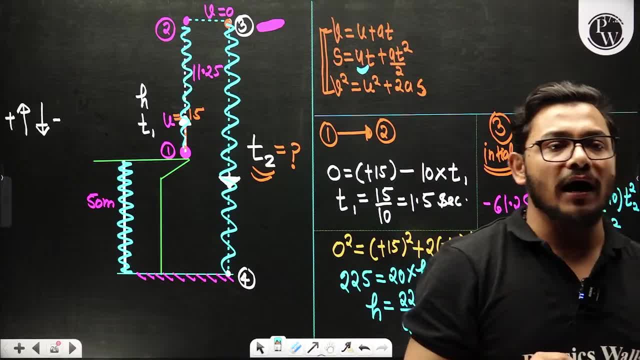 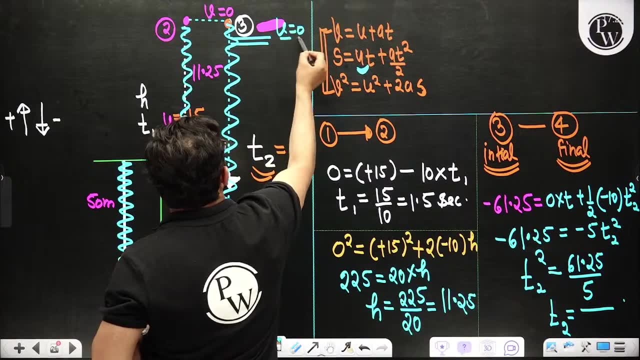 Did you understand anything? Yes, Why did U become 0? Because at maximum height, here, at point 3, the velocity is 0. Here U is 0 for me for point 3.. For point 3, the velocity is 0 for me. 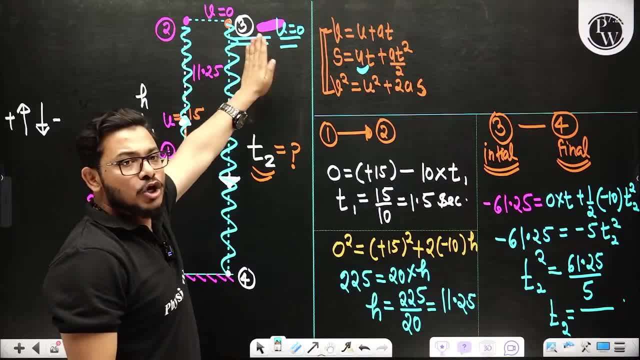 Because when it goes from 3 to 4, then point 3 is original for me, So you have to see all the properties at point 3.. Mr Chaudhary, did you understand? Mr Chaudhary is clear. 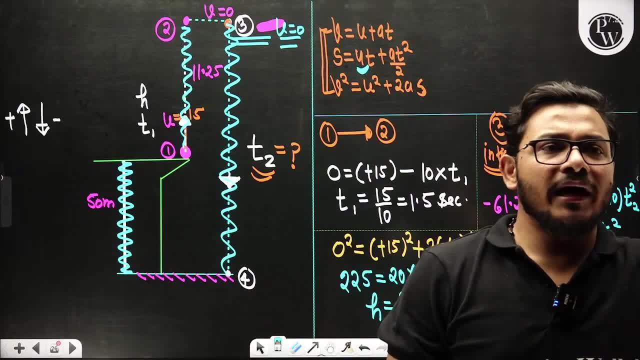 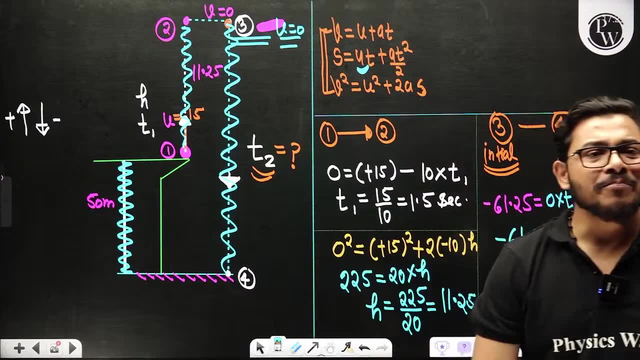 Mr Logan, Mr Adil, Mr Mechanical Trick and Asit Subham Sahoo, Adil Khan, All the children who are listening to the lecture. tell me, Did you understand everything, Yes or no? You got the concept yes or no? 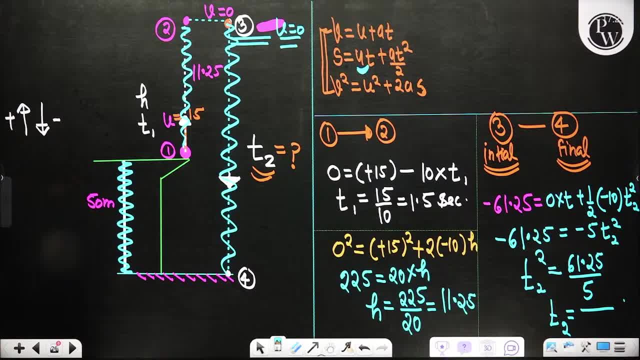 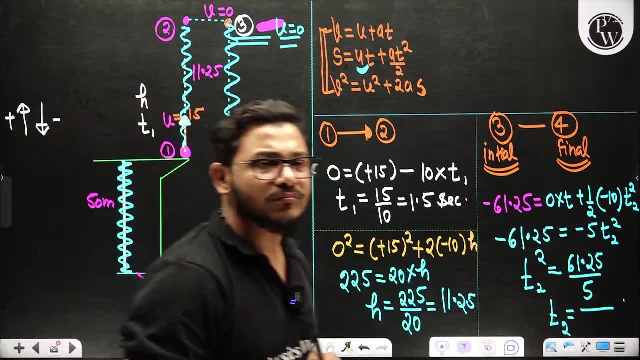 Did you understand what I have written? Did you understand Newton's equation of motion? How did Sir write Newton's equation of motion? Tell me quickly, please Now. did you understand everything Now? no child will ever be deceived in life. 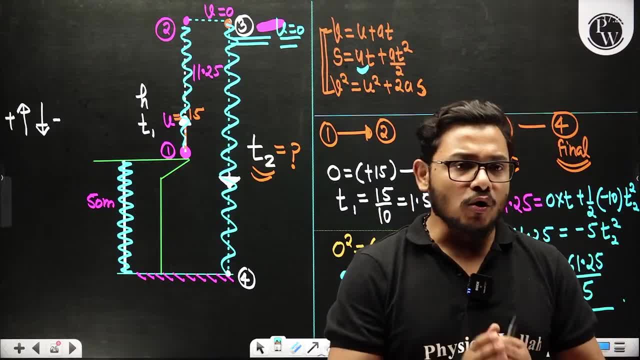 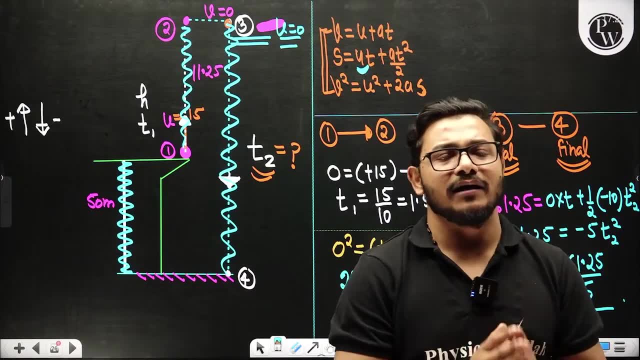 Did you understand everything that I have written? You don't have to do anything. You just have to keep in mind that where you have come from, where you have reached, then that velocity will be positive or negative. That one is the one idea, please. 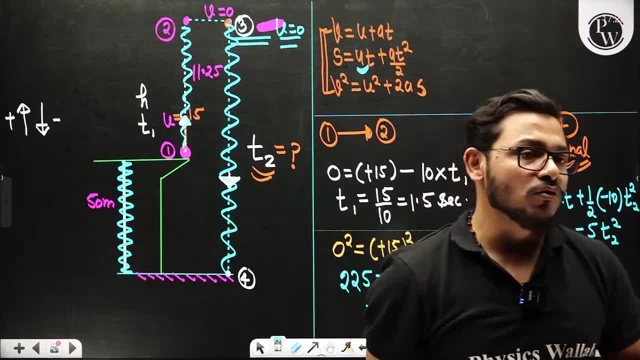 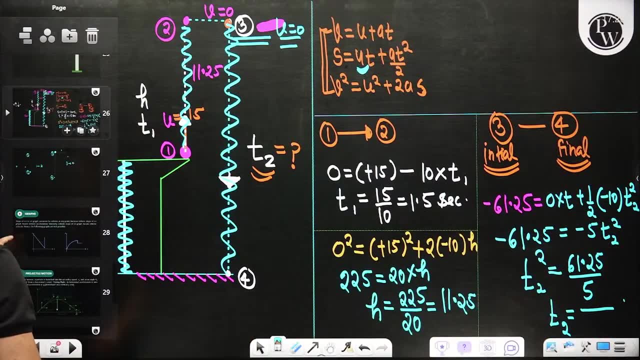 So in this way, you have to write that problem, And I hope you must have understood it. Okay, Very good, So did you understand Newton's equation of motion. There is no big problem in this. Now, the next point that I am going to show you is graph. 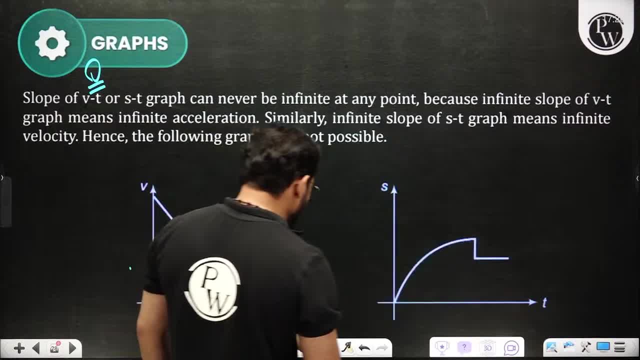 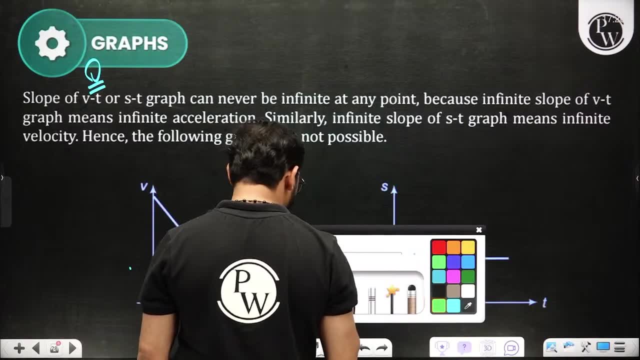 This is a very important concept of graph for you. Please listen carefully for one minute. This is a very good concept of graph. I will tell you some things here. Just understand this much. First of all, I will explain you the basic funda. 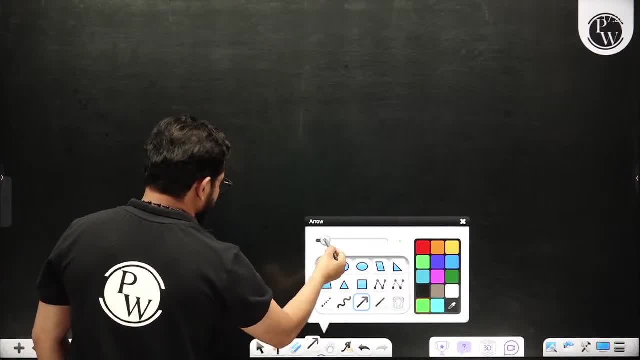 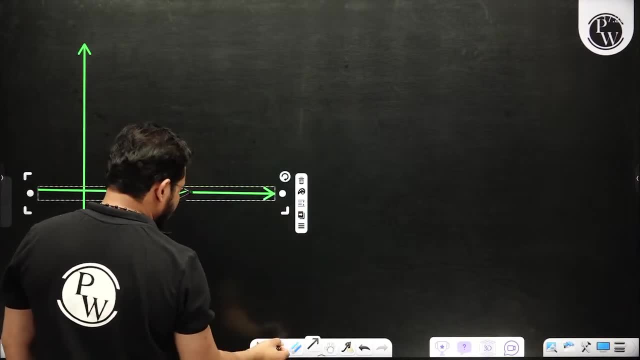 After that I will go ahead. I just ask you this, funda, in your examination in the question: What does its graph give you? This question has been asked in SSC JEE in the examination. First of all, let me tell you one thing. 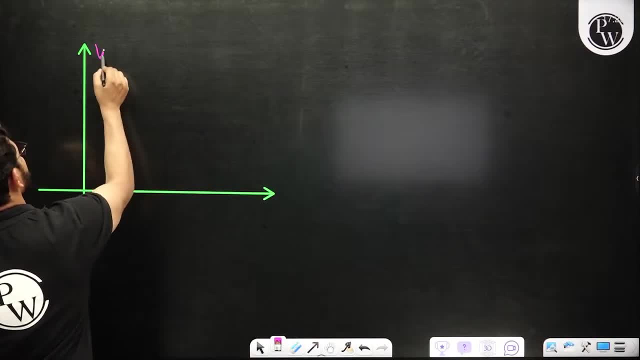 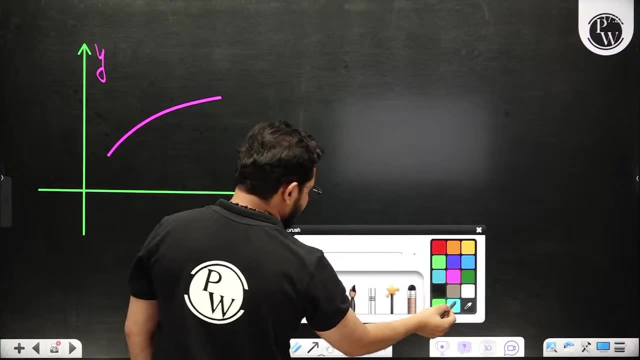 If I have made a graph of Y versus of X here. Okay, Please keep listening to me. If I have made this graph, Someone tell me to tell me the slope of this graph. So I am teaching you to write everything one to one. 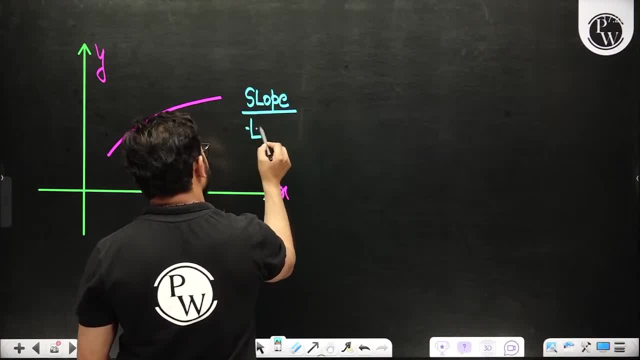 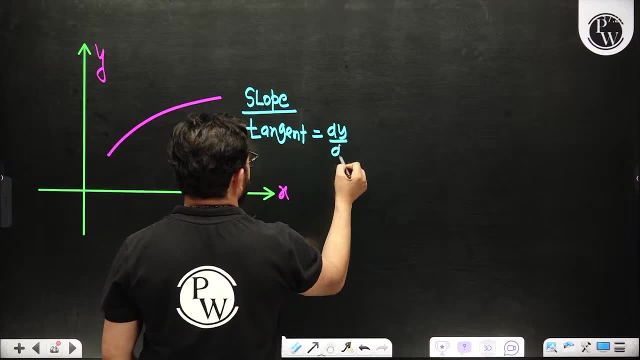 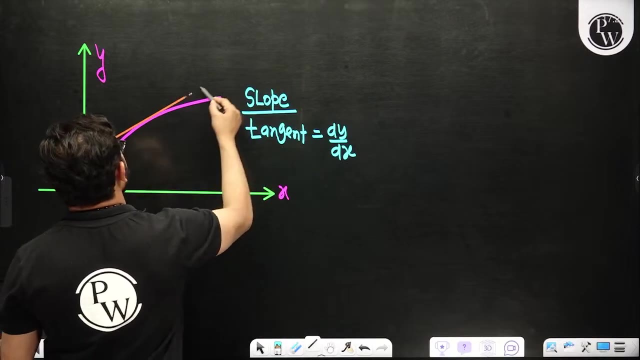 Look, the meaning of calculating the slope is: Draw a tangent. What does slope mean? Draw a tangent And tangent means dy upon dx. Please always remember It means to differentiate dy upon dx. So if you have calculated the tangent, 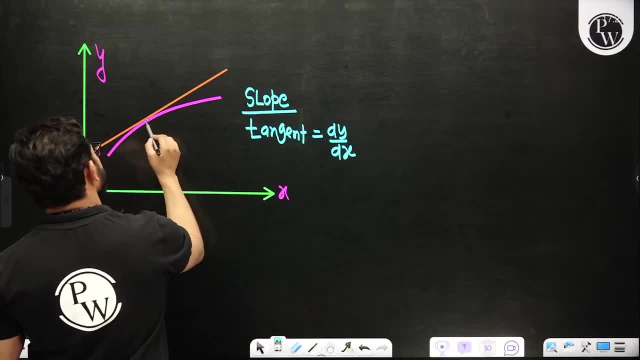 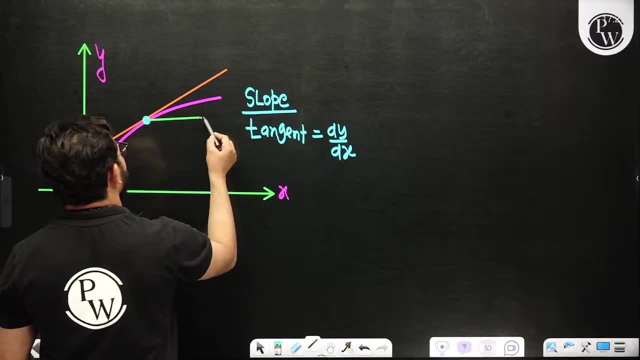 then you have to calculate the slope at that point, Just like you had to calculate the slope at this point. So what do you have to draw? You have to draw a tangent or dy upon dx. So how much angle will it make with the horizontal? 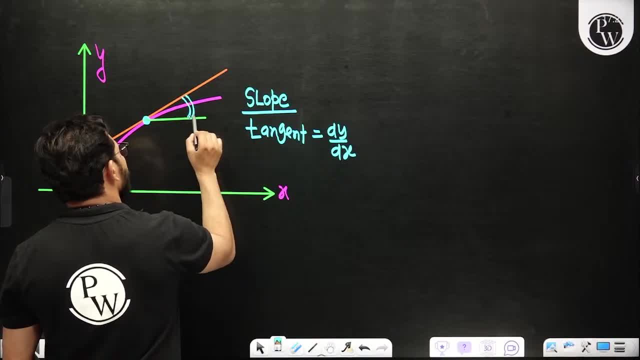 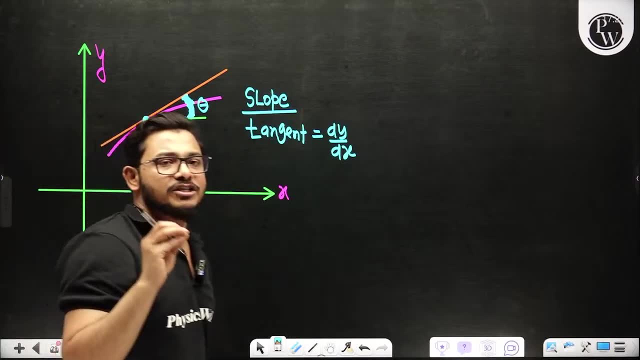 So, whatever the inclination angle will be, this is its slope, This is the inclination of this line, This is the angle it is making from the horizontal, So that one is called slope. So what is the meaning of slope? What is the meaning of slope? 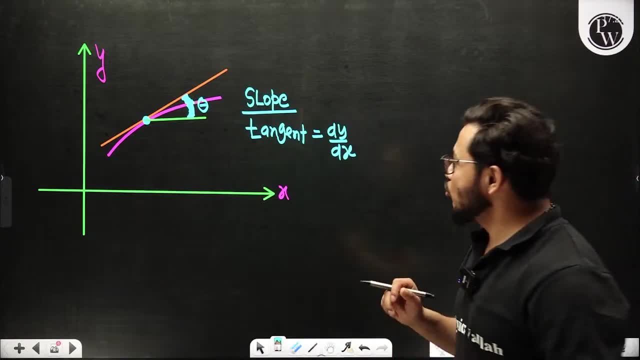 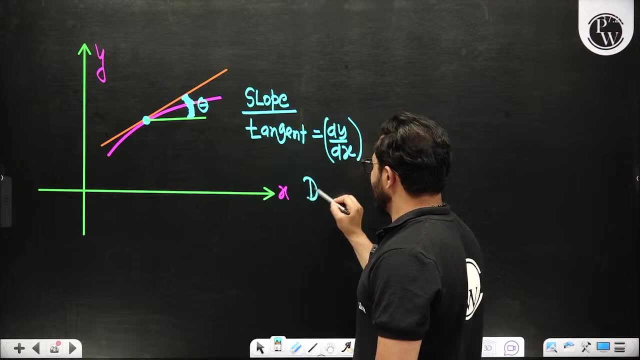 To differentiate, To write dy upon dx So you never forget in your life. Slope means to calculate the tangent, And tangent means dy upon dx. It means to differentiate, To differentiate. Okay, To differentiate, So you have to differentiate here. 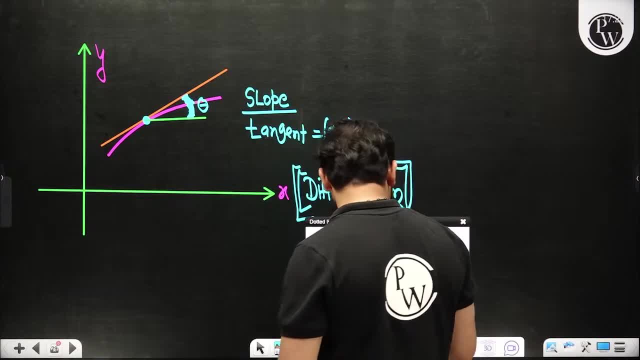 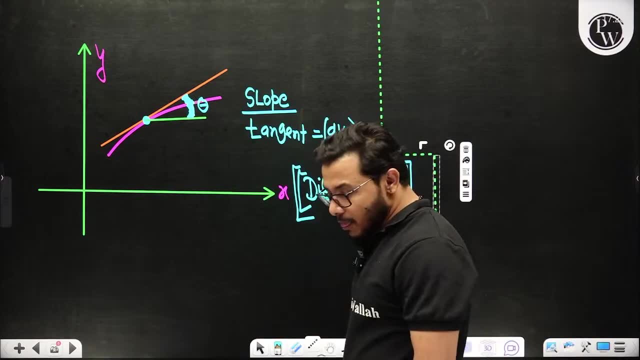 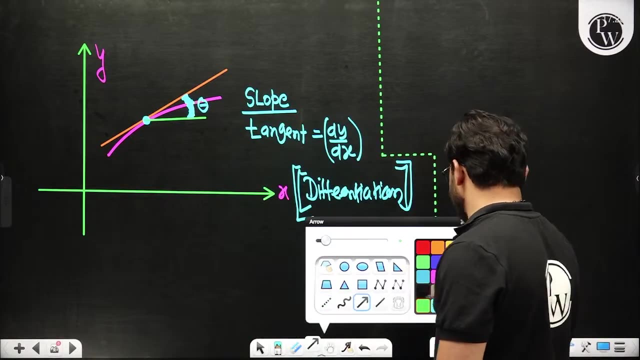 My mouth got dry while speaking. I can't drink water. My tongue got dry. I will leave you soon, 15 minutes before then. That one is the one idea, Y versus of X, The way I have written it. Now I will see this thing here. 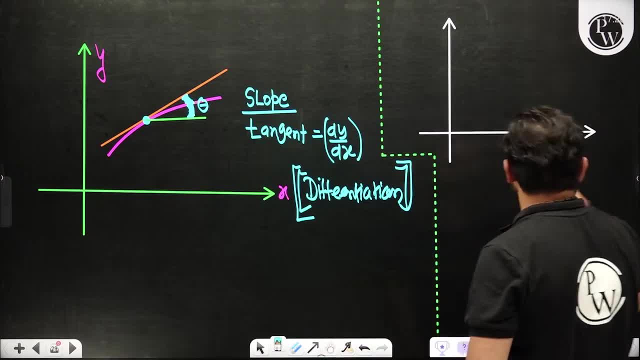 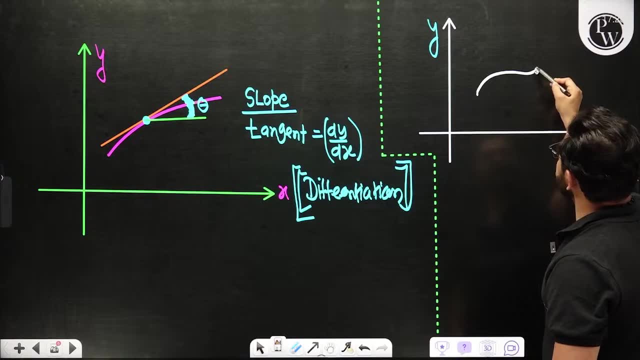 How it is being written here And that one is the one idea. If I make a graph of X versus of Y here, Let me tell you the basic concept, And I have made it like this. I have told you to calculate the area of this graph. 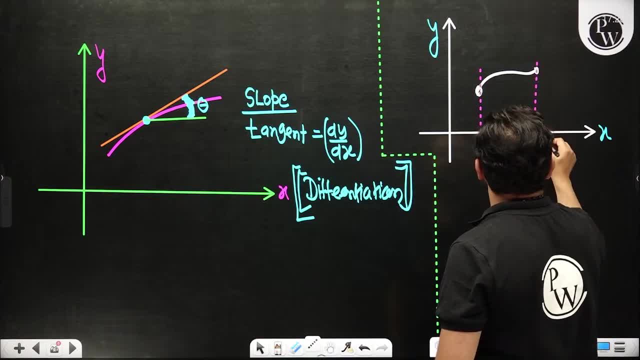 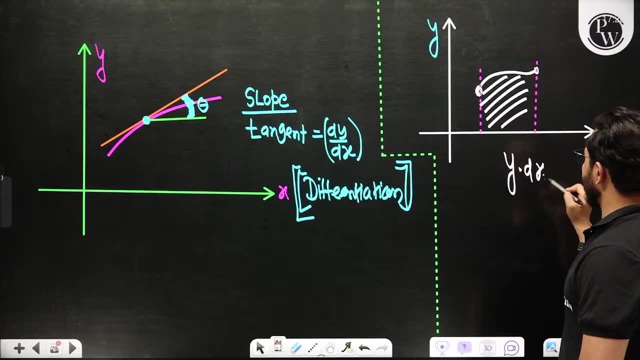 Area, So you don't have to do anything. The meaning of area is this: Calculate this. The meaning of area is to calculate all these things. What is the meaning of area? Write Y into dx, That's it, And do the integration. 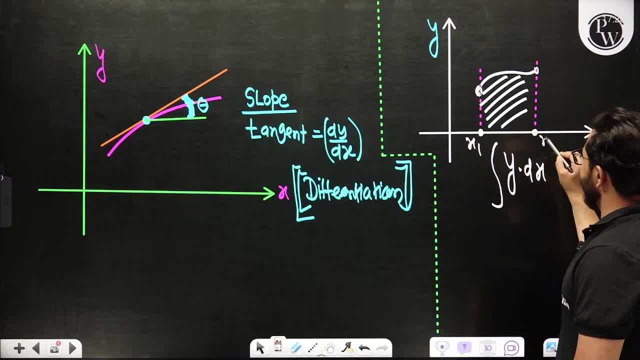 Suppose you went from here to here. So suppose this is X1 and this is X2.. So you integrate it from X1 to X2.. So this means to calculate the area. So what is the meaning of area? 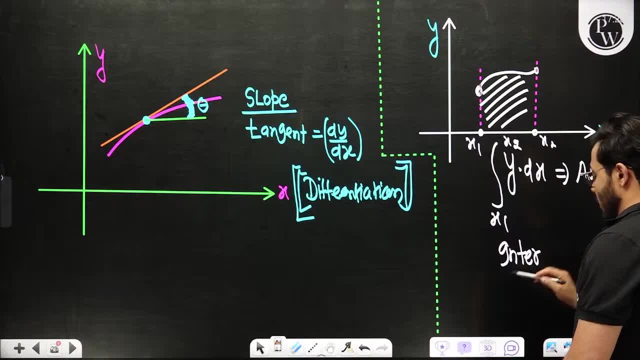 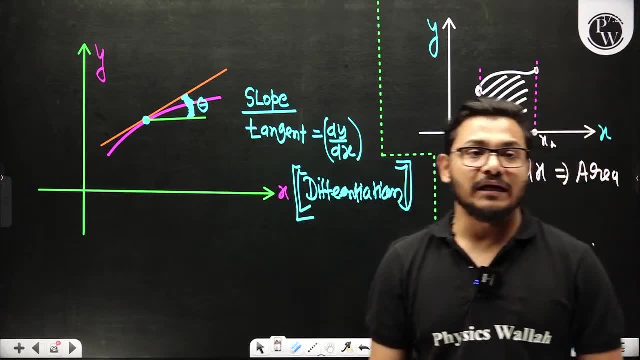 It means to do integration. What to do To do integration? I have told you the basic concepts. You will have to understand this, please. That one is to do integration, That one is to do integration. So I have made you like this. 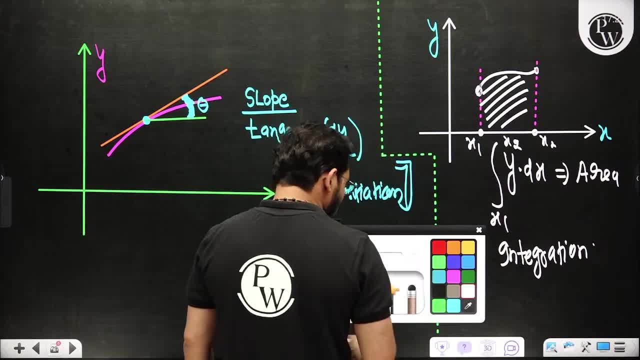 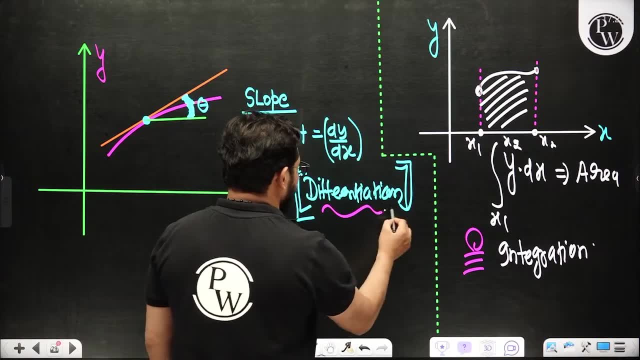 From X1 to X2, that one is area- And to do integration. So I have told you all the things here, That how to do integration And how to do differentiation. Okay, Now, what I do here You will see in a minute. 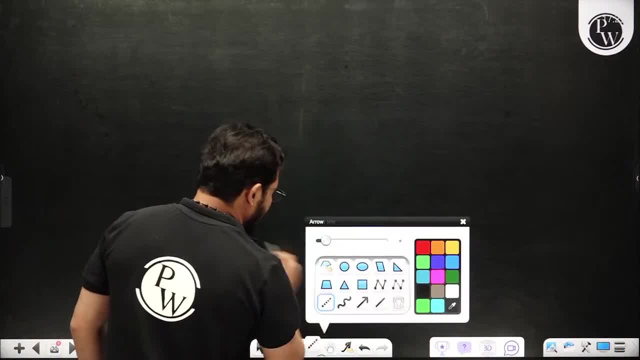 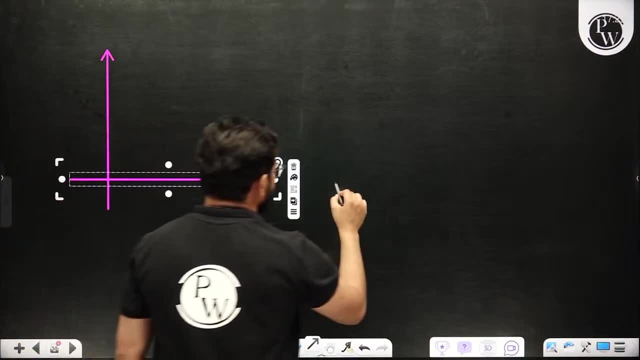 Now I will tell you the basic concepts here And I will tell you the important thing. Please see, for a minute, If I make a plane here, If I make a graph like this, I am making a graph like this. Please be careful. 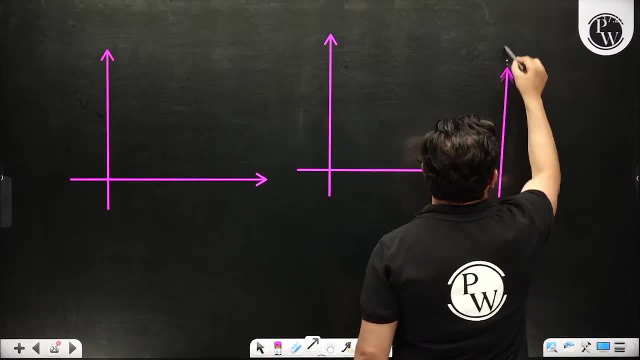 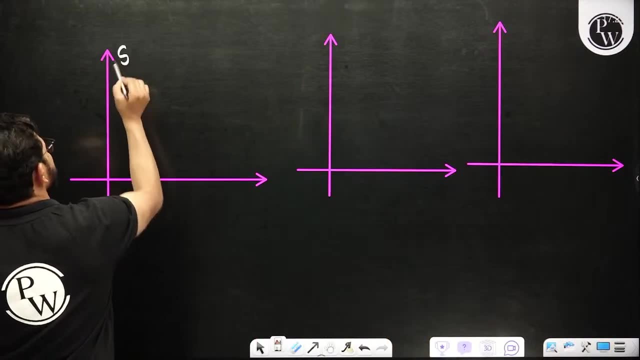 It is very good, I am making a graph like this And I am making a graph like this for you. I am making a graph like this. Okay, I have made three graphs like this. You don't have to do anything. First, you have made a graph of displacement versus of time. 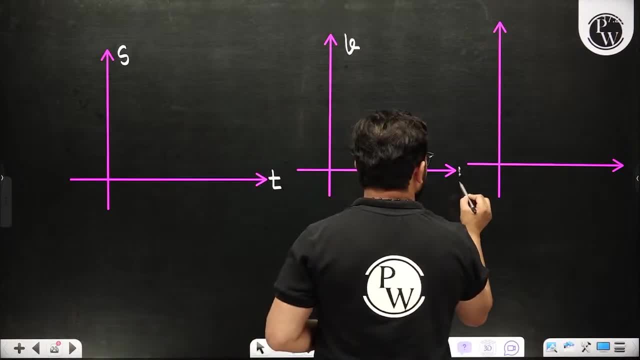 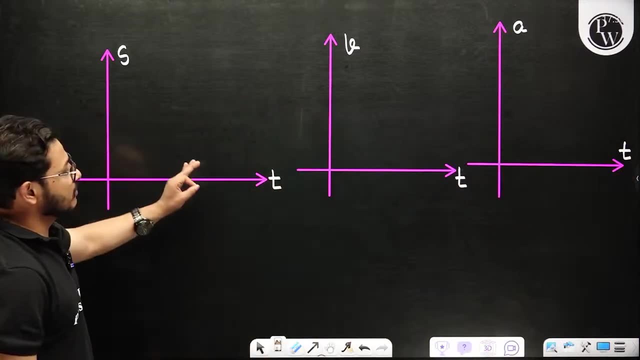 Second, you have made a graph of velocity versus of time. And third graph you have made of acceleration versus of time. Please be careful: Acceleration versus of time. you made One graph you have made of displacement versus of time. Second graph you have made of velocity versus of time. 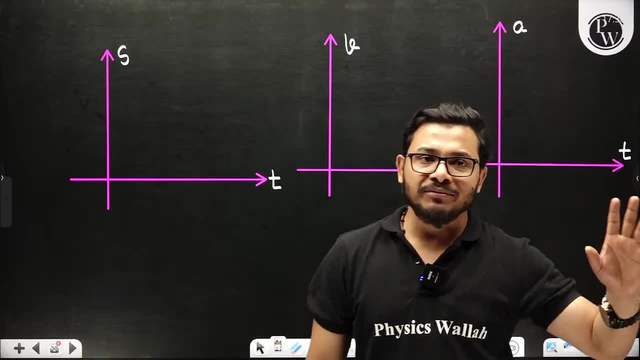 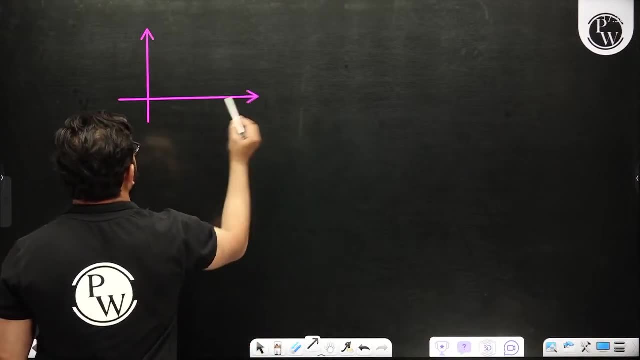 And third graph you have made of acceleration versus of time Means. you are trying to make three graphs. Three graphs Means how are you making? You are making like this: First graph is this: Please be careful: Three graphs And keep listening, please. 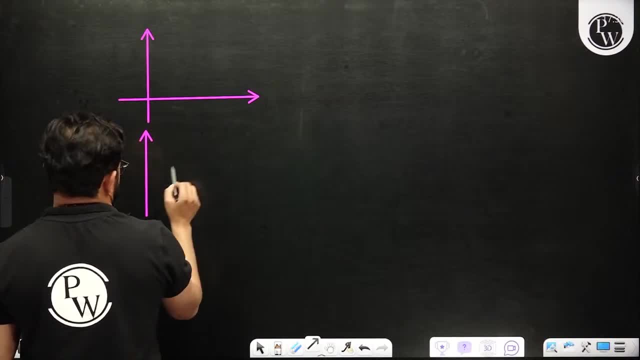 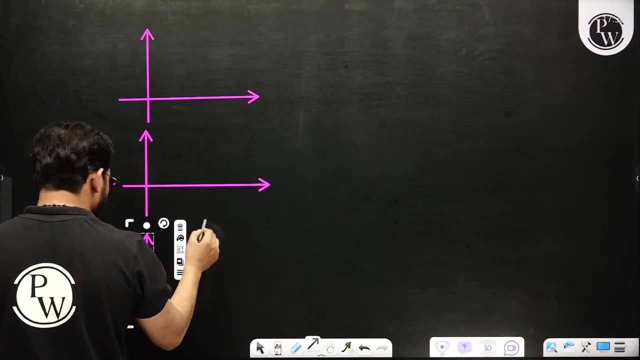 It works in entire swarm in CR, force and bending moment diagram. People can't understand. Three graphs to be made, Three graphs. So I will teach you from these three diagrams which I am showing you on the board. You just have to see these three graphs. 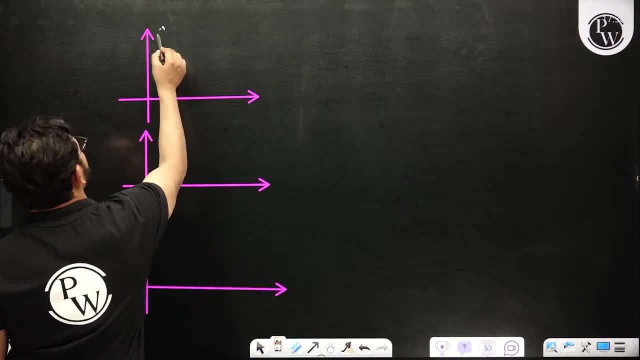 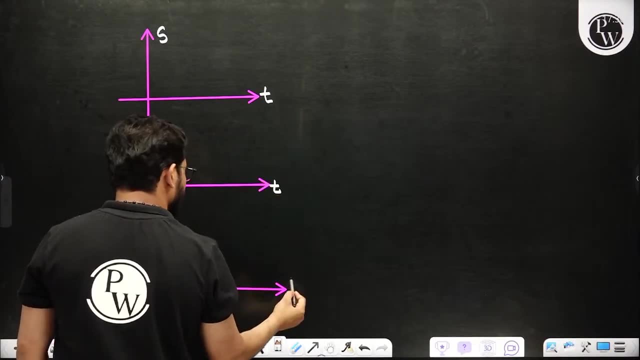 Here are the three graphs. Okay, First of all, who came Displacement, After that, who came Velocity? After that, who came Acceleration? And what is going on below everyone- Time, What is going on below everyone. 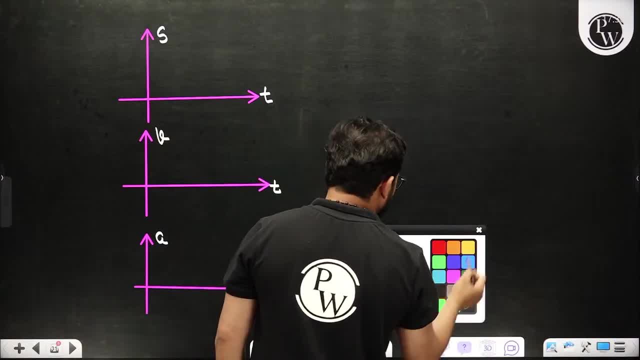 Time. What is going on below everyone Time? So just a little while ago you had told me one thing: What is the meaning of calculating slope dy upon dx? Tell me the slope of this, So tell me how much it became. 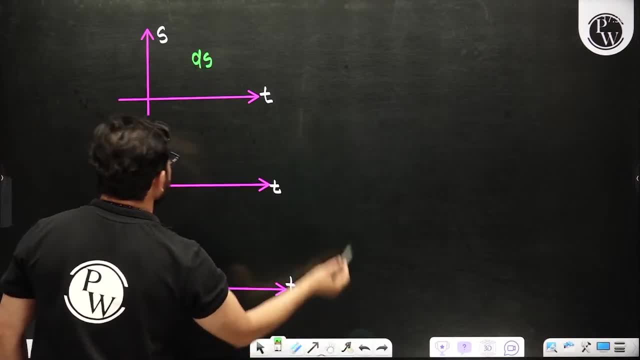 ds upon dt. This is the slope ds upon dt. Very good, Tell me its slope dv upon dt. What are you saying? I am writing absolutely right. So what are you seeing? Who is given the slope of the displacement versus of time graph? 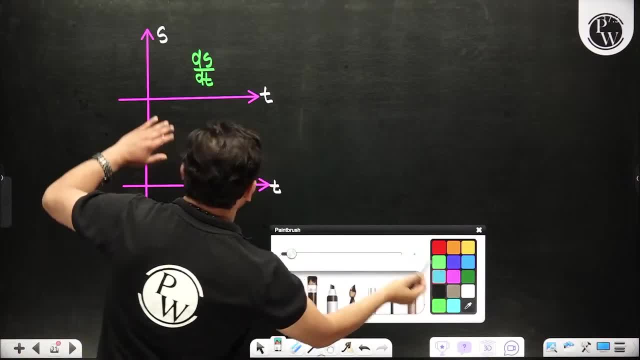 Velocity. If you don't believe, then check from the unit. What is the unit of displacement Meter? And second Time unit, Second. So meter per second becomes velocity. So who is given the slope of this graph? Velocity. 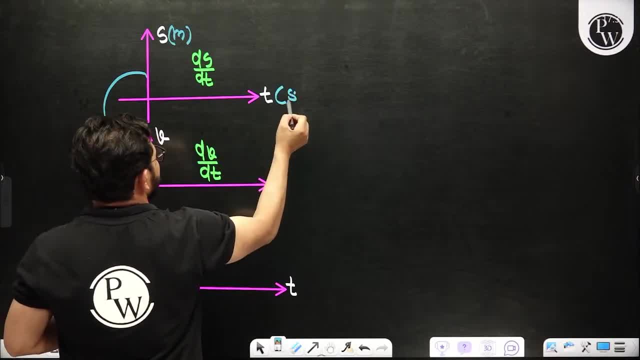 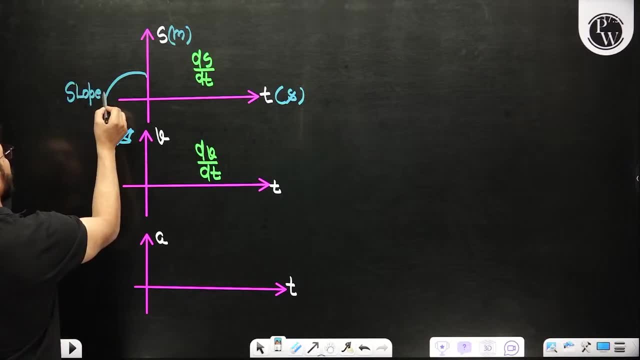 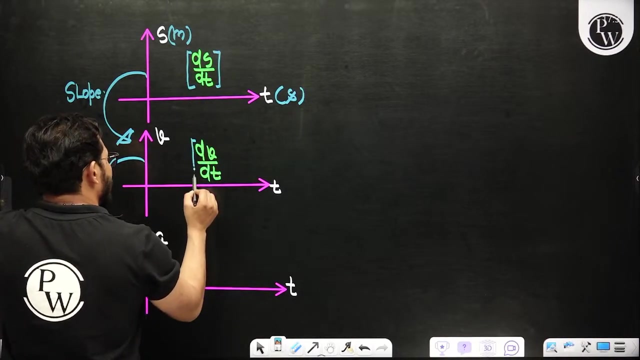 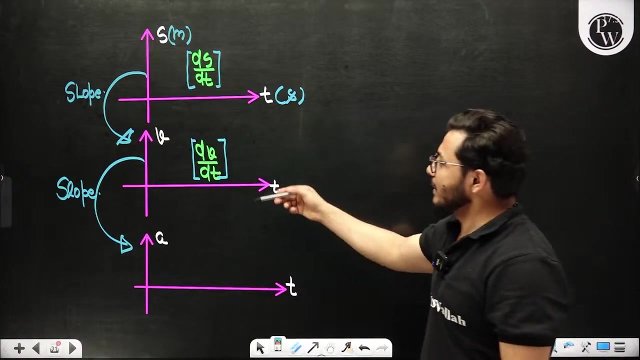 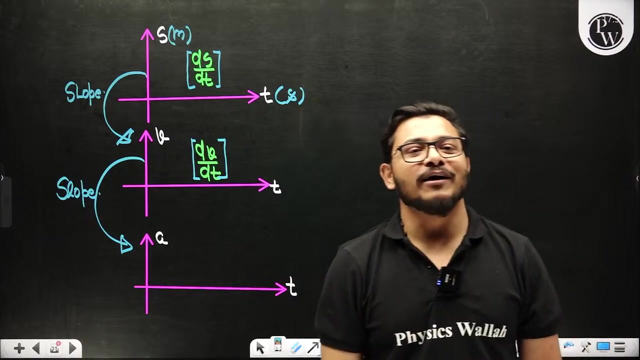 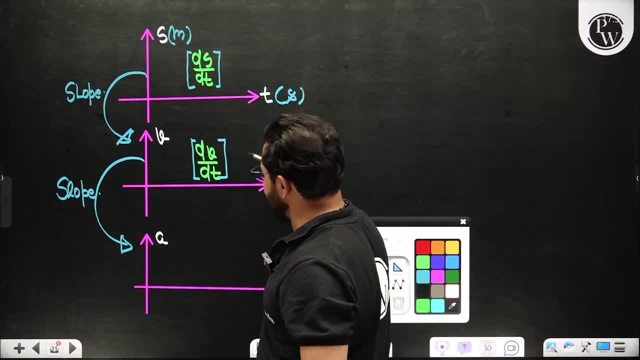 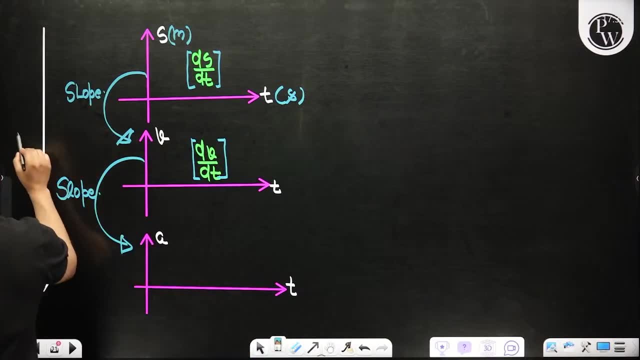 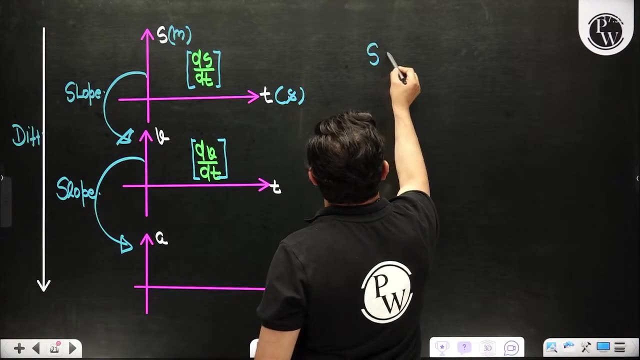 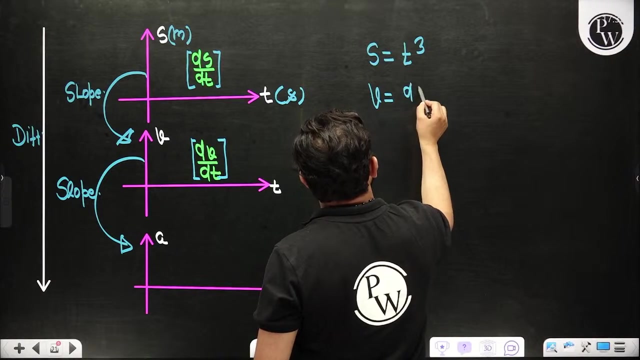 you are not doing differentiation, its differentiation velocity, its differentiation acceleration. so when you are coming down, my dear, what did you do? You did differentiation. okay, when you do differentiation of something, what happens in doing differentiation? Let me check and tell you. let's assume if, by chance, if it was like this, that displacement's power T depends on power 3, then I will ask you: do you know the velocity? how much it became? So what would you say? That, brother, do differentiation ds upon dT, then how much would it become 3T square? I said, man, I want acceleration. 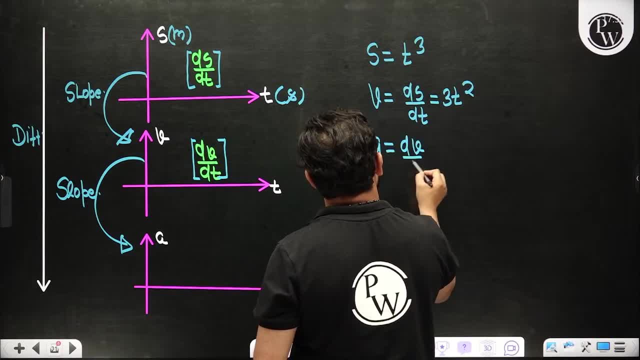 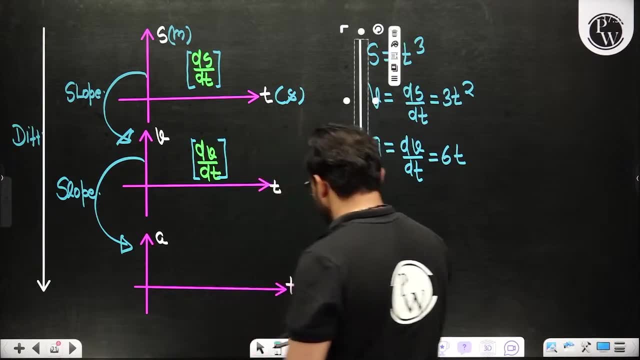 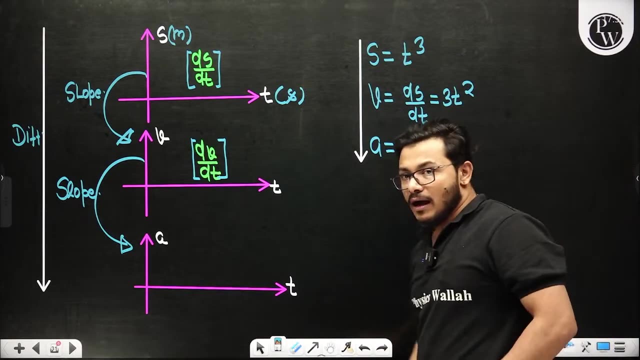 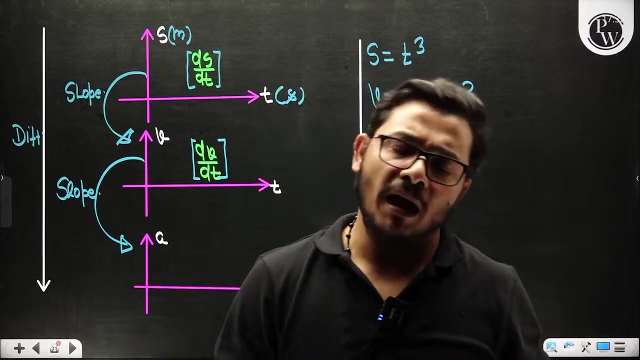 so what would you say Then? do differentiation, the dv upon dT. so how much? would you say 6T. so what are you seeing? As I went down, I kept doing differentiation. so differentiation means power is decreasing. see, first power was 3, then power 2 came, then power 1 came. so what are you seeing? If I ask you an objective question, if I ask you an objective question- and this objective question is very important, very important- if I ask you tell me if displacement versus of time's graph 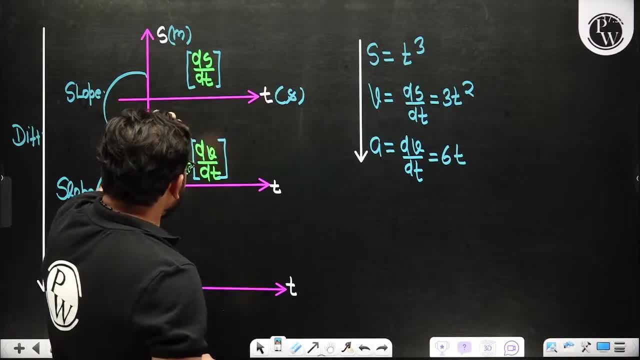 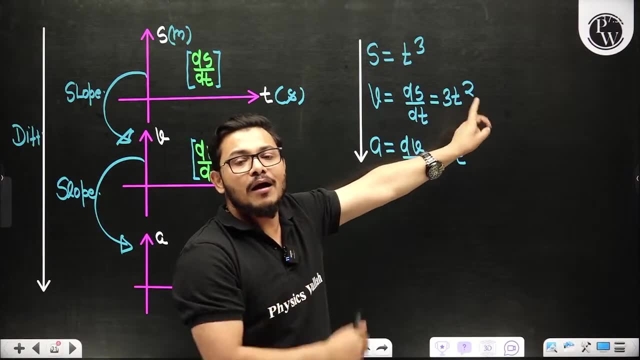 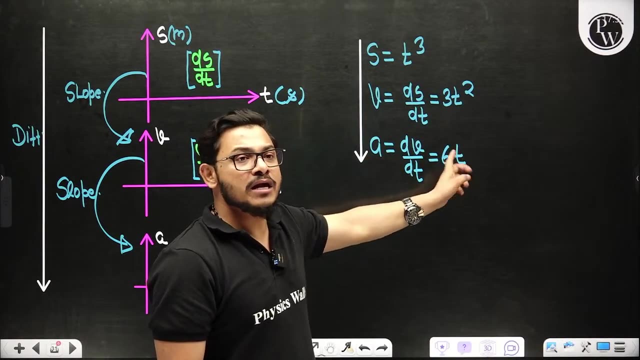 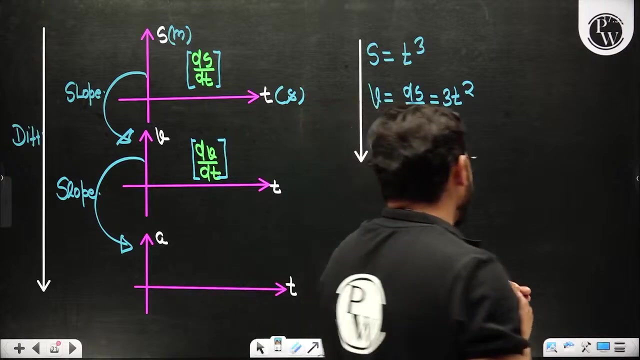 is a cubic graph. cubic means it depends on power 3, then tell me, how will the graph of velocity versus of time be made? So you say it will depend on power 2, power 2 means that it will be parabolic. power 2 means what? It will be parabolic. parabolic if I ask you what will be the value of acceleration? So you say it will be diagonal, because ab is equal to 60, so how will it be? Diagonal means acceleration will change with time, but it will be diagonal. so what I want to say? very good, very good. if I would say this to you in the question: 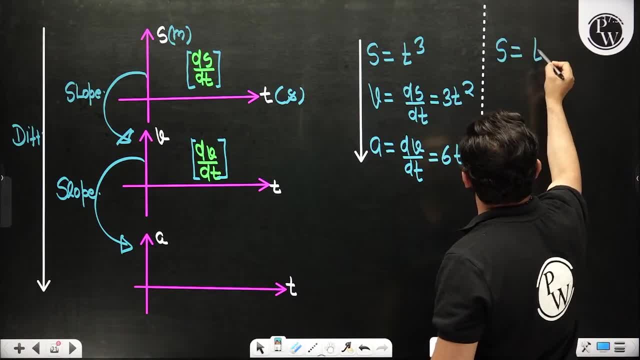 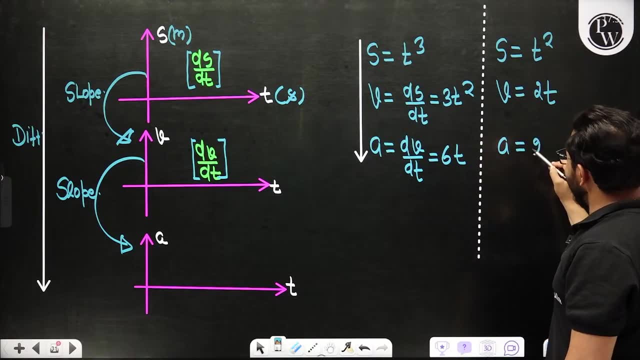 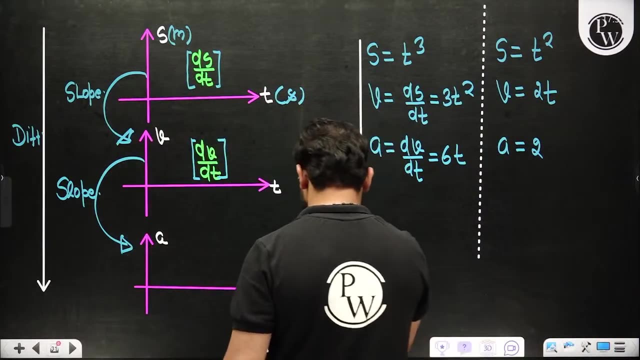 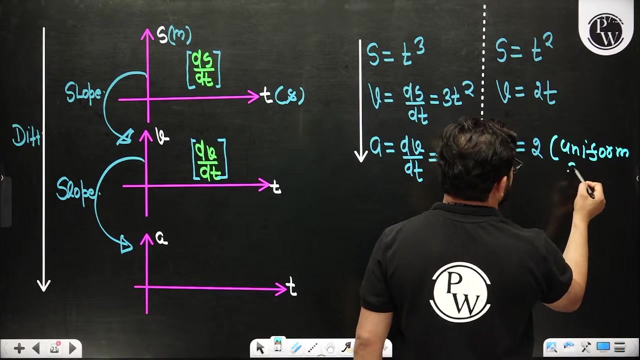 then ask me if the displacement value depends on the power of time, 2, so tell me how much is the velocity? if 2 would be, tell me acceleration, how much would be turned into 2?? Is this acceleration changing with time? My turn, tell me what is the change with time. this acceleration is constant. if the acceleration is constant, then they will say that it will be called a uniform acceleration. What will you say? uniform acceleration? what will you say uniform acceleration? this here is a uniform acceleration. then tell me one thing. 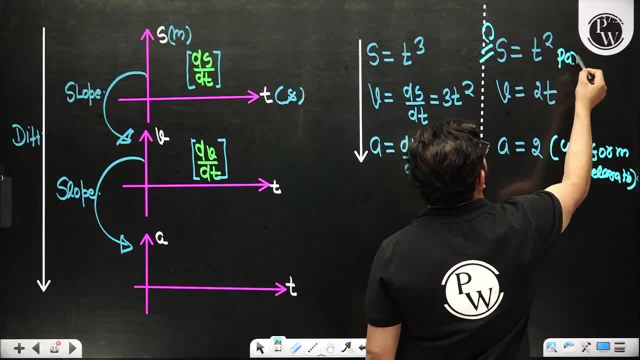 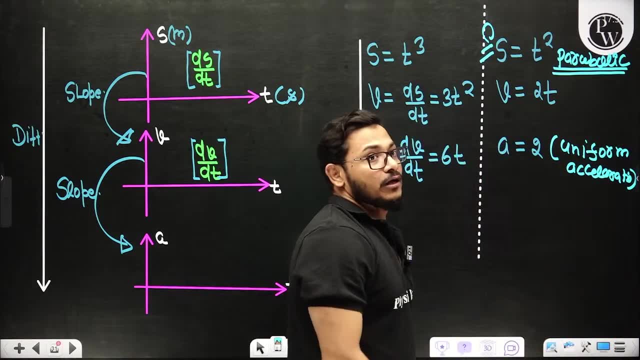 What is the graph of displacement Parabolic? What is the graph Parabolic? So how many times do you get asked in examination that who is called parabolic motion? So you say parabolic motion is called uniform acceleration. 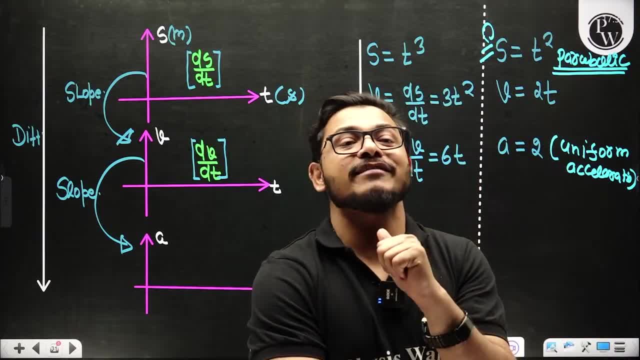 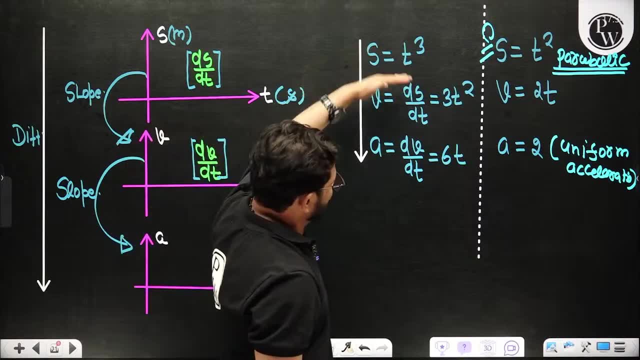 What an amazing thing. Parabolic motion means uniform acceleration. Don't do anything parabolic. keep doing differentiation. It is a simple thing. So what should I tell you? When you are moving downwards, you are reducing the power, And when you move upwards, what will you do to the power? 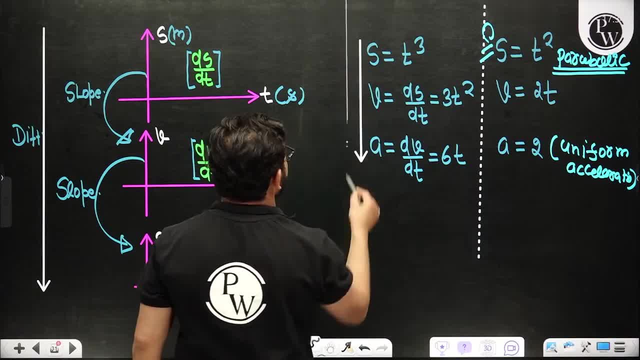 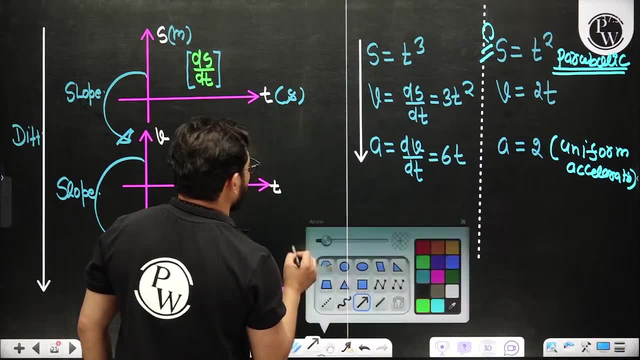 You will increase it. You will have to increase the power. It is a simple thing: When you are moving downwards, you are reducing the power. When you move upwards, what will you do? Move upwards? When you move upwards, what will you do to the power? 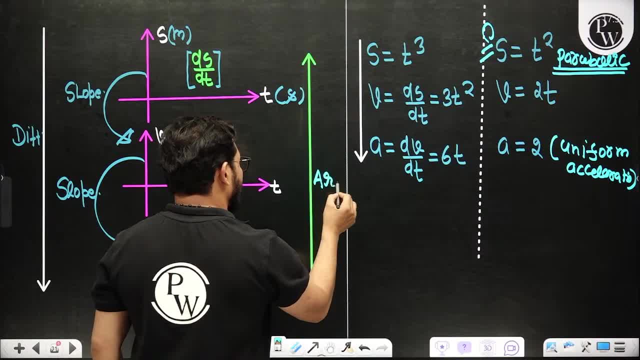 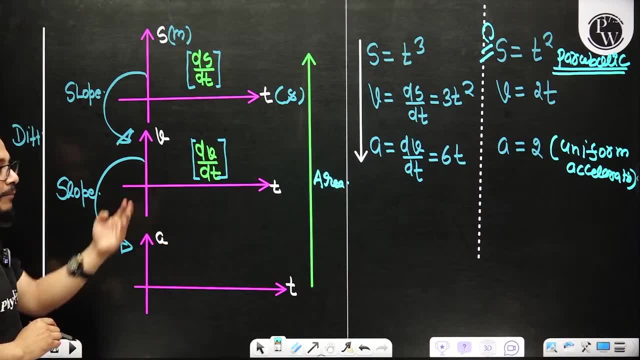 You will increase it Upwards. power means calculating the area Area. So you will understand what I said again. What did I say? When you moved downwards, you calculated the slope. When you moved upwards, you calculated the area. What does it mean? 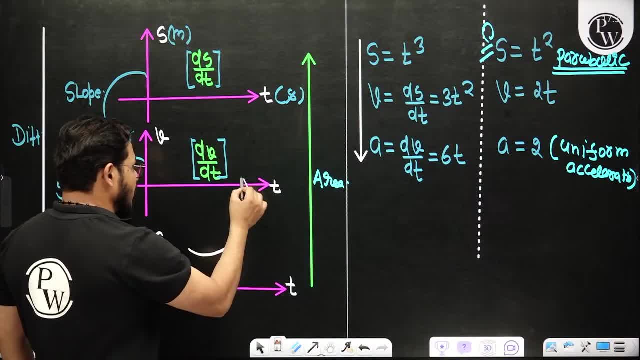 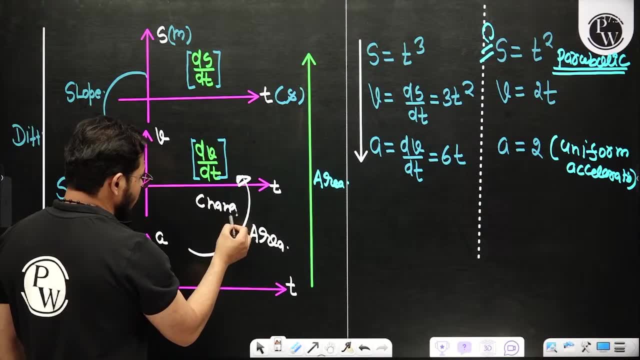 If someone asks you, what does the area of acceleration versus of time give you? So what will you say? The area of this graph will give you the change in velocity. Who will it give Change in velocity? What an amazing thing you are writing. 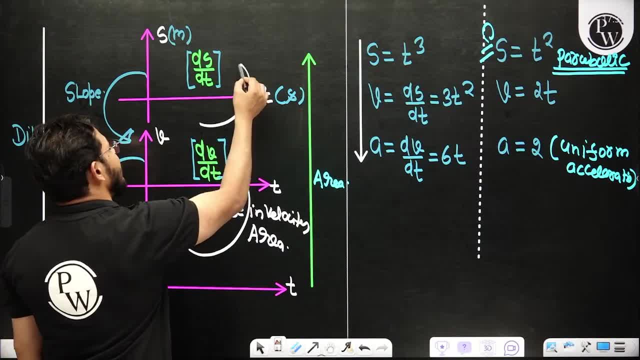 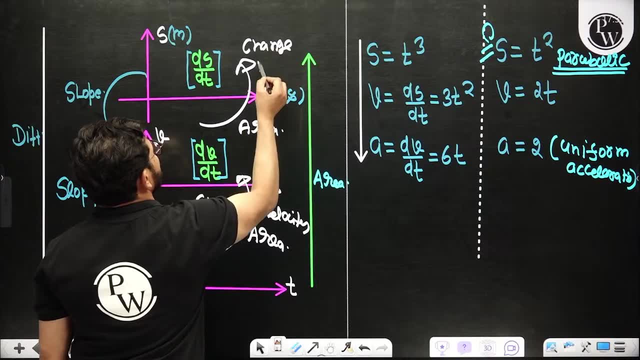 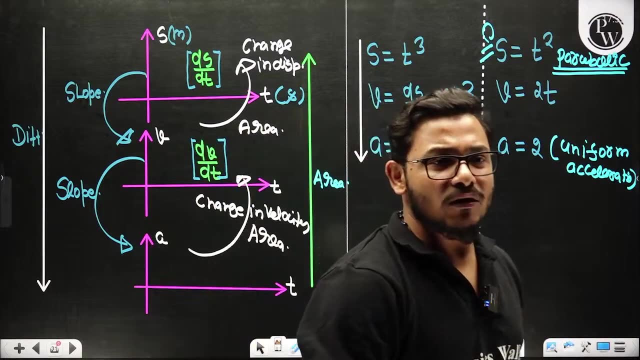 Very good. Okay, what will the area of velocity versus of time give you? What will the area of this graph give you? The change in displacement? Very good, Change in displacement. What an amazing thing you have written. When you move downwards, you have to calculate the area. 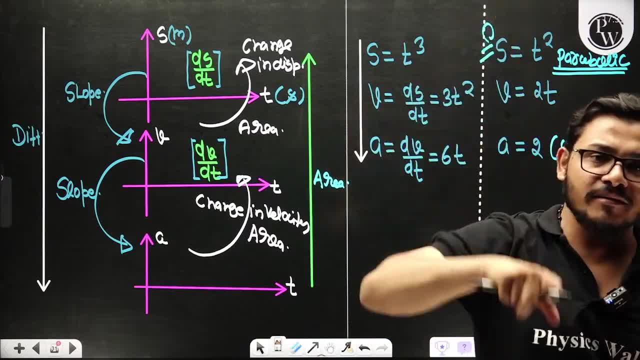 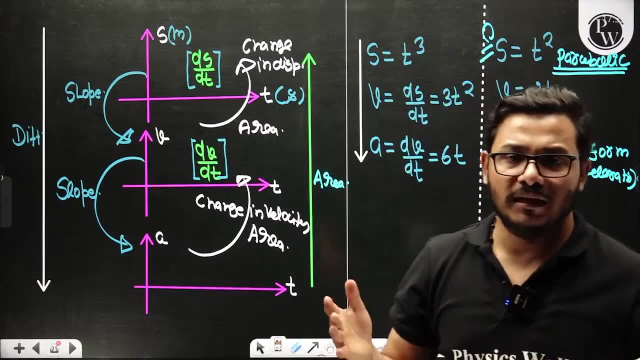 And when you move upwards you have to calculate the area. When you move downwards, you have to calculate the slope. You have to do differentiation. When you move upwards, you have to calculate the area, You have to do Intrication. You have told a wonderful thing. 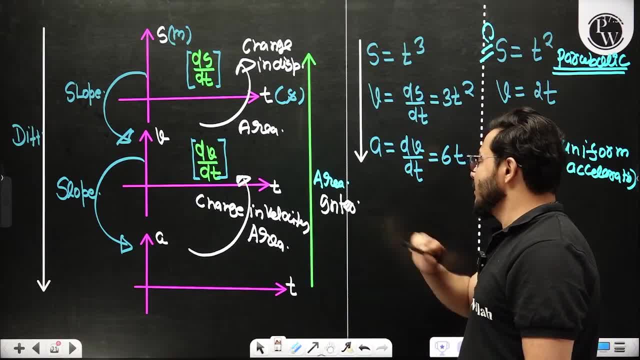 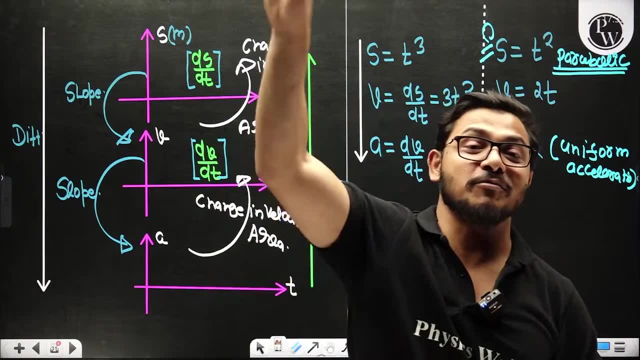 You have to do Intrication. Now you are seeing how questions are asked in examination. What does the area of that graph give you? What will that area give you? These are amazing questions. Shall I write a question and give you? 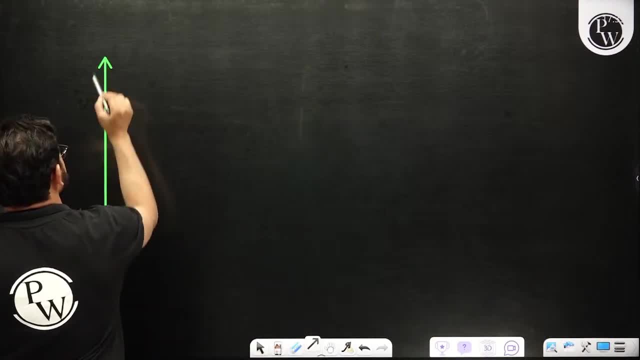 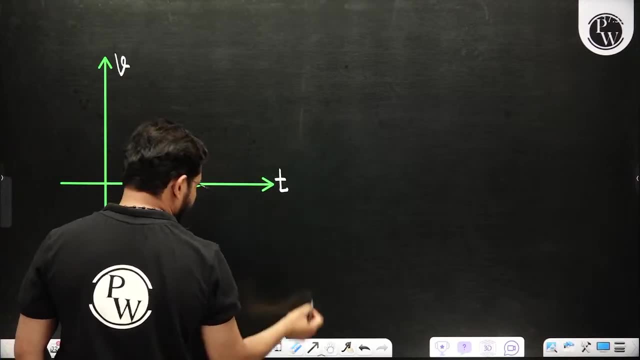 I am asking you in the question, the acceleration Is asking about acceleration. right, We have given a graphs of Velocity versus of time In question. he is asking: What is the acceleration value? Tell me Fast, what is the acceleration value. He asks about acceleration value. 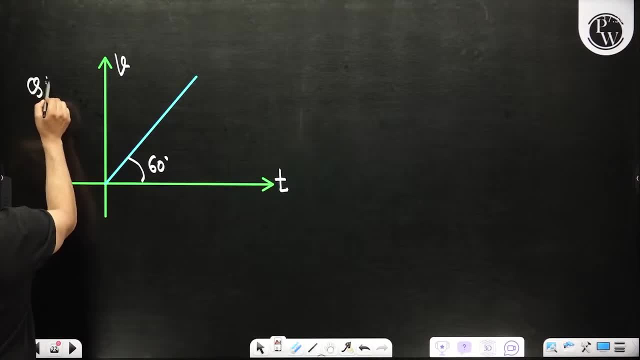 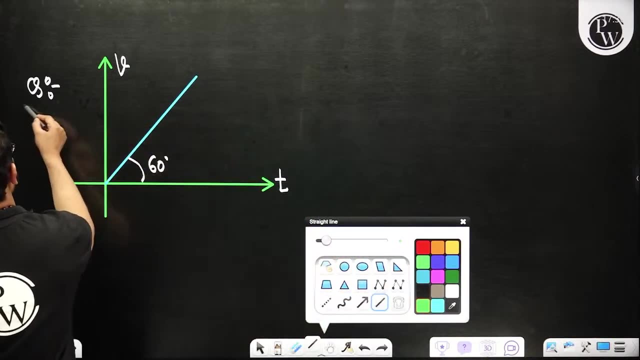 Ok, tell with the question, He is asking about acceleration value and He is asking you about, On observing this graph also- that how the curve graph of displacement versus of time will be made and how the graph of acceleration versus of time will be made. both are asking. 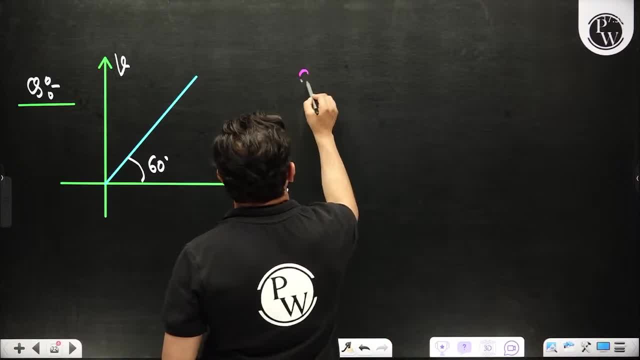 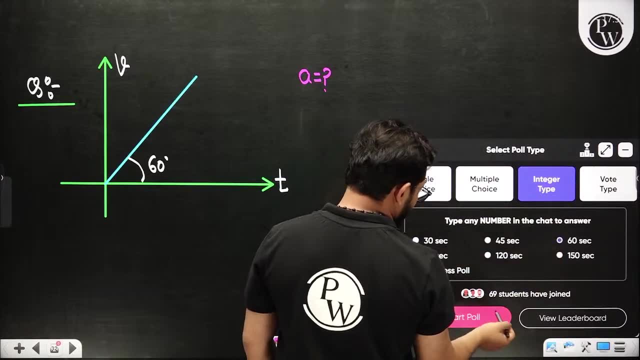 first question is that: how much will be the value of acceleration? quickly type: should I give you integer type question? ok, take it, I will give you integer type question. I am giving time of 60 seconds. tell me the answer. it is numerical value. tell me the value of acceleration. 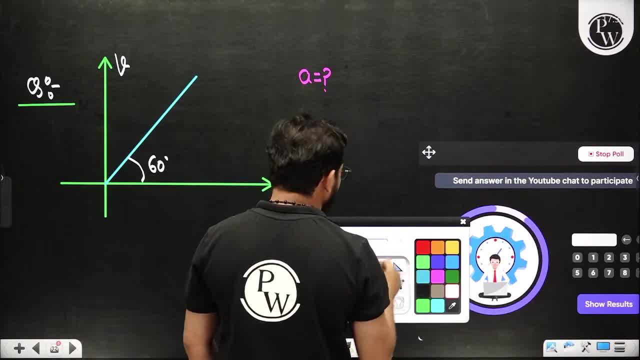 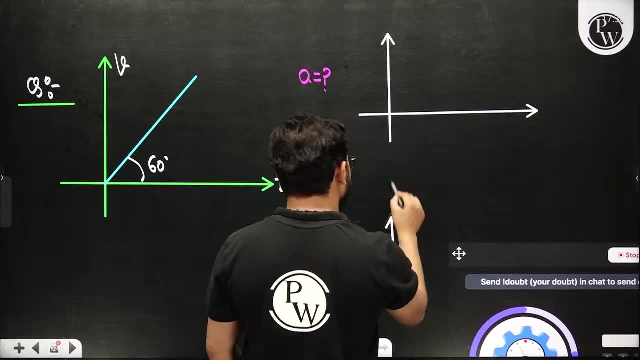 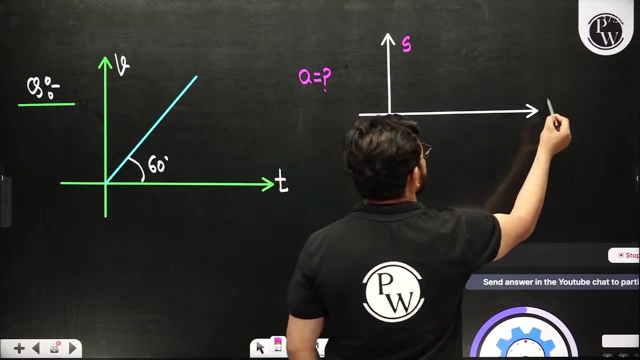 first question. second question is: second question: is that how the graph of displacement versus of time will be made. its shape is also asked in the next question. it is asking you that how will be the shape of graph of acceleration versus of time? asking all things, how will the shape of displacement versus of time be made? 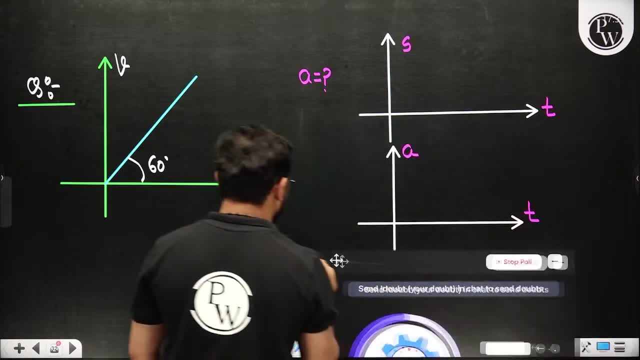 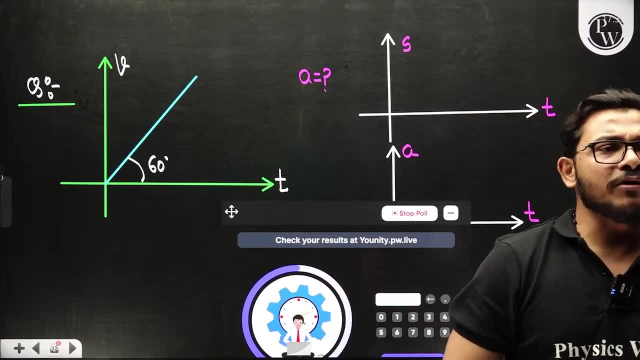 and how will be the shape of acceleration versus of time be made? come on, tell me fast how much answer would be. all of you type quick answer. be quick in typing the answer. where did you fall asleep? type the answer. all of you sitting over here. you can write. 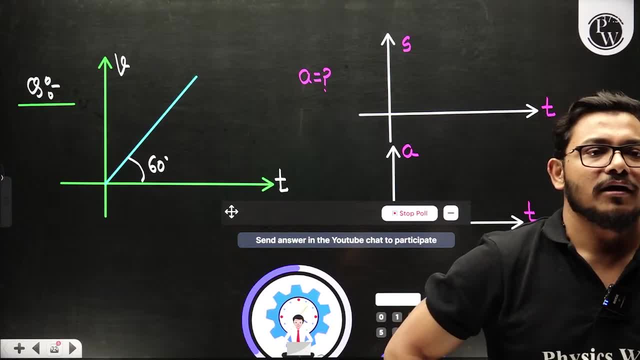 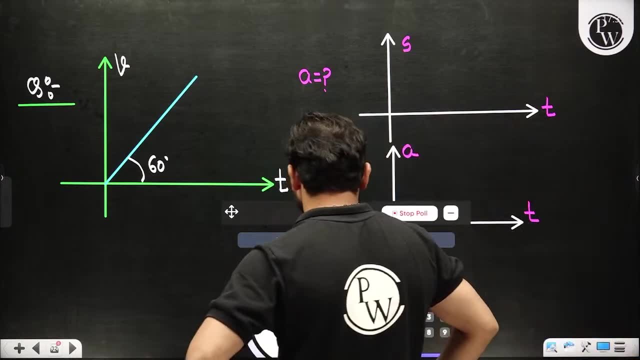 Yuvraj Aadil, Asit Haldar, Aditya Patel, Chaudhary Saab, Ravi Kumar- All the kids' answers are the same. Very good, Listen please one minute. Yes, you keep doing it please. 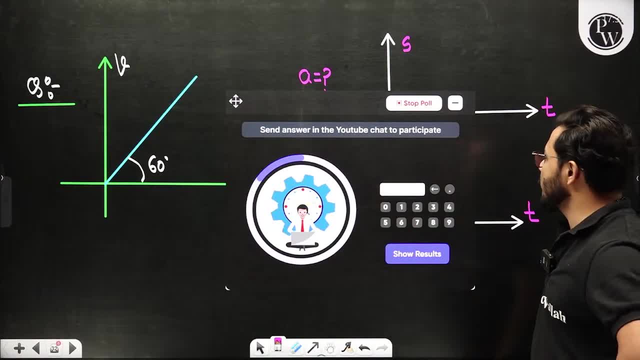 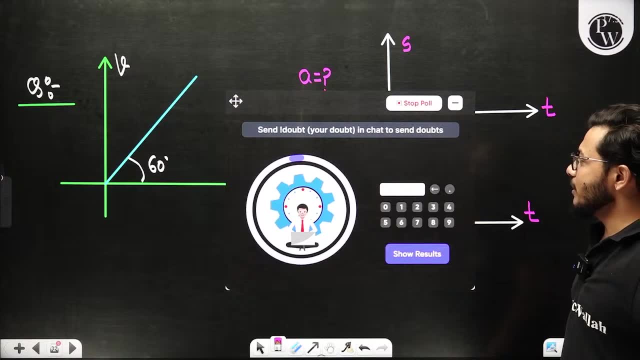 I am doing it And check your result at unitypw app. Send answer in the YouTube chat to the participant And participate. Very good, If I talk about the answer to this question, then I will tell you the answer to this question. 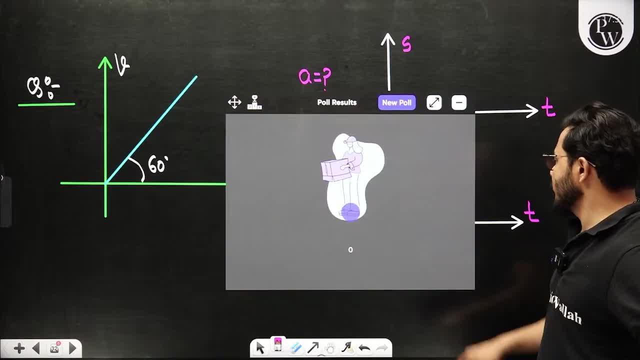 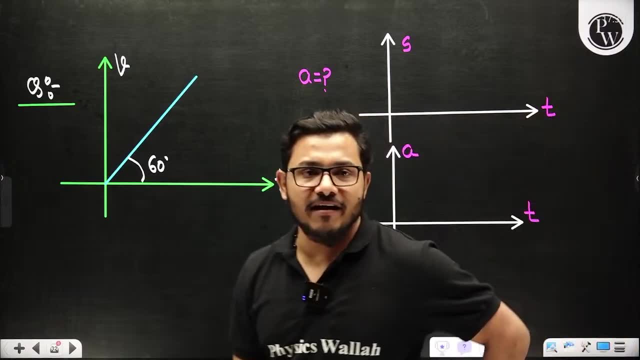 1.732.. 1.732 answer will come, So the correct answer has not come yet. Okay, you have typed it as it is. Okay, no problem. Acceleration value: Yes, please just look for one minute. 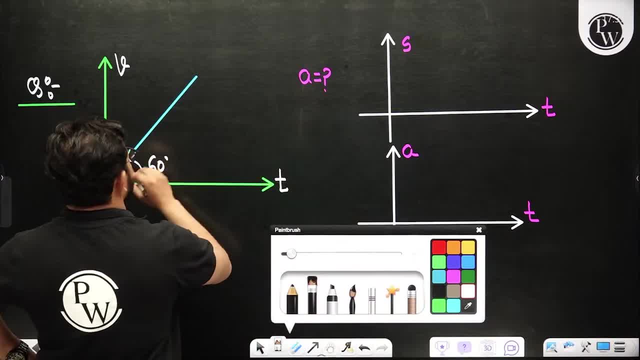 Can I ask you one thing? Will any kid tell me one thing? Tell me one thing anyway. This graph is a line, right? Line means how much does velocity depend on the power of time? It depends on 1,, right. 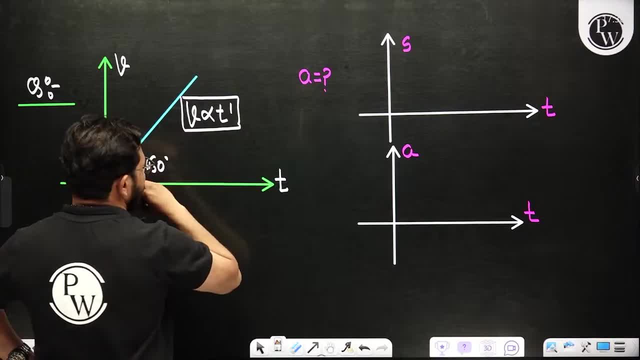 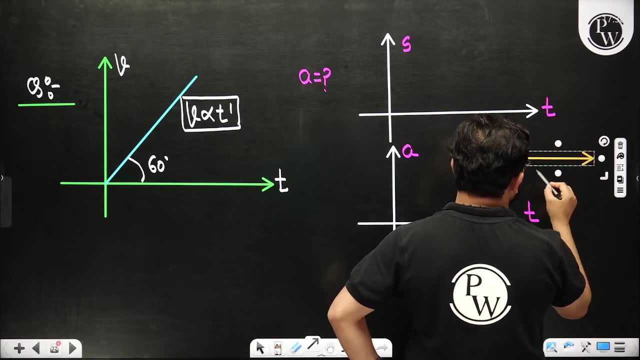 How much does velocity depend on the power of time? It depends on 1.. So look, I told you the sequence of three graphs. Velocity was between these two right. Remember? velocity was between these two. Exactly, Velocity was between these two right. 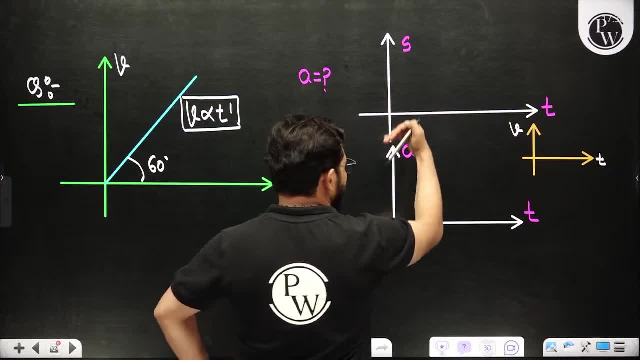 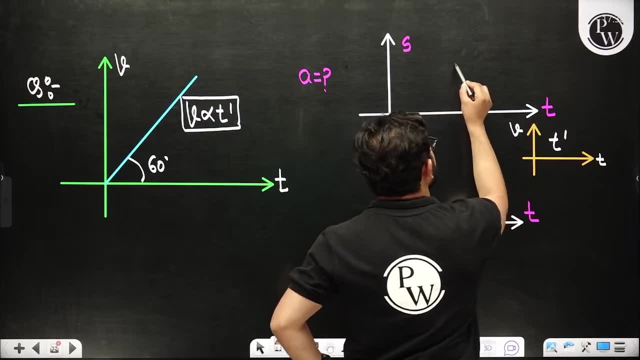 Very good. Velocity was between these two. When it comes down, we reduce the power, Remember, And when it goes up, we increase the power. If velocity depends on the power of time, then how much will this time's power depend on? 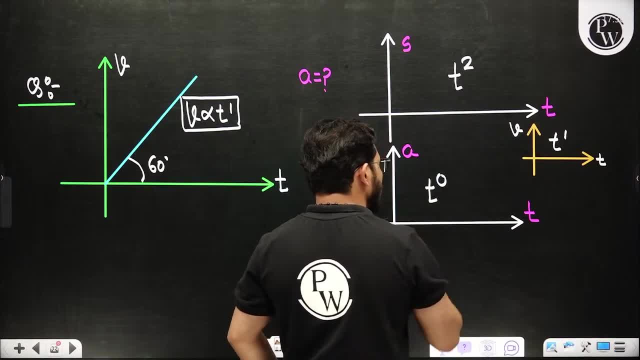 On 2.. So how much will acceleration depend on? On time's power? 0.. What does time's power depend on? What does time's power depend on? What does time's power depend on? It means to be constant. 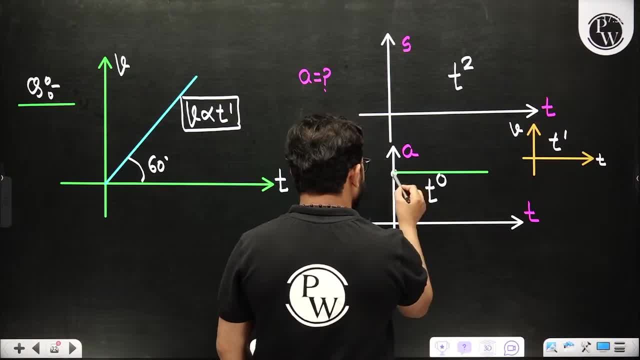 Like this, Like this, Like this, Because this value should never change with time. So this is the graph. Okay, The power of time should depend on 0.. The power of time should depend on 2 means to be parabolic. 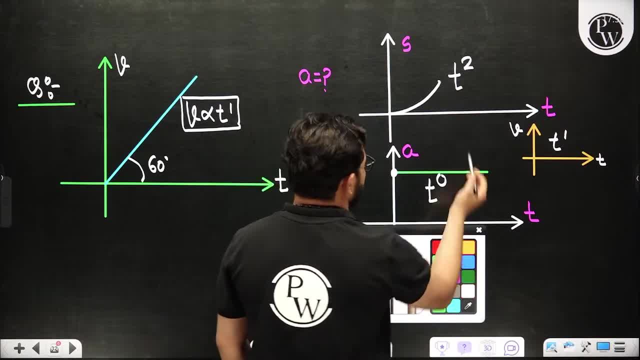 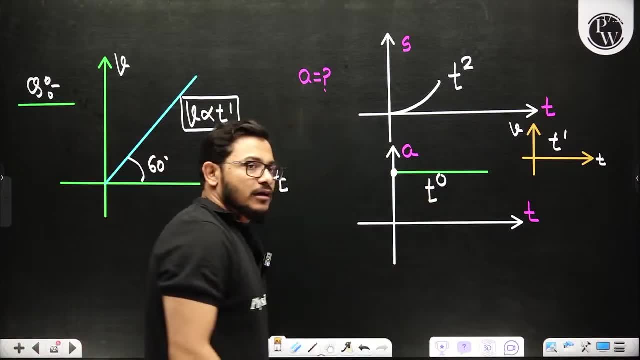 By doing this to become parabolic, To become parabolic. So what you are seeing is a parabolic graph. This is in the form of triangular And this graph is in the form of rectangular. How many children are there who have got the answer to this question? 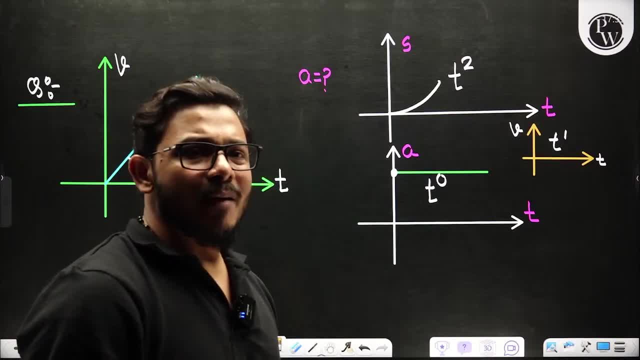 Acceleration parabolic. Are you crazy? Why will acceleration be parabolic? Now he will differentiate. What are you talking about? How can you make acceleration's value parabolic? Right now you are saying the answer is 1.732.. 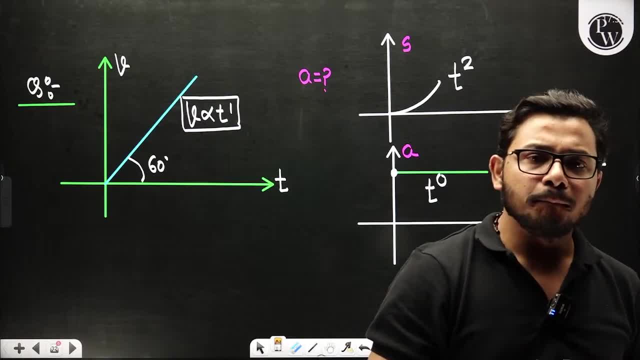 So it is constant. So why is it parabolic? Why will it be parabolic? Why will it be parabolic? That will be constant, Displacement versus of time will be parabolic And acceleration versus of time will be horizontal. 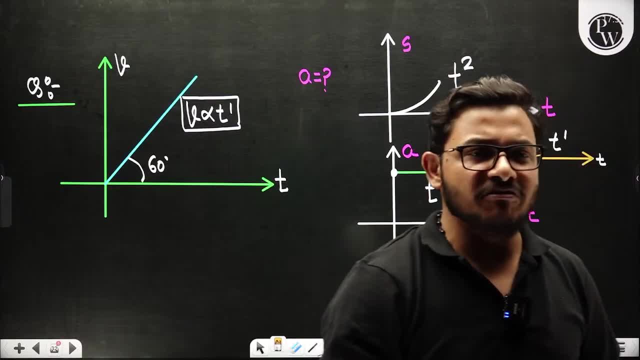 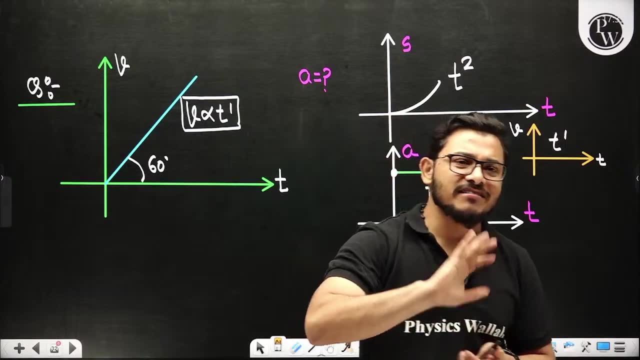 It will be constant. The talk is over. Displacement versus of time will be parabolic. Did you understand anything? Tell me quickly: All the children. did you understand my question to everyone? How many children are understanding the concept of such questions? 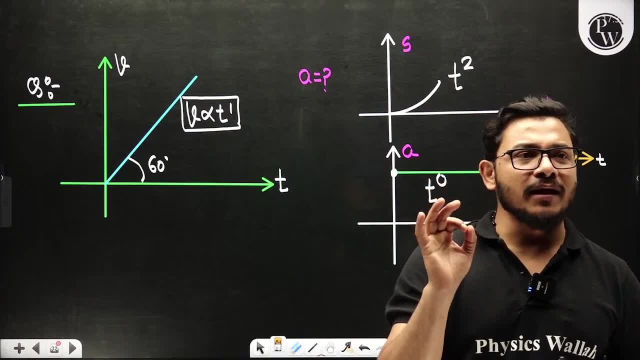 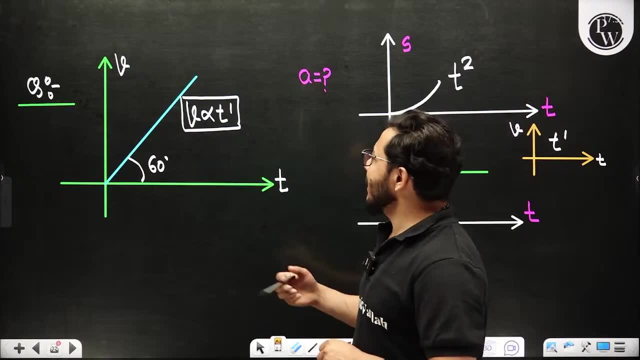 Did you understand? I hope you got the concept. Are the things clear? Is it fine? No problem, No problem, No problem. Some kid will tell that the motion I have written here. What is this motion? S's value depends on time's power. 2. 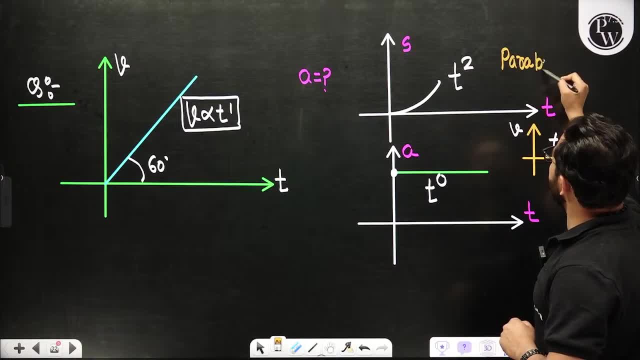 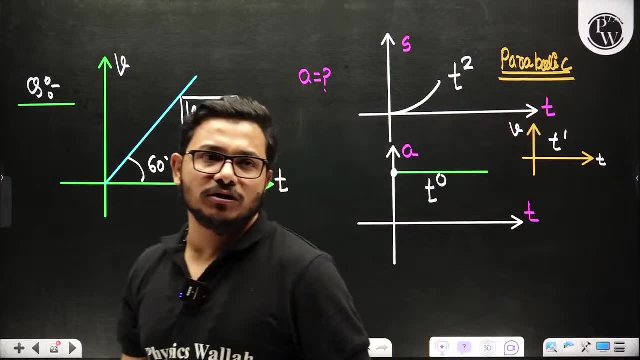 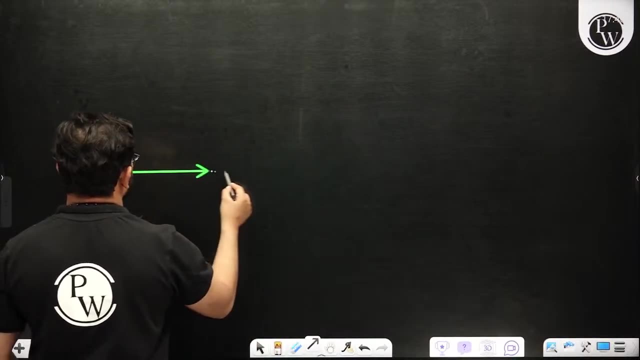 So what is this motion Parabolic? What is this motion Parabolic? Please remember: Never get deceived in life. That one is parabolic motion. That one is parabolic motion. This is parabolic motion. Let's do the question again. Okay, here is the question. 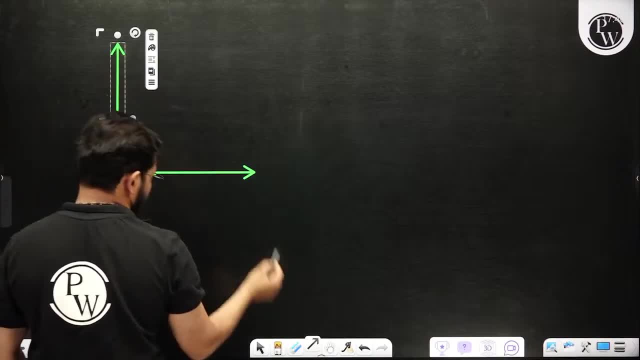 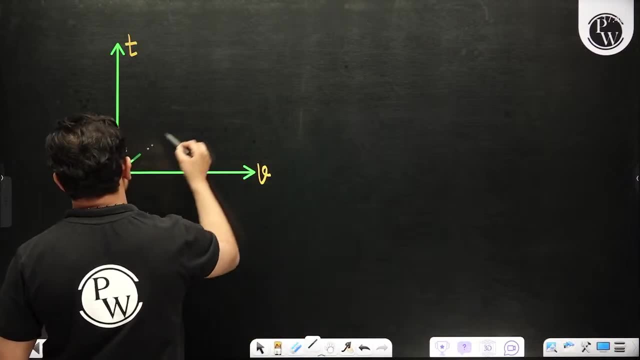 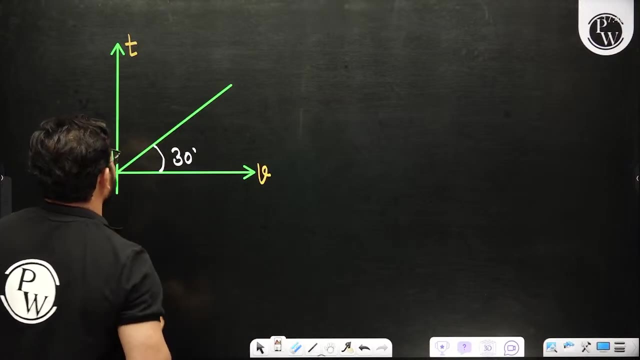 This was the question for you. In the question I am asking you: What will be the value of the acceleration? The value of acceleration is asked. Tell me the answer of the question. The value of acceleration is being asked. What will be the value of the acceleration? 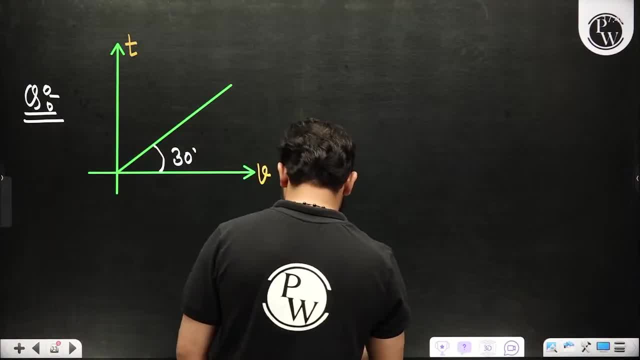 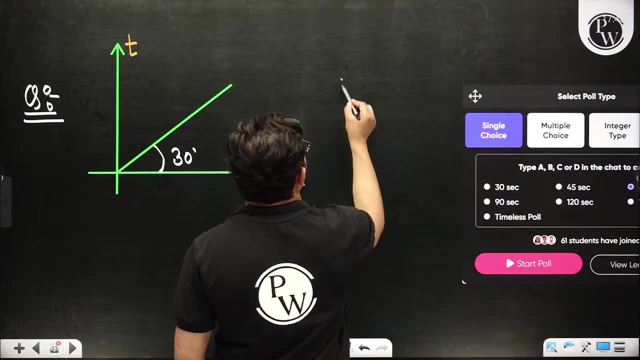 The value of acceleration is asked. Alright, Do you know the value of acceleration? Let me write one thing here. Listen to me. Let me tell you one thing: The value of root 3 is 1.732 and the value of root 2. 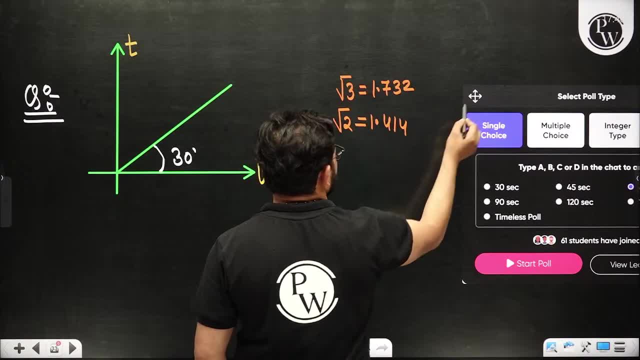 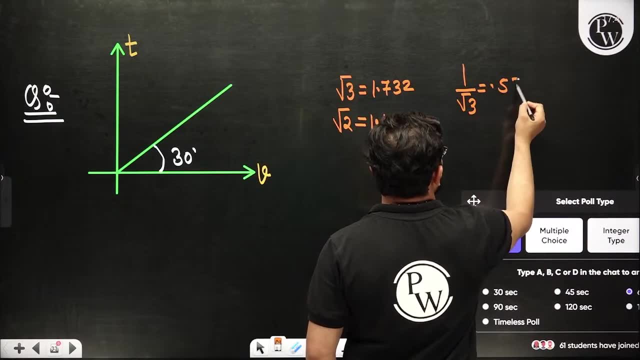 is 1.414. Let's talk about the next one. The value of 1 by root 3 is 0.577 and the value of root 2 is 0.707.. Remember that Now you can tell me the answer. 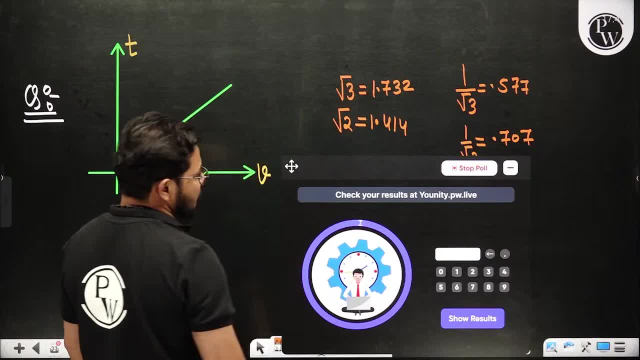 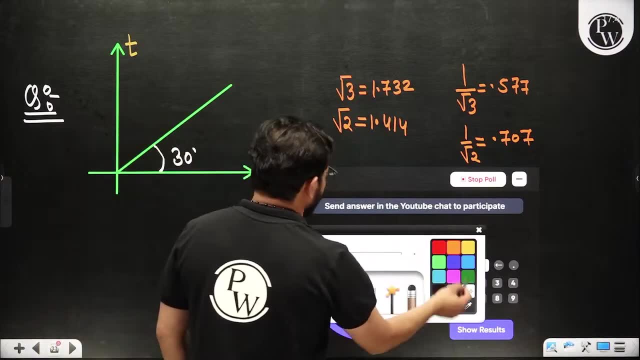 It is an integer type question. I will give you 45 seconds. Please tell me the answer quickly. So please tell me what will be the answer. You have to remember this value. Please don't get tensed. You have to remember this value. 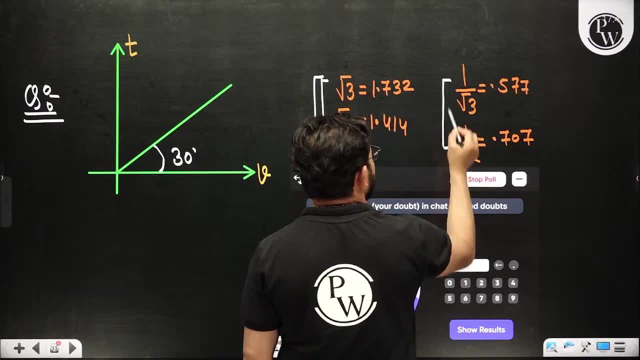 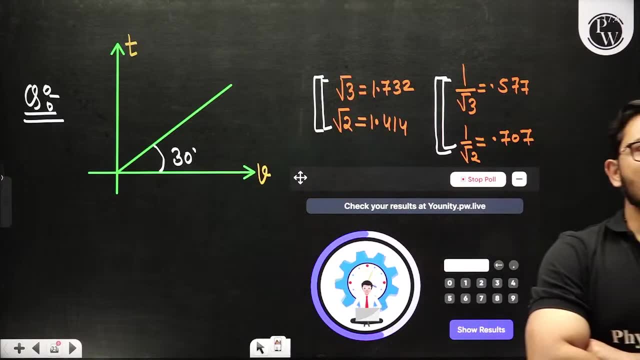 What is the value of root 3 and root 2?? I think 1 by root 3 is 0.57.. It is less than 0.577.. Very good, Write the answer quickly. All of you write the answer quickly. 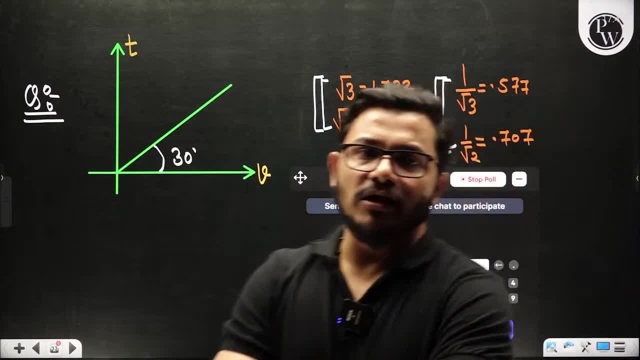 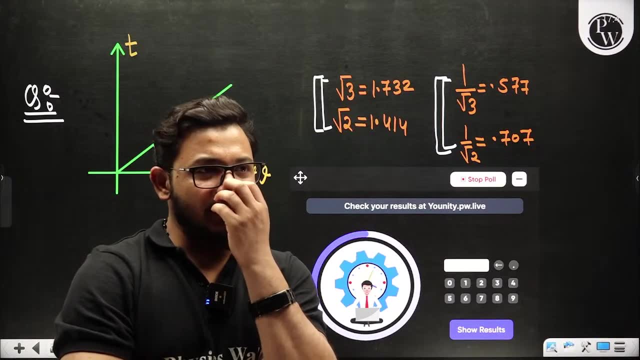 The answer is 1 by root 3.. All of you write the answer quickly. I don't have any problem. Write the answer quickly. All of you write the answer quickly. I don't have any problem. Write the answer quickly. All have good answers. 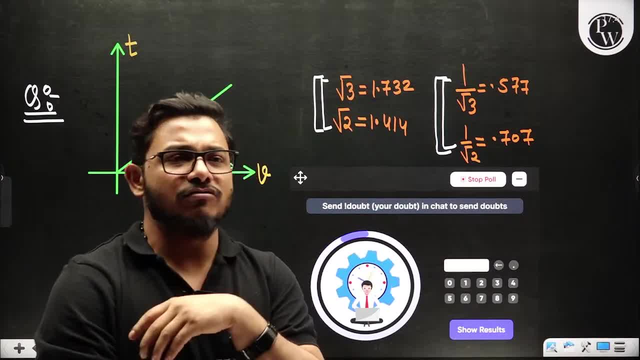 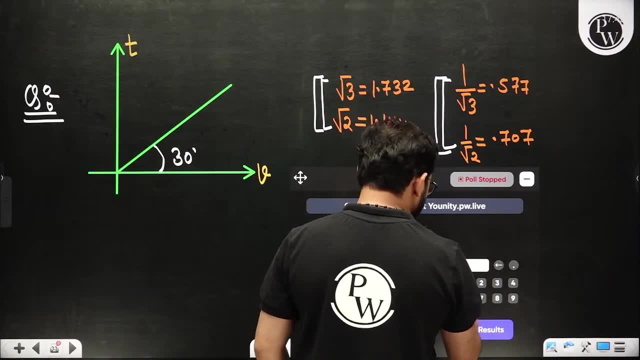 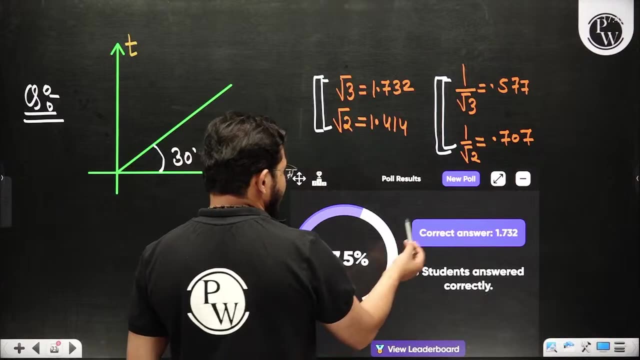 Write the answer quickly. Listen to me Now, I will check your answer. This question's answer is 1.732.. This is a 1.732 answer. Listen to me Now, you will tell me one thing: three students answered correctly. no one else answered. 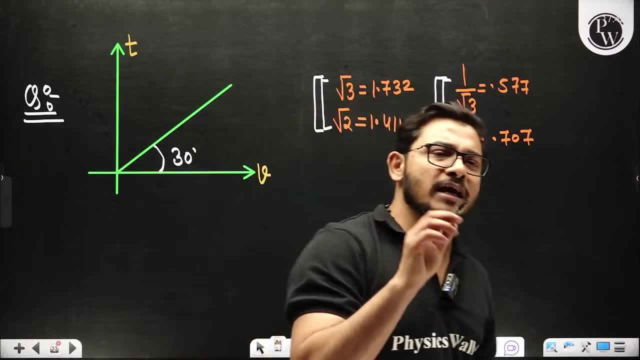 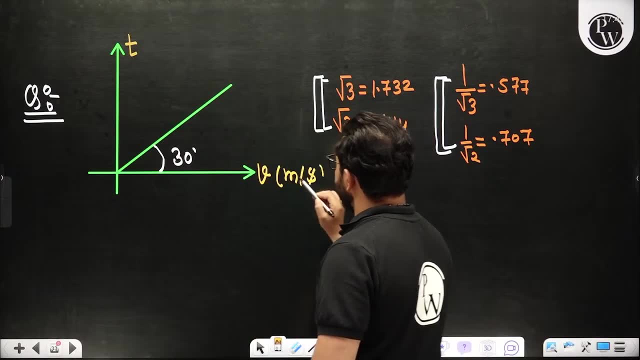 Listen to me, tell me how acceleration is made. This is meter per second and this is second. Will any child tell you how acceleration is made? Acceleration is made when there is time in velocity upon, Now, when there is time in velocity upon, then there is velocity above. 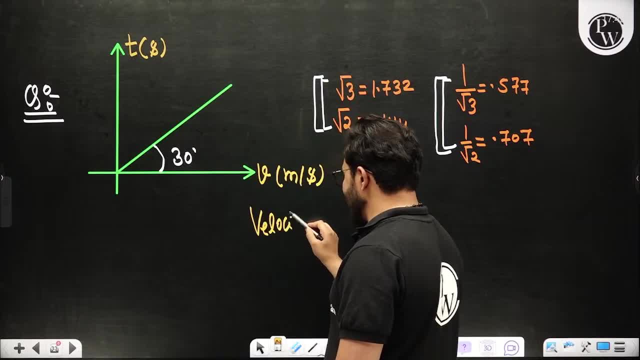 What is above, There is velocity And what is below, There is time. So what did you consider as base Base? You considered base as time. So remember, in life, whenever you calculate angle in kinematics, then calculate with time axis. 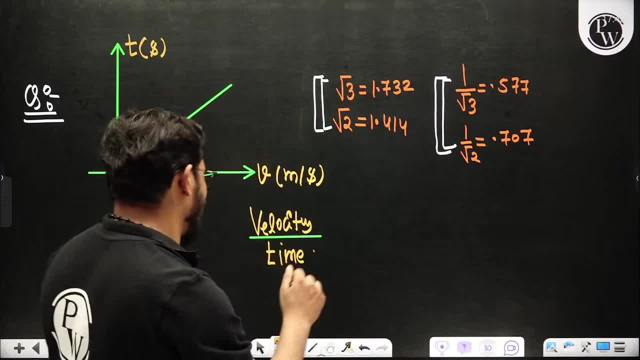 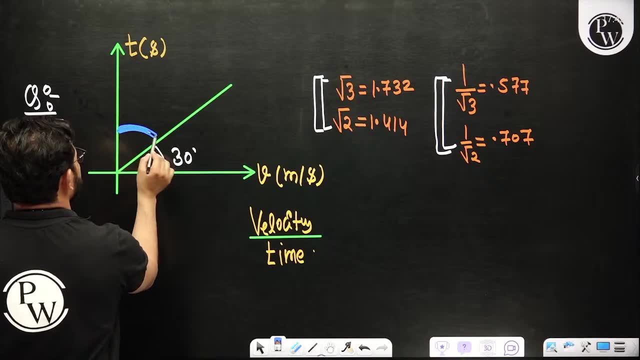 With whom to calculate, With time axis. So the angle which you have made with time axis- I think you have made this angle- You open your eyes and see. God has given you very big eyes. You have given this angle 30 degree velocity. 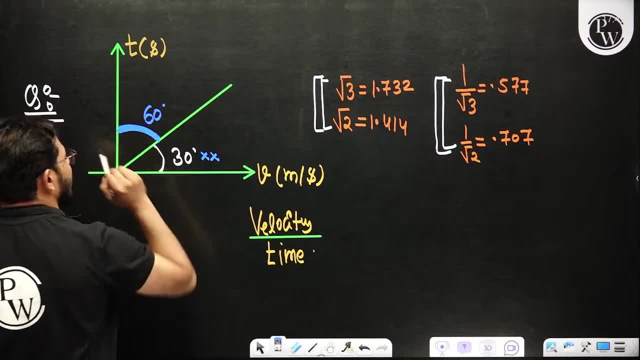 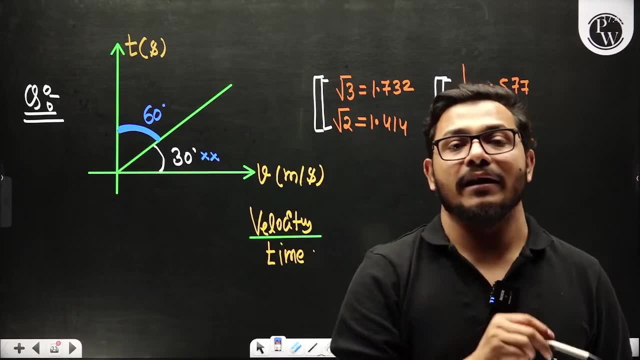 You have measured with velocity, You will not take this angle. You will have to take this angle: 60 degree angle. Why will you have to take 60 degree angle? Because you have to consider base as time, And this question is the problem of your examination. 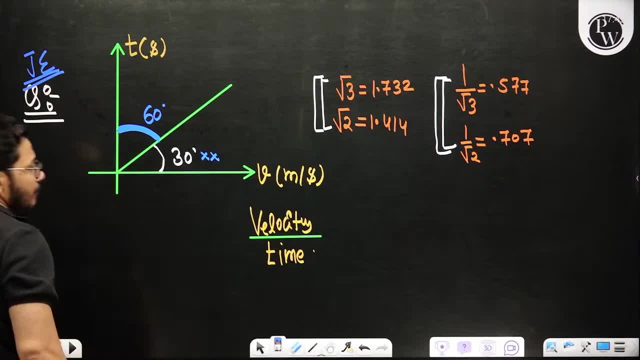 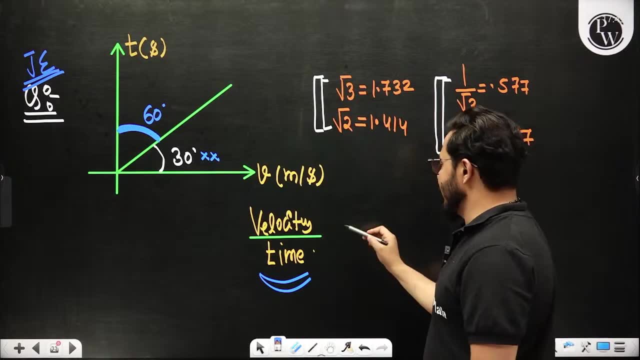 This is the question of JEE. Now, I knew that this is what people do, which I know, So you understand one thing: Put a little mind: Whenever you calculate angle, considering time as base, then that angle is still 60 degree. 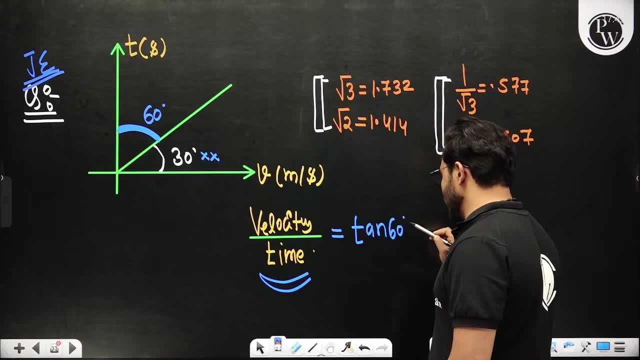 So that one is become is equal to 10 of 60 degree. So the value of 10 of 60 degree will still be the same as it was before, And that was already root 3.. So that one is the answer. So this was the graph of time versus of V. 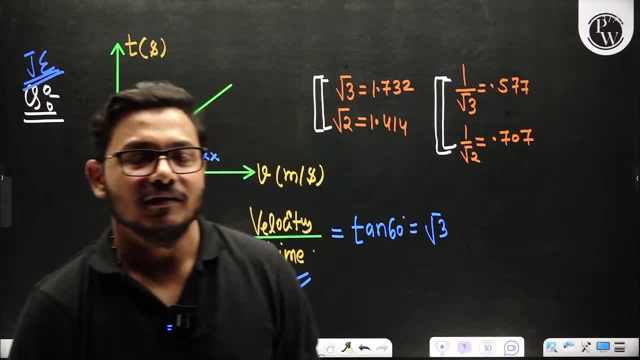 So you have to take the angle from above. So the value of 10 of 60 degree is the same as root 3.. So the answer of that one problem becomes is equal to 1.732.. So what did I tell you after the lesson? 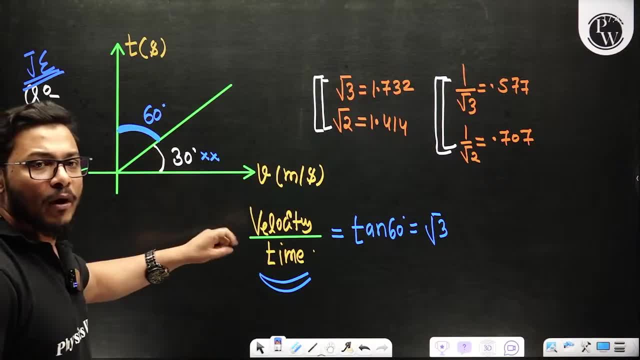 You got the concept, So in this way you can solve all the questions in kinematics. So this is the end of the video. Thank you very much. See you in the next video. Bye, bye, Bye, Bye, Bye, Bye. 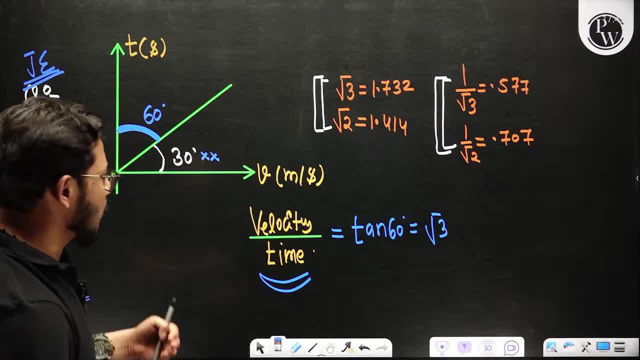 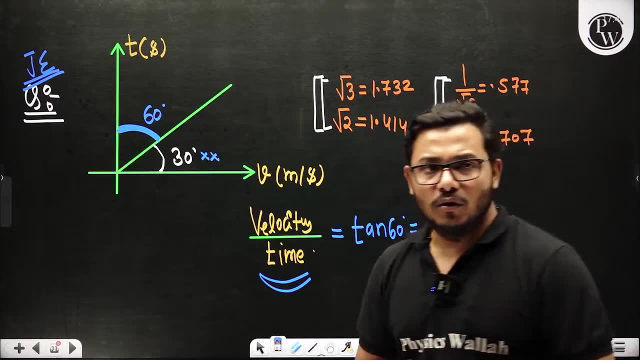 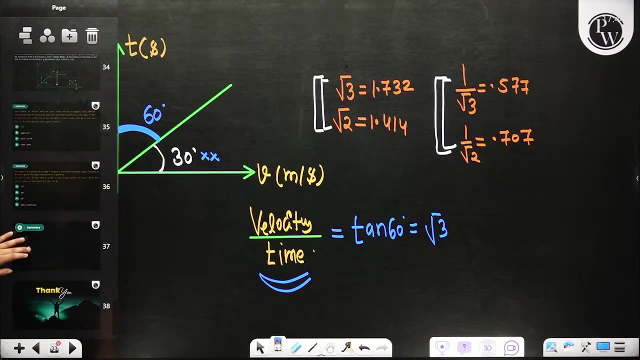 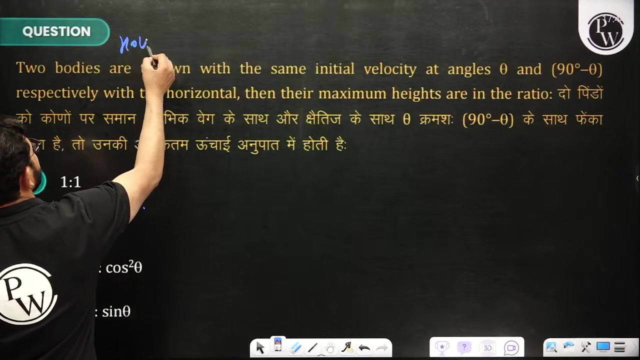 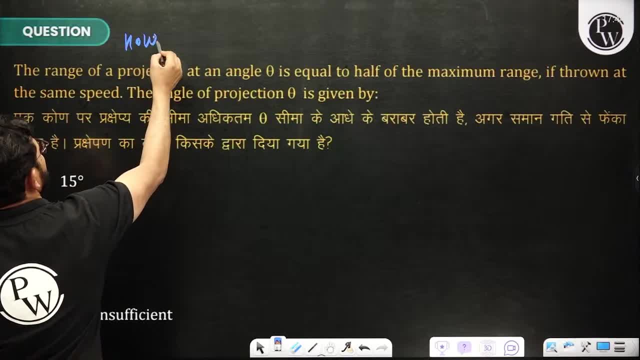 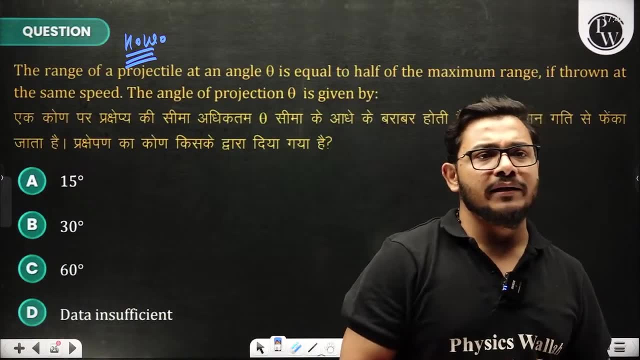 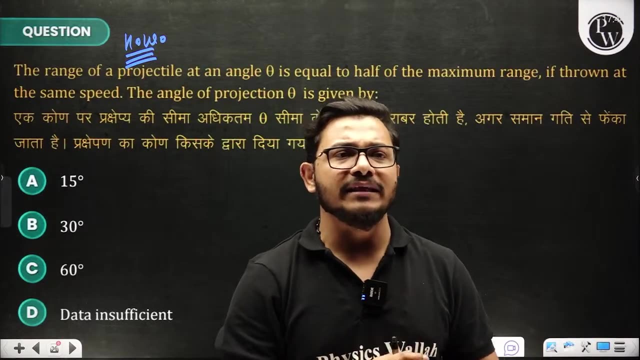 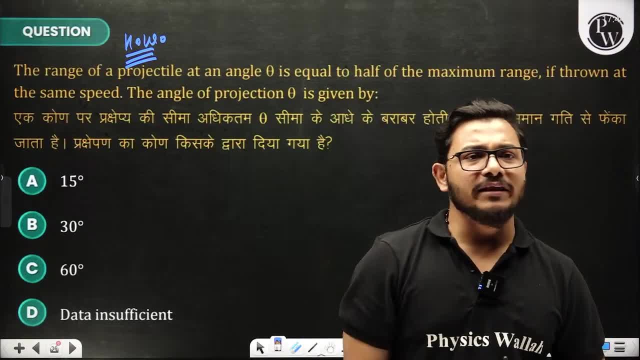 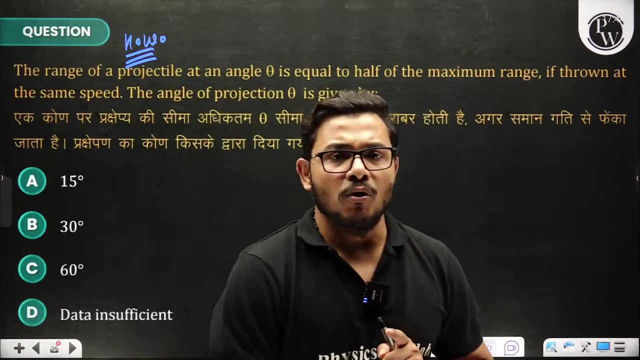 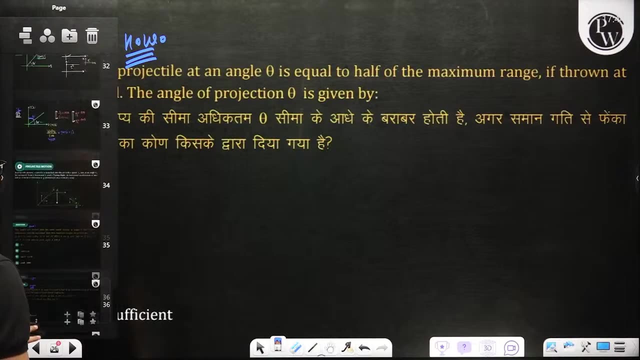 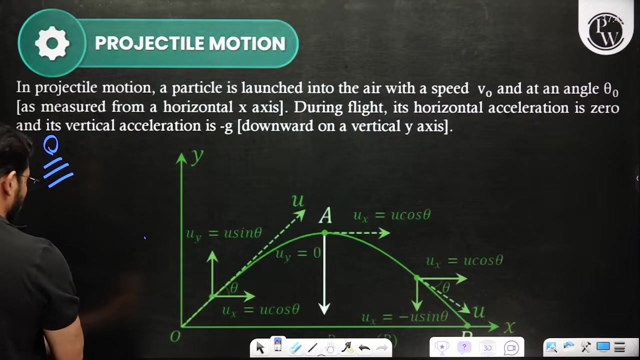 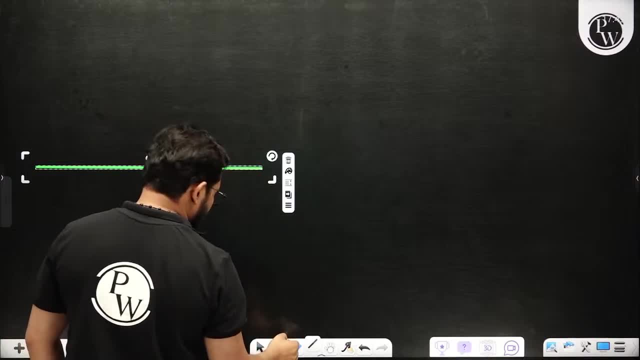 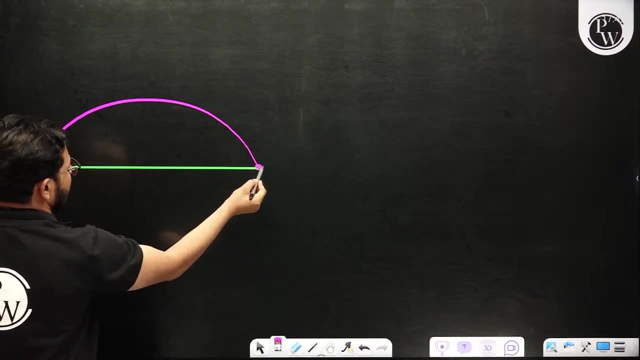 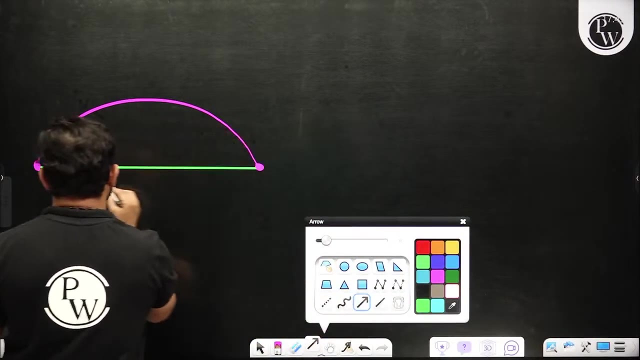 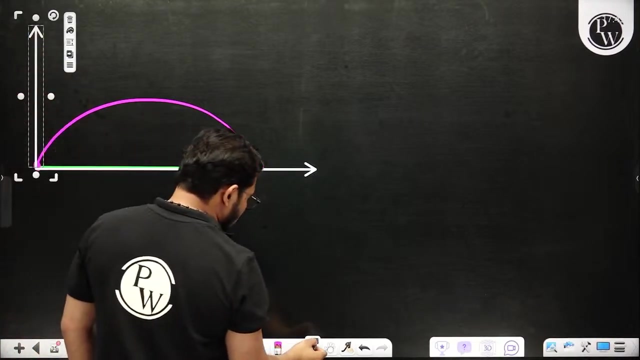 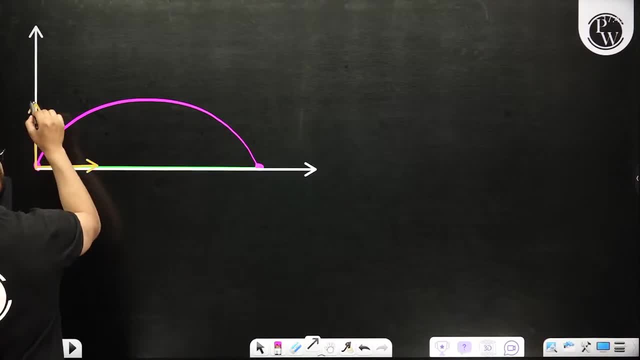 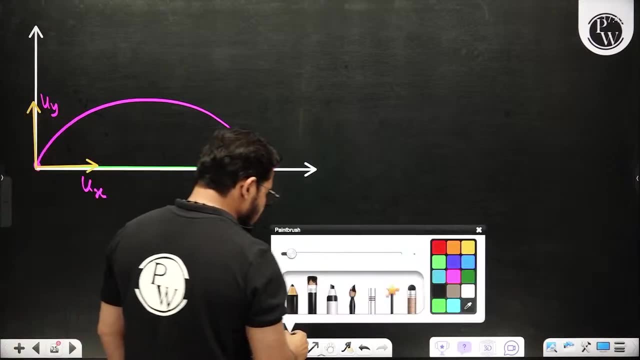 one component will be horizontal and one component will be vertical, and the horizontal component will be Ux and the vertical component will be Uy. so if I ask you in any question that, what is the value of the flying time? so the value of the flying time will be tf. 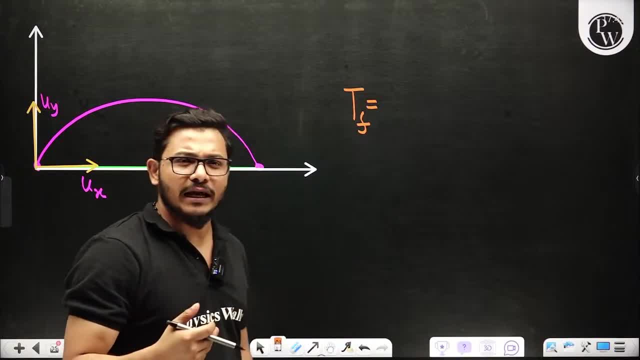 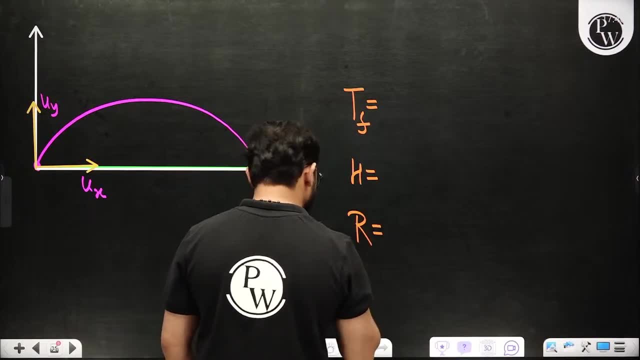 so what is the value of tf? what is the value of tf? so in this case, you have to calculate this and write the maximum height formula and write the range formula: maximum height and range. what is the meaning of range? this is the range that you have calculated. 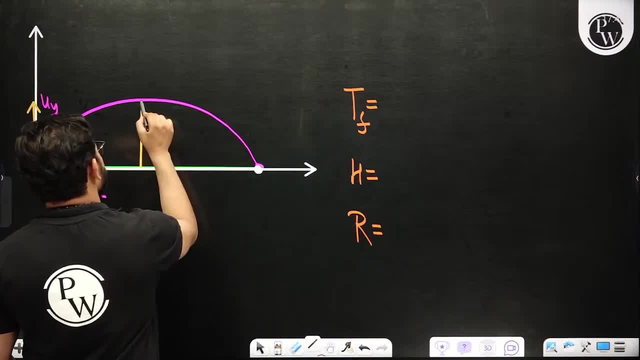 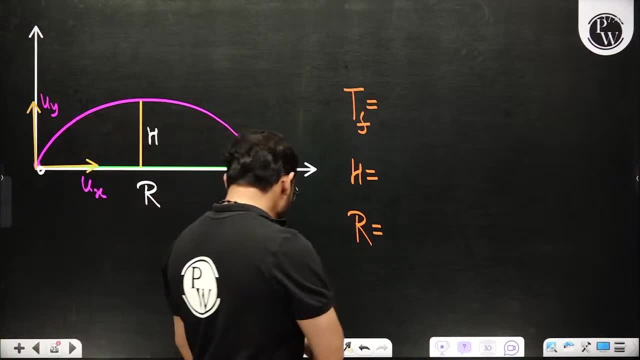 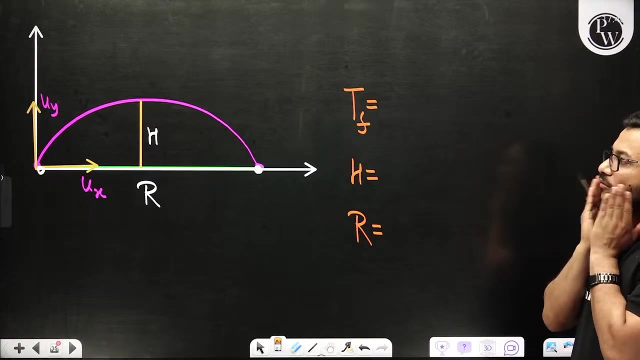 and this is the maximum height that you have written. that one is capital H and this is capital R for me. so when I write the range formula, I will write the formula of flying time. what is the value of the flying time? so how will you calculate the value of the flying time? 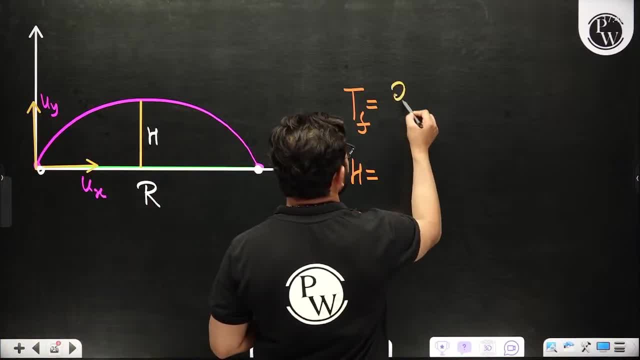 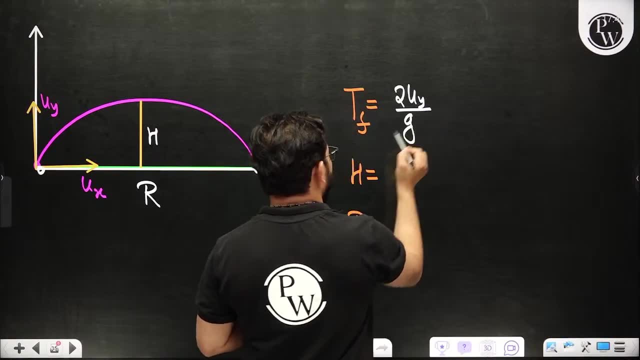 what is the value of the flying time? so the value of the flying time will be 2 time of. keep on listening that. 2 time of Uy and into g, that is all. and what is the formula of maximum height? Uy square, and upon me 2g. 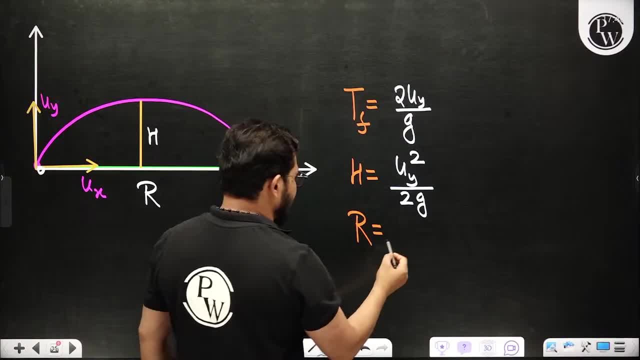 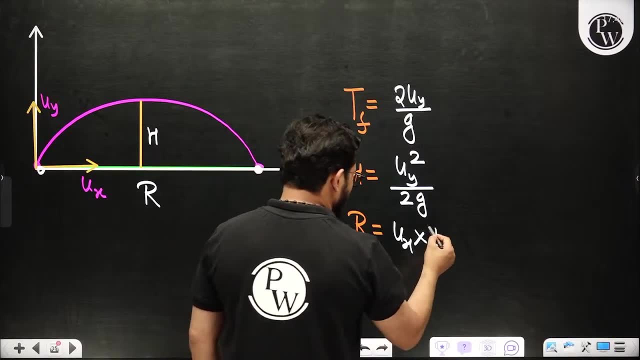 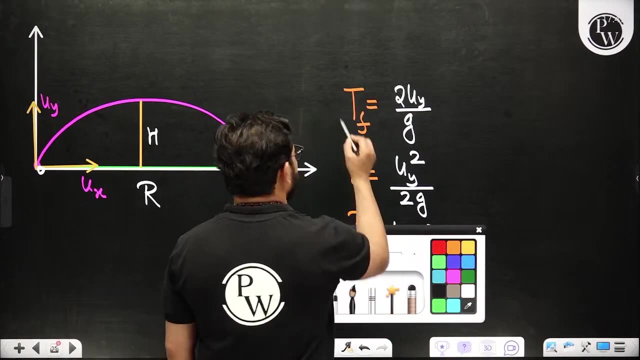 did you understand? and what is the formula of range? range becomes equal to Ux and into tf. that is all you have to remember. Ux into tf, Ux into tf. distance becomes equal to velocity into time, into tf. these are the three formulas. you should never forget these three formulas. 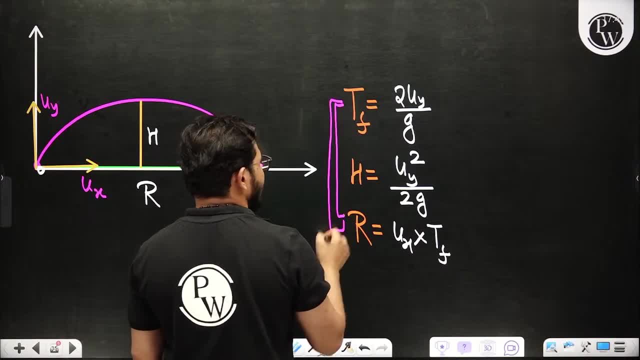 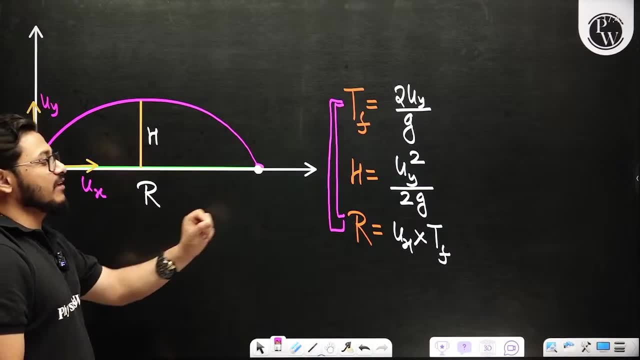 that is all. the flying time becomes equal to t, is equal to 2 Uy upon me, g, and maximum height becomes equal to Uy square upon me, 2g, and range becomes equal to Ux into tf. if I talk to you here, suppose you have taken the velocity of a particle as U. 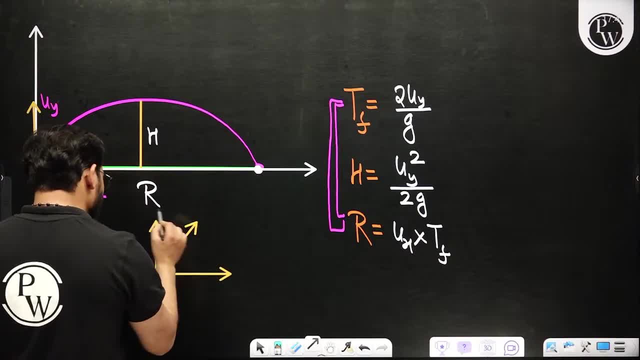 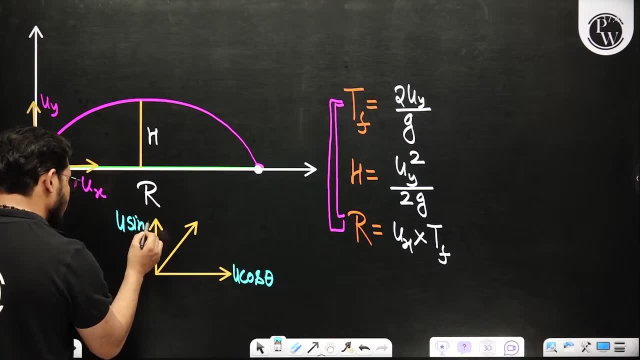 and at the angle theta you have taken its two components: one component, Ux, you have U cos theta and you have Uy, which is U sin theta, U sin theta, and that one is the U and this angle is theta. so if you want, you can put the value here. 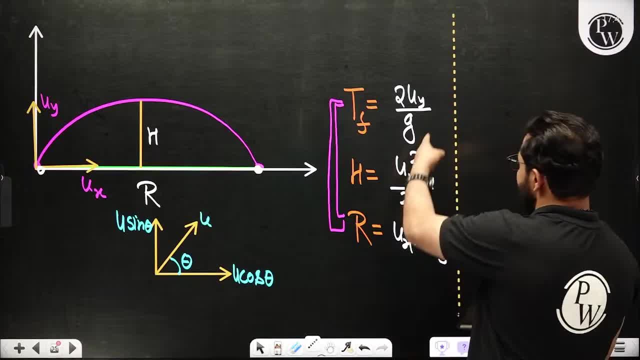 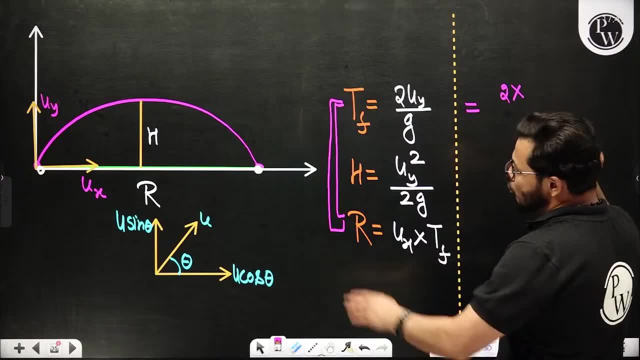 I think it is easy to remember the terms, so you don't have to do anything, you just have to put the value here. when you put the value so to Uy. so what is the value of Uy? U sin theta upon me, g upon me g. 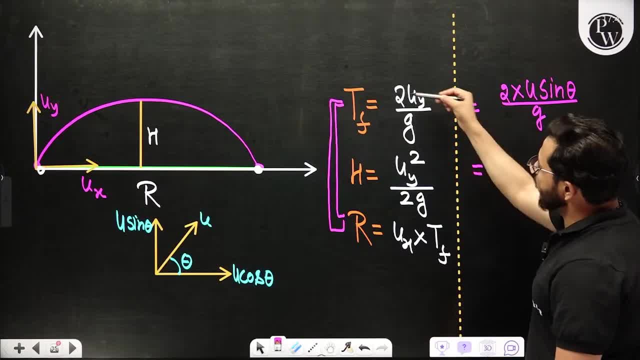 now, when you wrote the maximum height formula. so you subtract 2 and take it up, so Uy power becomes 2, so U sin theta becomes square, and what becomes upon me, upon me becomes 2g, upon me becomes 2g. ok, guys, did you understand? 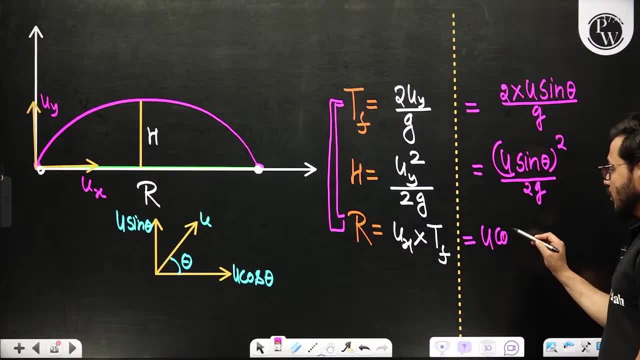 upon me becomes 2g. very good, what is the value of Ux U cos theta and what is the value of tf 2 U sin theta upon me g. now you do one thing: this 2 sin theta into cos theta becomes sin 2 theta. 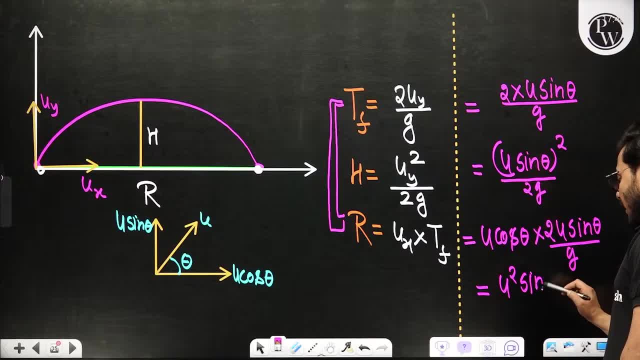 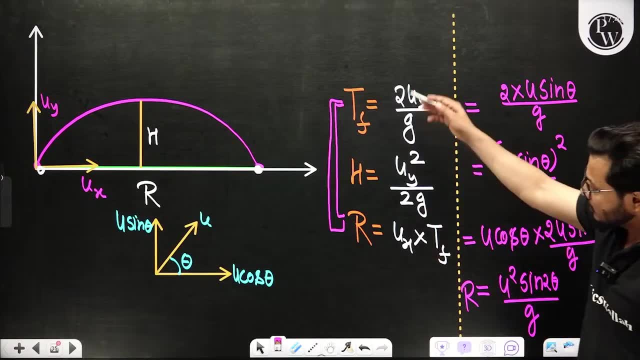 so the answer is U square sin 2, theta upon me g. so you can write these formulas of range. so I think that you don't have to remember these formulas. so that's why you remember these 3 formulas, that one is the one concept and in the same way. 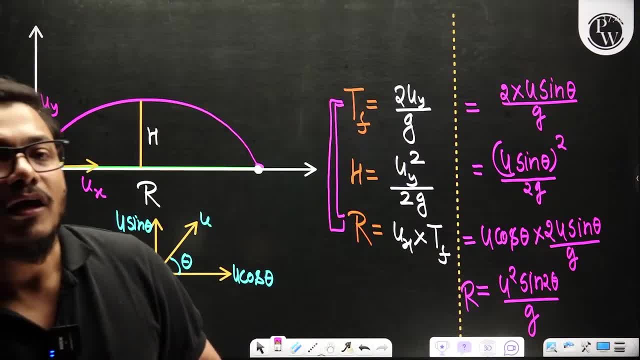 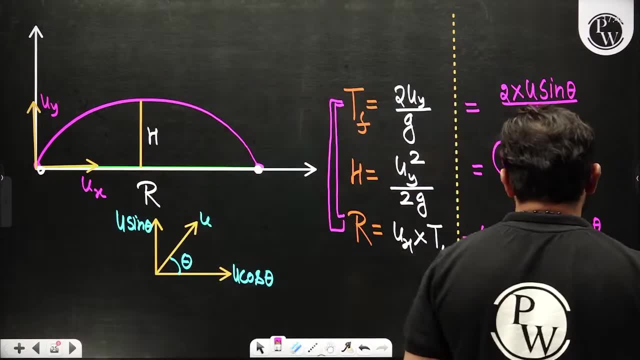 you will know the answer of the question. the answer of the question which I gave the homework question yesterday in the group. the children had already sent the answer. you check in the group. Subham sahb, are you not in my group? go and check in the group. 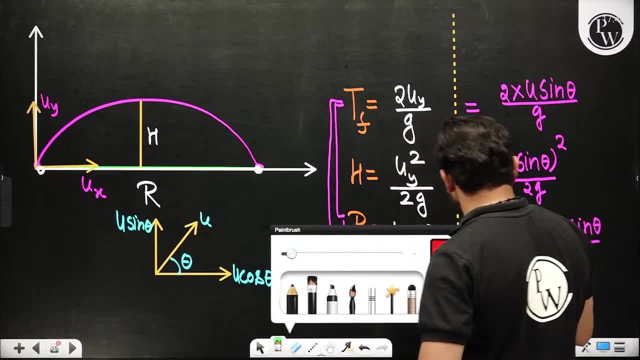 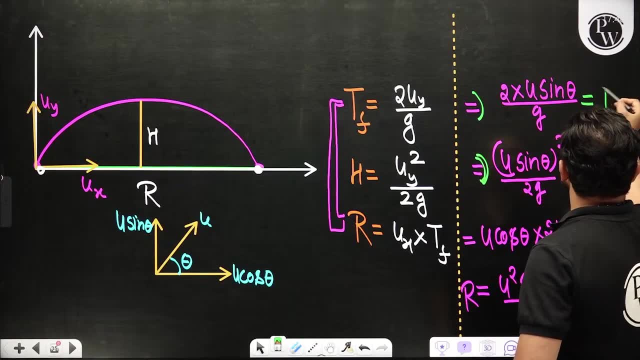 I chat with you so much in the night and in the night I sleep at 11 am and I sleep by chatting with you. I keep watching all the things. I keep telling the questions of all the children in the answer that: what are you asking me? what is going on? 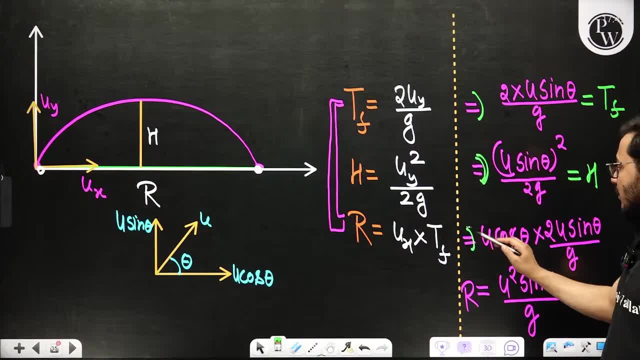 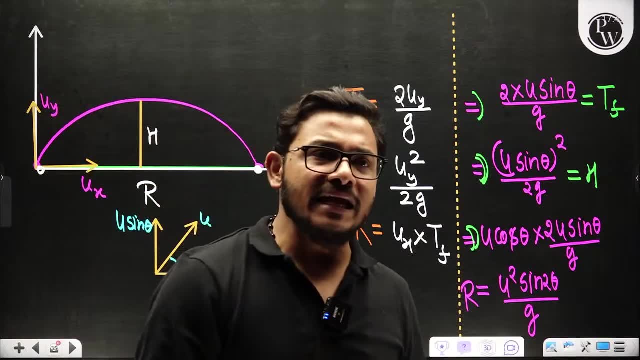 I tell the answer of all the children and in the night I replied till 11 am to all the children. you know that till 11 am I have replied. so the answer of that question. and where will you get the pdf? pdf. go to the pw app. 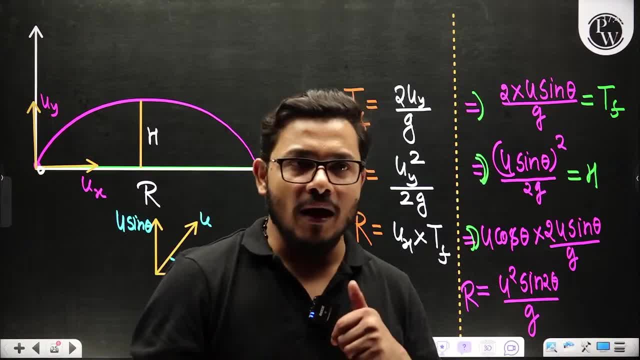 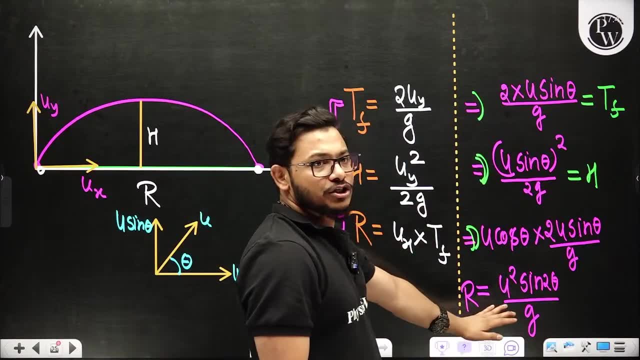 there you will get join in the group. all your questions, all the answers query, all the answers solution you will get in the group so that one is called the flying time maximum height and range, that one is called the projectile motion. did you understand? as this is my question, 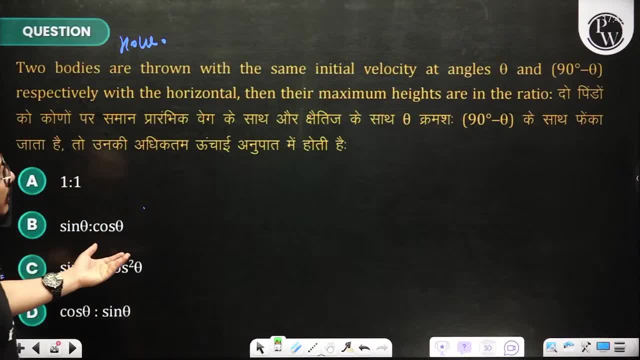 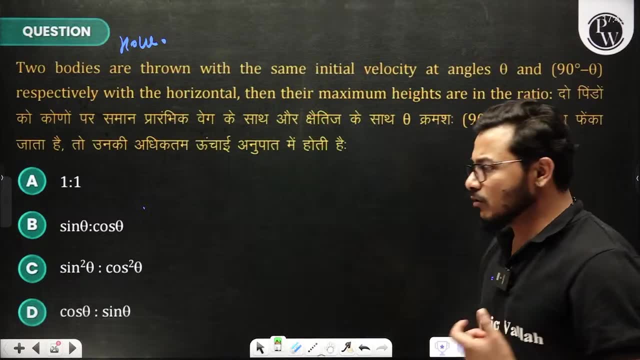 please see this question. in the question he is saying that this is homework. you can do it. if you don't want to try, then I will tell you. if you don't want to try, then I will tell you, because if I tell you then it will be a problem. 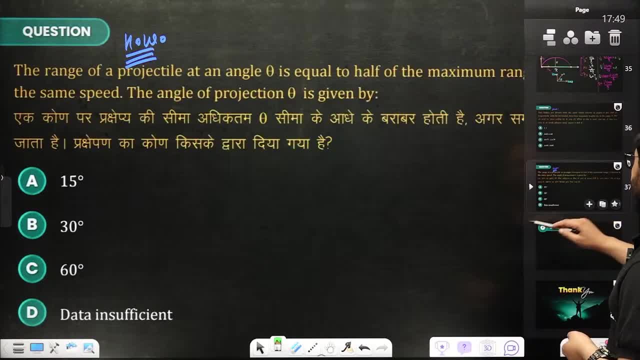 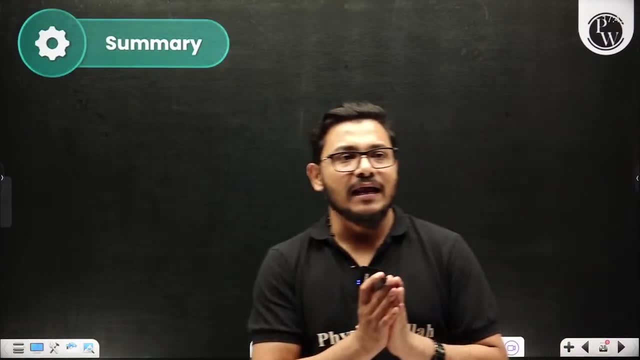 ok, so in the class- I will finish here, there is another class for you. you can solve this question, you can do it, you can do it, you can do it. so do you have projectile motion and everything is clear for you? yes, 40, root 2, my husband told me. 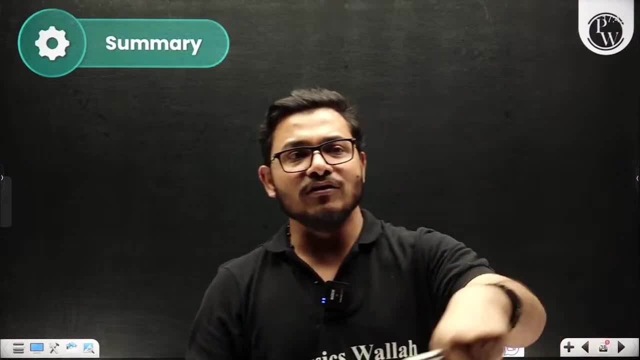 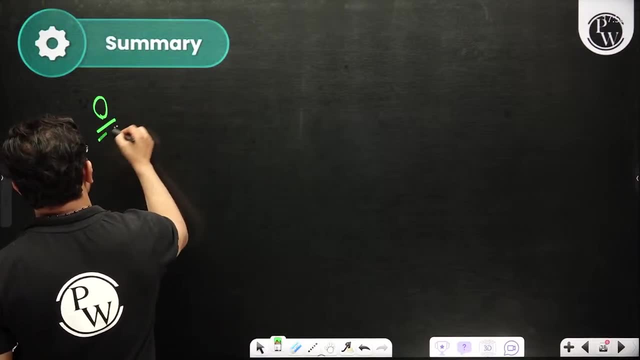 now my husband told me the correct answer. it was 40 root 2. maybe in the group some kid had sent me 40 root 2 answer. ok, so in today's class we will finish this topic here and you all must have understood everything. so I have. 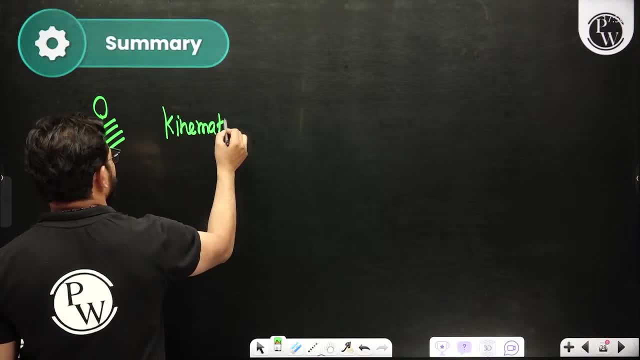 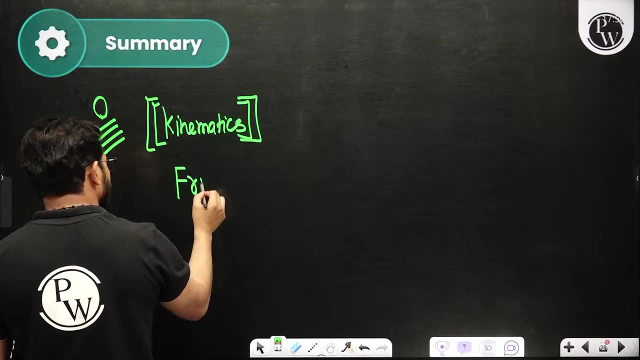 finished kinematics. you have to study only this much in kinematics and nothing else. and listen to me, do you know what I will study in tomorrow's class? don't miss tomorrow's class. I will teach friction in tomorrow's class and remember in your exam. the question is out.